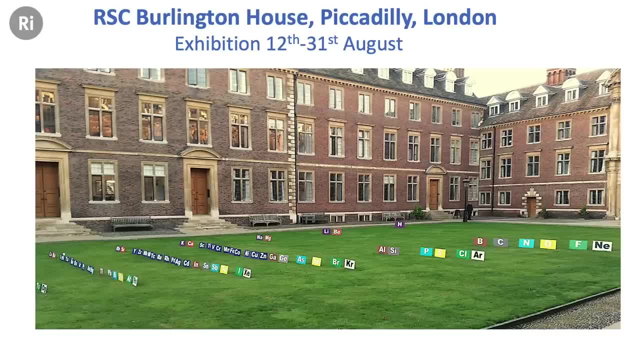 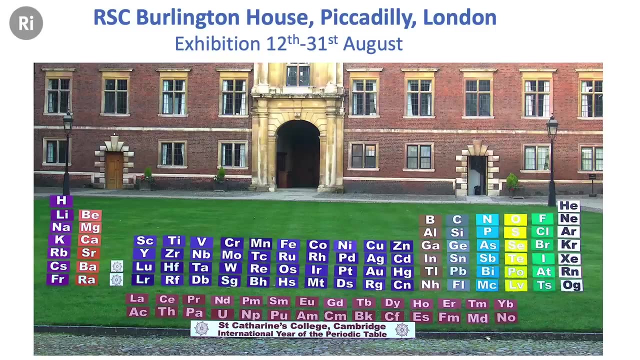 actually set out on the grass and they're all different sizes and all placed in exactly the right position so that when you stand in just the right place, order comes to the elements there. and it looks like that. So this was really a photograph that was taken. 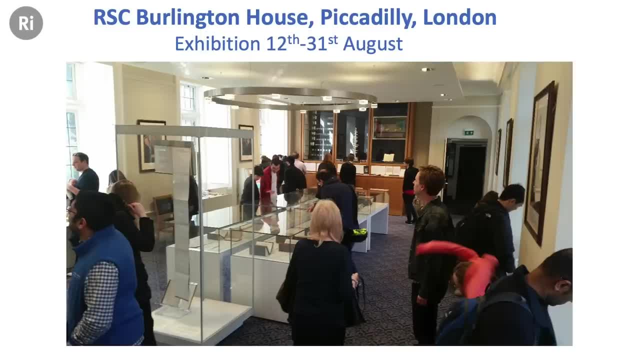 This is inside the exhibition. as I say, Do go and see these things when they come to the Royal Society of Chemistry, to Burlington House. There's all sorts of different forms of periodic tables on display, In fact the long chart in the tall cabinet. 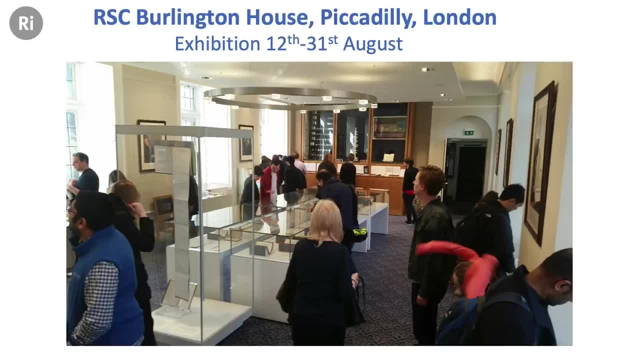 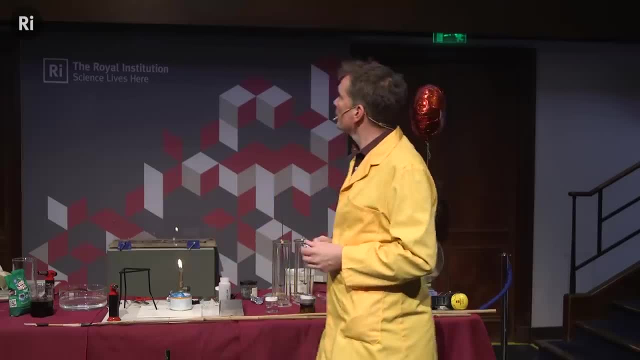 there is the very, very, very first periodic table, which is really quite exciting and very different from the ones, But hopefully after today you'll understand what makes a periodic table And they can look quite different indeed, And this is one that was donated to the college commissioned. 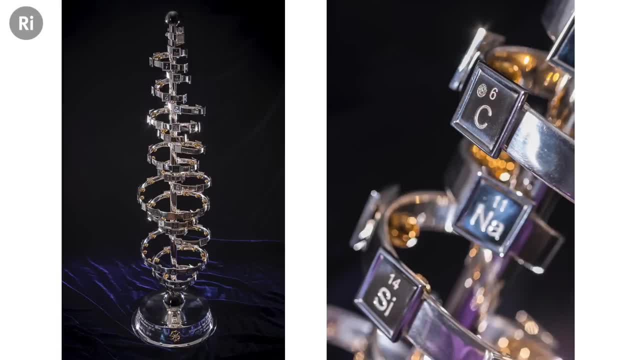 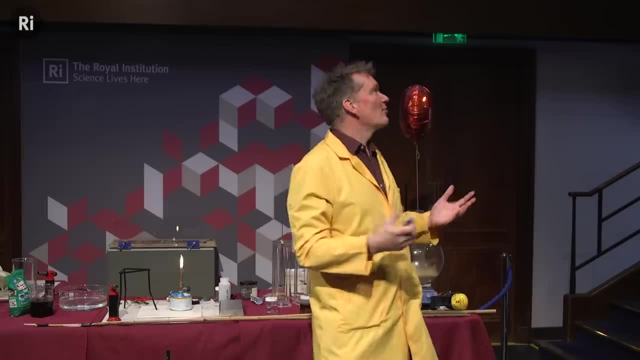 for us for this year, for the International Year of the Periodic Table. It's absolutely fantastic. It's made out of silver And it really is a periodic table, But it looks very different from the versions that we're going to be looking at today and we're familiar with. 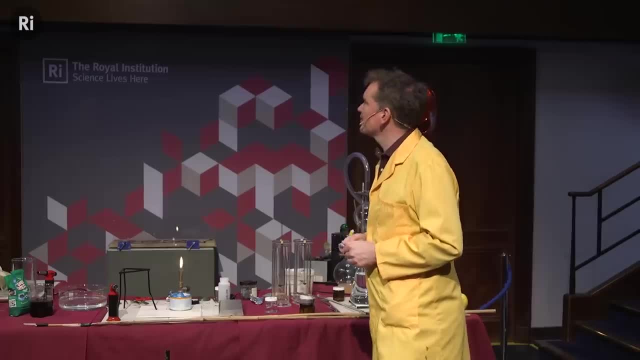 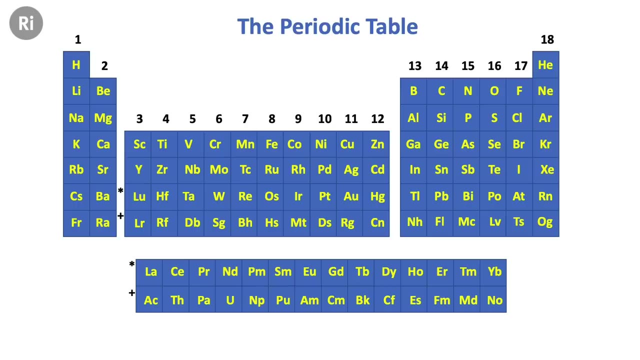 But nonetheless it still works. So go and check this out if you get a chance in August. Well, we're going to be sticking with our more familiar form, But we need to understand exactly what it is that makes a periodic table and how it works. 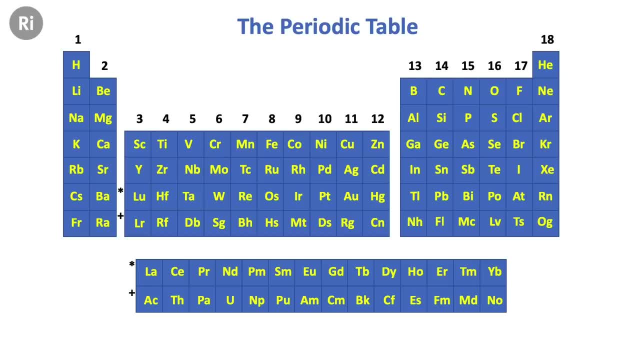 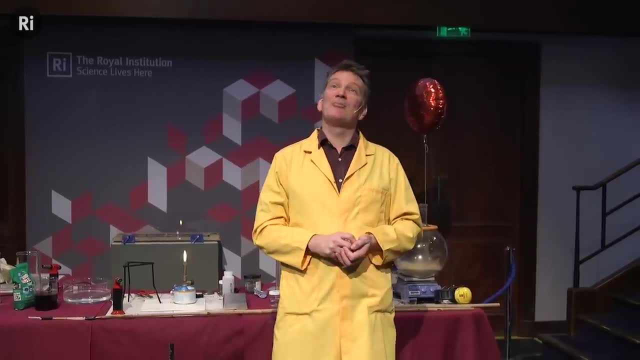 And in order to do this, we need to understand the very structure of the atom itself, of what all atoms are made of. Now, as far as a chemist is concerned, atoms are made of just three, Three things. We have positively charged protons. 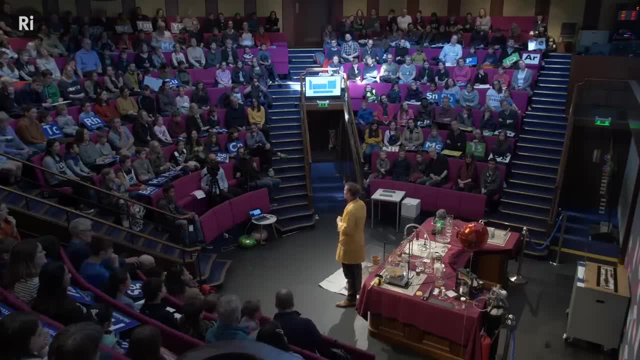 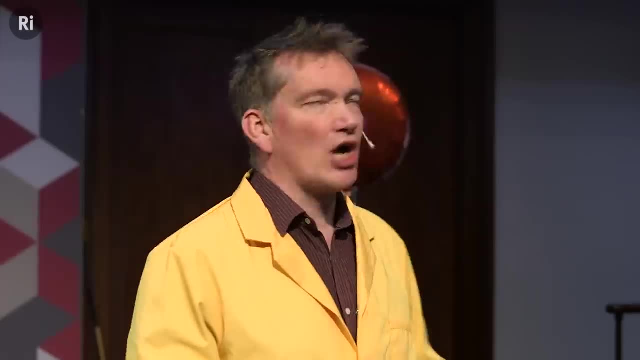 in the heart of the atom, in the nucleus, And sometimes, well, almost always, apart from one atom, we have neutrons which have no charge at all, And then, whizzing around the outside, we have negatively charged electrons. And so long as it's a neutral atom, we have the same number of positively charged protons and negatively charged electrons. Physicists, of course, love smashing things up even further and breaking everything, But we're not going to be concerned of what we could smash. 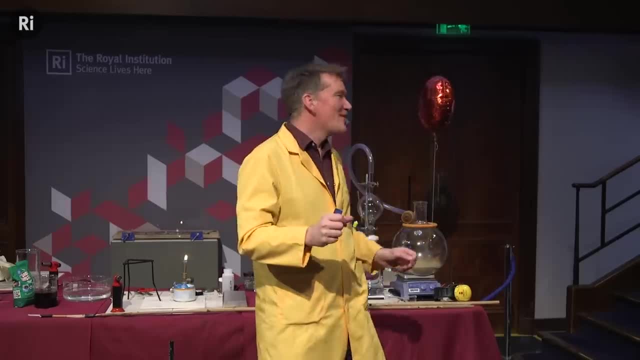 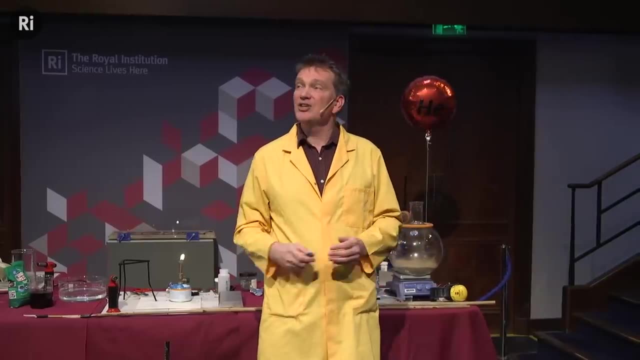 those things up into, into quarks and things, all sorts of nonsense like this. We're just going to stick with our lovely protons, neutrons and electrons. So let's go then to the very very first atom. 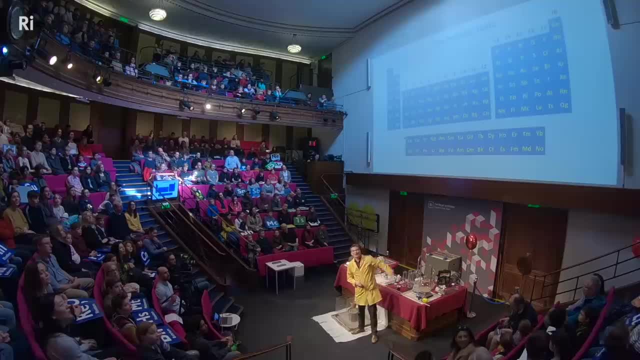 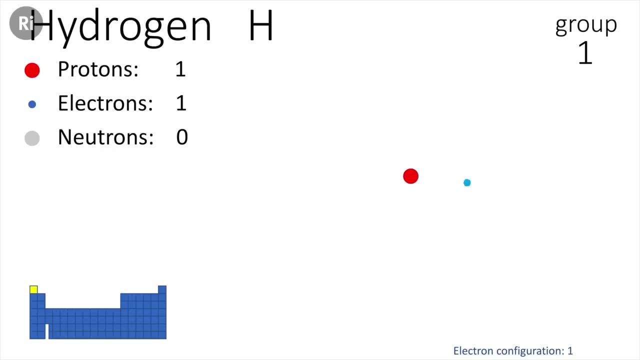 And this is hydrogen. So where is hydrogen Right at the top there? very good, So you are atom number one, the first atom in the periodic table, the first element, And what makes you unique and different from every other one is that in the heart of the nucleus. 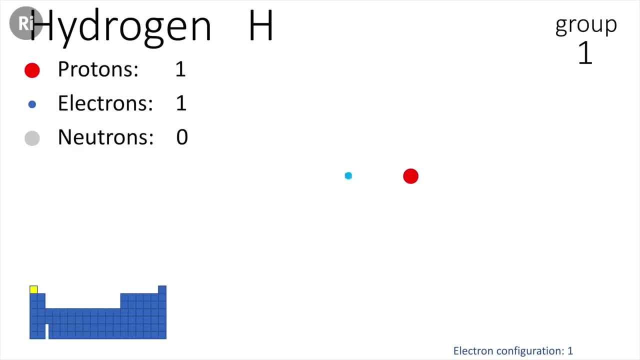 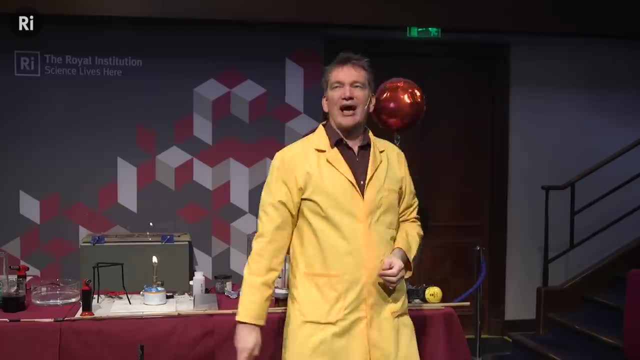 you have just one proton. That's what makes a hydrogen atom, And in the neutral atom it's balanced by the electron- one electron whizzing around there. So this is what we see When we go to the next atom. well, 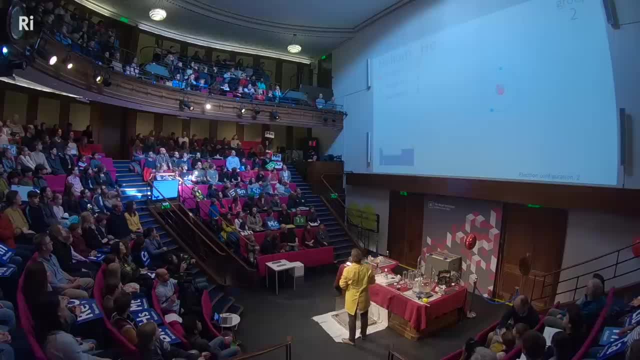 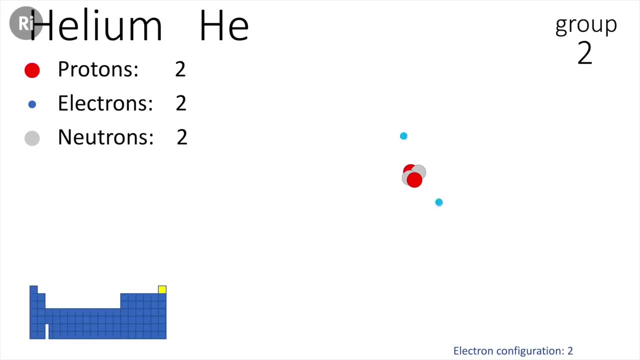 this is the element helium. So right the way over here. very good, helium. OK, so there's helium. Well, helium now has two protons in the nucleus. It happens to have most of the helium that we come across also happens to have two neutrons. 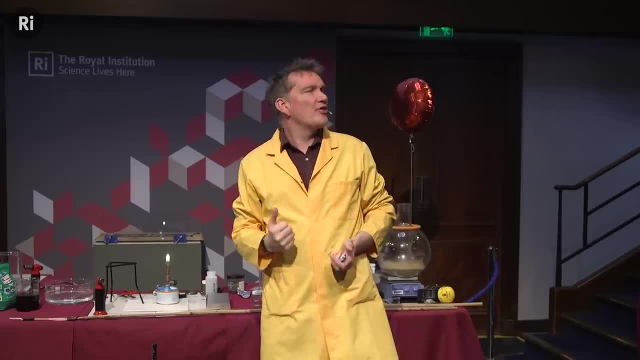 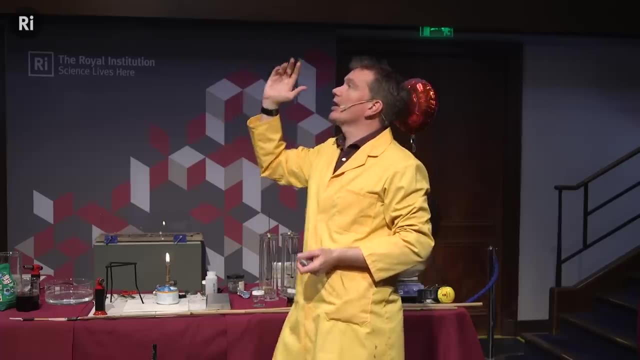 We're not going to be interested in neutrons. They increase the mass of the atom, of the nucleus there, But they don't really alter its chemical properties. But what makes helium special? What makes helium special is the fact that, unlike hydrogen with only one proton, helium has two protons. 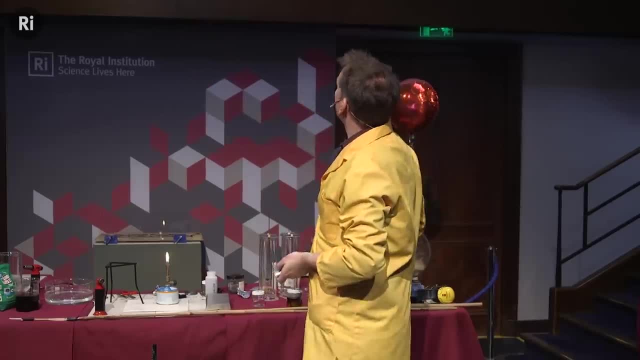 in the heart of the atom, balanced by, in the neutral atom, two electrons whizzing around. And then we come to atom number three, which is all the way back over here again, which is lithium. Oh, you're already there. 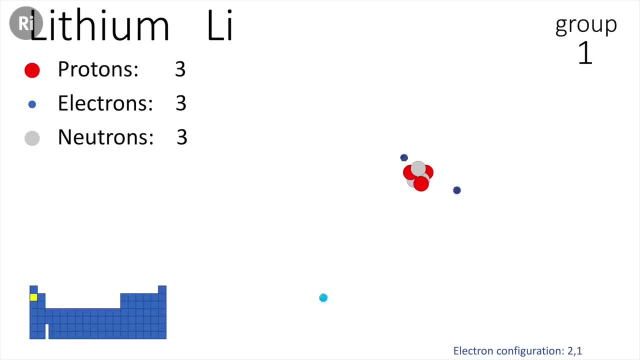 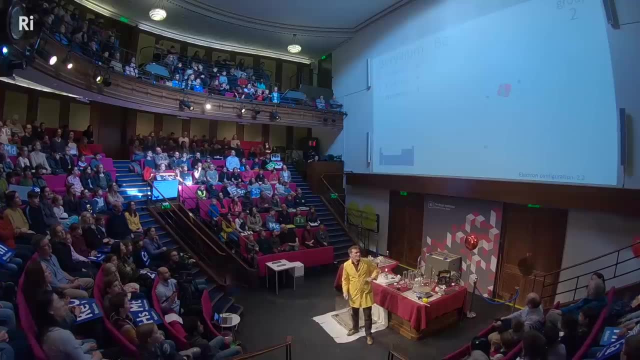 Look at that. OK, very quick. So element number three here: lithium. three protons in the nucleus there. OK, now we're going to move across. So element number four is beryllium. OK, so, four protons, four electrons. 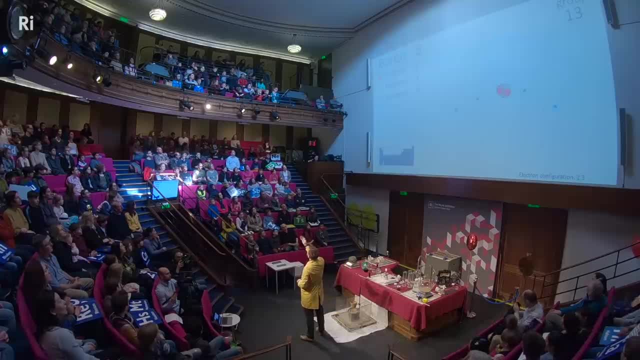 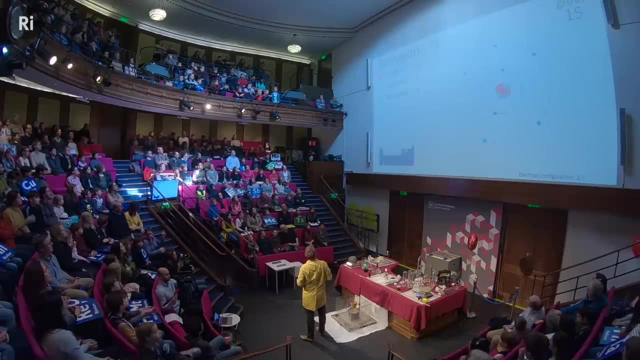 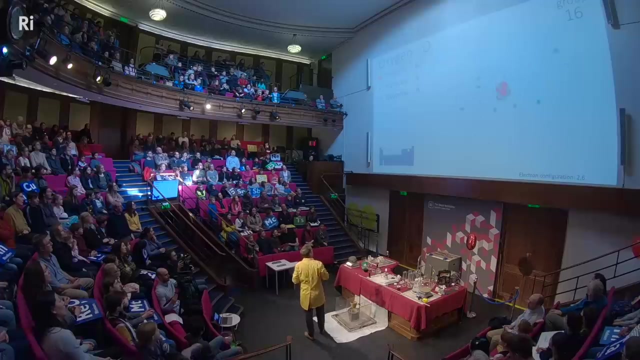 Then we come back over to this side With boron, five protons, five electrons, Carbon six- OK. then we have very good carbon Nitrogen with seven- OK. oxygen eight. So each time we're increasing by one proton. 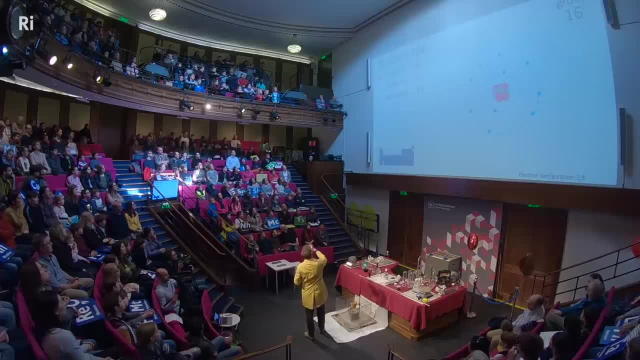 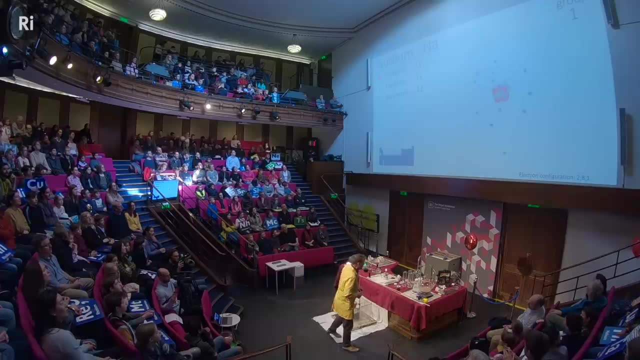 Fluorine, here with nine, And then neon 10. And then we come all the way back to this side And we come to the element sodium, number 11.. Very good, OK. well, so far, so good. 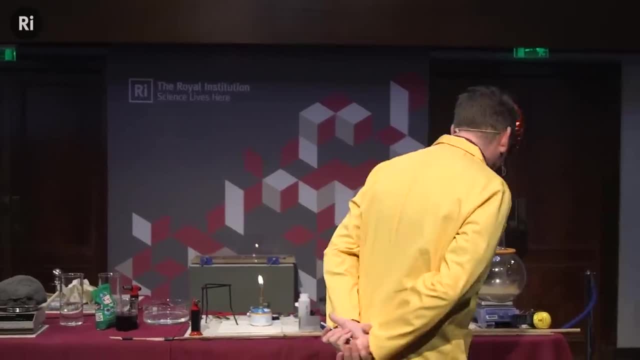 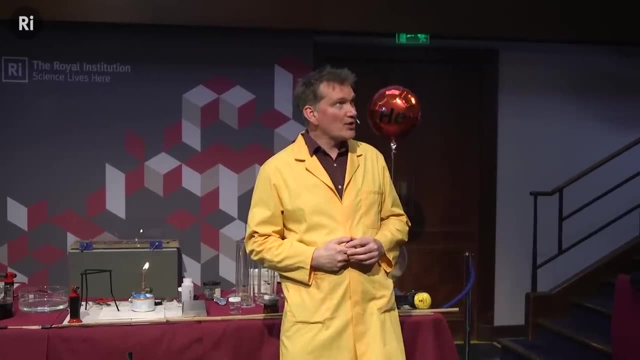 Now I'm not going to go. I'm going to go through all 118.. That would be just a little bit tedious. But this is the underlying order. It is the order of their atomic number. This is the number of these positively charged protons. 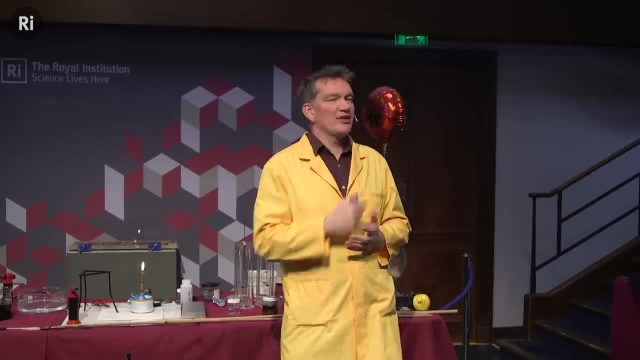 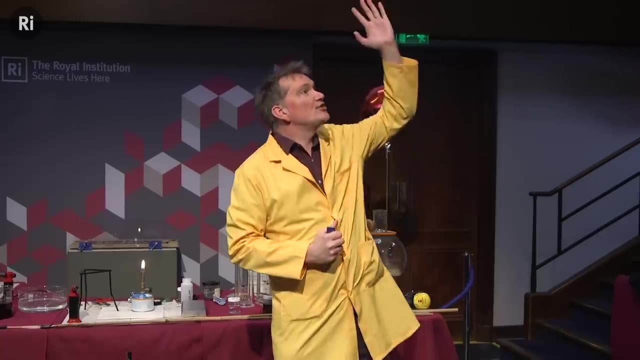 in the heart of the atom. But there's more to a periodic table than just having them arranged in order. We also need to group the elements that have similar chemical properties in these vertical groups. This is really important, And this is what any periodic table must achieve. 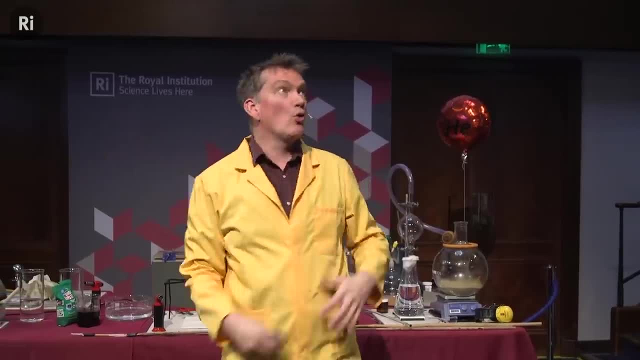 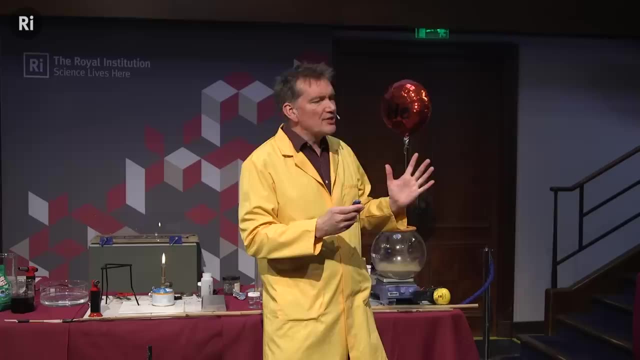 So we've got this underlying order as we move from one element to the next, where always each atom is getting heavier And we're adding more protons and electrons. But we also need this order with the similar properties, And this is what we're going to look at now. 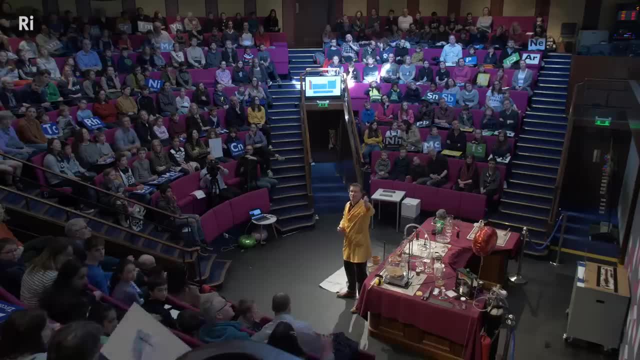 So let's have a look at group one. So these are all the purple ones. So if you're a purple, we've got a purple card. Hold it with a card. OK, well done, Very good. So these are the group one elements. 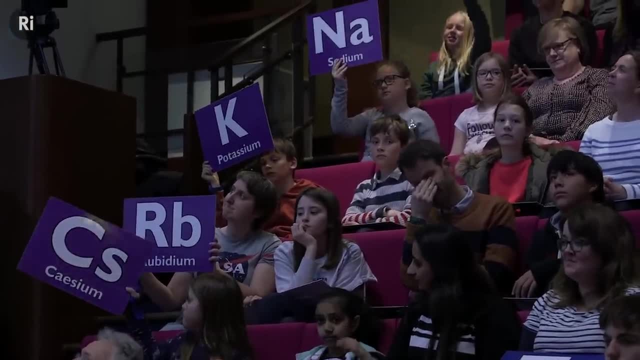 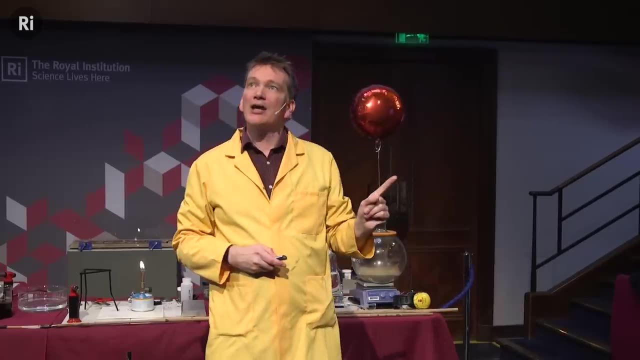 Now what they all have in common in terms of their atomic structure- and we'll see some of their chemical properties in a moment- But what they all have in common is that they all have just one electron in their outermost shell. Of course, hydrogen only has one electron anyway. 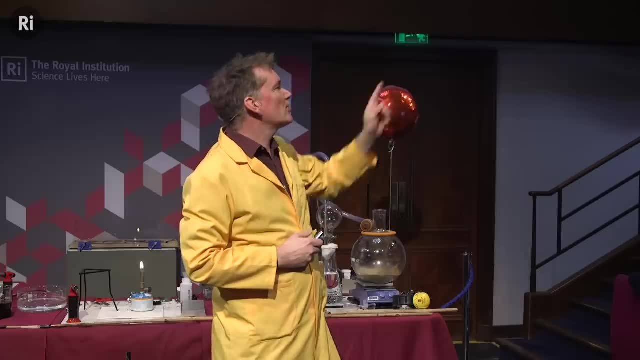 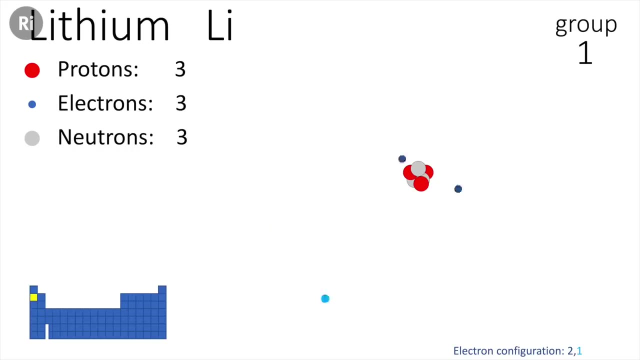 But then all of the others have one in their outermost shell. So let's look at lithium again. Lithium has, well, three electrons in total, three protons, But there's one in the outermost shell. there, When we come to sodium, more electrons. 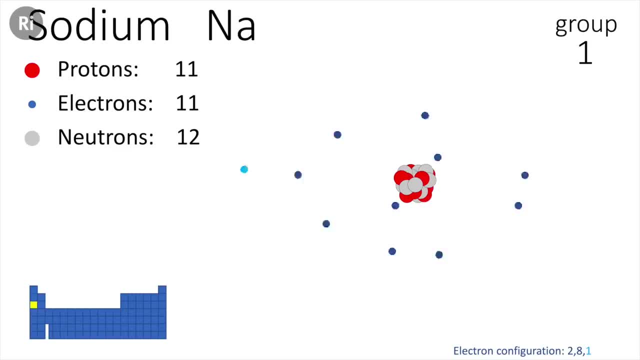 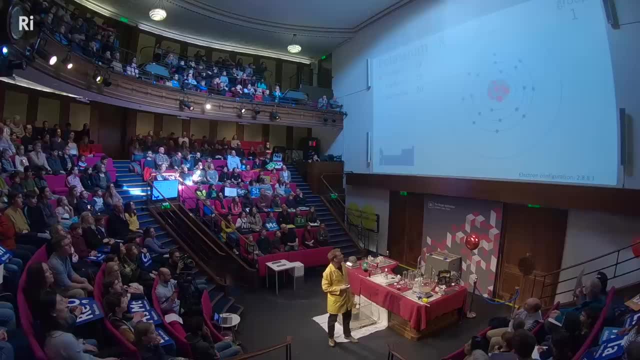 But there's still one in the outermost shell And it's relatively easy to lose that one electron, And this gives it similar properties to lithium And in some ways even to hydrogen. Then keep on going, potassium, So the nucleus in the heart of the atom there. 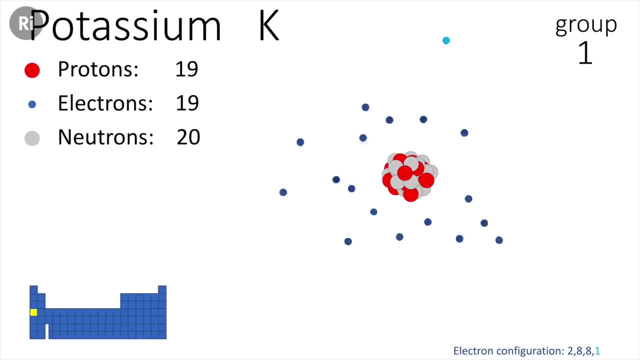 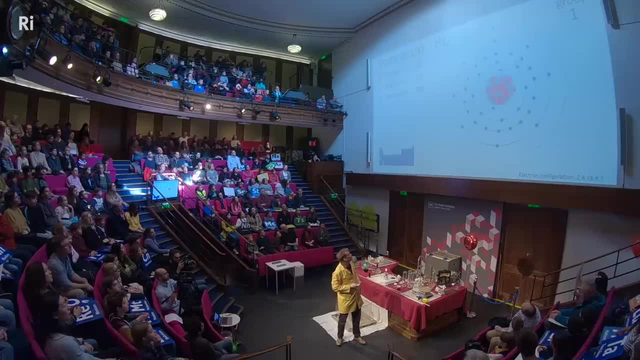 is getting much bigger and heavier. The atoms are getting heavier, But there's still one electron right in the outside there whizzing around, which gives them all similar properties. Let's go to rubidium, Getting pretty massive now. Loads of electrons. 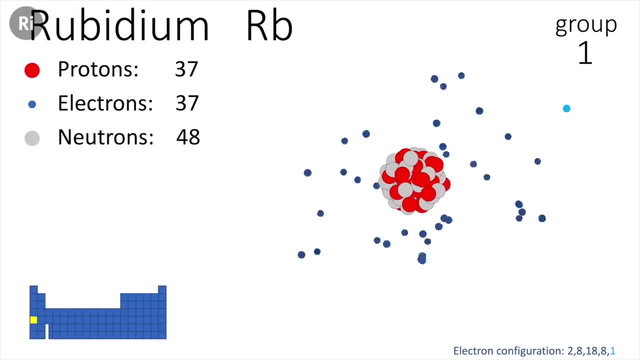 But there's still the outermost one And we get to cesium. Really crazy craziness going on now. But there's still that one. There's still that one electron whizzing around. It's quite away from the nucleus. 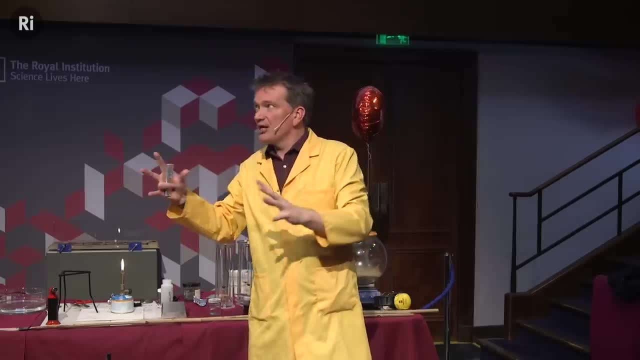 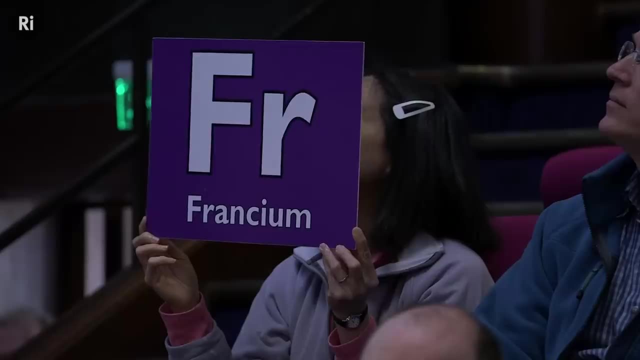 It means it's quite easy to remove that one electron. That is what gives us its chemical properties, And we'll look at these in a moment. But they all have something similar there. There is, of course, francium, the heaviest element. 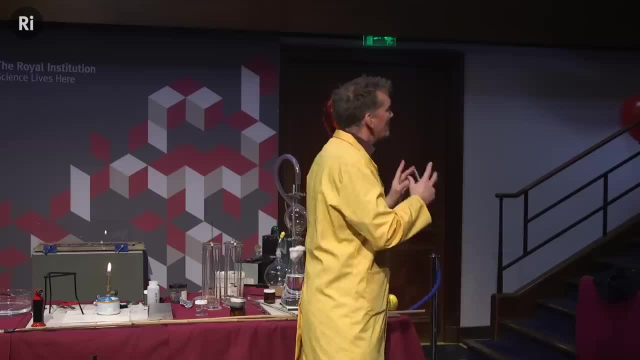 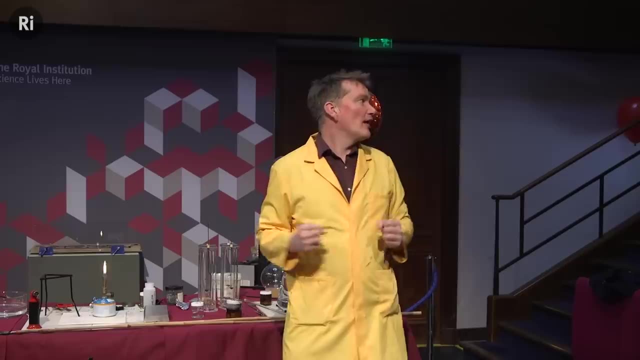 in this group. I'm not going to show francium because there would be too many electrons, But also because actually francium, I'm afraid, falls apart quite easily. This is where, well, for the very heaviest of elements. 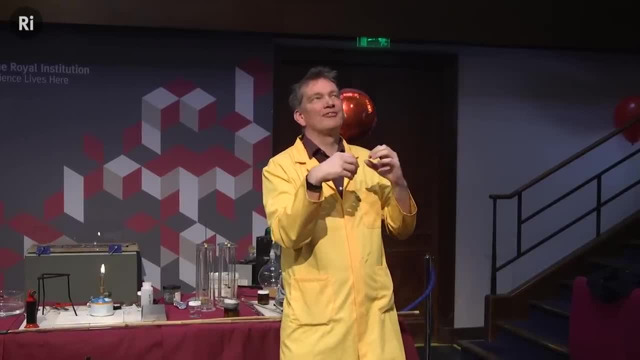 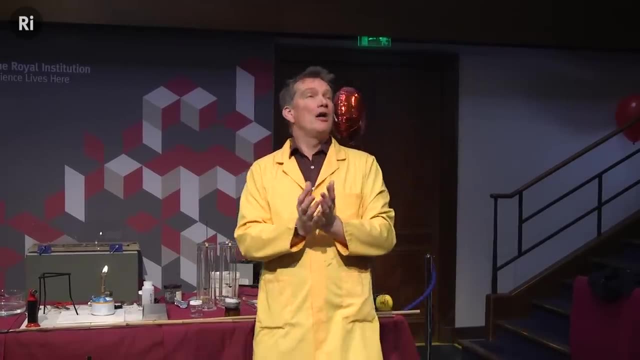 the nuclei are getting so large, But basically bits fall off. essentially, This is actually radioactive decay. What happens is, for instance, we could lose two protons, two neutrons. This is the heart of a helium atom, essentially. 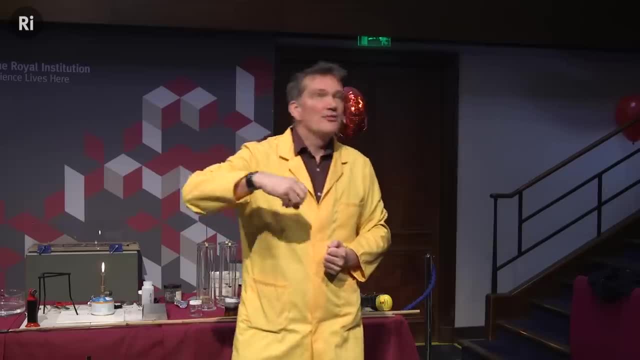 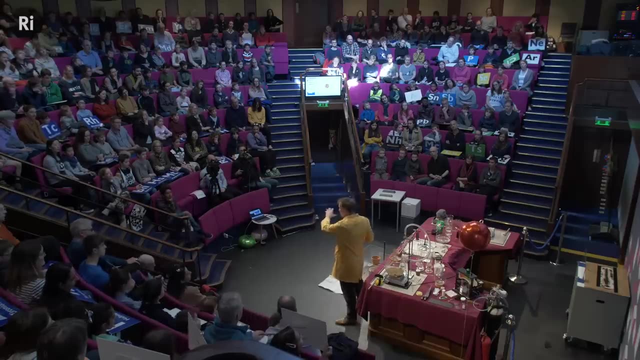 So an alpha particle is a helium nucleus. This can ping out And then it's changed into a different element. So this is why we're not going to be looking at the very, very heaviest elements in the groups there, because these are unstable. 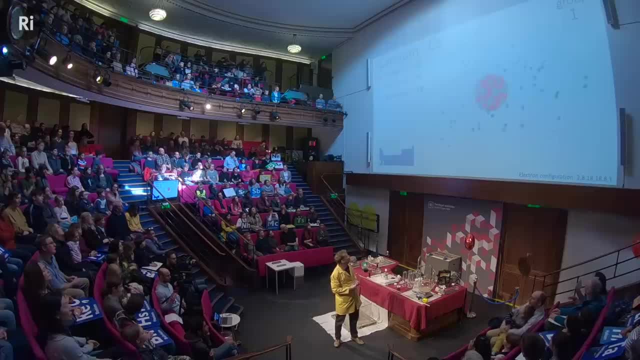 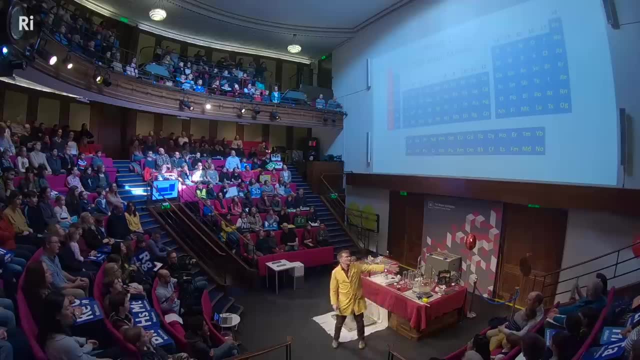 They are radioactive. So cesium is one that we can look at. It is stable, But it has this one All important electron whizzing around there. So that's our group one. So here they all are again. So let's just see group one again. 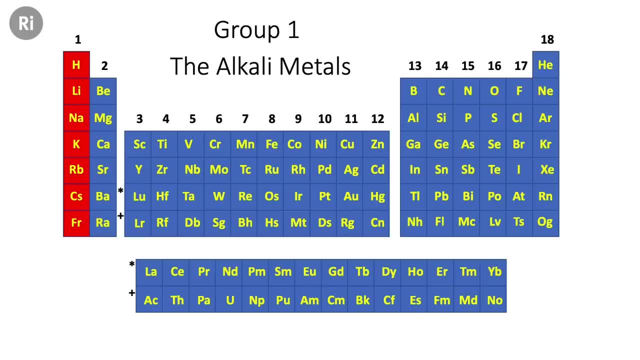 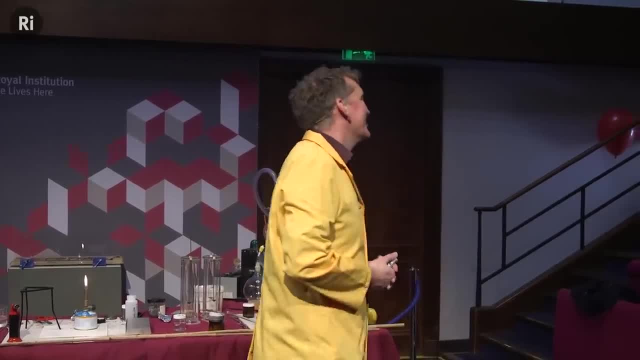 So all the purple ones all have one electron in the outermost shell. Then we move to group two. So group two, the orange ones. very good, We're very busy, aren't you? You've got two to do, yes. 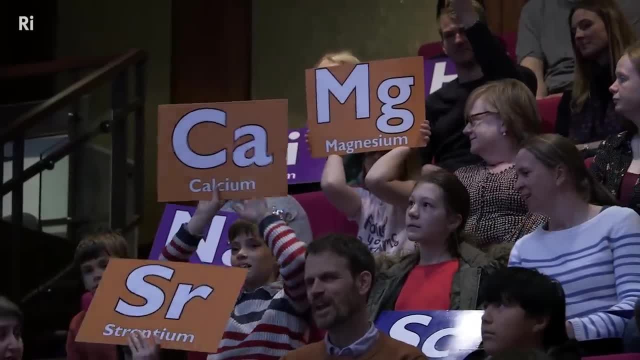 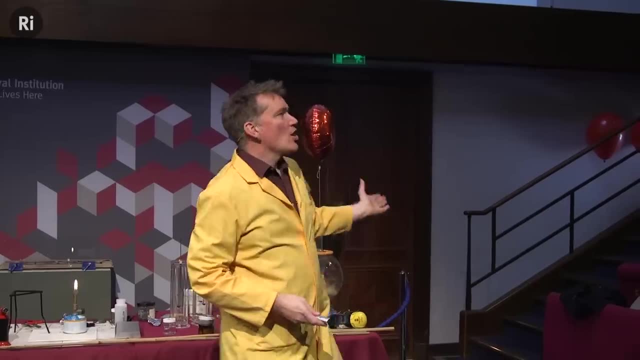 OK, so group two here all have two electrons in the outermost shell, And this gives them similar properties to each other, as we shall see, but different from those from group one. OK, we're going to move around all the way to here. 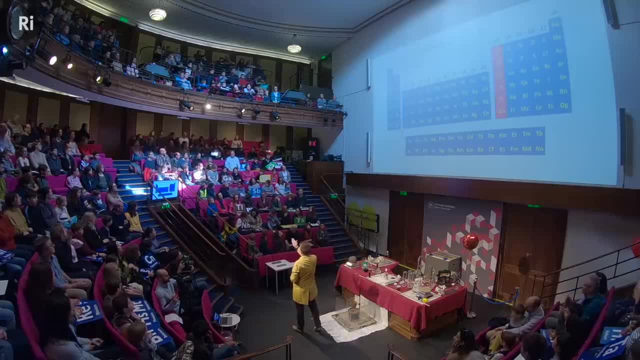 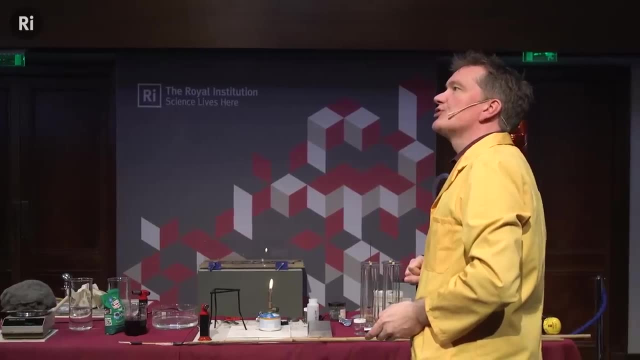 now to the brown cards. So these are group 13,. OK, or sometimes called group three, And there are good reasons for this. They all have three electrons in their outermost shell that they can use. OK, we come to group 14,, the dark gray ones. 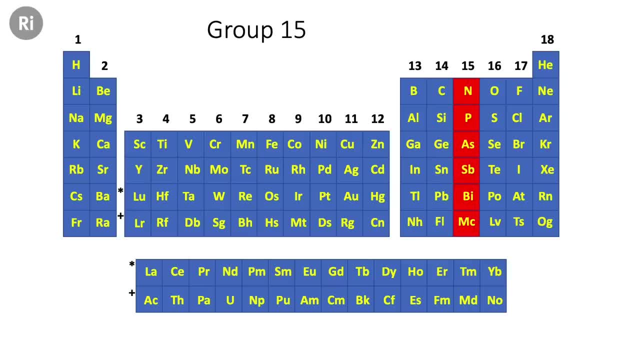 with four electrons very good. Group 15, the light blue: very good, All beautifully aligned, all with five electrons in the outermost shell. 16, the nice yellow ones, very good. Six electrons in the outermost shell. 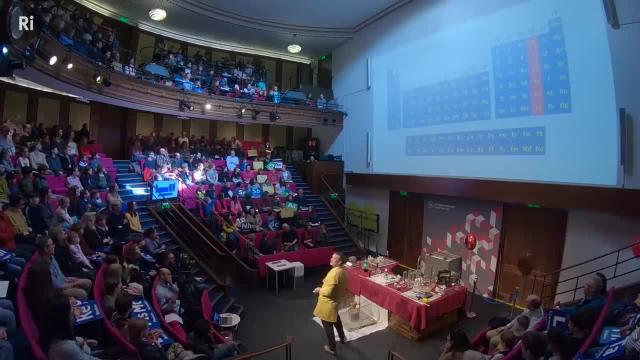 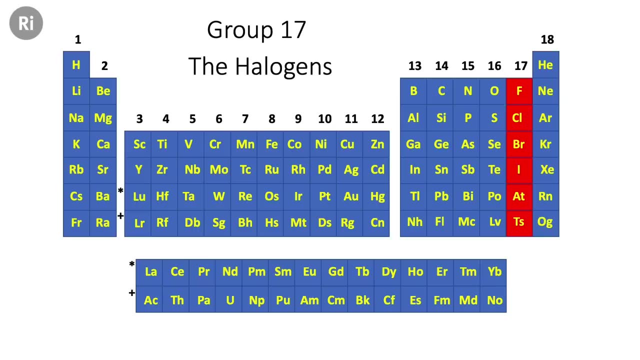 Sulfur's a little bit the wrong way up, but it doesn't matter, because it works either way. And then we have group 17.. I like these ones. These are the so-called halogens. We'll come back to those in a moment. 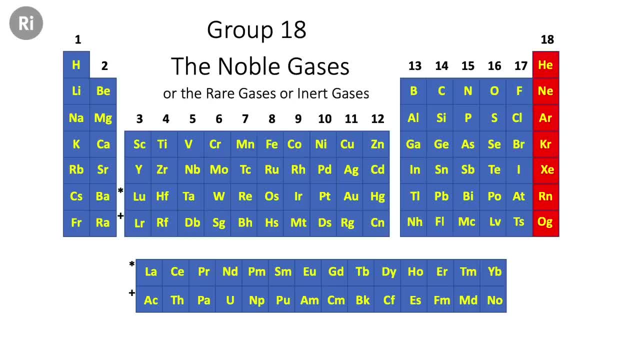 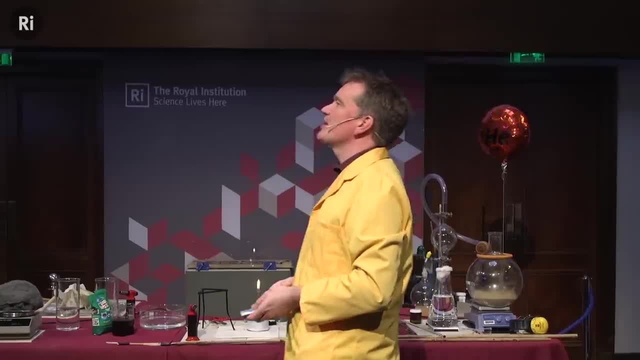 And then, right on the end, the final ones. here we have group 18, the so-called noble gases. OK, we'll come to those in a moment as well. Let's go back for a moment to the halogens, so the green ones. 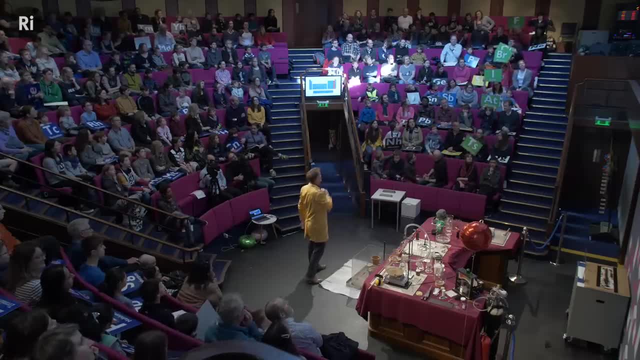 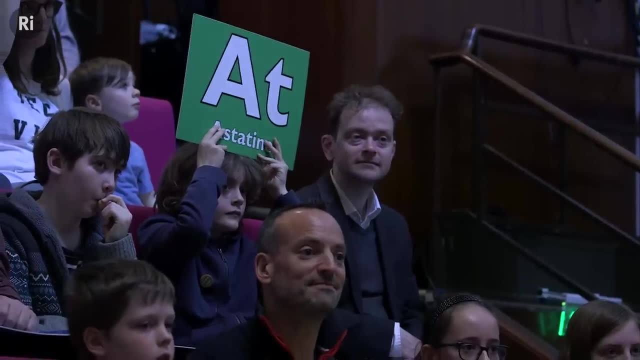 So just show us again our halogens here. OK, these are one of my favorite groups. These are some of the most reactive elements in the whole periodic table, So fluorine in fact, when this was first put into the periodic table, into Mendeleev's periodic, 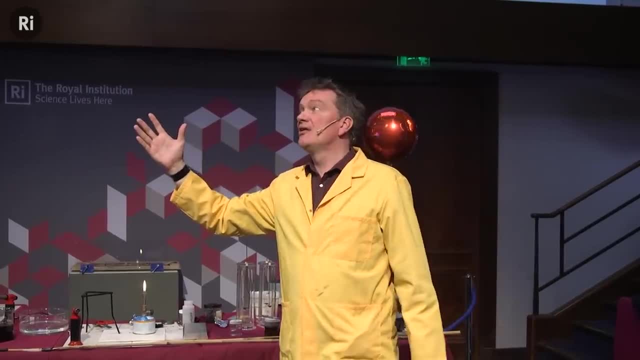 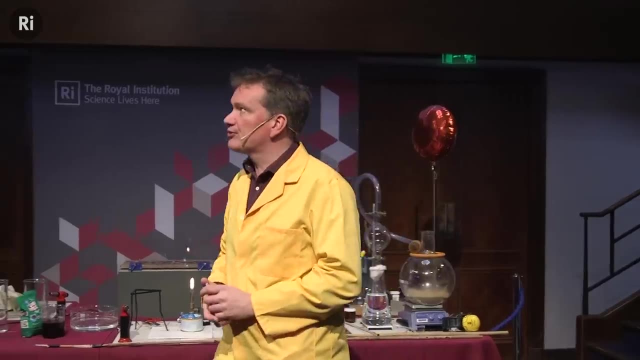 table. the element hadn't even been prepared yet. They knew it was there. It was in certain salts, so particularly calcium fluoride, and also the acid was known hydrofluoric acid. But nobody had yet isolated fluorine. In fact Humphrey Davy here tried to do this. 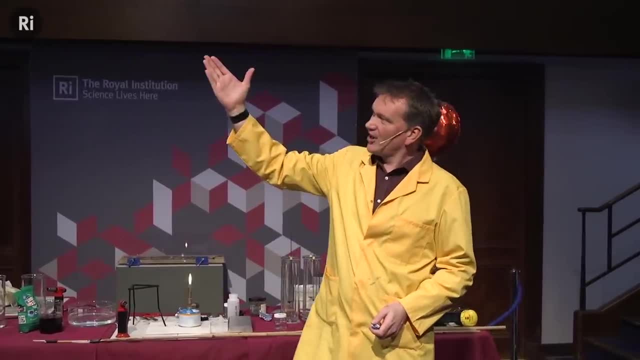 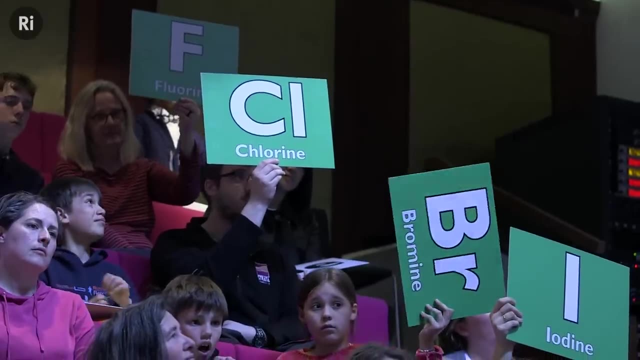 nearly killed himself. Other chemists did kill themselves trying to isolate fluorine. It is so reactive. Underneath fluorine we have chlorine. Chlorine is a toxic, poisonous gas And it gets its name from the greeny color, So chloro here chloros means greeny yellow. 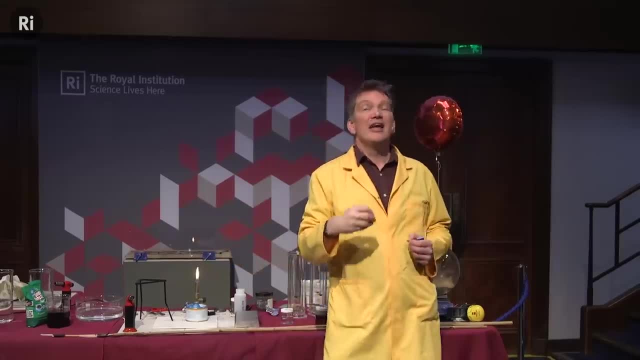 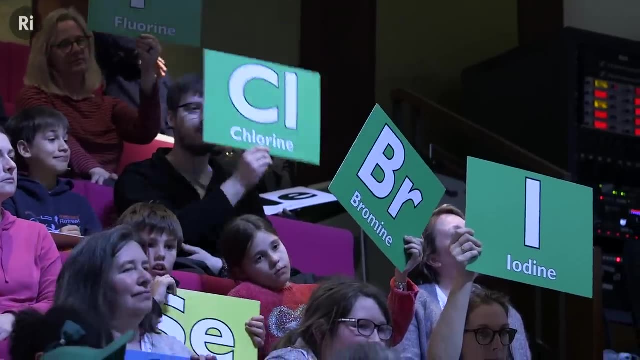 It's the same as you might have heard of chlorophyll, But it's not because it contains chlorine, It's because it means well greeny leaf chlorophyll. So it's the color there that gets its name Bromine. oh bromine, one of my favorite elements. 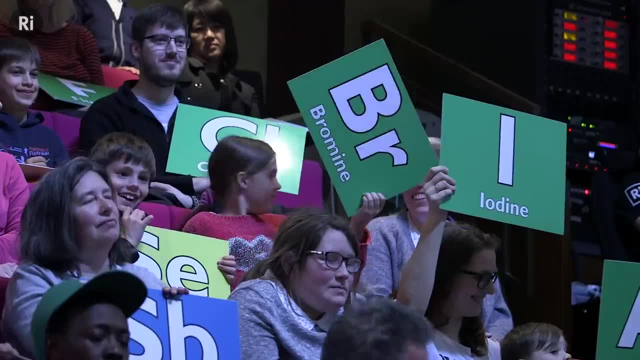 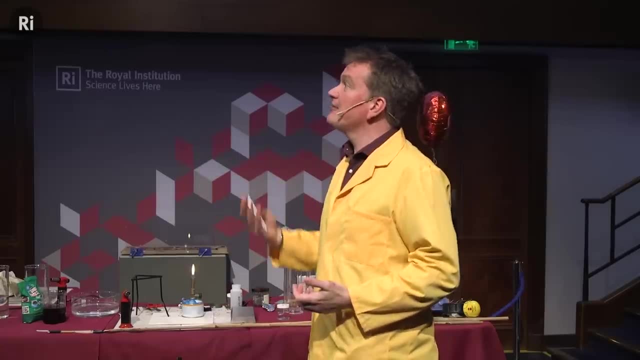 It's really evil looking. It's a liquid, a dark brown, orangey liquid, And it gives off this vapor, really heavy, choking, horrible smell. In fact, its name, bromos, comes from the Greek meaning stinky or smelly. 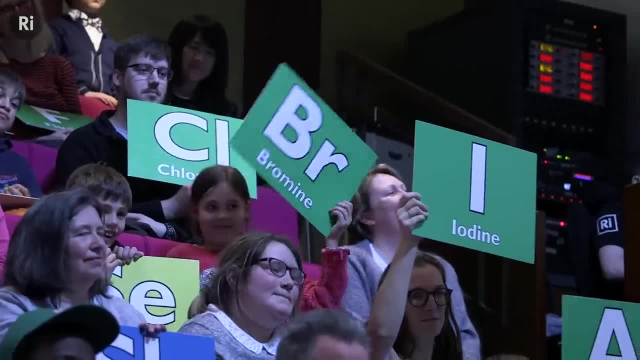 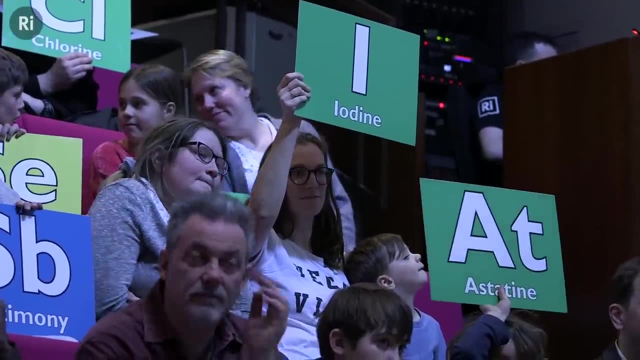 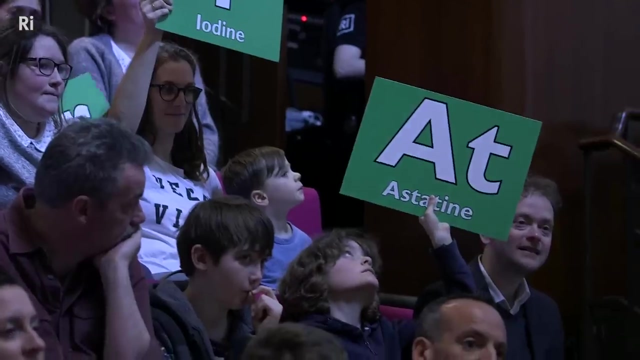 So that's how it gets its name. Iodine underneath gets its name from the beautiful violet color of this substance, And this- actually iodine and chlorine were named by Humphrey Davy here in the Royal Institution. Acetine gets its name from being unstable there and tenosine 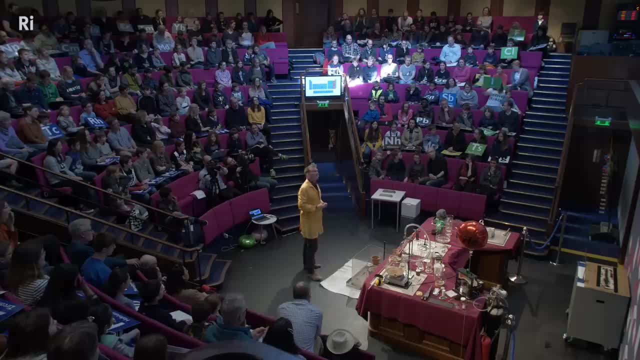 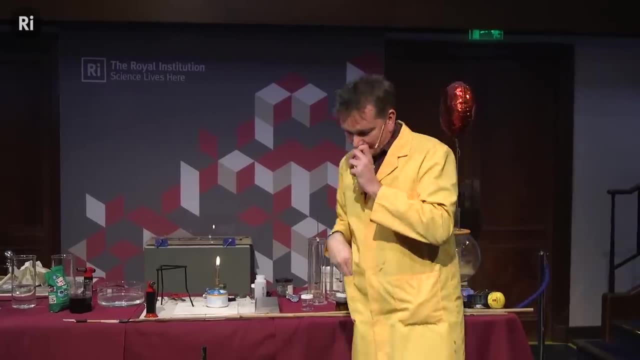 from the state. So quite a nice fun group. I thought I might show you one of these elements now, despite the fact that some of them are very, very toxic. I'm going to show you some iodine, And remember this gets its name from this beautiful violet. 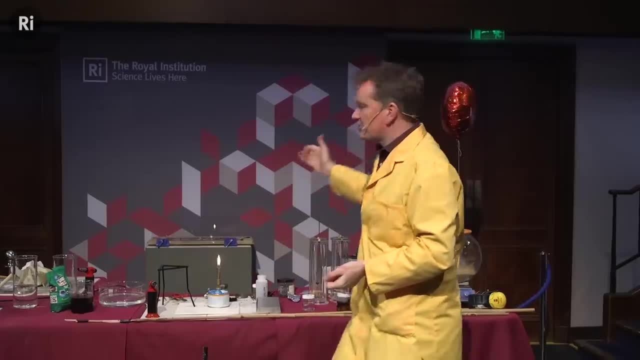 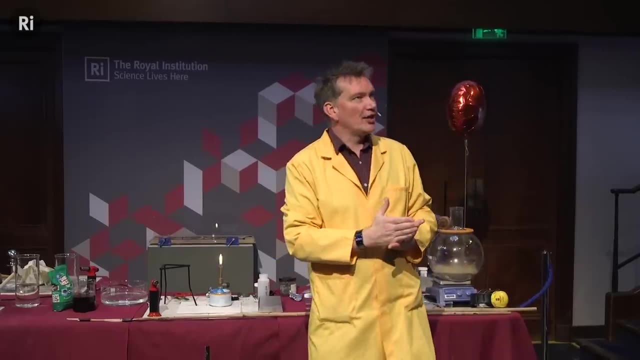 color. So we're going to make some iodine. Now at the back of the lecture- and this is why you had to come in through the sides- I've put a very explosive compound. This is called nitrogen triiodide, And this compound has nitrogen bonded to iodine. 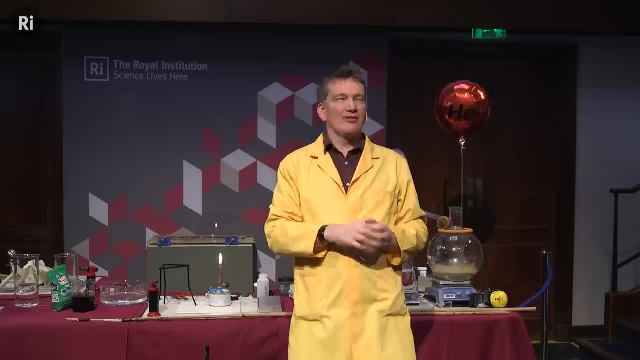 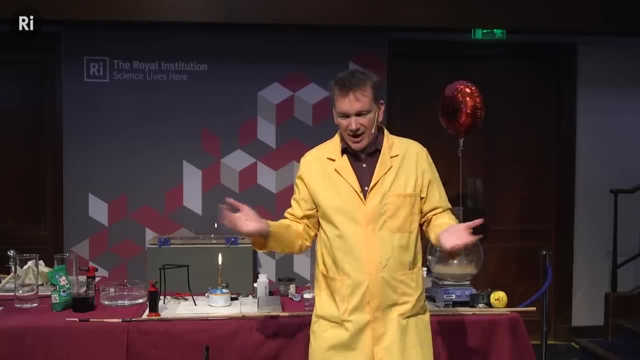 But these are very, very weak bonds And I'm hoping that when I just touch this compound- not with my finger, as you shall see, but when I touch this- it should explode very violently. And this is because these weak nitrogen iodine bonds all 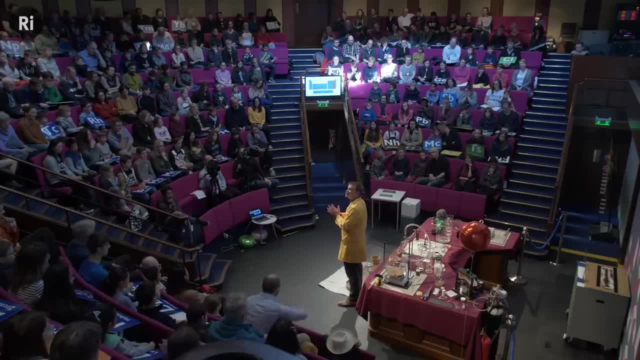 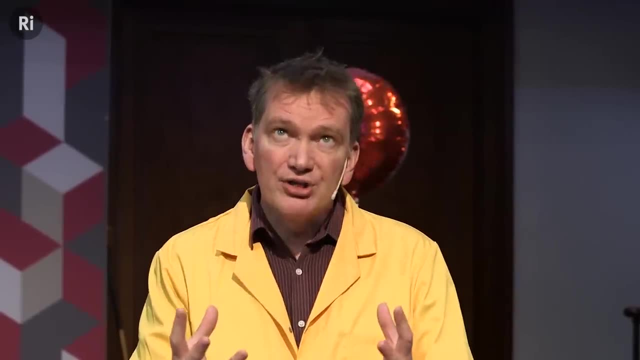 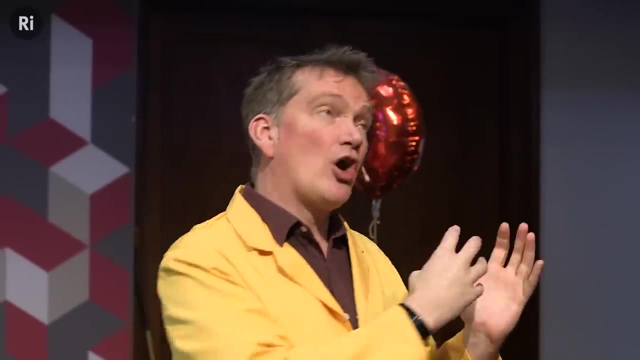 rearrange during the explosion and form the very, very strong bonds that we have in nitrogen molecules. So nitrogen, like the nitrogen that we breathe in, are molecules of nitrogen where two atoms are very strongly bonded together to form very stable molecules And it's this that drives- I hope will drive- this explosion. 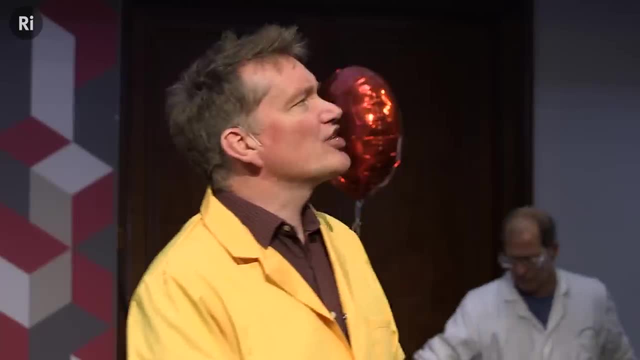 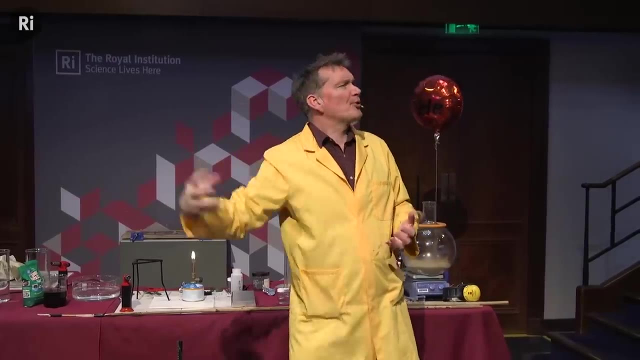 It's the formation of the nitrogen gas, But we can't see the nitrogen gas that's going to be formed. It's invisible. I mean it's in the air around us, Of course we can't see this, But we should be able to see the other byproduct. 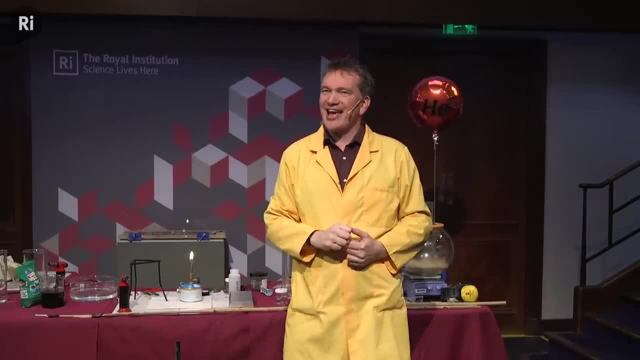 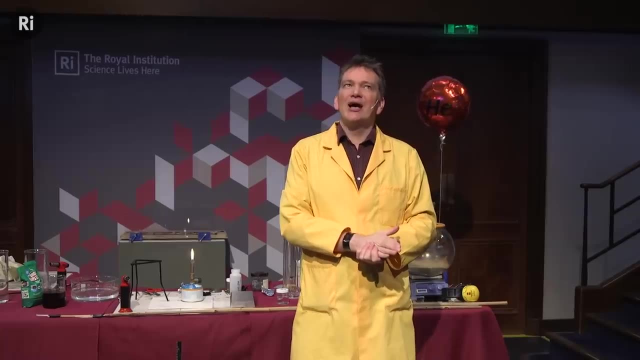 of this reaction, which is the iodine. So you need to look very carefully And you should see a purple cloud if it all goes well. Now this reaction is a little bit loud, OK, And it is quite a sharp explosion. 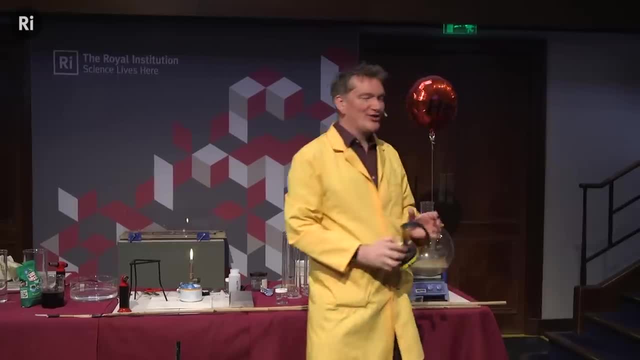 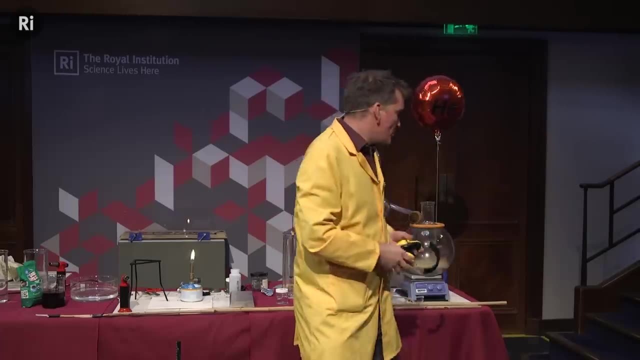 So I will be wearing these ear defenders, And this is always a good sign When you see the lecturer wear ear defenders. you really do need to just cover your ears Now. you won't need to stick your fingers in your ears, Just put your hands over them. 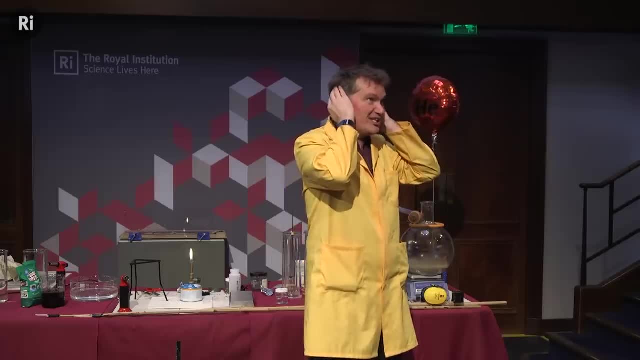 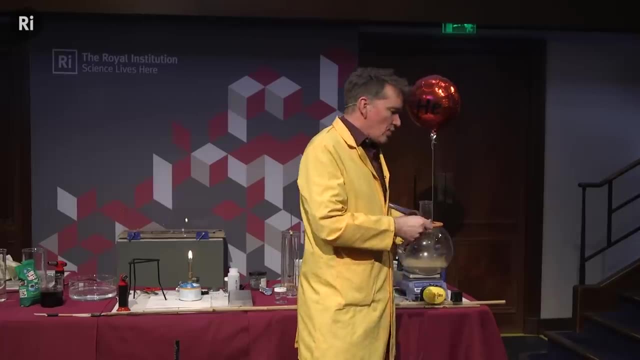 And this will stop the shock wave which could otherwise, if you're close, particularly close, damage your ears. So just cover them. You don't need to cover them really tightly, Just put your hands over your ears. OK, Let's give it a go. 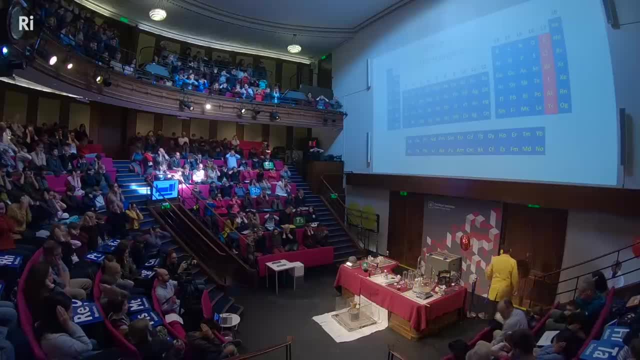 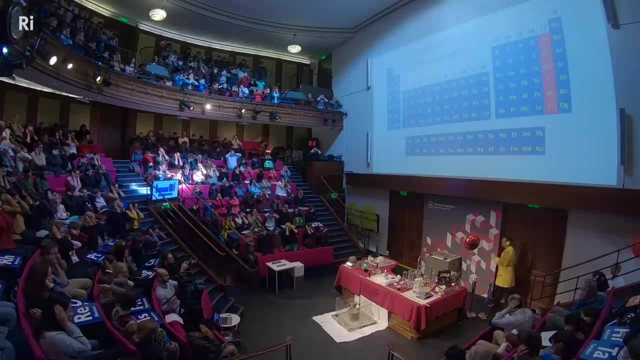 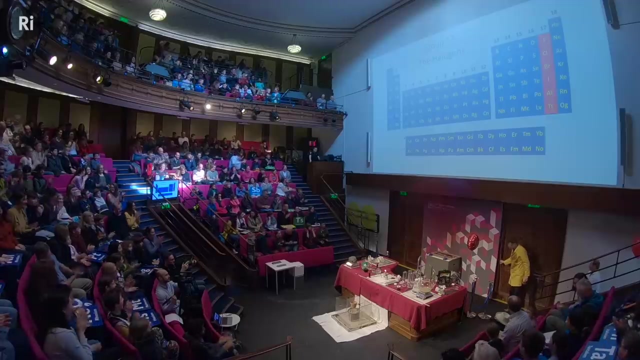 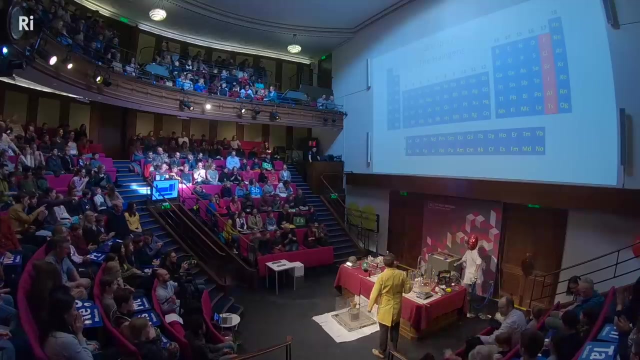 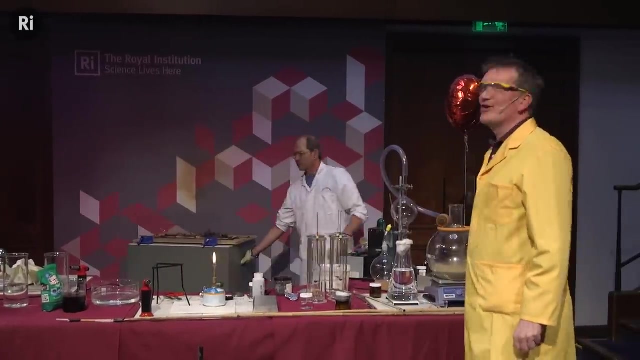 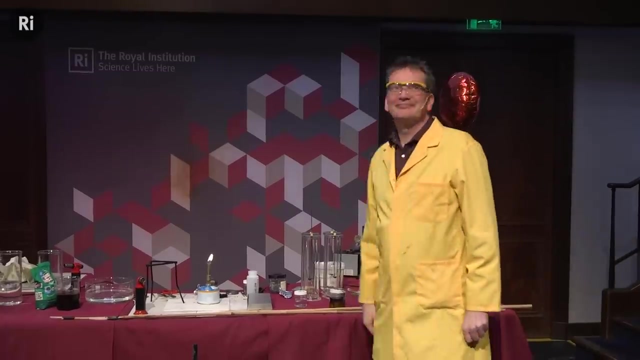 So let's put these on, OK, And just check that everyone's got their ears covered. So just cover your ears, OK, And there we are. So I hope you saw the nice violet cloud. It seemed to have changed the screen a little bit. 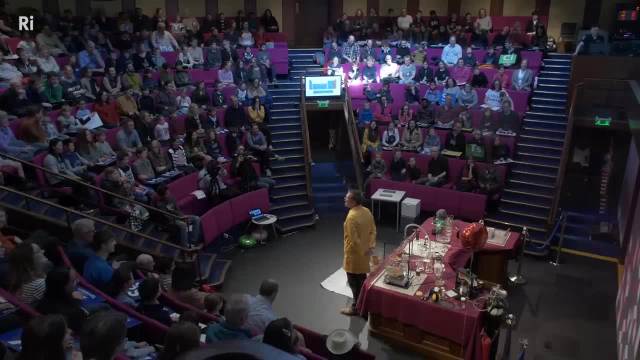 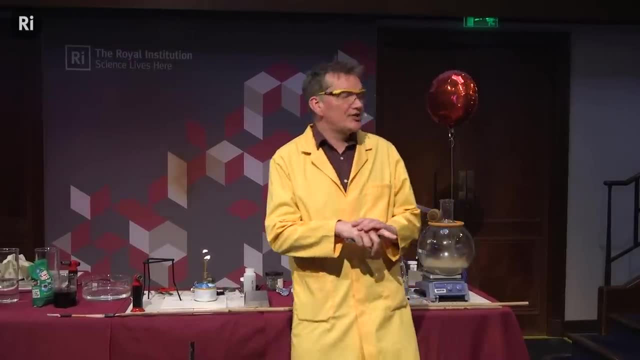 Never mind. So iodine is, of course, something that you will be familiar with. Maybe you've got some at home. in a first aid box There's tincture of iodine, So if you have a cut you can use it as a disinfectant. So when you have the solution and you're using it, and you're going to have the first aid, and you're going to have the second aid, and you're going to have the second aid, and you're going to have the second aid, 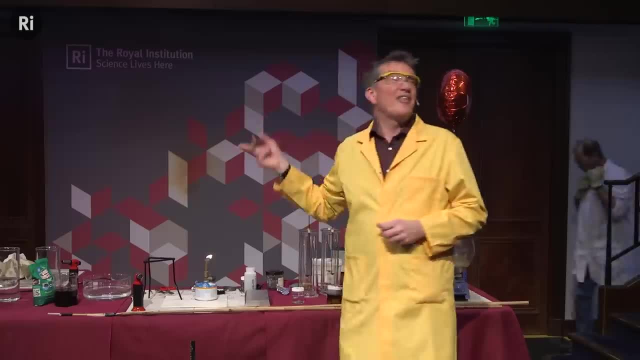 and you're going to have the first aid and you're going to have the second aid and it has this sort of browny color. This is the color that we'll see on the screen. That will actually disappear gradually during the course of the lecture. 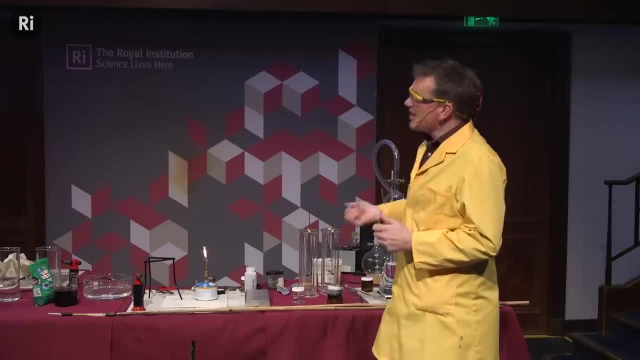 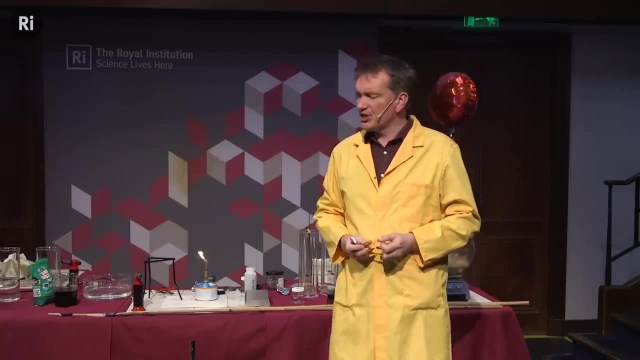 It'll probably be gone by the end of the lecture, which is quite interesting. OK, anyway. so that's one of the elements from group 17.. This group all, together with these similar chemical properties, are known as the halogens. 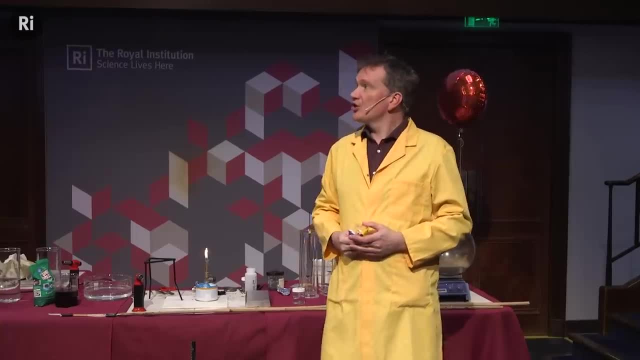 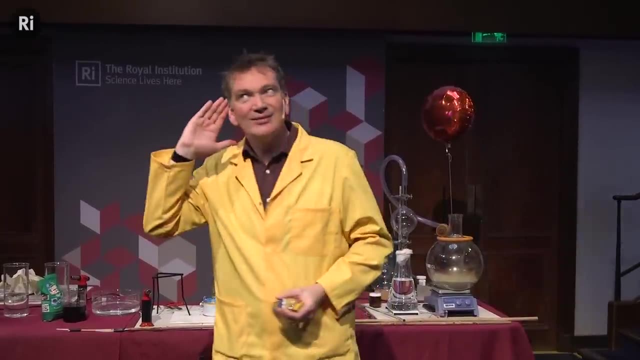 And this word actually means the salt makers, because they are very easily readily formed salts. I mean, we know, for instance, that our common table salt the proper name is Sodium chloride- Exactly sodium chloride, And that is then made with some sodium from this side. 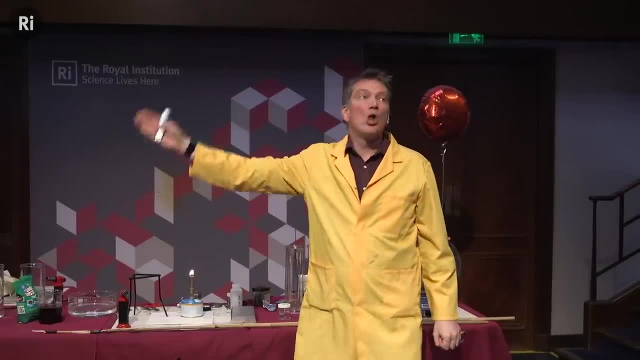 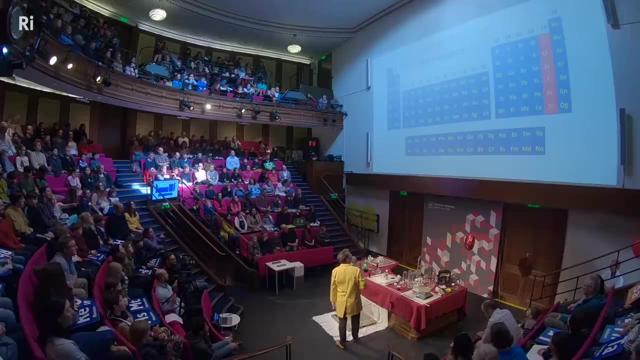 with the chlorine from that side. So these are all capable of forming salts. The group as a whole are known as the salt makers. OK, now that's the halogens group 17.. Let's have a look at a couple of the noble gases. 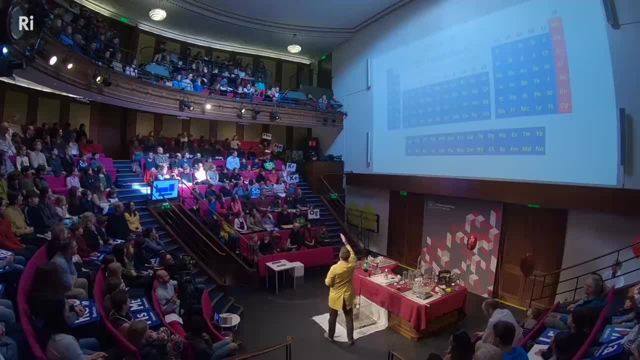 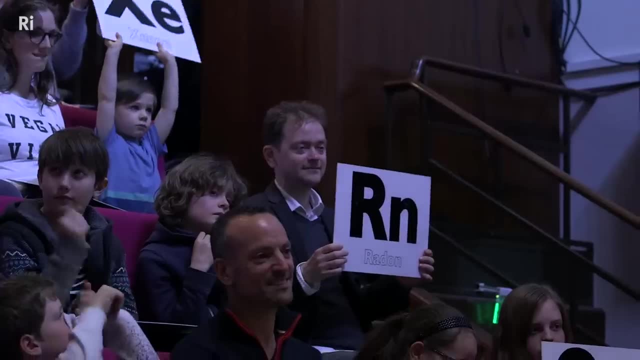 So where are you? noble gases? So very good. OK, so these are all the noble gases. Now, this is quite a remarkable group. This is the last group, This is the last group of elements to be discovered. None of these, none of these, are in Mendeleev's table. OK, 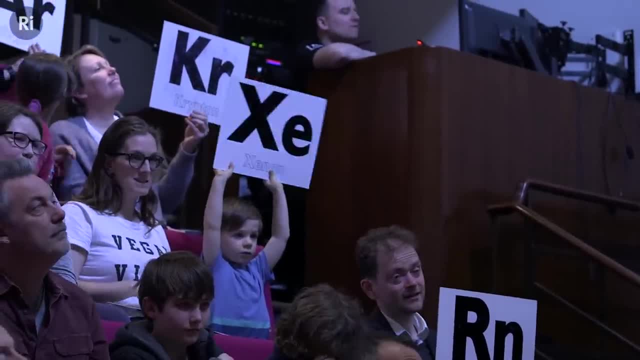 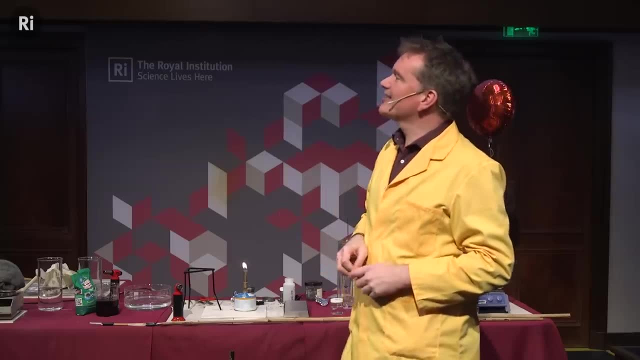 Actually the helium had been suggested and sort of somebody thought there might be this strange element in the sun. Mendeleev thought he was mad and so didn't include it and had nowhere to include it in the periodic table. Anyway, this whole group was discovered after his table. 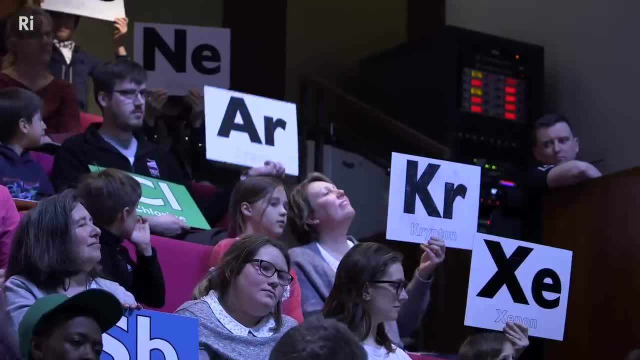 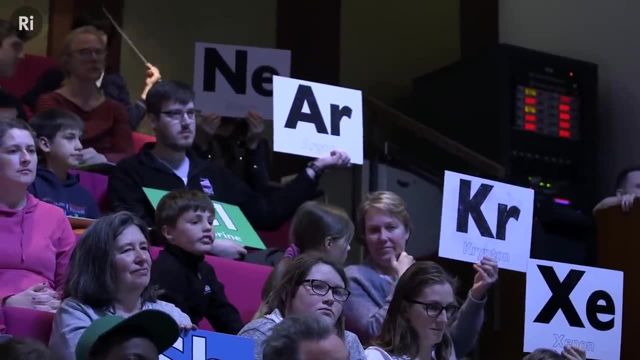 The first of these elements to be discovered was argon, And this was- it's actually- the third most abundant gas in the atmosphere. Remarkable, OK. So the first most abundant is nitrogen, then oxygen and then well, it's not carbon dioxide. 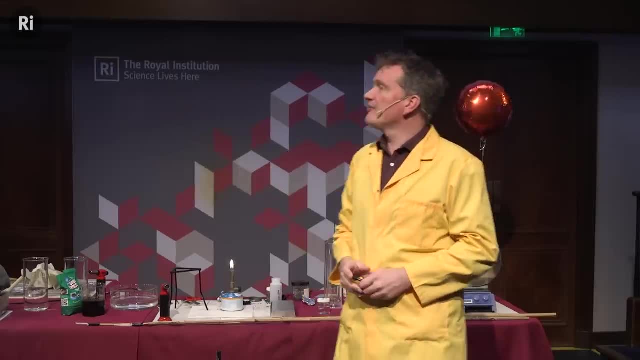 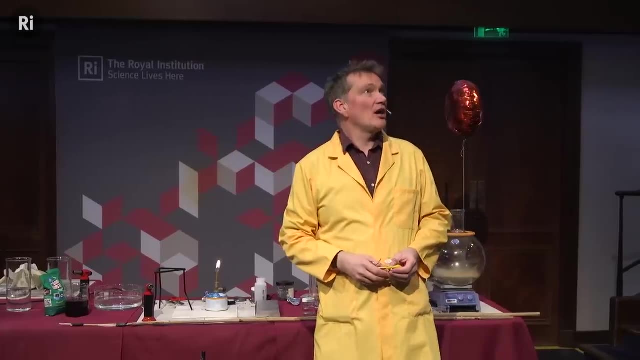 which some people think It's actually argon. There's 1% argon in the atmosphere And yet people knew about nitrogen, People knew about oxygen for 100 years before they noticed the argon And the reason for this. actually, 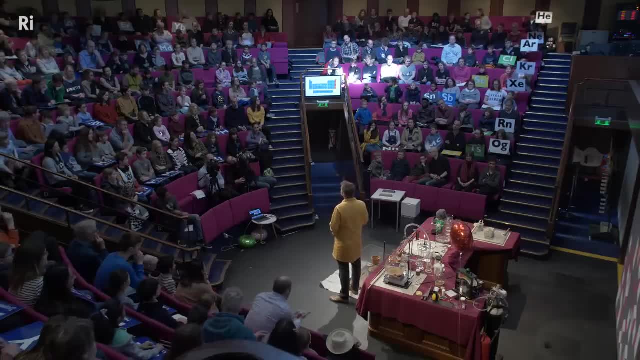 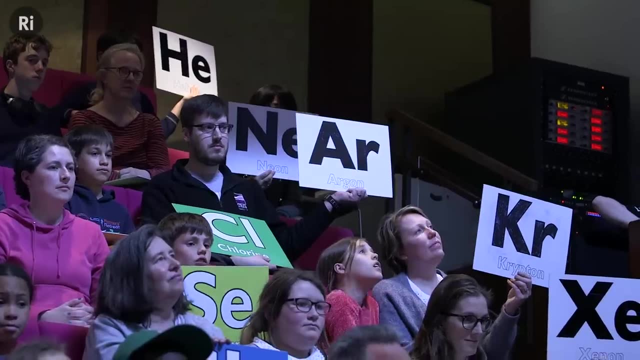 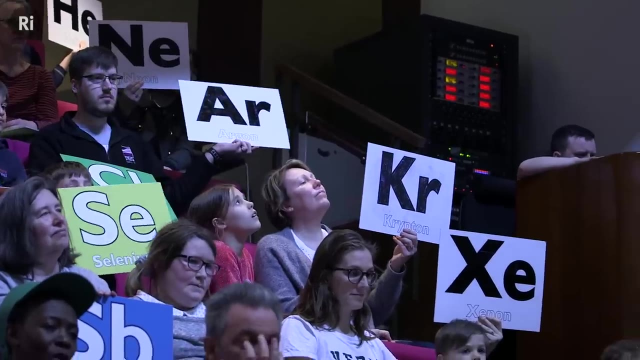 is because it doesn't do anything. In fact, argon doesn't combine with any other element at all in the periodic table, Neither does helium, Neither does neon. OK, Some of the other ones just begin to. So, some of krypton, xenon, radon. 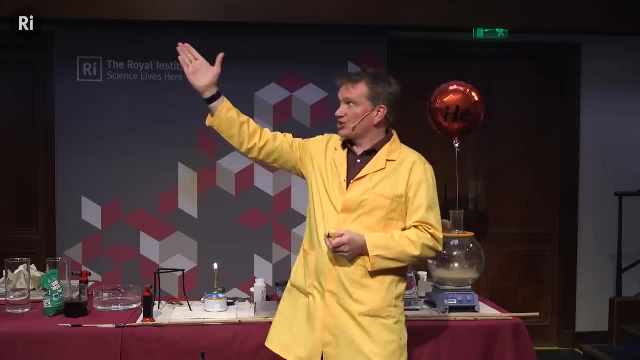 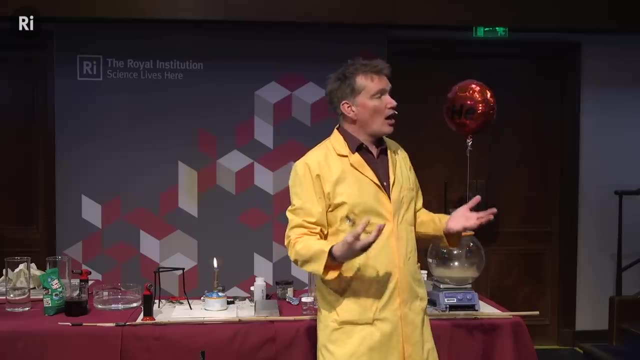 they have been made into compounds with some of the most reactive elements, such as our fluorine and maybe oxygen, But otherwise these are very inert And actually this is what gave the name to argon. Argon comes from the Greek word argos, which is, of course, 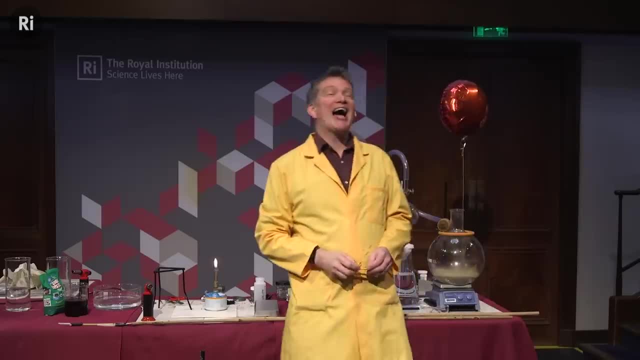 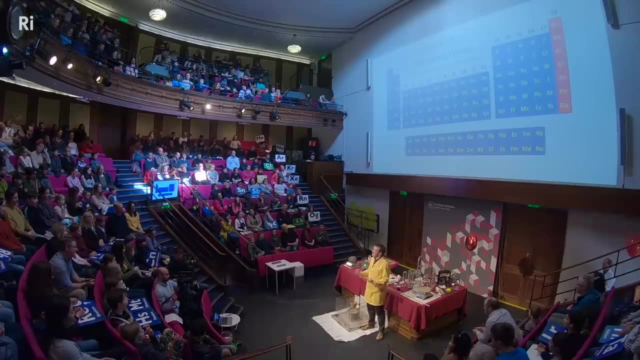 a well-known shop, OK, And argon is a very common name And argos well, I don't know. I presume they knew this when they named their shop. It means lazy or inactive, OK, Inert, OK. 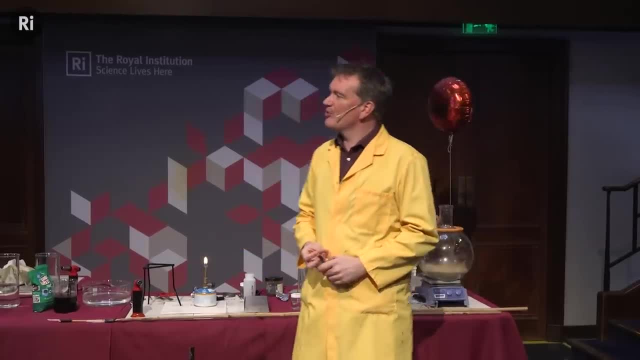 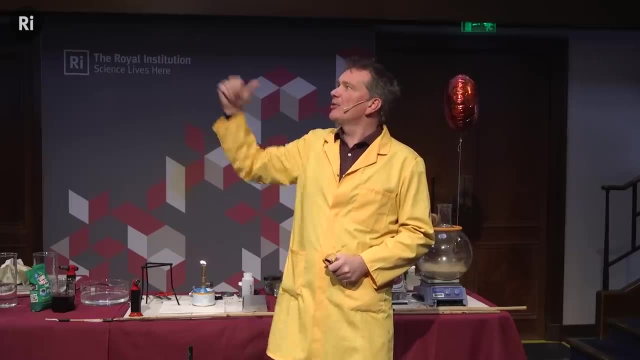 So not doing any work. So it's just an easy shop to do your shopping with. So this is because of this, the fact that it didn't react with anything else. It was a completely new element when it was discovered. Nothing like this had been seen before. 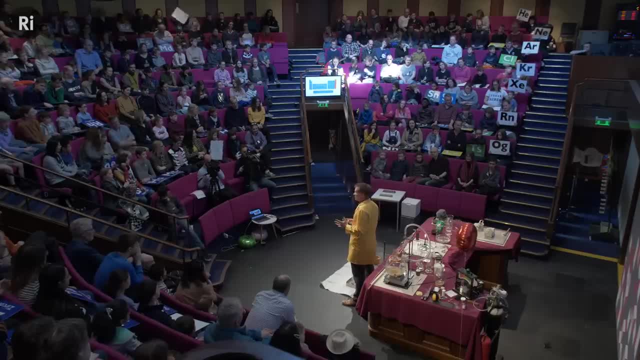 OK, so now remember as we go down: all of these elements have similar properties. So all of our gas, All of our gases here, have similar properties. They are all gases as far as we know. We don't know about oganesson, since there are only 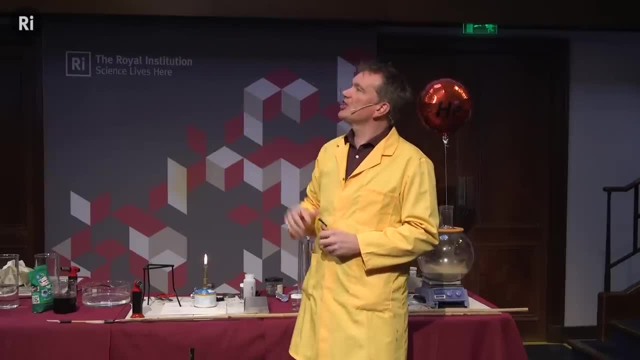 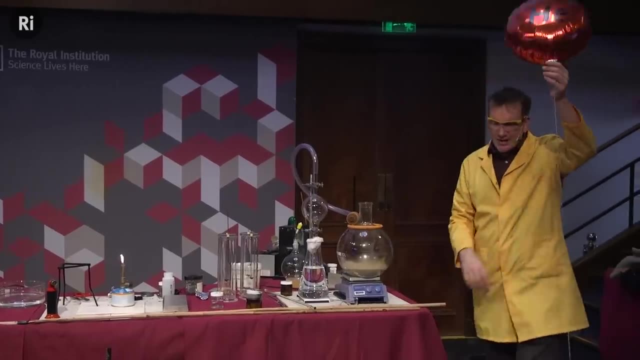 about five atoms ever made anyway, But the rest of them are certainly all gases, And I have a balloon with, well, one of them here, And this is our helium. OK, Now, remarkably, I say, these are so inert. OK, 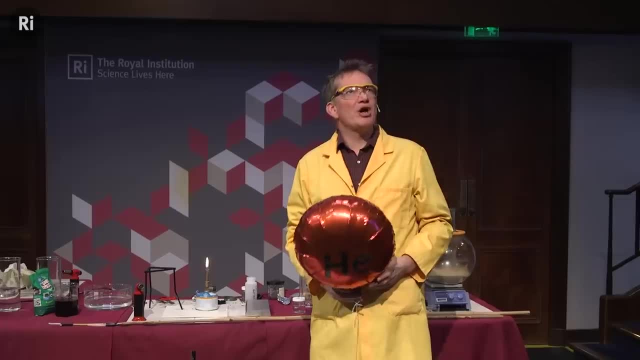 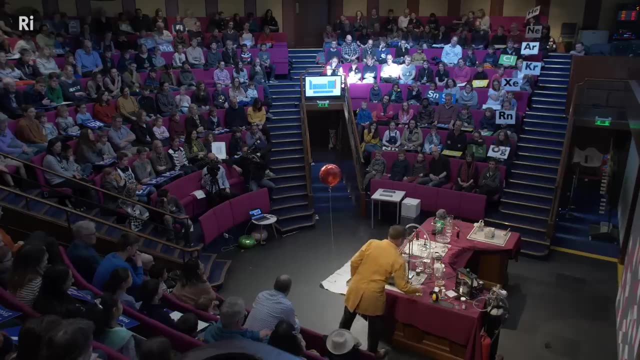 These even don't bond to each other, And this is quite remarkable. So whenever with all of the other elements, so most of them are actually nice shiny metals like this piece of an aircraft, I'm sure they won't miss it. 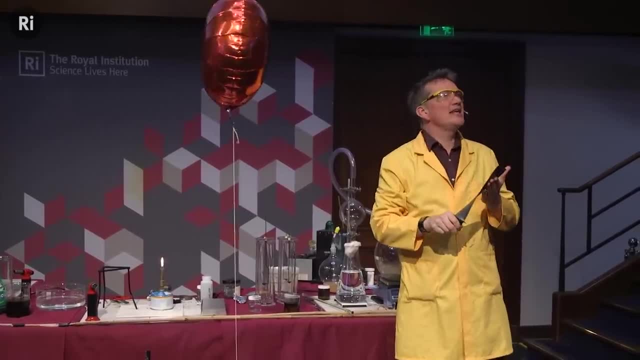 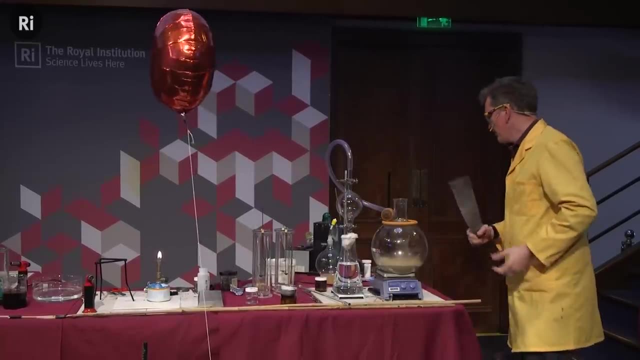 It's just the turbine blade. This is actually made of titanium, But it's a solid, And this is because the atoms of titanium are all bonding to each other OK to form a very, very high melting point. solid here, But helium, none of these elements, in fact. 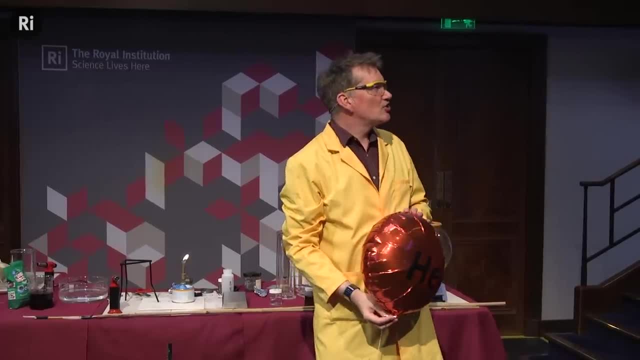 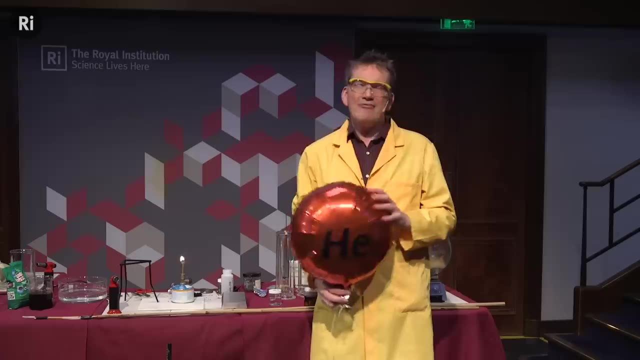 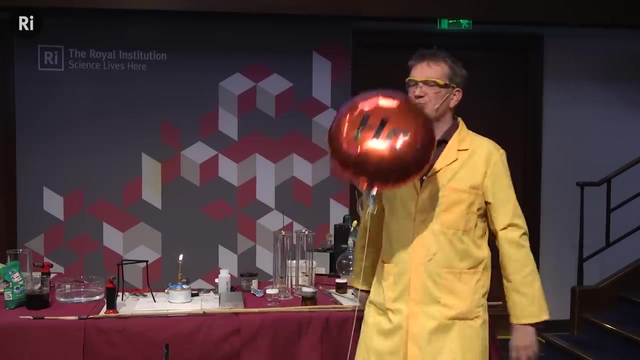 do bond to each other And they exist as individual atoms. And if ever you have a helium balloon, this is pretty much the only time you will ever come across individual atoms. so individual atoms in this balloon here, OK, But as we see, they are lighter than air. of course, 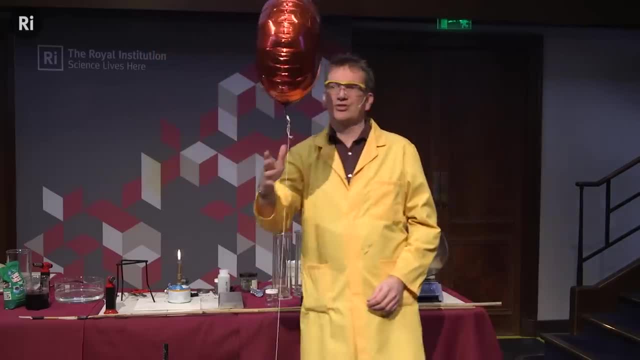 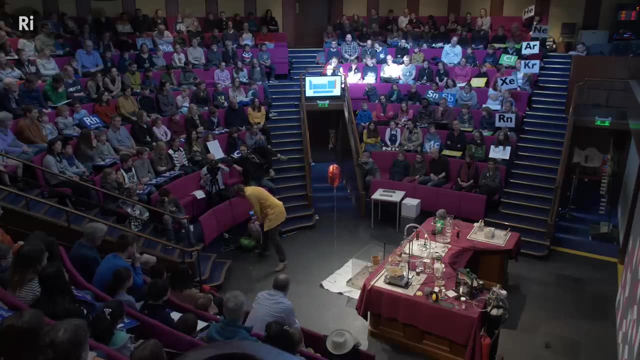 Helium is element number two. It's only got two protons, two neutrons and two electrons, so lighter than air. Well, I have some of the next element underneath it, some neon down here. So this is the element neon. 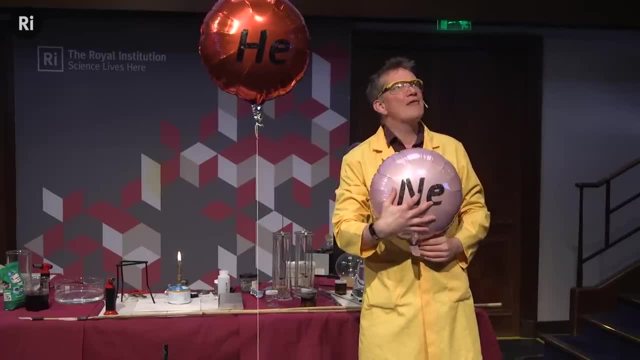 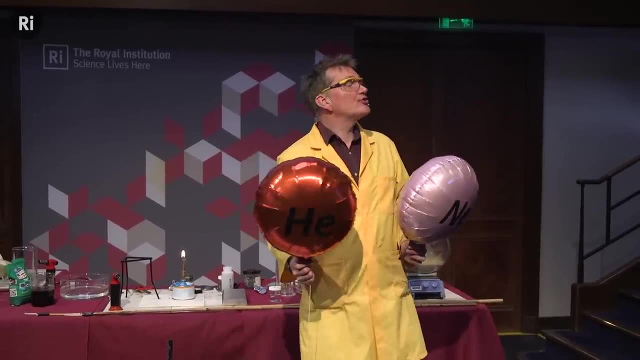 Now there's a rather remarkable thing, And that is that whenever we have equal volumes of gases- and so these are clearly pretty much equal volumes, the same size- so long as they're at the same pressure and temperature, they actually end up containing equal numbers of particles. 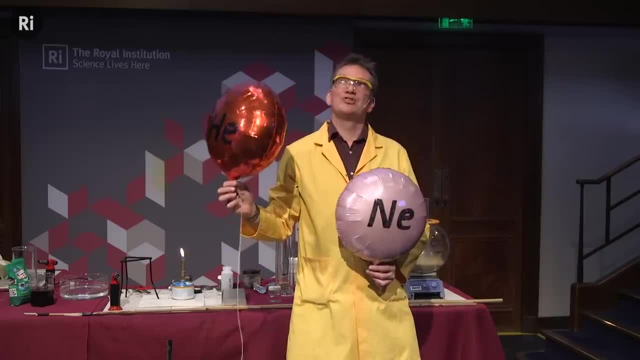 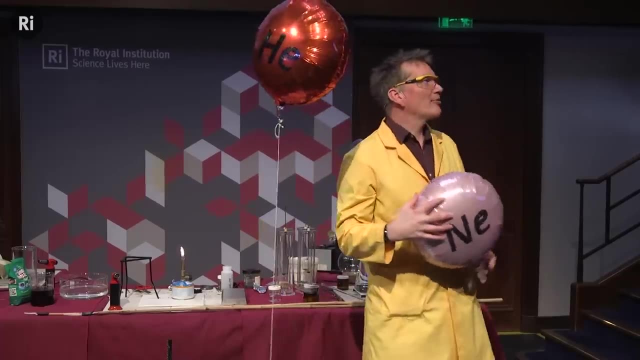 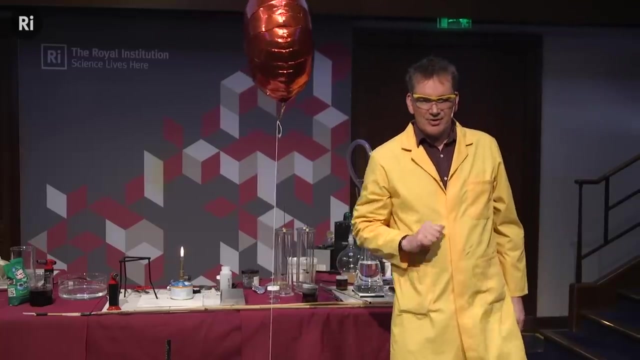 In this case, what it means is there is the same number of atoms of helium in here as we have atoms of neon in here. These are, of course, lighter than air. What about our neon? Well, it's probably the balloon itself that. 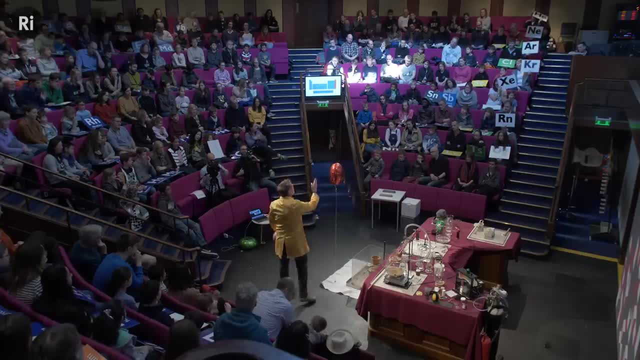 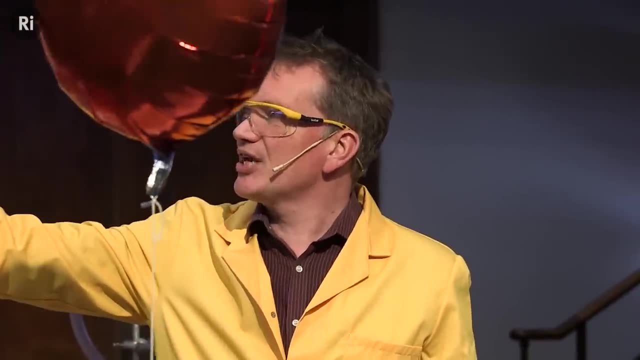 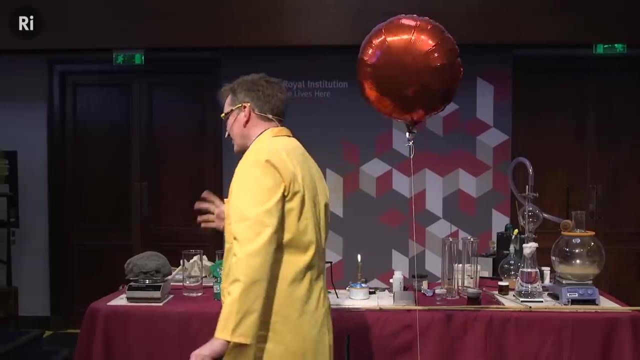 is sinking here. But remember, as we go down the group we are increasing the number of protons, neutrons and electrons, so each atom is getting heavier. Now I can't have a balloon of oganesson because there were only five atoms, or six or so, ever made. 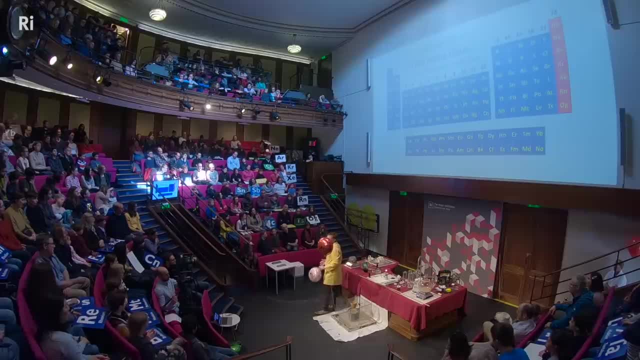 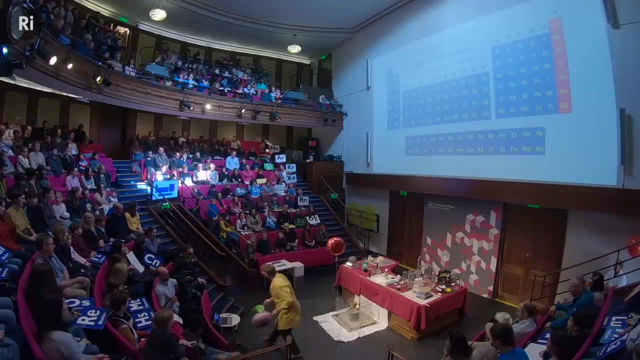 and they disappeared like that Radon. I can't have a balloon full of that because it's very radioactive, so that wouldn't be good. The heaviest one that I can have is the xenon, And this is a balloon of xenon. 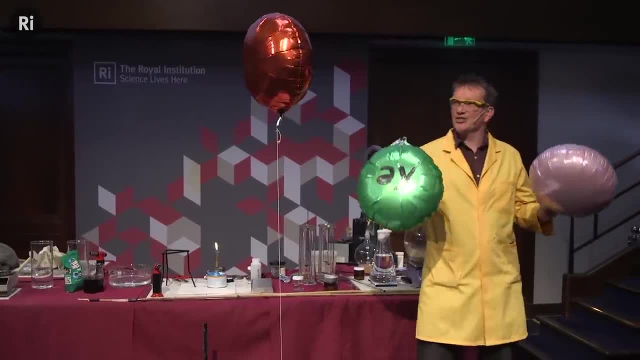 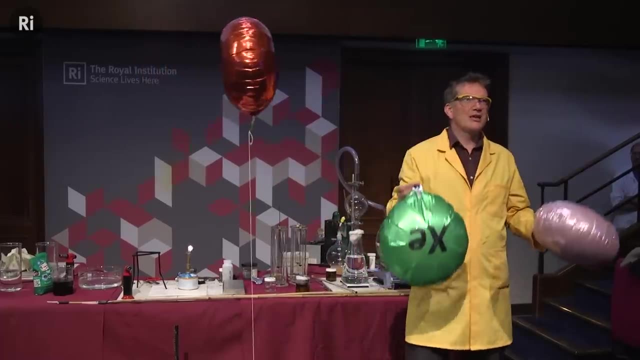 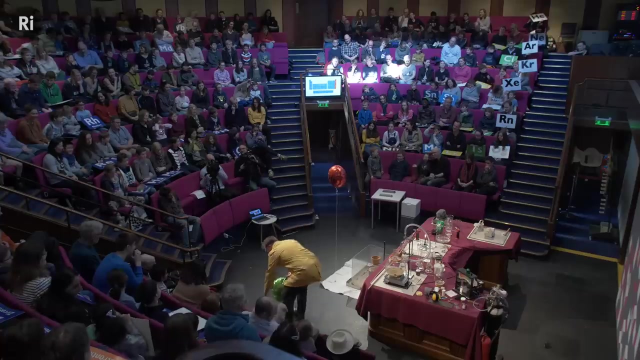 So it has gone down a little bit over the course of the lectures, but pretty much the same number of atoms, maybe slightly less than we have in here and in here. But what about the mass of these? So it really is actually quite heavy for a gas. 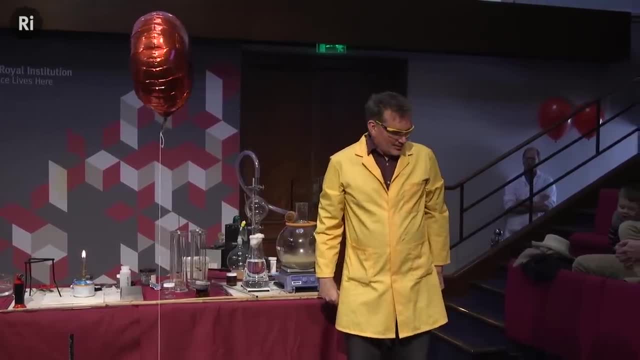 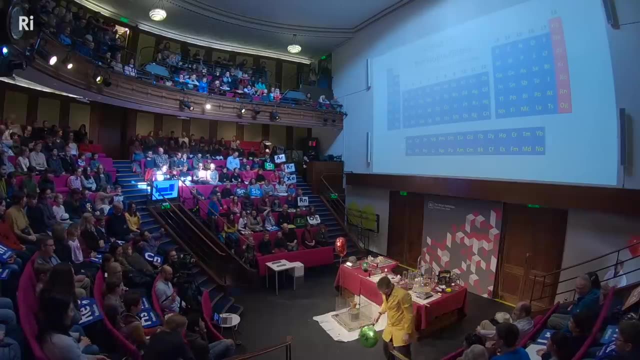 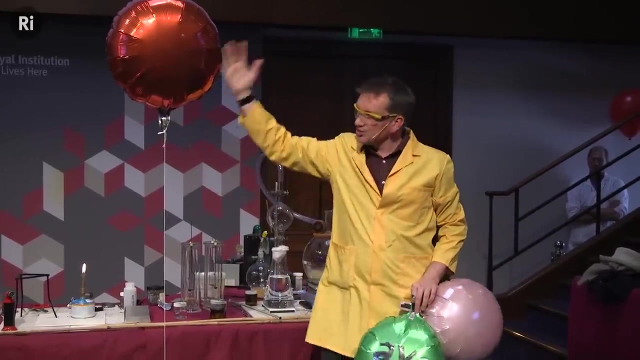 So I said it's the same number of atoms, So this really wouldn't be a very fun balloon to take to your parties. But this shows very nicely then that as we go down the group what's happening? they're all still gases. 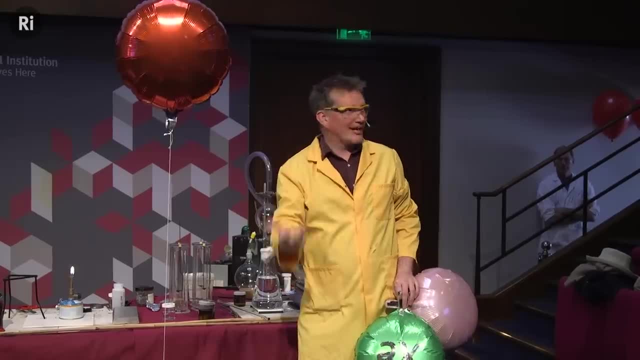 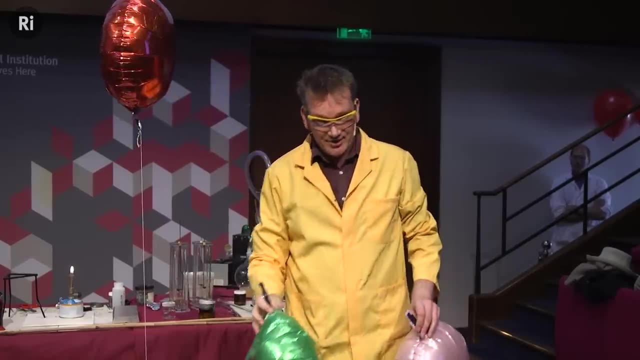 but because we're increasing the number of protons, neutrons and electrons as we go from one period down to the next, one row to the next, the atoms themselves are getting heavier. Very important, OK. well, thank you very much. Noble Gases. 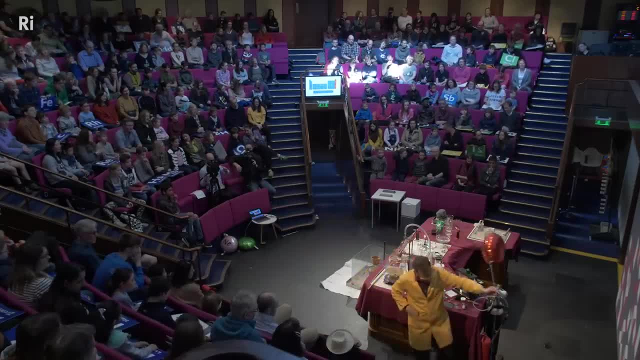 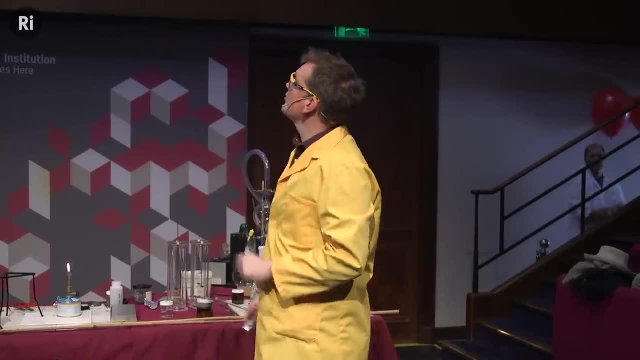 You've been very good holding your signs up. Thank you. Now we mustn't forget the other elements in our periodic table. We have a lot in the middle, the dark blue cards. These are the so-called transition metals. Do you want to give us a wave, transition metals? 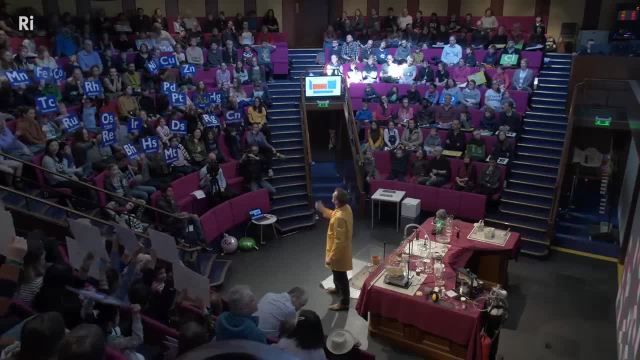 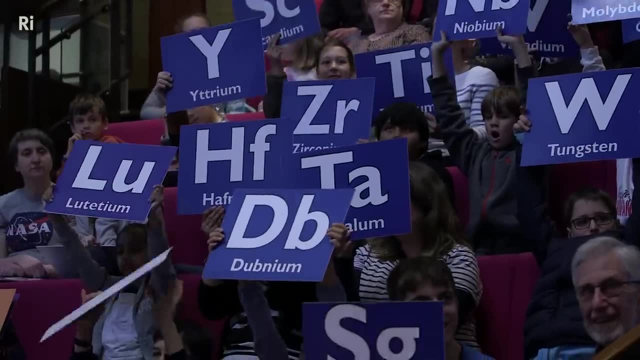 So we have all sorts of things like titanium that we saw in the blade there. We have iron, copper, nickel, all sorts of nice fun metals here: gold, very beautiful mercury there. OK, so these are our transition metals. 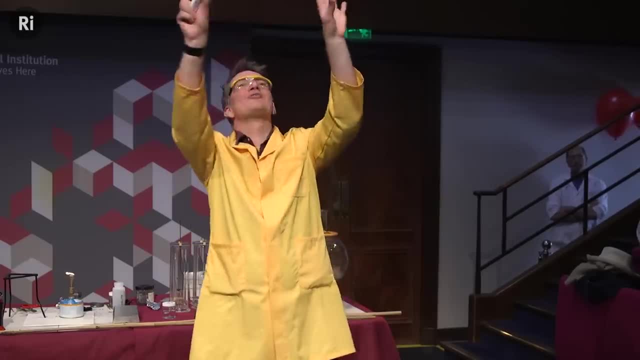 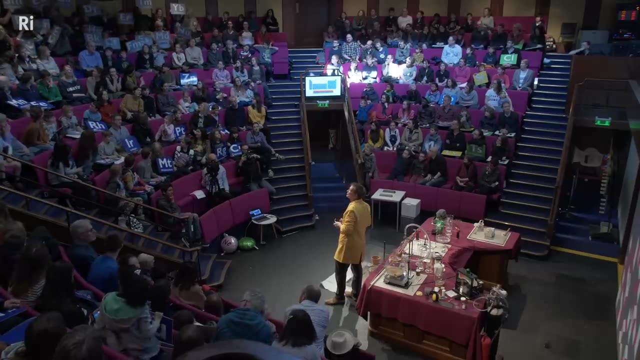 And then we also have the light gray. Now, you're all right, We're back there. So, yeah, I'm afraid that it's rather important. Some of these are becoming more and more important now, such as neodymium. So we have our magnets and containing those, 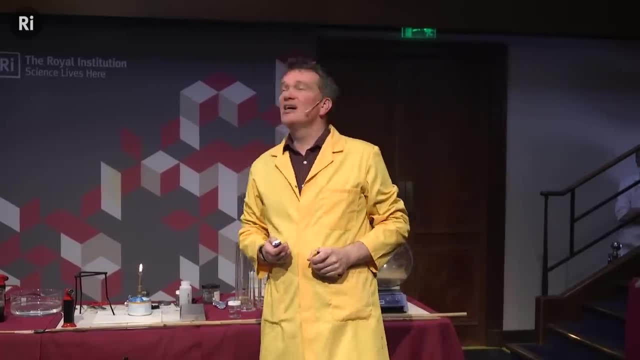 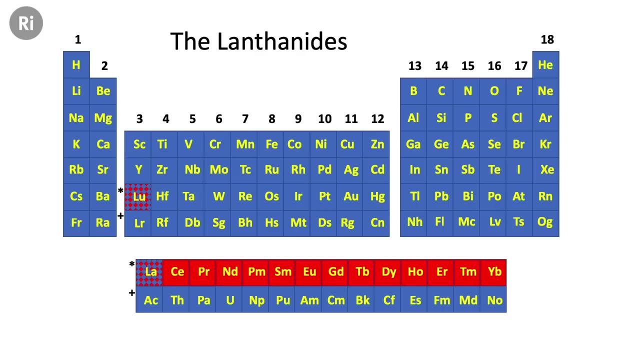 very important, very strong magnets. But these elements here, they ought to be in the main body of the periodic table. So there's a little place marker there. The asterisk and the little cross shows where they should go, these so-called lanthanides. 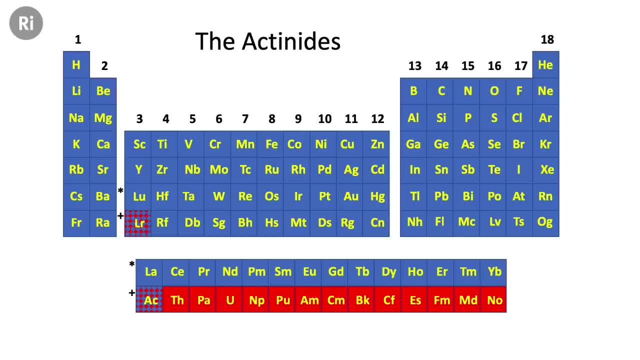 and actinides, But it would make the periodic table very long, And so this is why we've put you out the way at the back there, OK, But you ought to be in the main body of the periodic table, OK, so these ought to be in there. 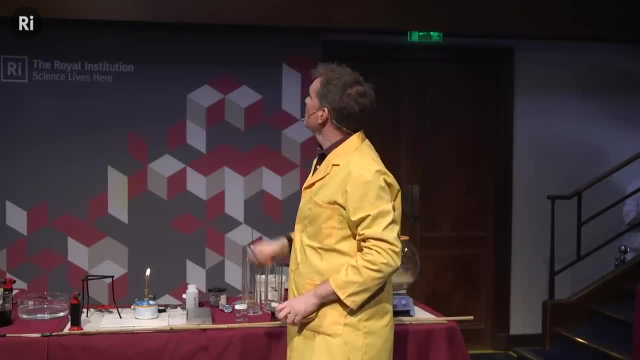 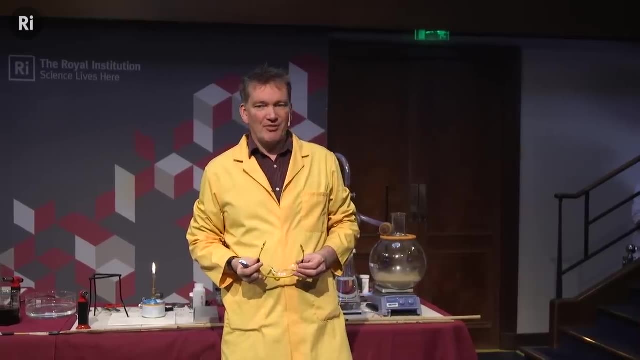 But it would just make it very long, too long for the screen. OK, so that's a brief overview of the elements in the periodic table. Now what we want to do is look at the chemical properties of some of these, And we're going to start off with, well, the first two. 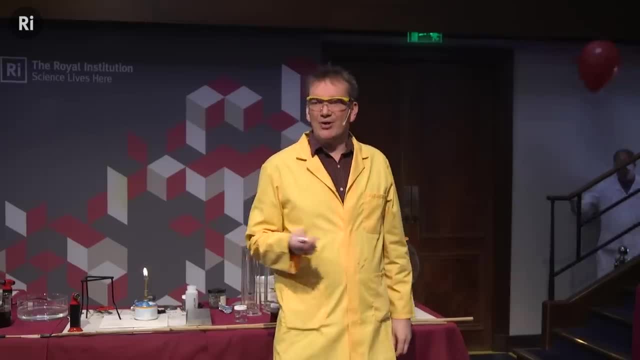 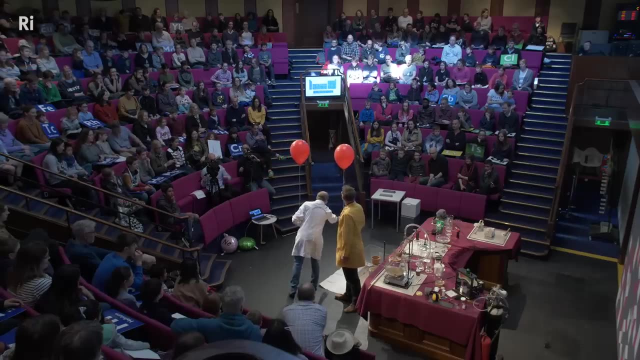 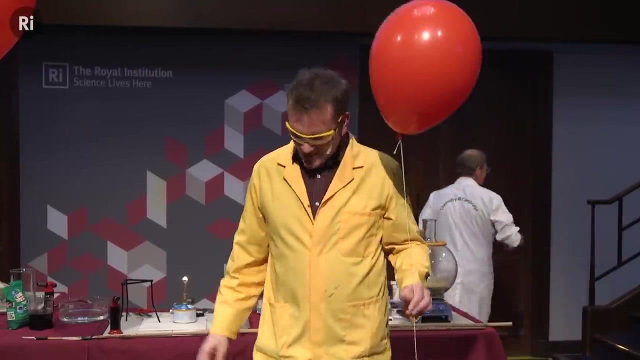 elements, And I think Chris has prepared a balloon of hydrogen for me and a balloon of helium, so we could compare these two. OK, Chris, you seem to have used the same color balloons. I think I deliberately told you You used different colors, so I know which one's which. 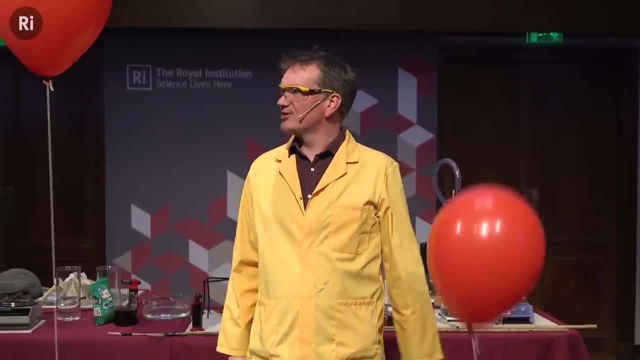 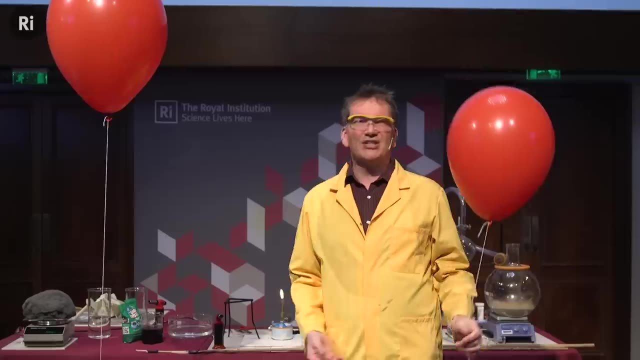 OK. well, one of these, apparently, is filled with hydrogen. One of them is filled with helium. I have no idea which one's which. There is a difference between them, So remember whichever one it is. the helium actually has individual atoms in here. 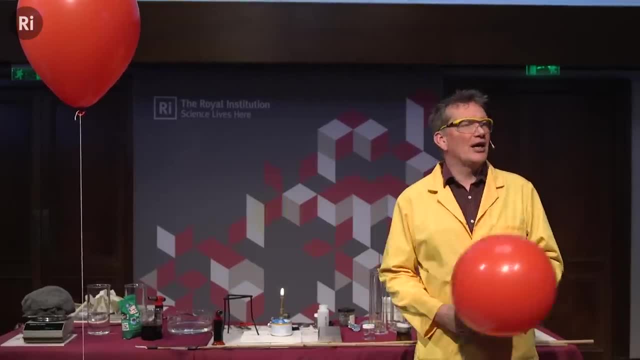 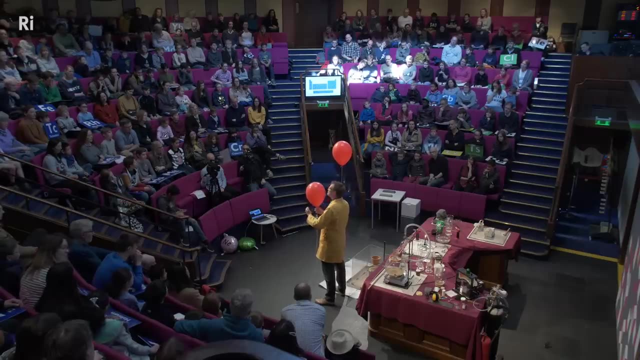 The hydrogen. well, hydrogen forms molecules Like every other element in the periodic table. apart from the noble gases, they all stick to each other. Hydrogen forms molecules where two hydrogen atoms bond together, So one of these is filled with hydrogen molecules. 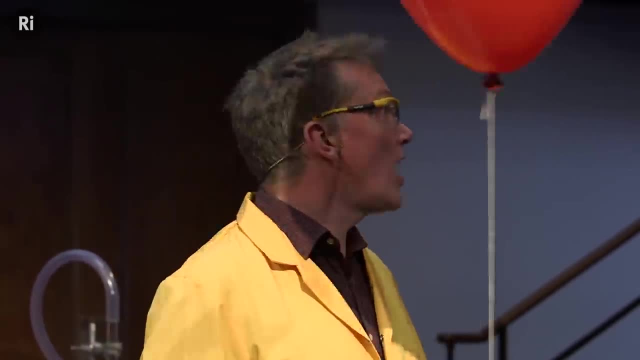 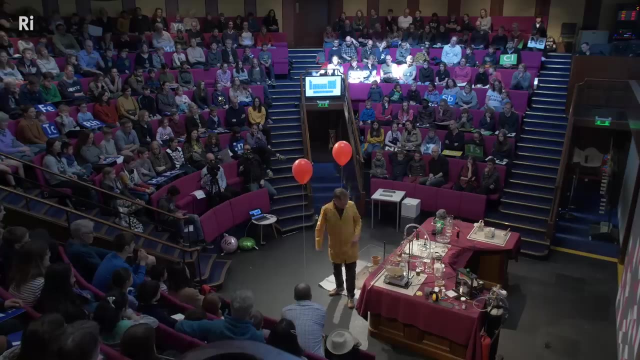 One is filled with helium atoms, But actually the hydrogen is still lighter. Hydrogen is the lightest element, But I don't know which one's which. So, oh dear, never mind. Anyway, but I do know a way to find out. 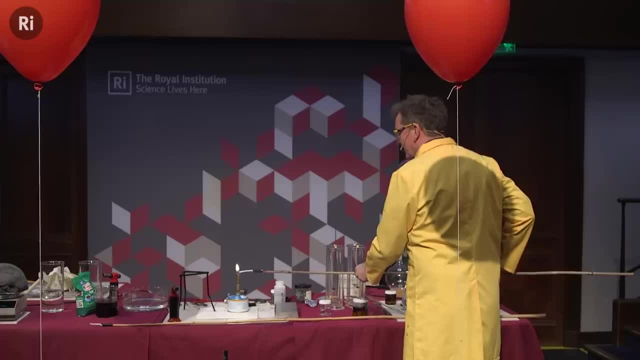 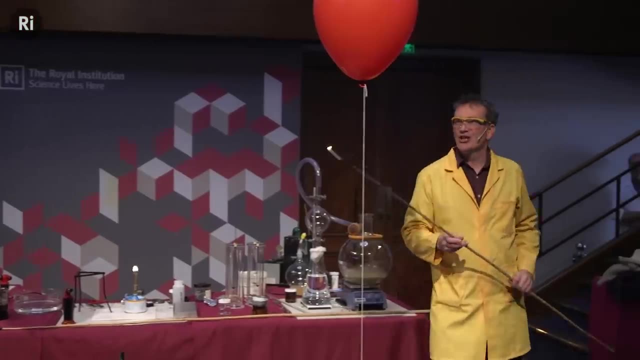 We can use a test, a chemical test. I'm going to use my little candle here, my lighted splint, to see if I can see which one's which. So let's try this first, First balloon then. So it's either going to be hydrogen, 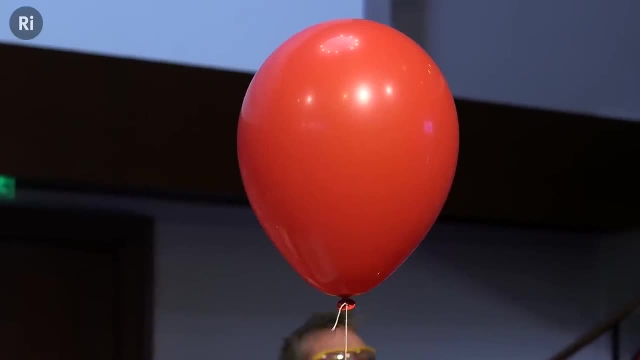 or it's going to be helium. You don't need to cover your ears unless you really, really, really, really don't like any bangs at all, But otherwise you'll be fine. It should be fine, even if it is the really explosive one. 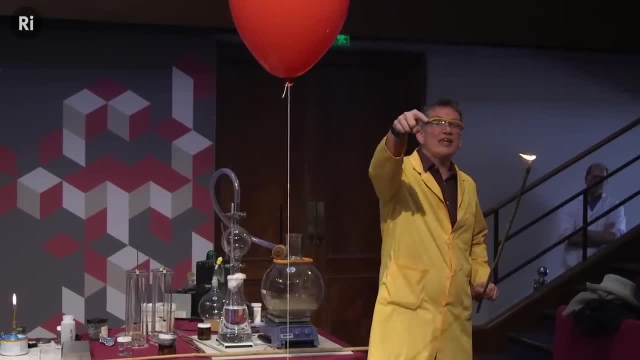 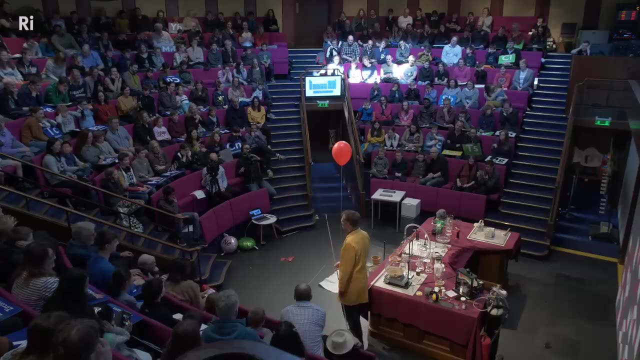 We don't know, We'll see. OK, well, let's give it a go Now. watch very carefully what happens with my flame. OK, We'll see which one. this is OK. so well, all that happened there. 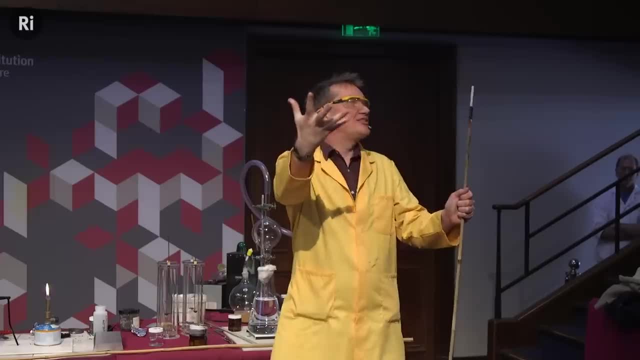 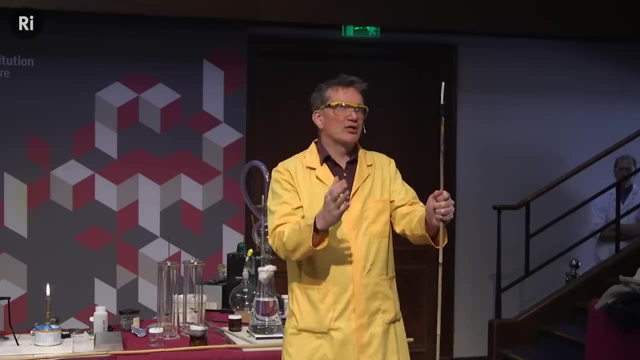 there is. well, it actually made my flame go out. It didn't burst into flames. It must be the helium. So the helium, remember, is incredibly inert, unreactive, It does not react with the atmosphere. There's no explosion. 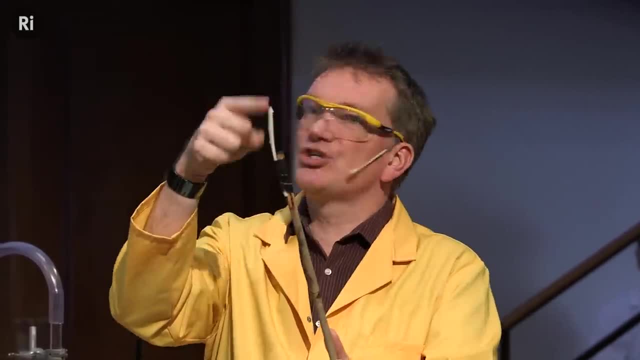 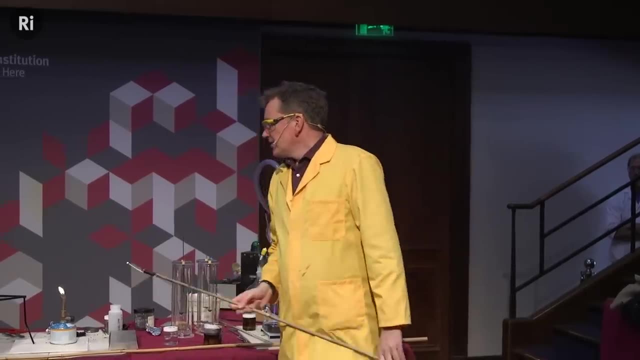 All that happened was the balloon burst and it even put my flame out. So it extinguishes flame because, well, it doesn't do anything. OK, because it's completely inert. So that means we hope that this one- unless Chris has played a trick on me and they're both helium- 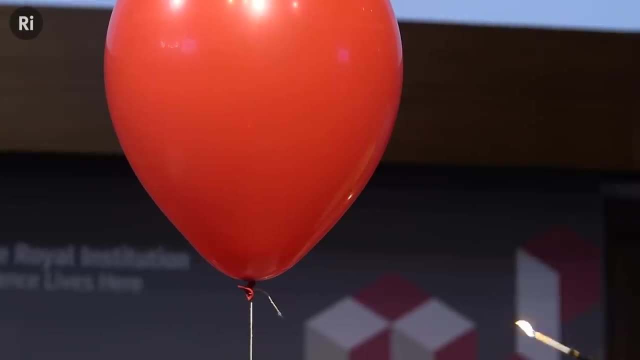 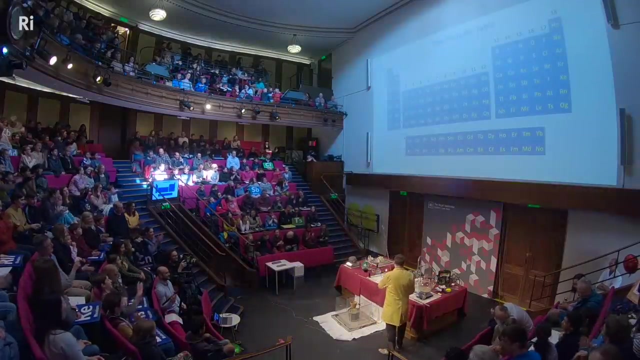 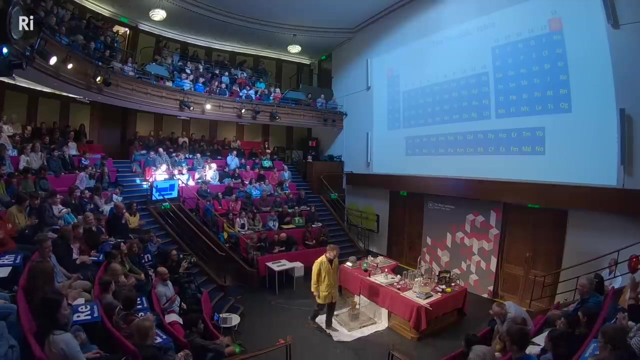 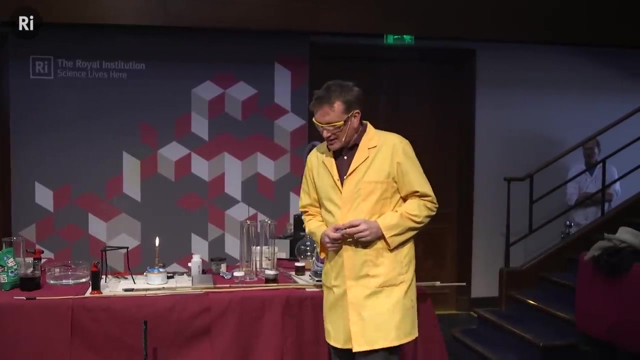 we hope that this one is hydrogen. So let's try the hydrogen one then. So let's see if this is hydrogen. Oh, that was nice, So that was very nice then. They clearly have Very different, very different chemical properties. 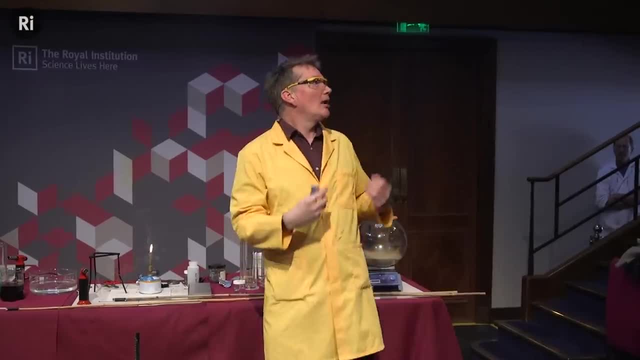 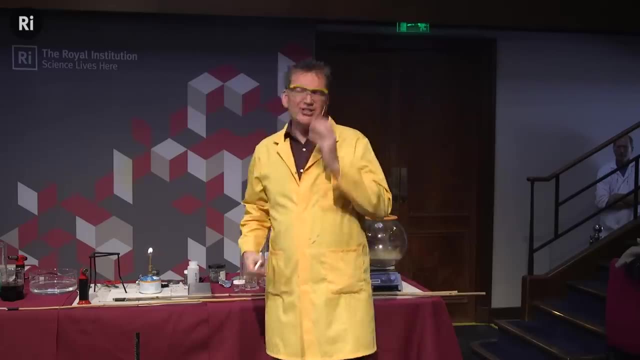 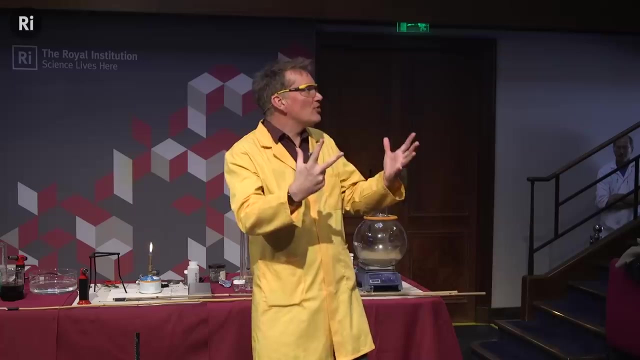 Our hydrogen, our hydrogen molecules were explosive with the air, So they were combining with the oxygen. The helium didn't do anything whatsoever. So very different chemical properties, these two first elements, But of course, when the hydrogen does react, the flame that you saw there. 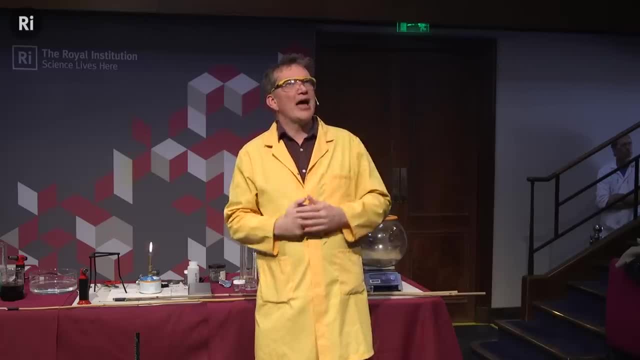 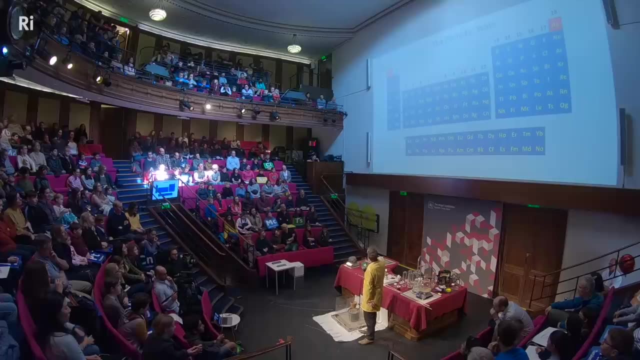 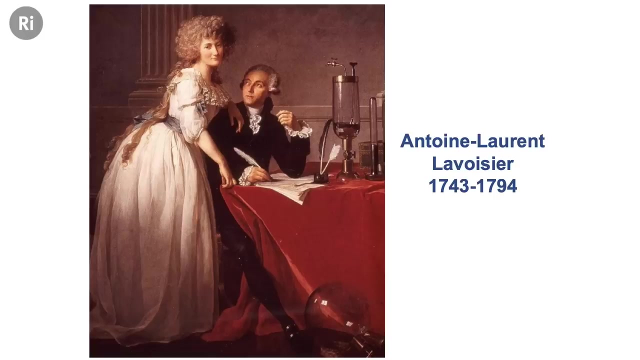 it's the hydrogen gas there, reacting with the oxygen from the air to form water, to form hydrogen oxide, H2O2.. OK And well. hydrogen was first appreciated that it was an element by this chap here and his colleagues. This is Lavoisier, the French chemist. 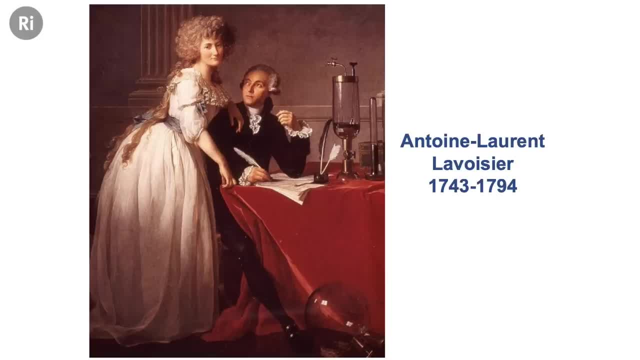 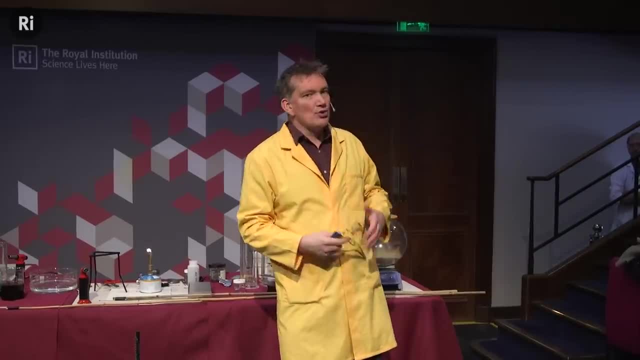 And he first drew up a list of elements, a modern list of elements, Unlike the Greeks who thought, for instance- you may have heard that they thought that things could be broken down into the principles of gases like air, fire, earth and water. 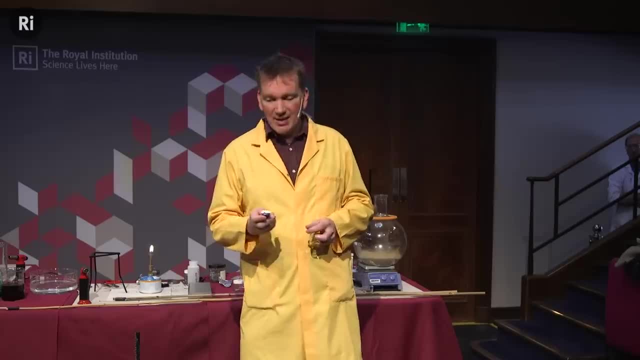 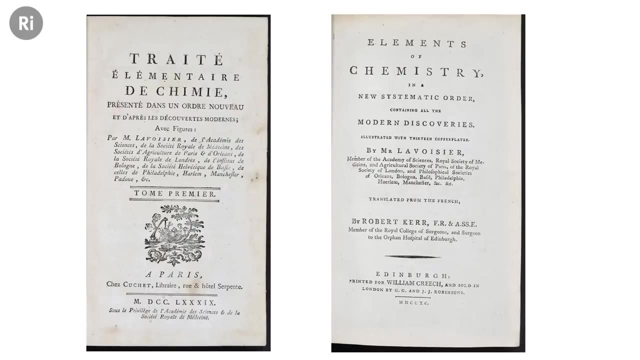 Well, he drew up, and his colleagues, the first list of elements in their modern forms And it was in the book here, his Traité, published in 1789.. And this is the English version from 1790.. And here is the list. 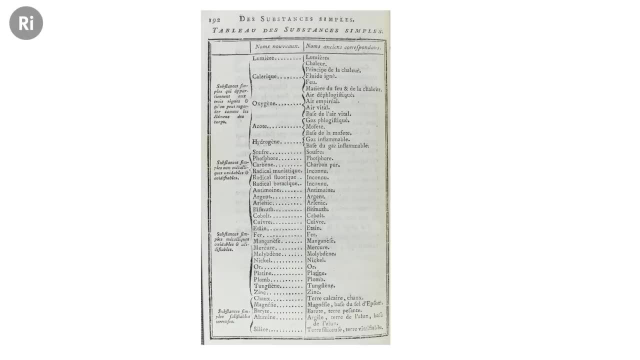 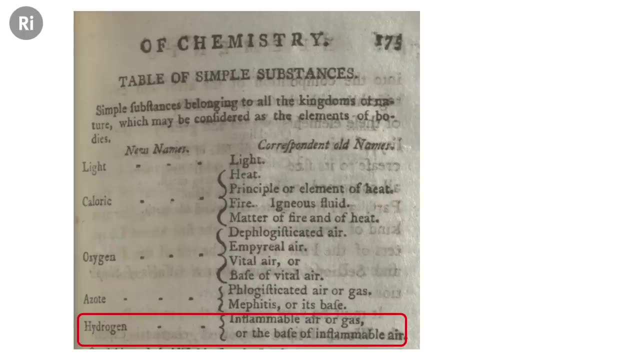 It's in the original French here. We're going to look at this in a little bit more detail, But one of the elements here- this is from the English version- is hydrogen. OK, So he recognizes. In fact, he even gave it its name: hydrogen. 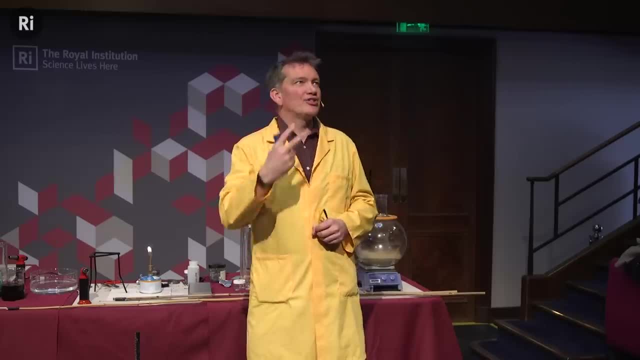 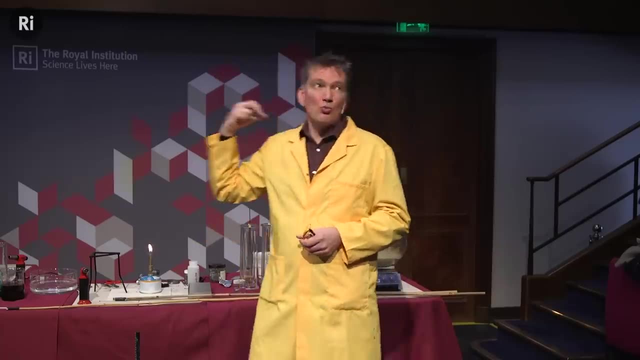 And the name here derives from the Greek Well. of course, I'm sure you know that hydroelectric electric means electricity generated using water from a dam. So hydro means water. This means water maker Because, as you just saw, our hydrogen. 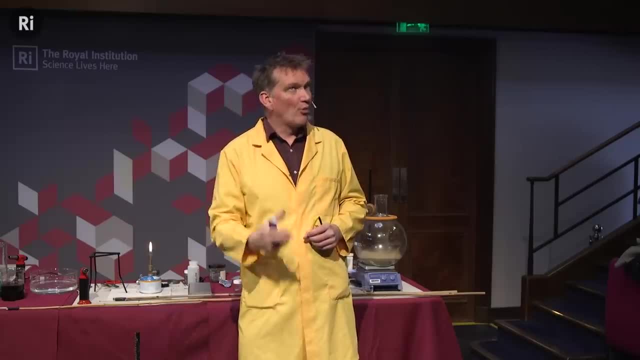 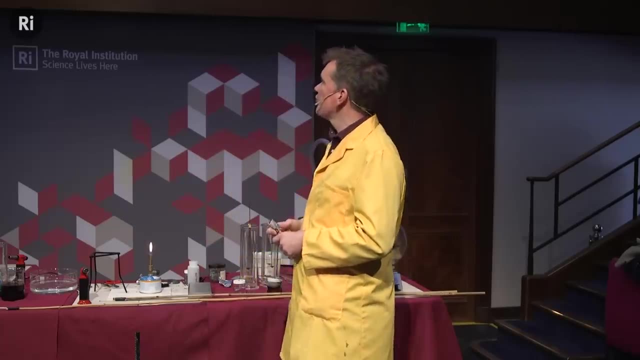 easily reacts with the oxygen from the air to form water. So that's its unique property in a sense, It can easily form water. It's the only element that can form water when it combines with oxygen, So Lavoisier named this because of that reaction. 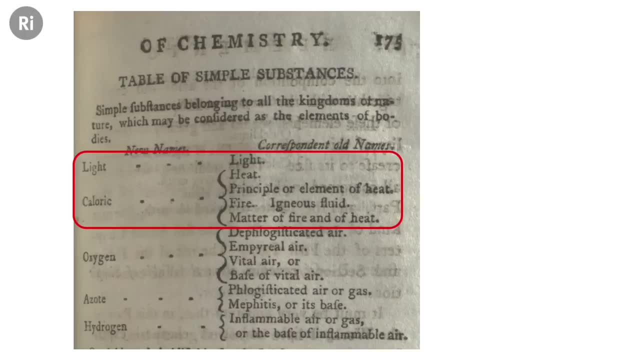 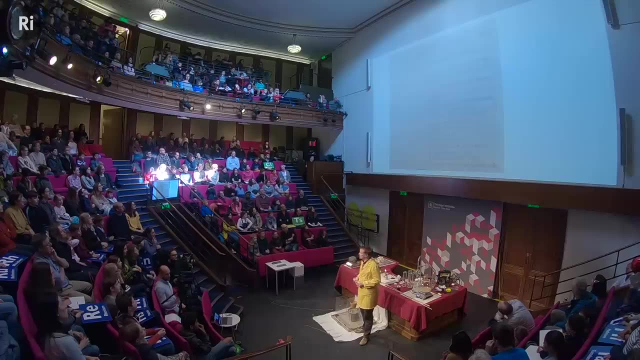 But it was a little bit wrong here, because two of the other, The so-called elements that are in his list- we've got light and what he's called caloric, which is heat- There's another word for that- And this is because he thought that these were also contained. 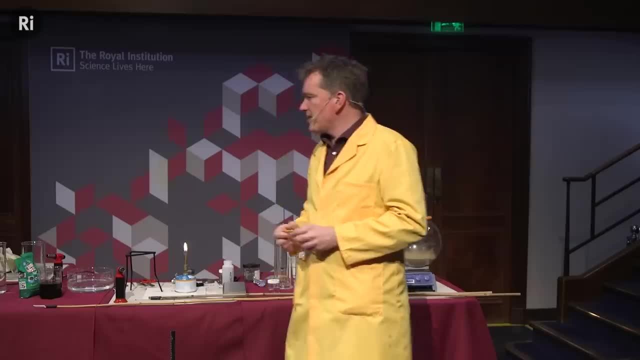 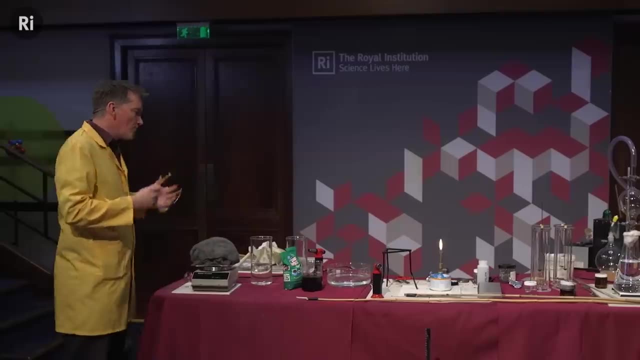 in different substances, And they could be released, And so they must therefore be there Now. Lavoisier made some very, very careful measurements. He measured how much of one reagent combines with another during a chemical reaction, And this was one of the very, very important things. 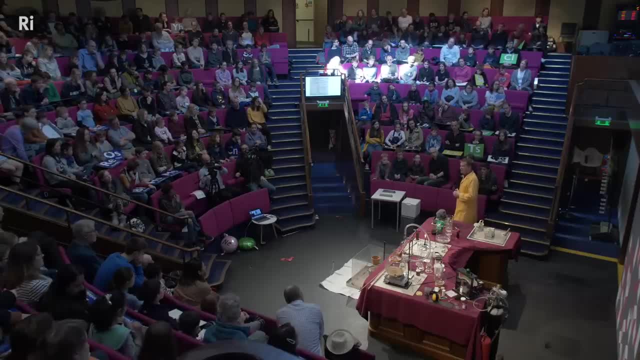 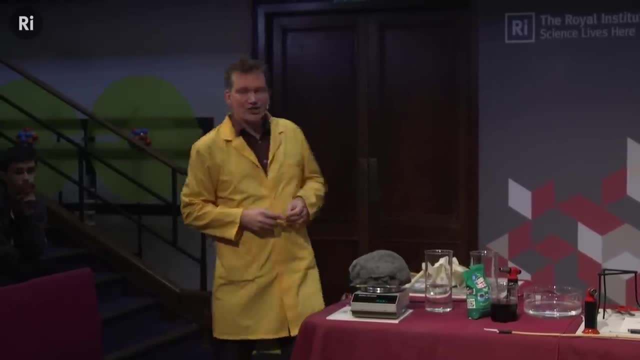 He measured how much hydrogen combines with oxygen, for instance, And this became very, very important later, And we're going to try this in a moment, And we'll also see why he thought that light and heat should be in the list of elements. 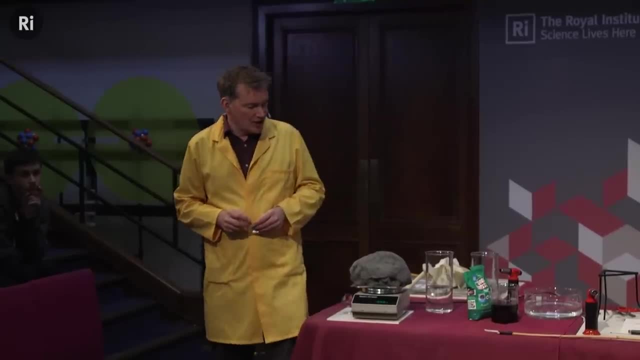 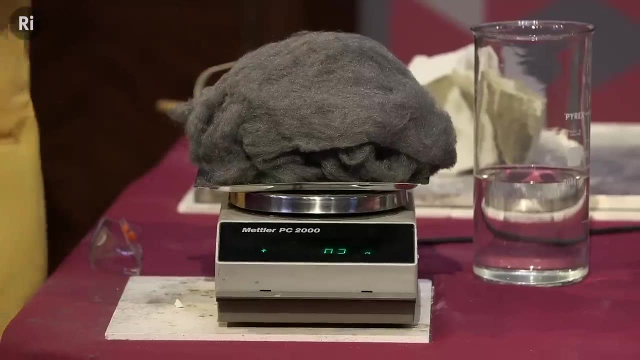 I say we would not include them, now We know that they are forms of energy instead. Well, I have here some iron wool. This is very finely divided iron And we're going to combine this with the oxygen from the air, So it's a chemical reaction. 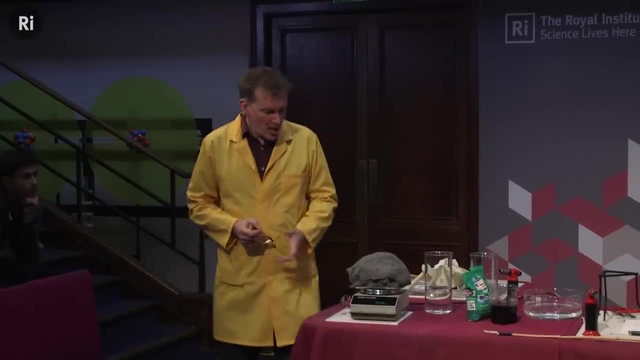 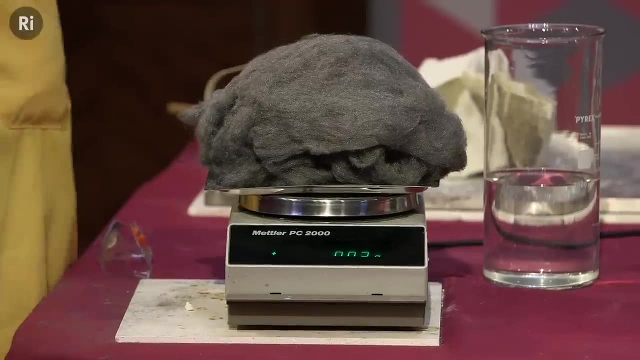 In a sense we're going to be burning the iron wool here. We're going to be seeing how the mass changes. So I've set my balance here to be 0.. And we're going to see if it goes down, if it stays the same. 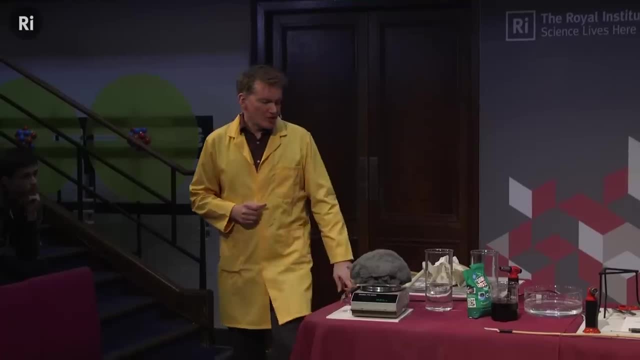 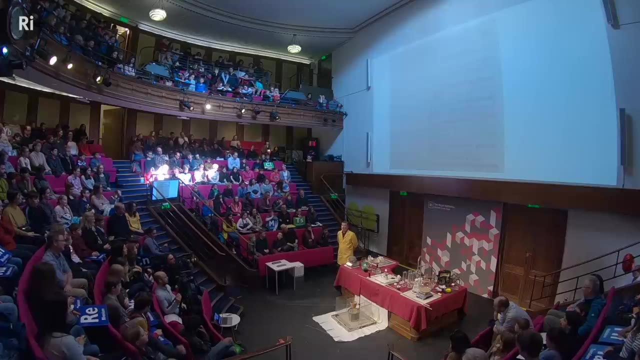 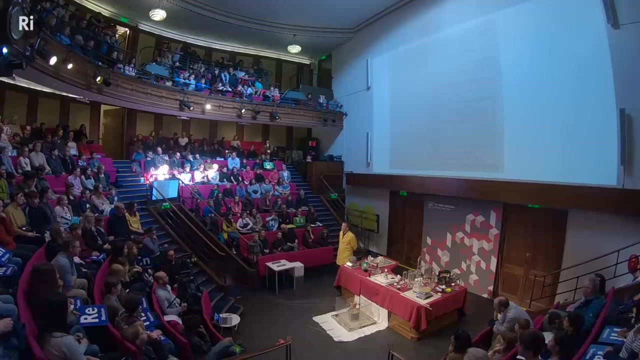 or if it goes up. So we have three possibilities. So actually maybe we'll have a vote. We'll have a vote to see who's right. So who thinks that the mass will stay the same during the reaction? No one. Who thinks the mass is going to go down when it burns? 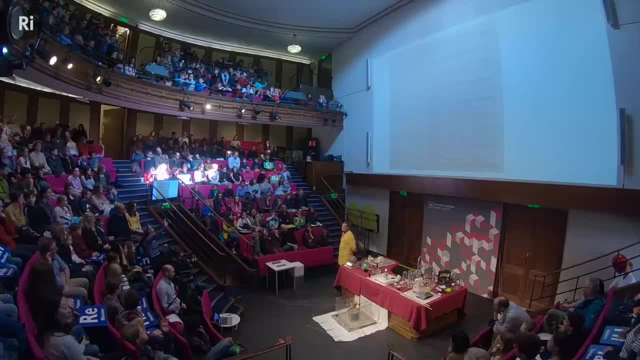 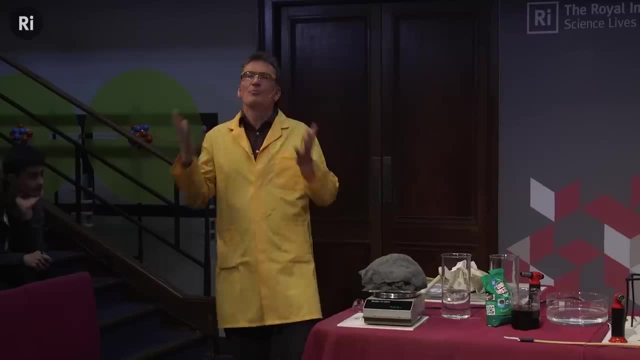 There's quite a few hands there. OK, Quite a few hands. Who thinks it's going to go up? Oh, even more hands. I think if we had to ask the audience, we would say it's going to go up. Well, let's try it. 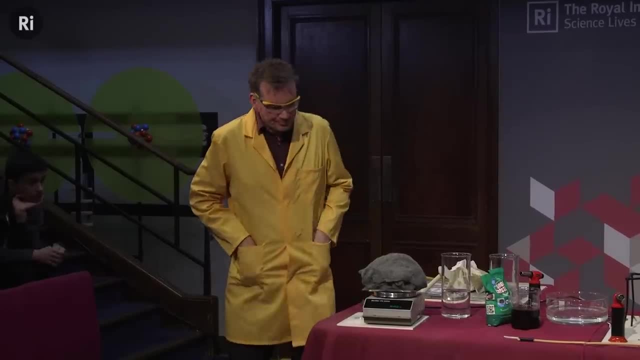 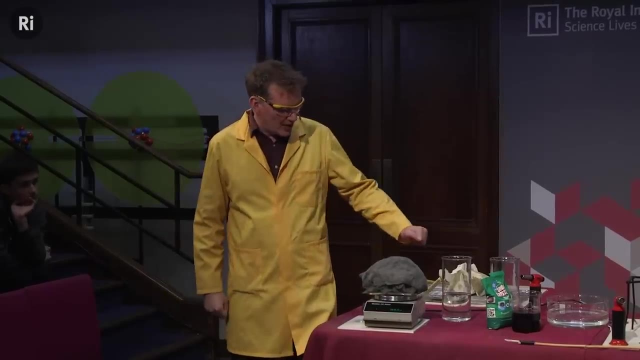 We need to do the experiment, And this is the sort of thing that Lavoisier did. So I'm just going to start this, start the reaction, And actually maybe we could have the lights down for this, perhaps. So I'm just going to start the reaction here. 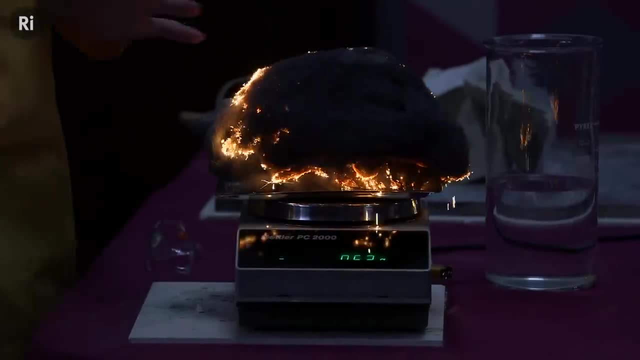 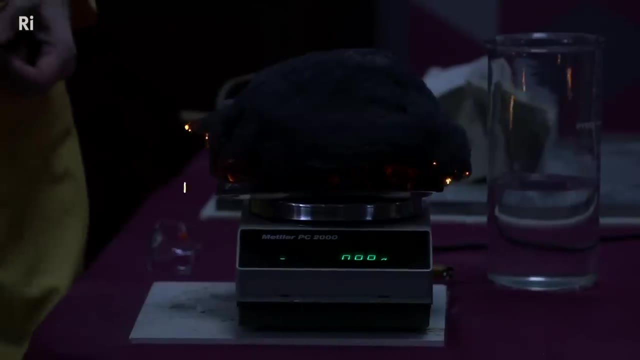 And you can see the beautiful light that's being given out. And this is why Lavoisier thought that light is contained either in the iron or in the oxygen. He thought it was in the oxygen. The mass has actually gone down. 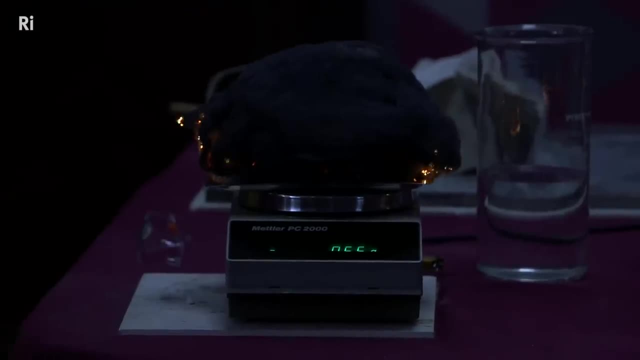 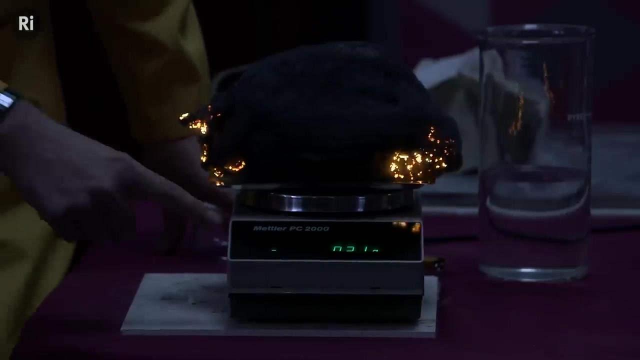 It's almost a gram heavier lighter. So if you said it goes down, you were temporarily right, because it's going back up again. If anyone said it stays the same, well, it's almost back to where we started now. In fact, now it's back where we started. 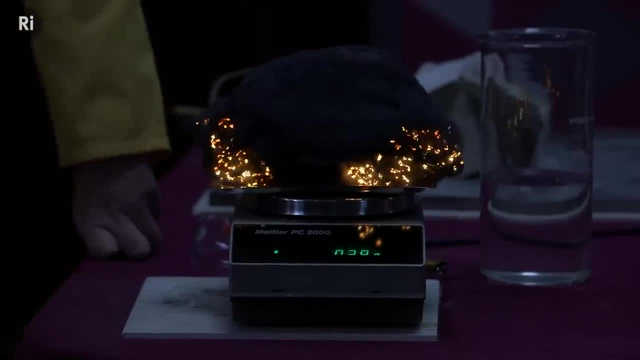 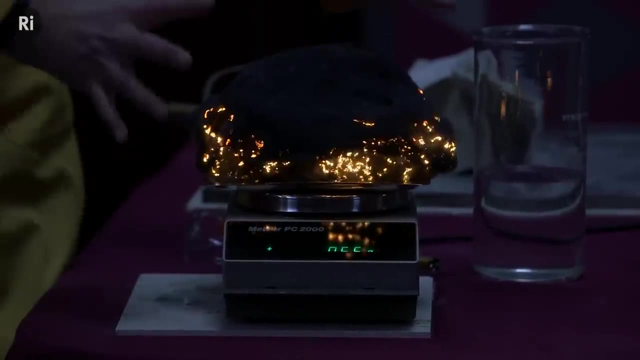 But actually now it's continuing to get heavier. So if you did say it's going to go heavier, you were quite right. OK, now, why is this? Well, I say, We can certainly see the light And I can feel the heat very nicely here. 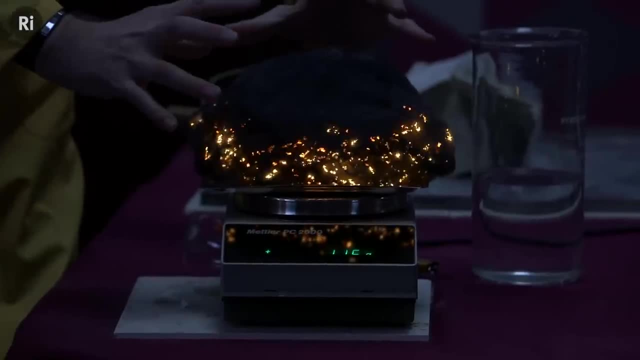 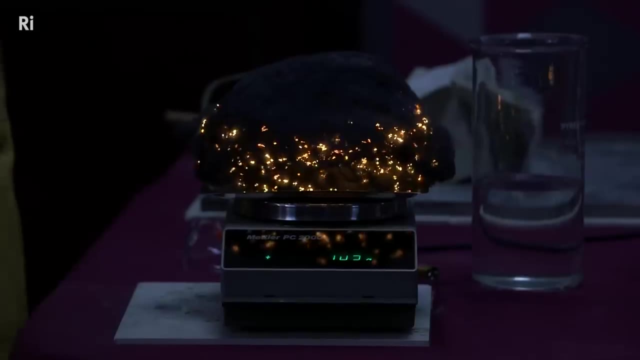 And it's probably this heat that's given out And it decreases the density of the air that's trapped in here. That's probably why the mass went down initially, just as it became a little bit less dense the air there, But it is actually going up. 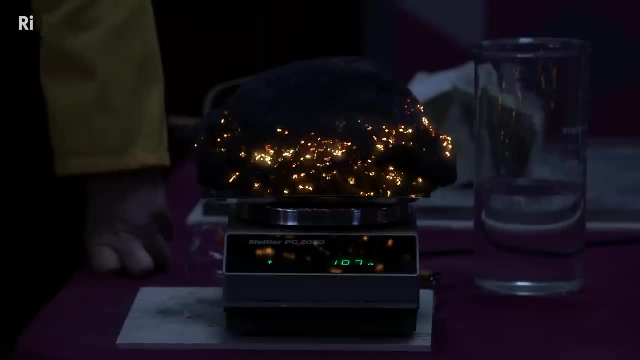 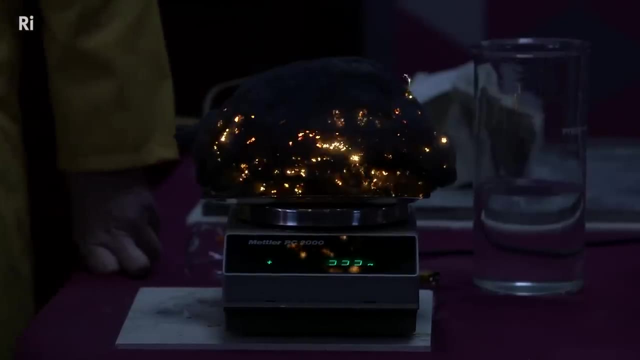 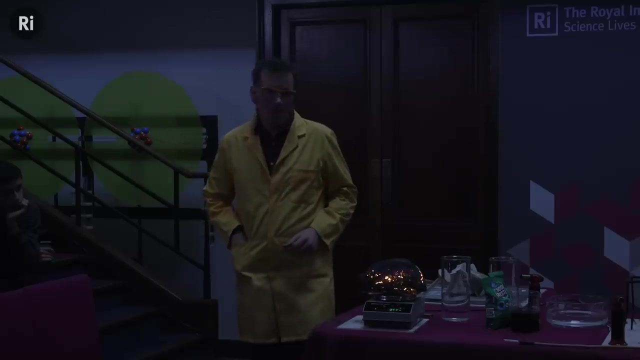 And why is this? Well, none of the iron has disappeared. It's still all there. However, it's now combining, or combined, with the oxygen from the air, And so we haven't lost any iron. What we've actually done is gain some oxygen. 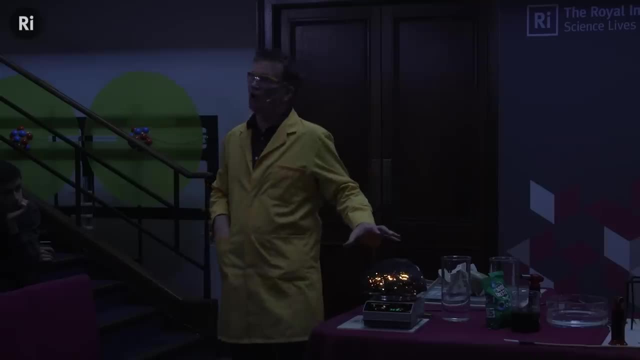 And we've formed iron oxide, So the mass, of course, is heavier, because it still has the iron And now it's also got oxygen built into this structure that we have here, this solid. So it's over three grams heavier now. 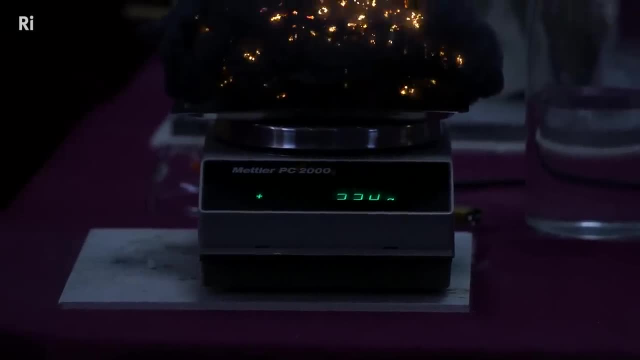 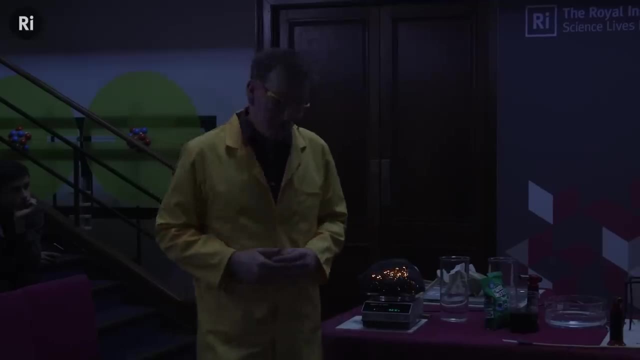 due to the combining mass of the oxygen that's now trapped into the solid here. But we've actually gained some oxygen And we've formed iron oxide, But the light and heat were given out. That's why Lavoisier included them in his list of elements. 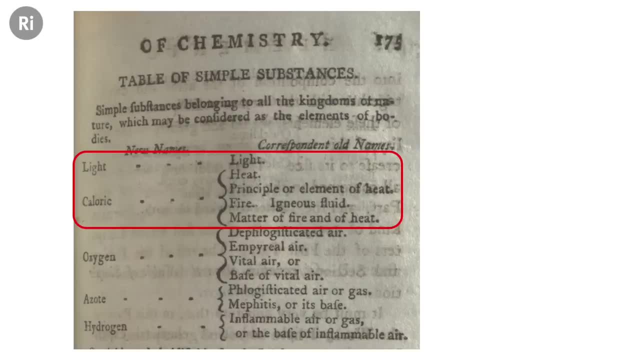 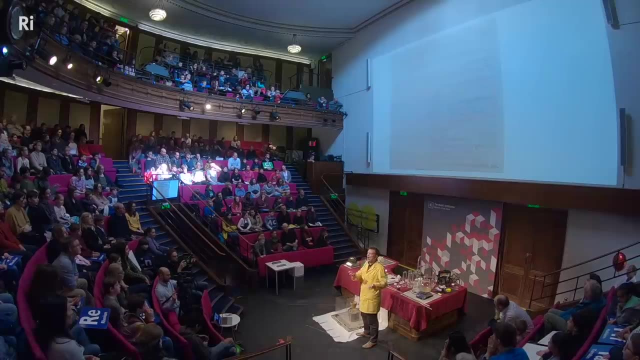 Also in his list we see where we see oxygen. He named the word oxygen as well And azote. well, that was the name that he gave to nitrogen gas. It comes from the Greek meaning no life, because it doesn't support life. It is a suffocating gas. We don't call it that any longer, And that's because actually pretty much every gas is poisonous or toxic or suffocating, other than oxygen. So it's not a unique name. So this is why the name was eventually changed. 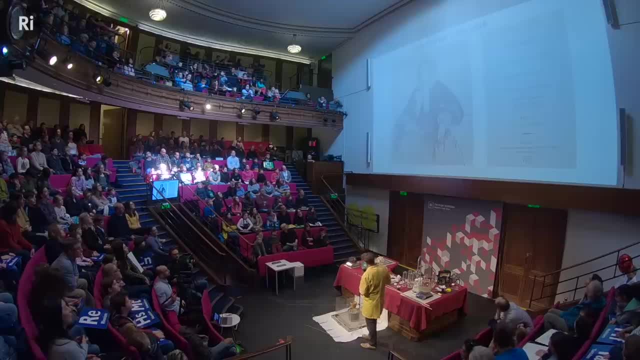 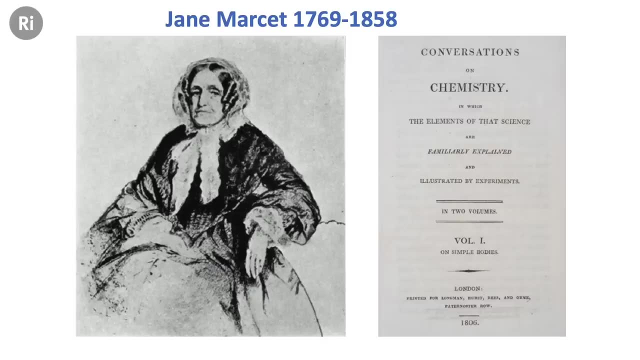 But rather than using Lavoisier's list and going and looking at that further, I'm going to use the list from another of my heroes from this time, And this was the chemist. well, the authoress, Jane Marseille here. 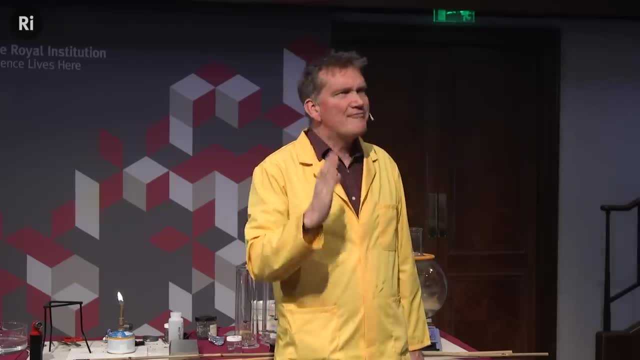 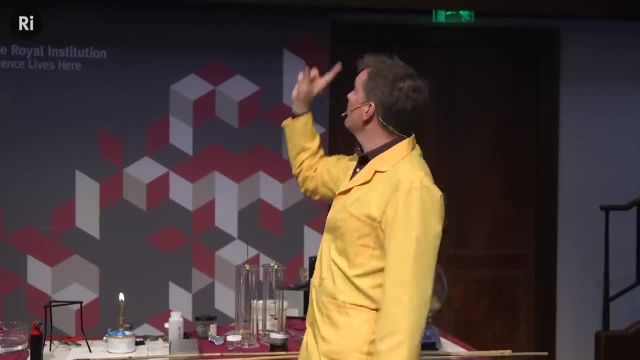 She published a series of books that were really very, very good, And they got a lot of people excited and interested in science and, in particular, in chemistry, And so the book that I'm particularly interested in is Conversations on Chemistry. 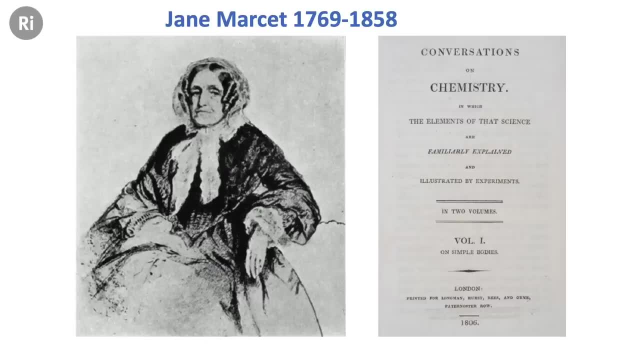 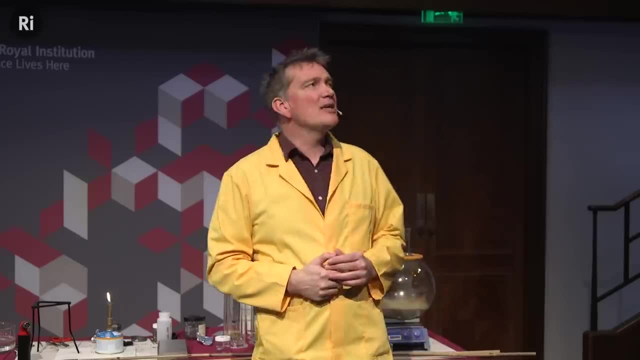 And this really did have quite a huge impact. It went through many, many editions And this is why we're going to be looking at this, because we can see how her list of elements changes Went through many editions, but it also got many people. 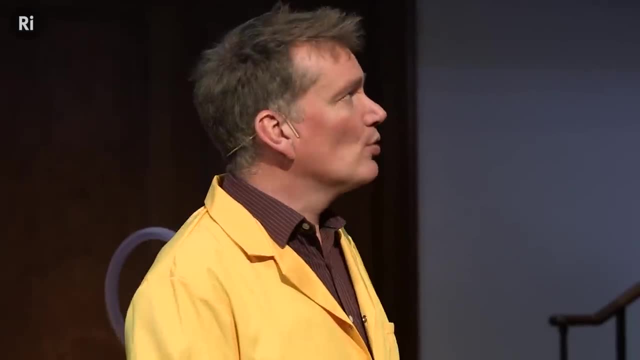 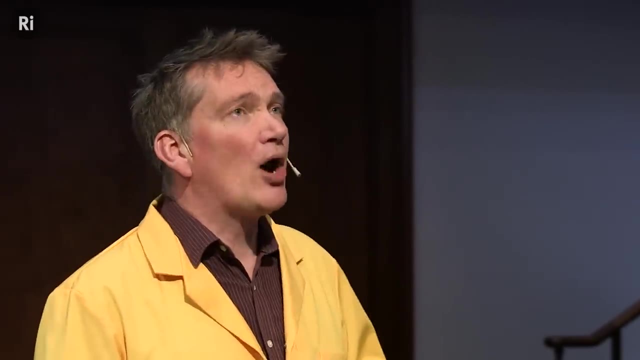 started on science And actually one of the most famous people that got interested in science thanks to her book was a young bookbinder's apprentice, And this is Michael Faraday. of all people, He probably should have been binding the book. 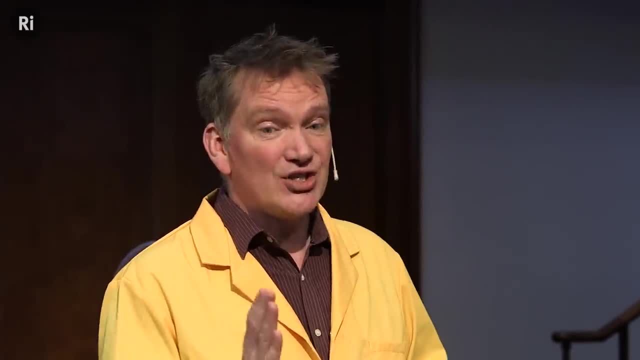 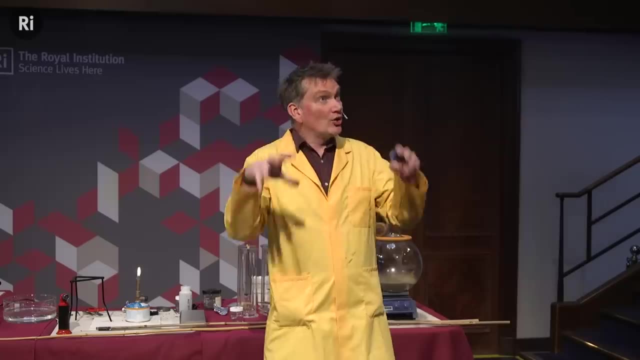 But anyway, he was reading the book and doing the little experiments in here And it got him excited, interested in science. He then approached Humphrey Davy, made notes of his lectures and got a job here in this building And he became one of Britain's most famous scientists. 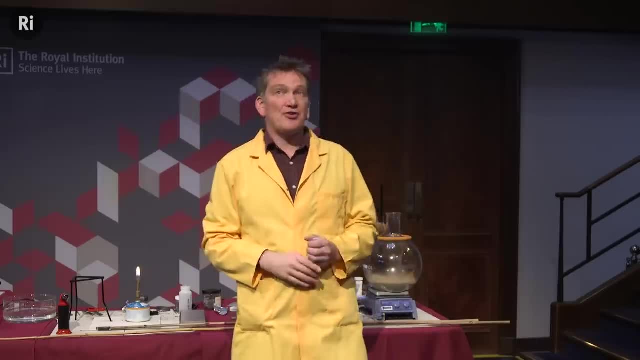 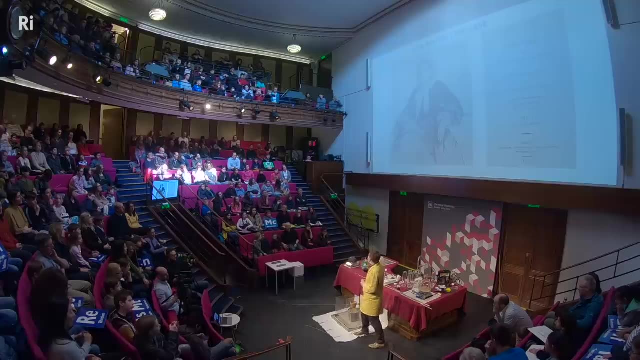 But it all started thanks to this lady. They became good friends throughout their lives. They corresponded with each other. She often came to this very room attending his lectures to hear him talk about science, And then she would update her books with all the new science. 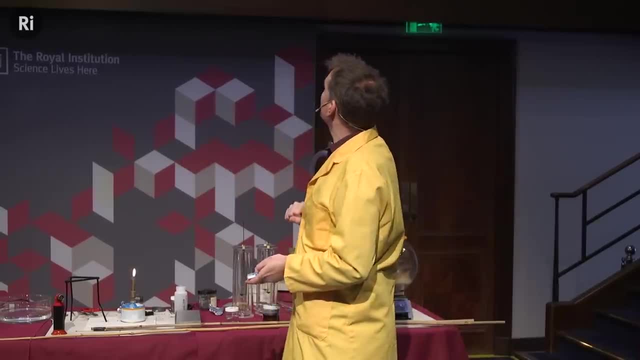 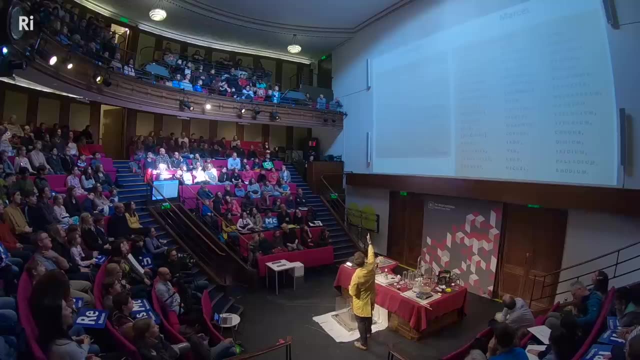 And she would say: well, I've got a book about science there, So absolutely fantastic. But let's have a look at her list of elements from the very first edition from 1806.. And here it is. So it's very similar to Lavoisier's list. 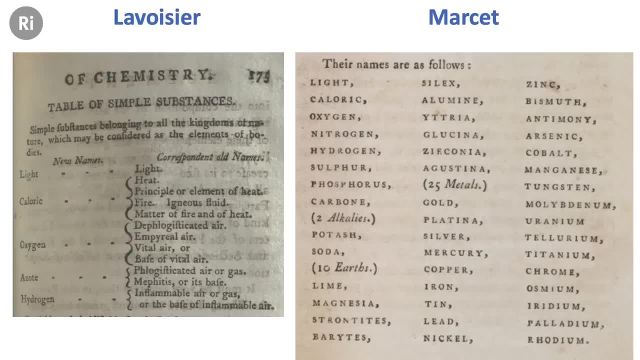 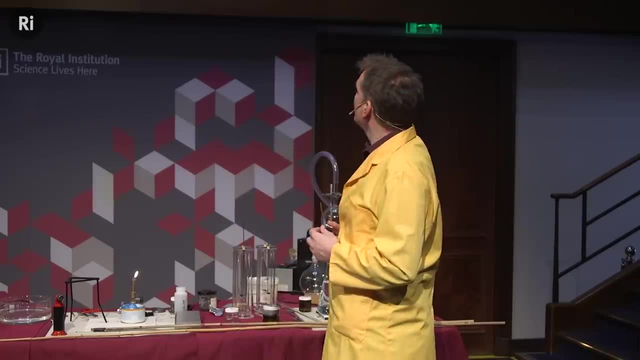 Also, at the top we see light and caloric and oxygen, then nitrogen hydrogen, So it starts off exactly the same. This is because, well, this is the list of elements. There are a few more elements in here than Lavoisier had. 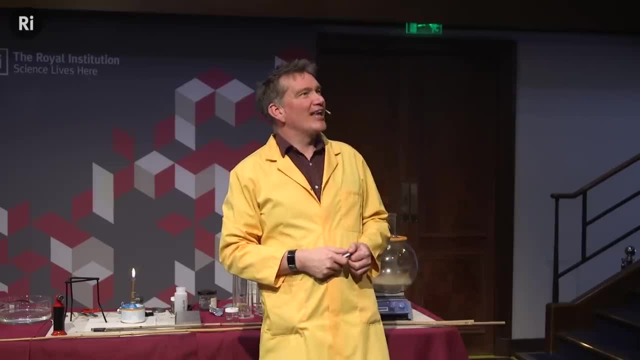 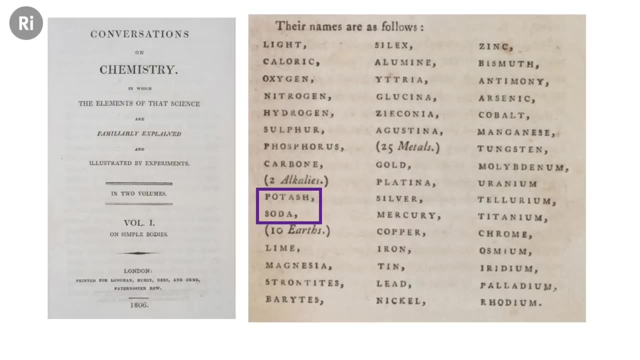 because it's a few years later, It's 20 years later, But there are some things that aren't elements, that are not elements that are in. There are some elements in this list and in this list here- And these are- we see potash and soda. 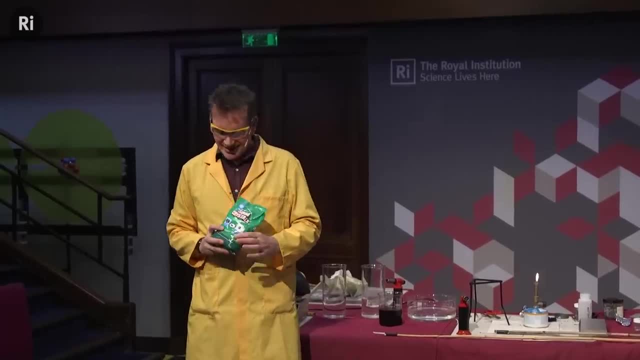 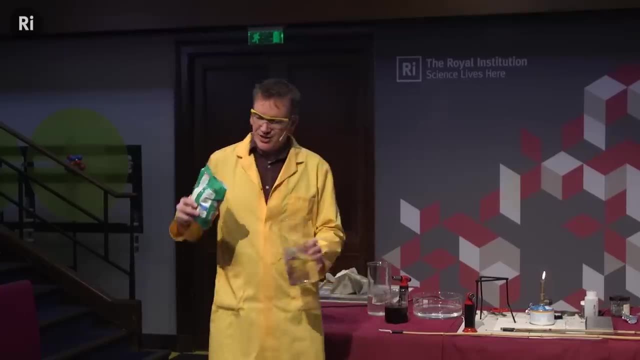 Now I have some soda crystals here. I bought these from Sainsbury's And it's just washing soda. What this actually is is just sodium carbonate And it dissolves in water quite nicely And I could use this to wash my clothes if I wanted. 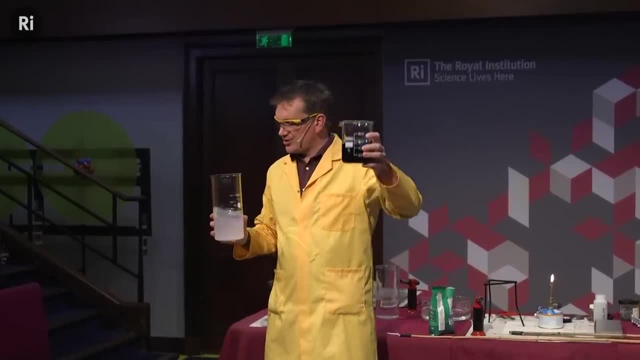 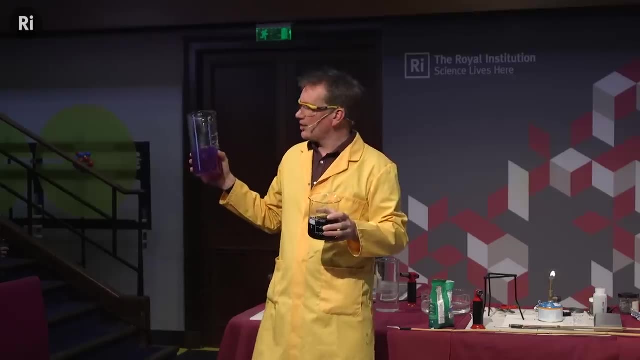 It's an alkaline solution. If I add some of this, this is a very dark green. This shows that it's a neutral solution. If I pour some in here, it goes to this beautiful blue-purple color here to show that it's an alkaline. 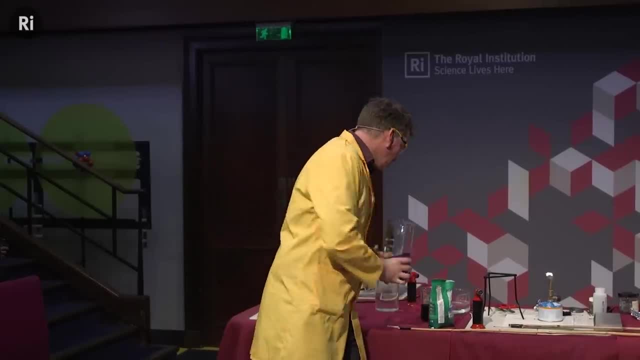 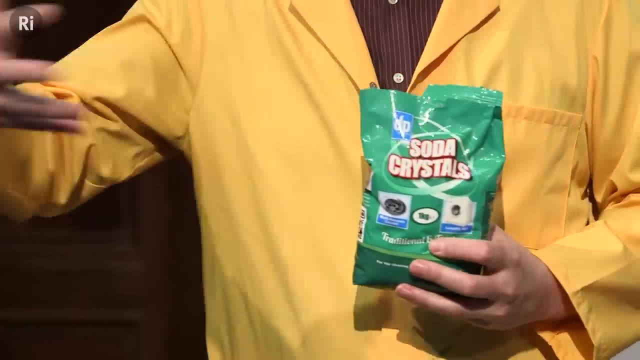 the opposite of an acid. Now why is this in the list? Well, it's in the list because Lavoisier could not break down this substance. He could heat it up to very high temperatures and it would lose some carbon dioxide. 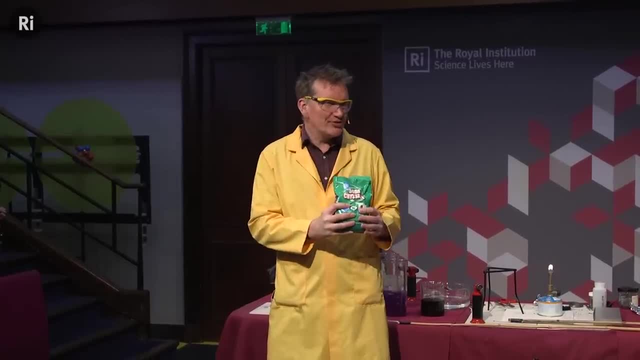 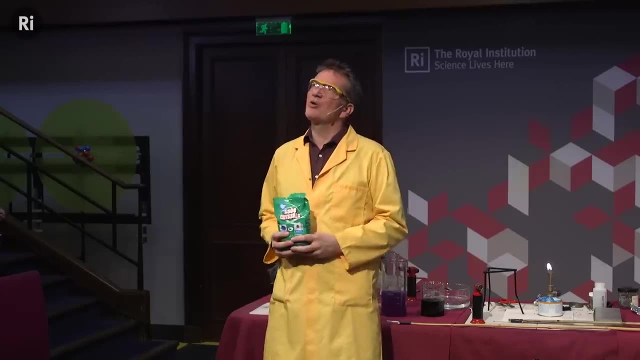 But it couldn't be broken down any further. They couldn't get the real elements out of this. So as far as Lavoisier was concerned, this was a simple substance that couldn't be broken down. He suspected that maybe there would be some element in here. 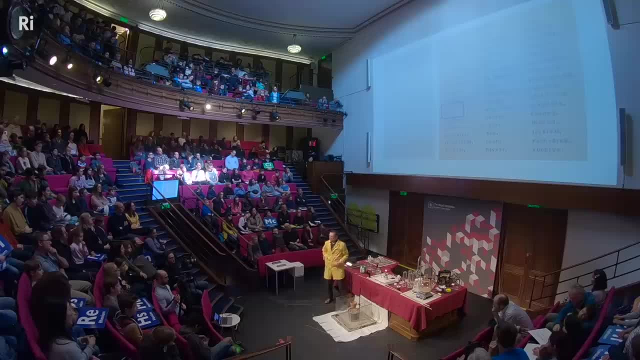 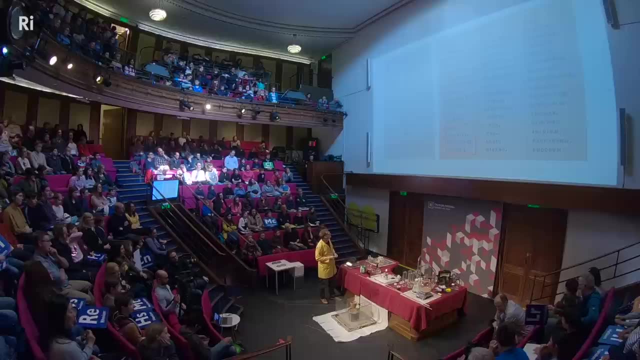 but he couldn't get it. Similarly for the potash that's mentioned here. This is potassium carbonate. This couldn't be broken down either, And we also have some other ones here, So it's lime, magnesia, strontite and barytes. 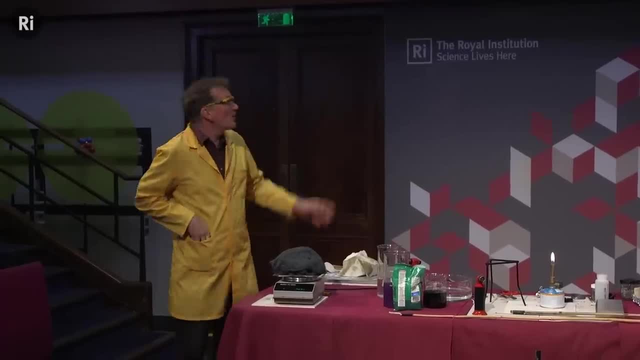 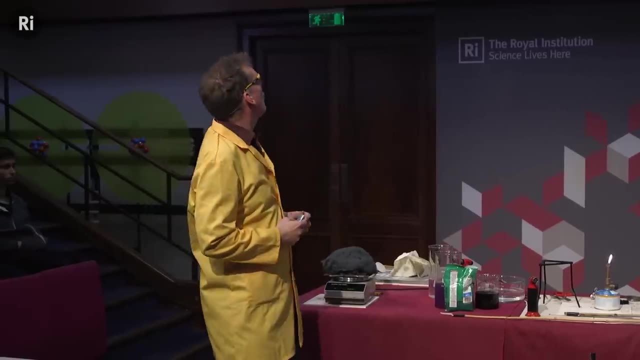 But again, these are substances that could not be broken down. The lime, what it actually is, is what you get if you try to break down, by applying a strong heat, some calcium carbonate. Now, calcium carbonate is commonly known as chalk, or it's a marble. 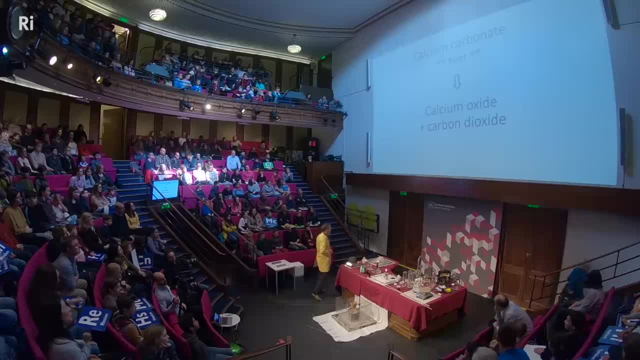 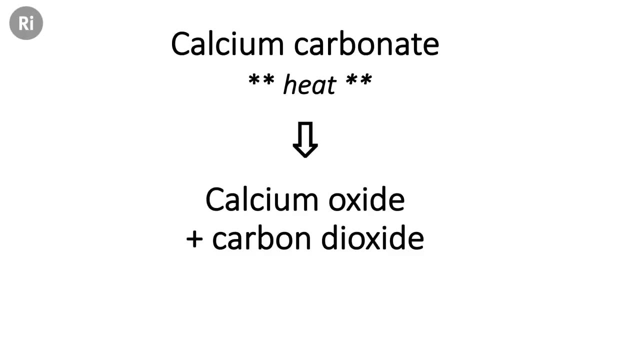 So calcium carbonate. if you heat it up very strongly, what you end up with is lime, And I've got some here. Now we're going to look at this. It's quite an interesting substance, So this was included in Marseille's list. 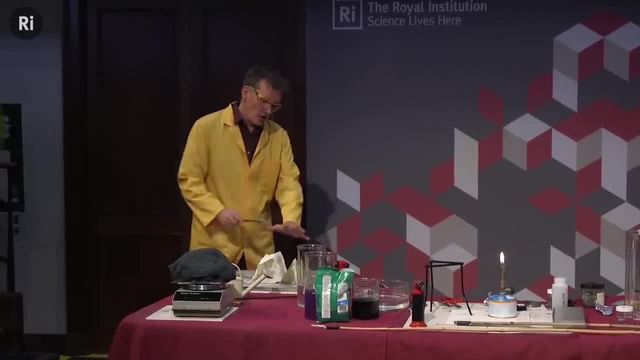 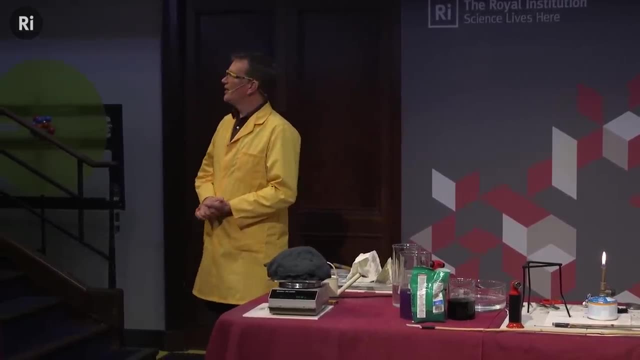 of simple substances. It's quite hard, It's not hot, It's just been lying around here, But it can do something really quite fun And I need a volunteer. Oh, Your hand went up very quickly in the gray. Do you want to come down please? 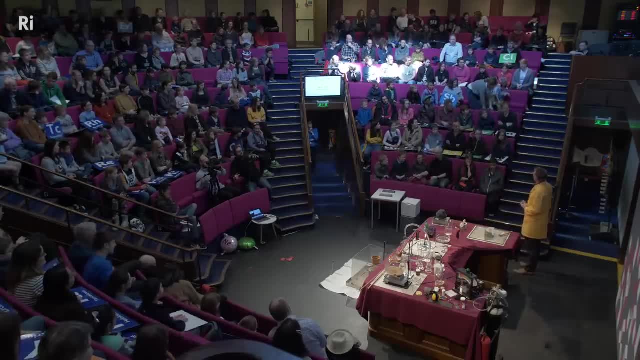 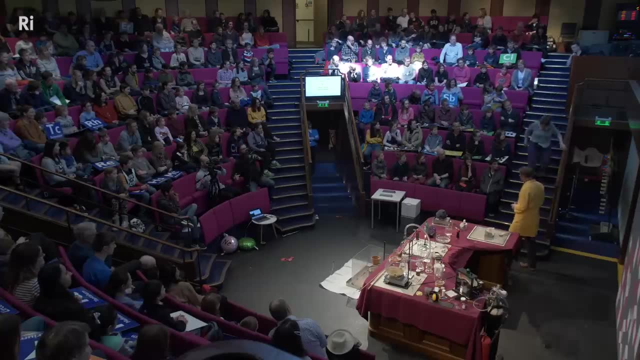 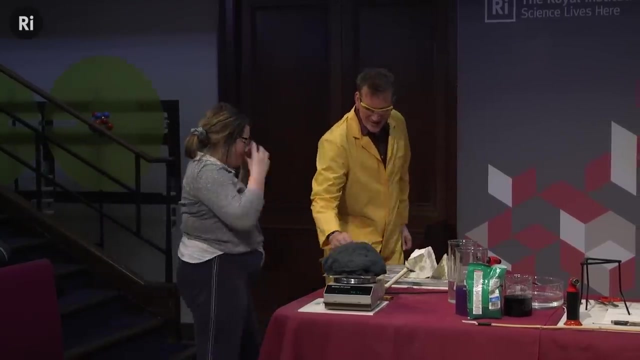 OK, All right Now. OK, Very good, Thank you, And you might need to see if you can put those over your goggles. So extra, extra goggles, This is good. Extra, extra ones. Now get a tiny little watering, can there? 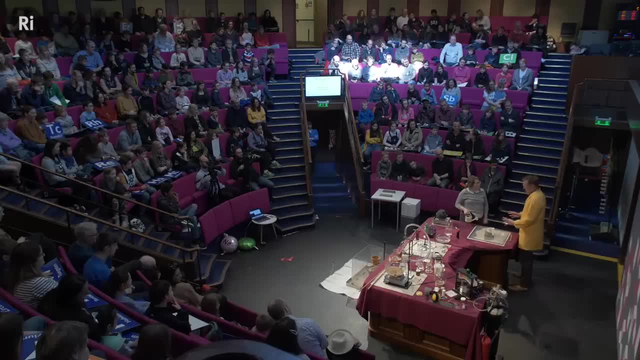 if you don't like to pick up that without spilling too much water- And what I'd like you to do is to pour water all over this- Just flood this And then just step back a bit just over to there. OK, 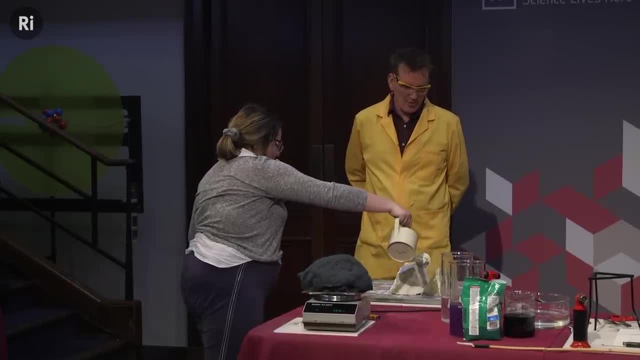 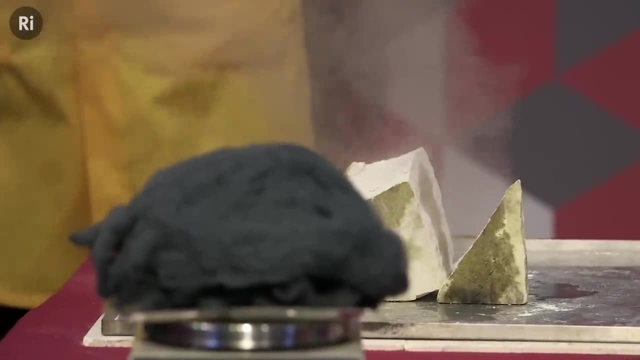 Thank you very much. So if you just pour water all over it, Give it good flooding all over both pieces, That's good, That's very good, OK, And just step back. Thank you, OK. So far Now it was cold. 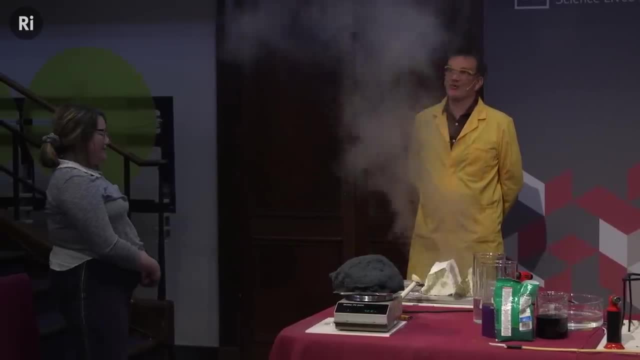 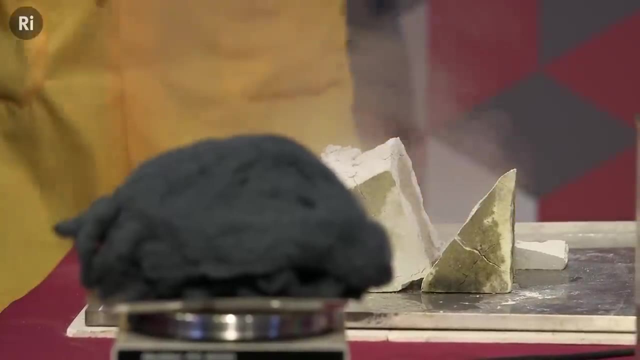 And the water was cold And a violent reaction is taking place. In fact, this reaction is so violent that this is steam being given off, And the reason I had to ask you just to step back there is because actually little bits can ping off of this sometimes. 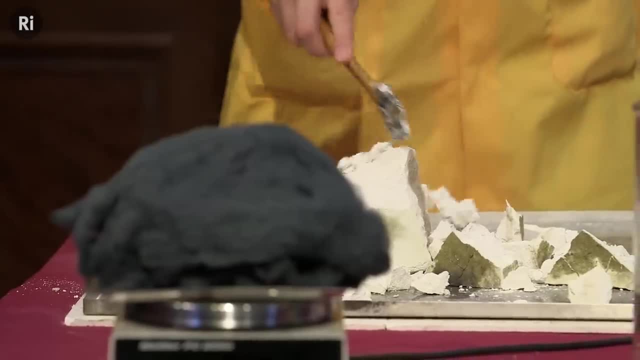 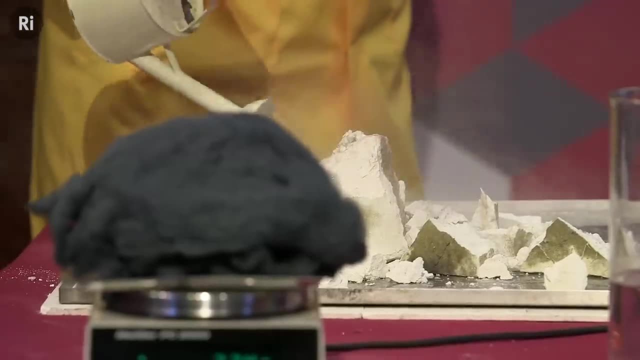 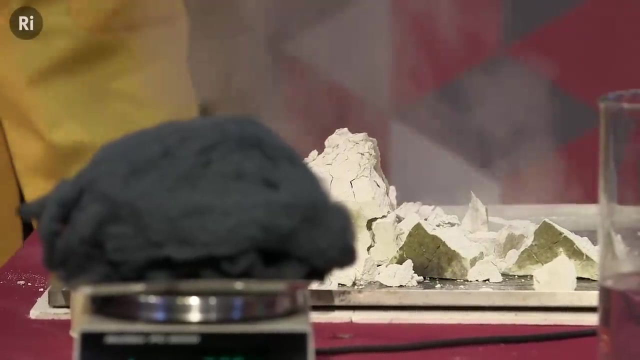 It really just depends. So now it's much flakier. I'll add a bit more just to get it right in there. So the substance was lime. Well, lime is sometimes also used for calcium carbonate itself, But this substance really is also known as quick lime. 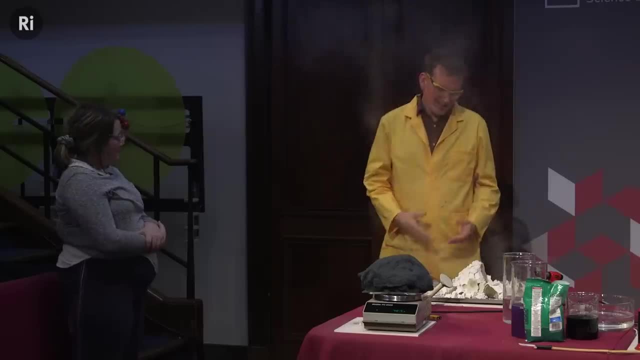 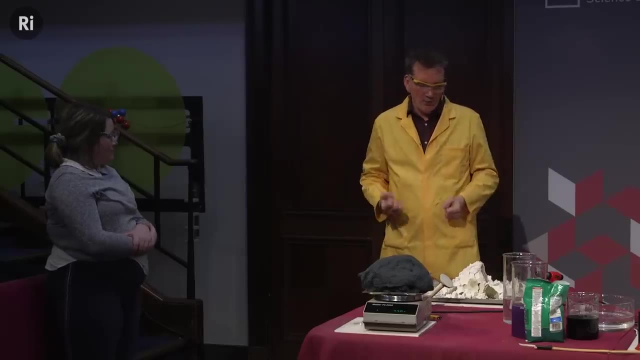 And the quick here doesn't mean it's fast, because it isn't really very fast. Quick is an old word meaning living, So for instance, Quicksilver means living, Silver is mercury. We have the quick of our fingernails. 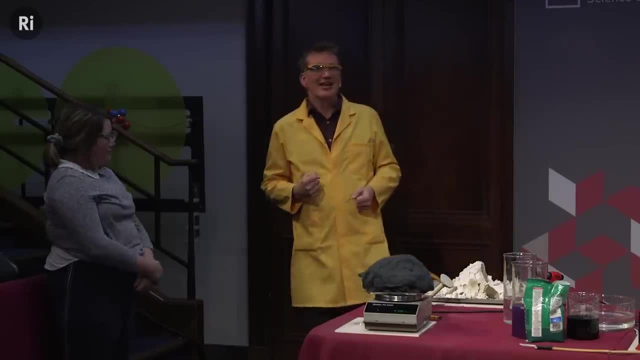 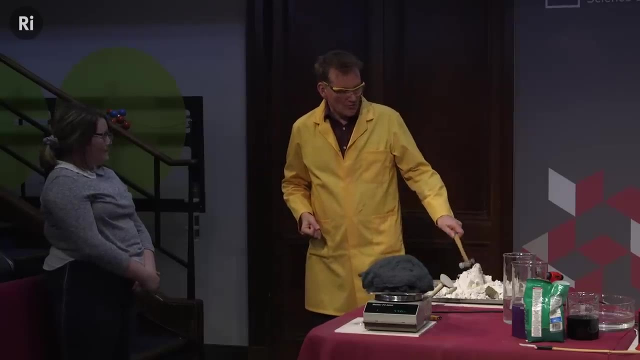 the living tissue there. And there's a phrase: the quick and the dead. It doesn't mean the fast moving and dead people, It means the living and the dead. So this is a living rock, This living lime here very violently reacts with the water. 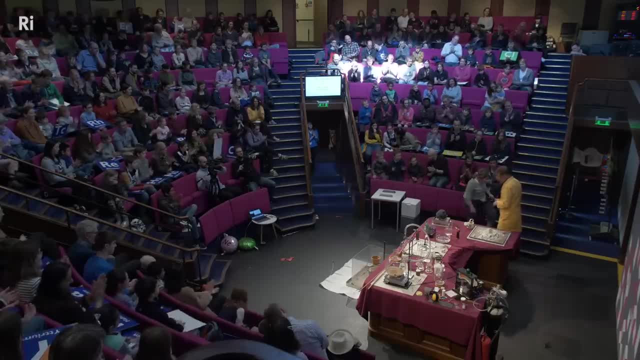 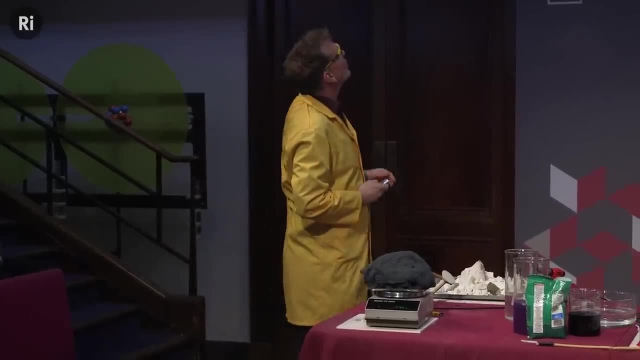 I think a round of applause there. Shall I take your goggles there. Thank you, Yes, Thank you very much. Thank you. The chemical reaction taking place there, the calcium, the oxide that we have, reacts with the water And it forms calcium hydroxide. 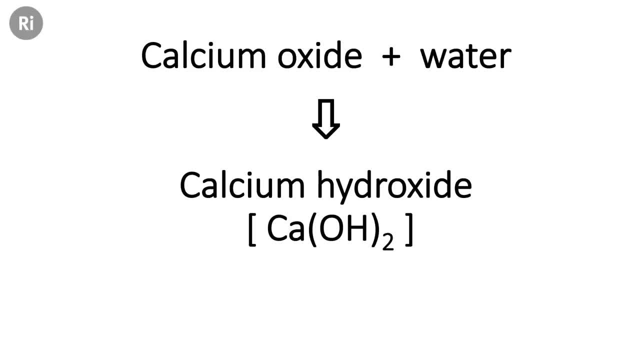 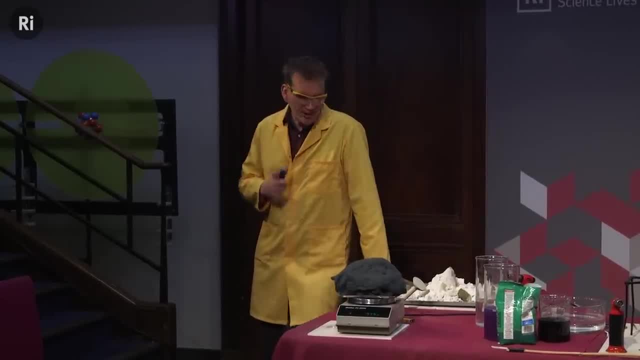 This doesn't dissolve very much in water. This is sometimes called an earth. It does give an alkaline solution. These were eventually called alkaline earths, But they couldn't be broken down any further at the time, So they were simple substances. 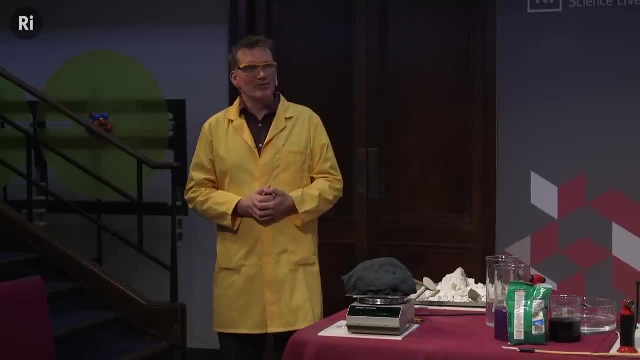 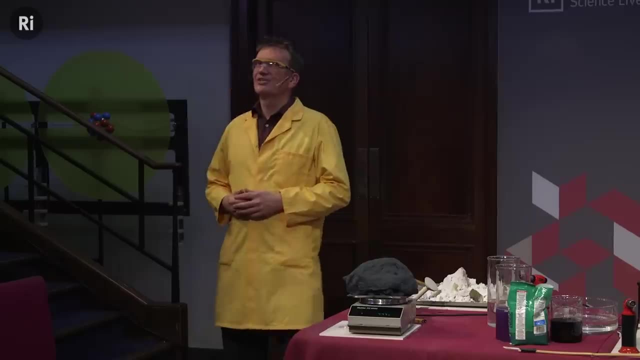 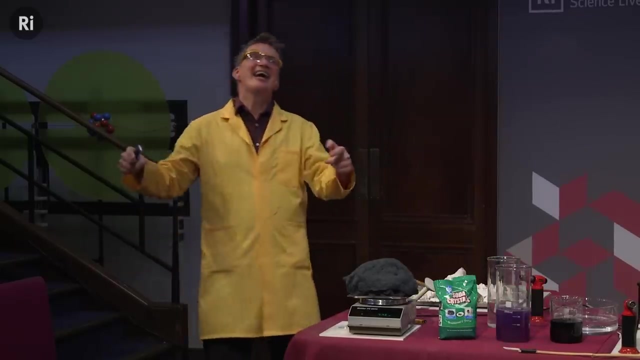 They were, as far as Lavoisier was concerned, elements, simple substances. But then what happened? well, somebody did actually manage to isolate some elements, not only from this, also from our soda, And this was Humphrey Davy, here, in this very building. 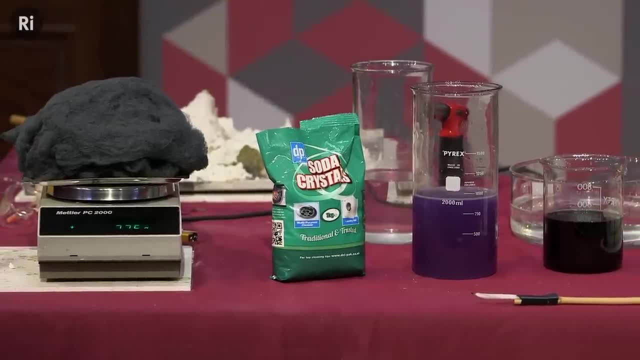 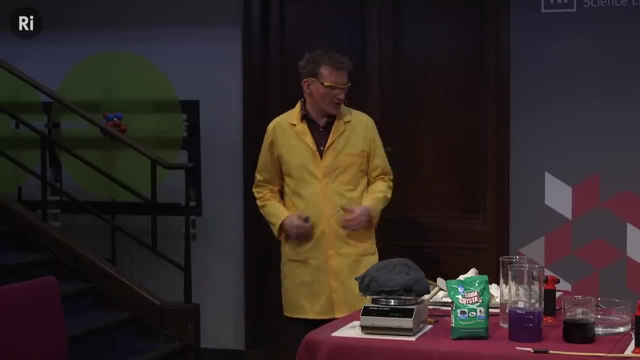 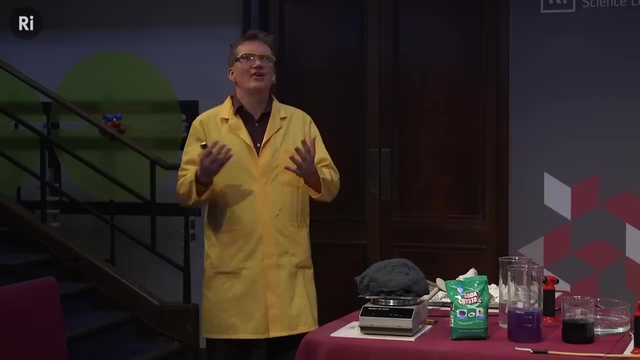 He isolated from the soda. he isolated a new metal that he called sodium, because it was in the soda. From this substance here he isolated a metal that he called calcium. Now, so these elements now appear in the next edition of Marseille's book. 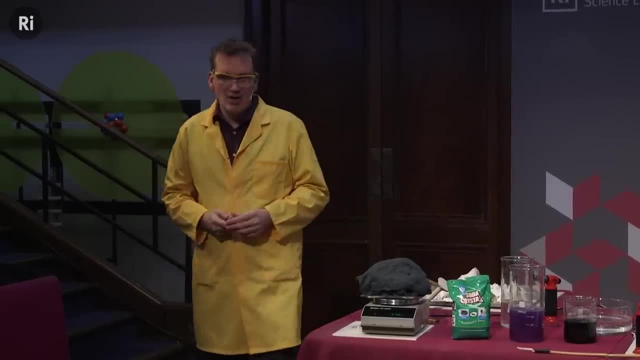 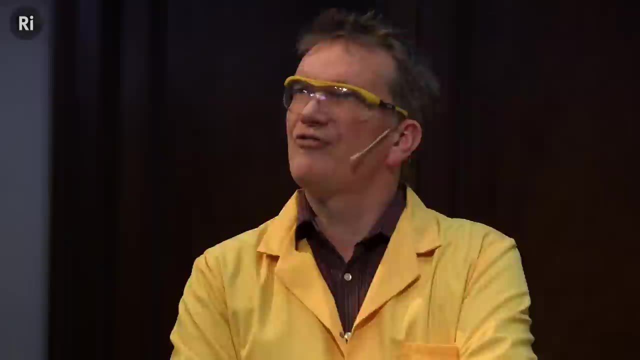 OK, OK, So these new metals that really are elements. they feature in here, But she needed a way of trying to classify these because this is some 50 years or so- or more, 60 years- before the first periodic table. So this list is getting quite long of elements. 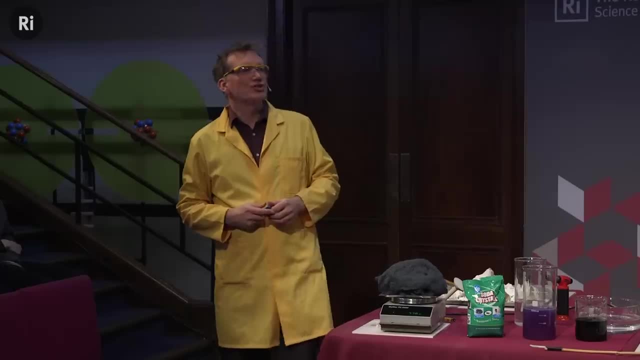 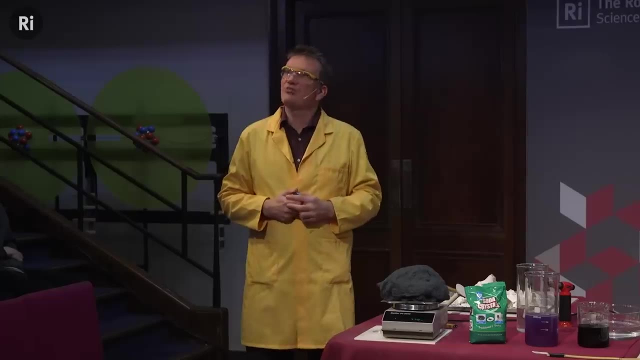 And she thought, well, how can I divide it up sensibly? And so what she wanted to do is to classify things about how they react with oxygen. OK, So, because most of the elements, almost everything, and of course the noble gases, weren't known at this time, 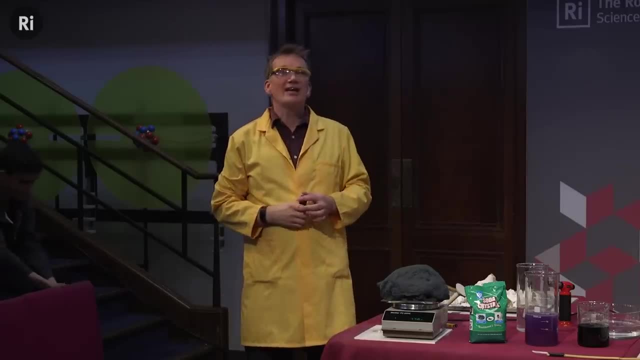 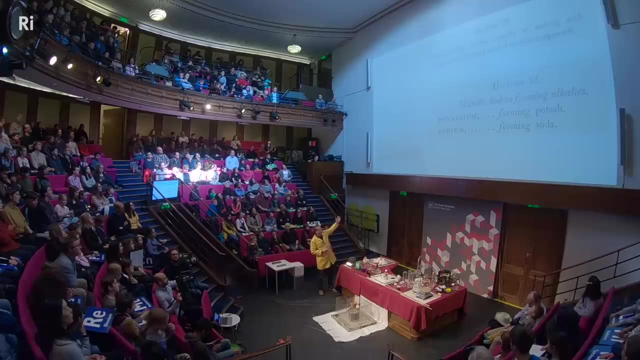 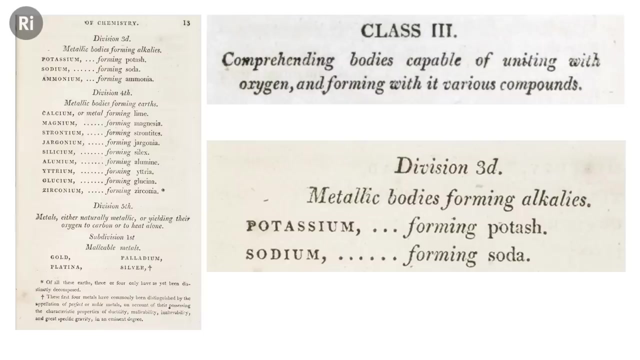 almost everything combines with oxygen, So this was a nice, convenient way to classify the elements, how they react with oxygen. So in the well second edition, third edition, she says here: these are metallic bodies that form alkalis, And so this is now the metal, potassium that forms potash. 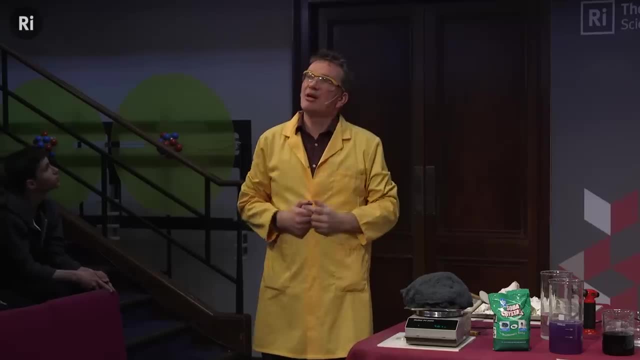 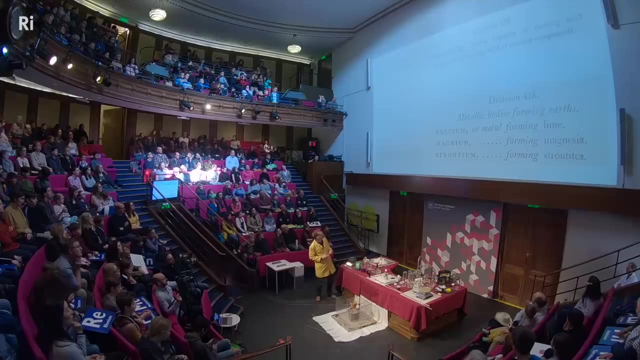 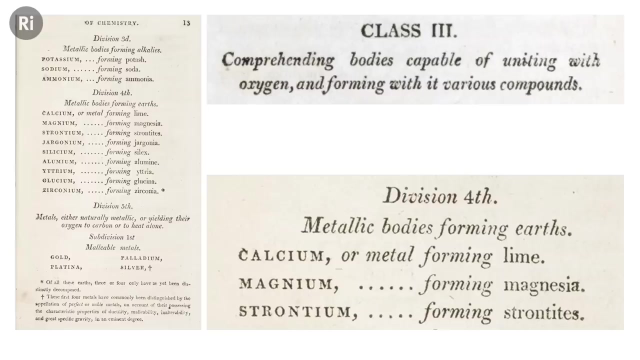 and sodium that forms soda. So these are the metals that were newly isolated. We shall look at these in a moment. OK, We also are. We also have. We have the metal calcium that forms our calcium oxide here, Initially Davy when he first isolated these. 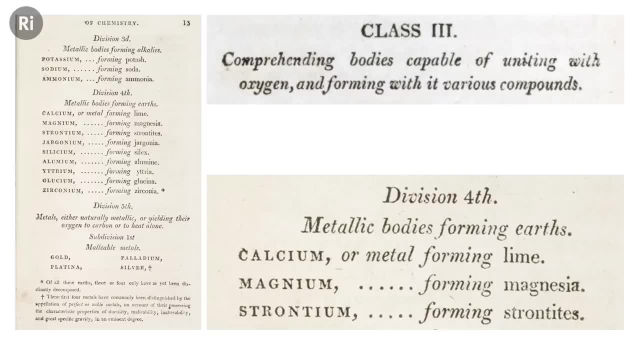 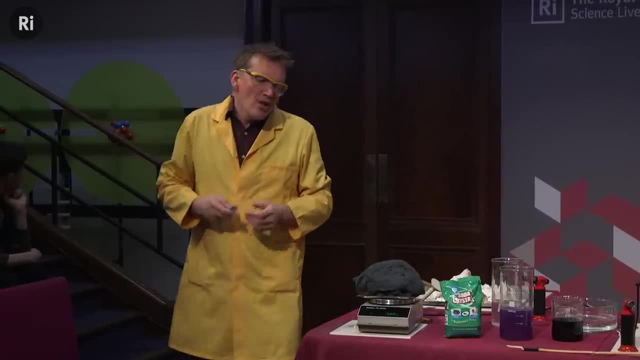 and proposed the names. he named magnesium. He called it magnium for various reasons. Eventually this became magnesium. So these are the new metals that were isolated. Now, this idea of how the elements react with oxygen is something that also Mendeleev picked up. 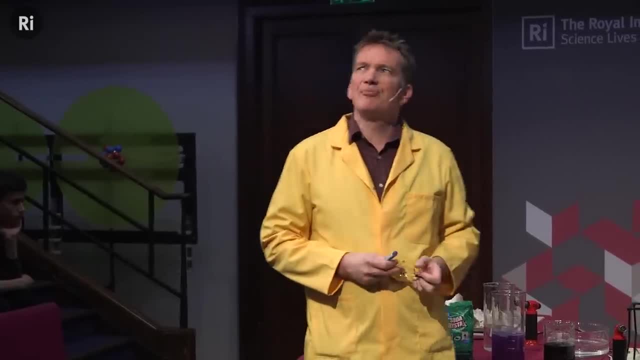 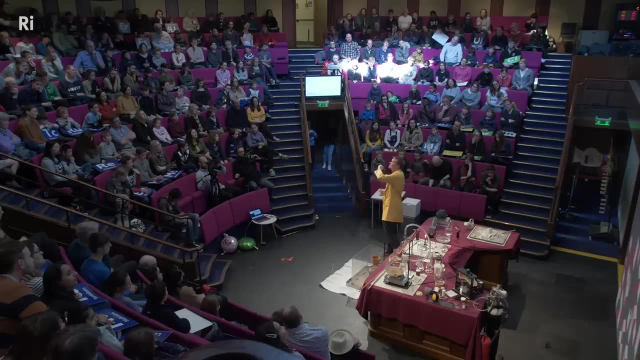 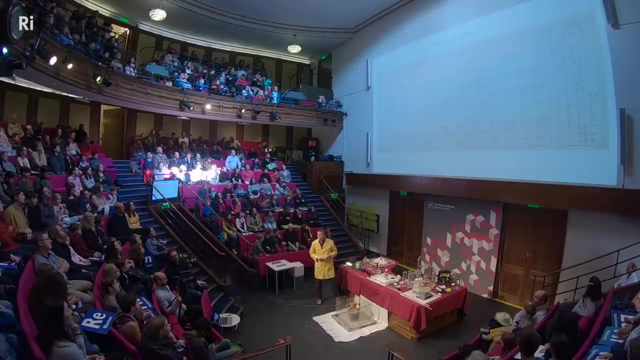 on in his periodic table. So remember, the very first one was published in 1869. This was in the first volume of his textbook. Well, in that one, actually, the groups of similar elements went horizontally across the page In the next version that he put together two years later, 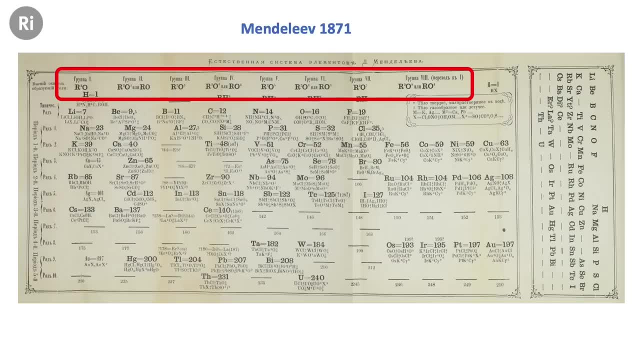 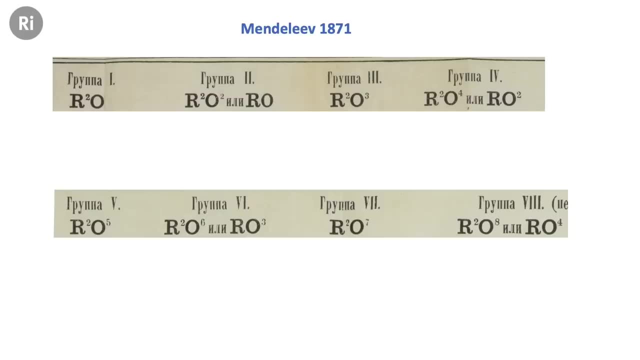 which came in volume two of his textbook. he now has the groups of similar elements going vertically. But what I wanted to draw attention to was what's right at the top. there He calls these vertical arrangement groups of elements. It's in Russian. 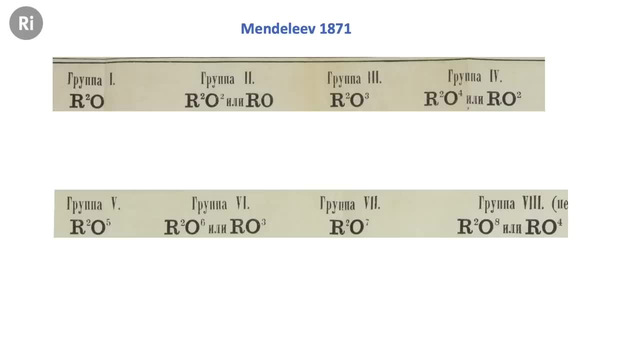 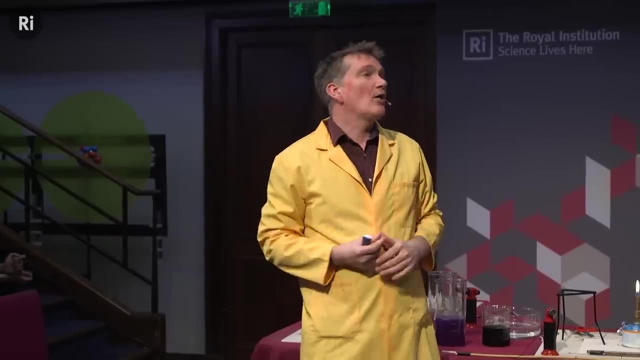 It says grouper, Grouper one, two, three and so on. But he also gives these generalized formulae for the formula of the compounds when they react with oxygen. Now, so the general formula is that we have two atoms of the element with one atom of oxygen. 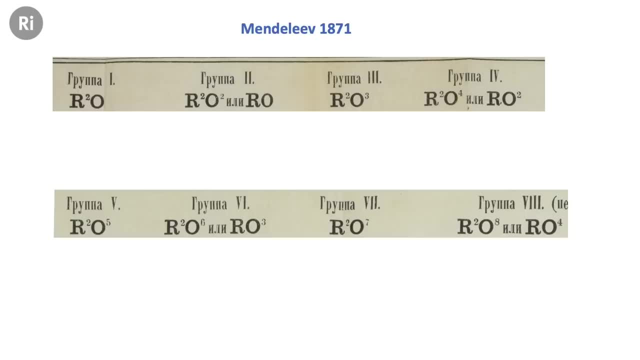 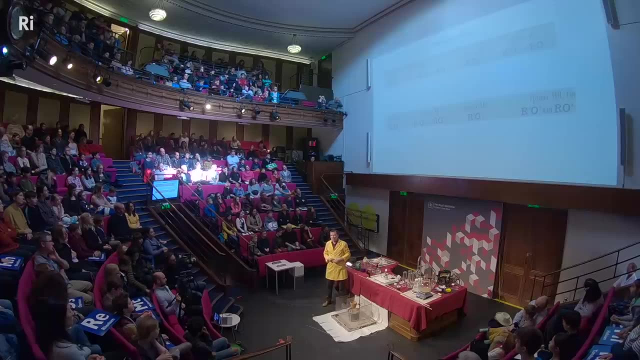 then one to one, or, as he writes here, two atoms of the element react with two atoms of the oxygen, and so on. So there are these different trends as we move across the periodic table, So according to how they react with oxygen. 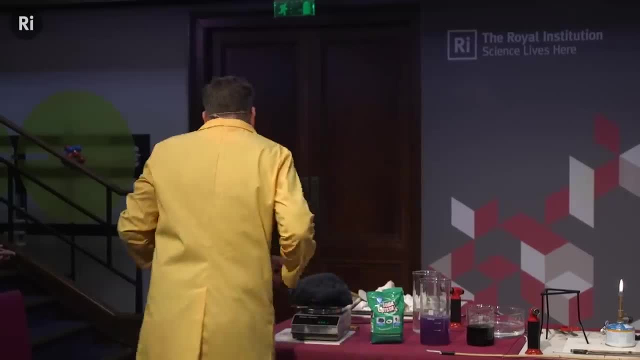 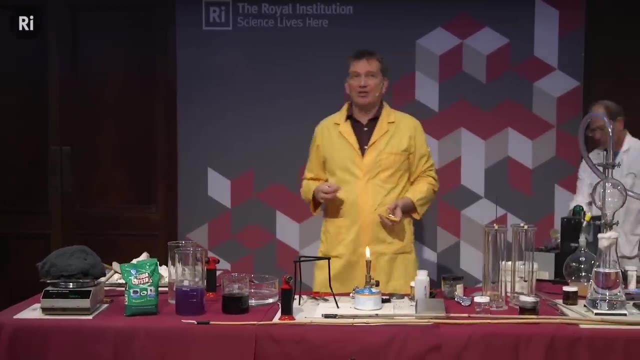 And this is what we're going to look at now. So we'll start off with group one. In fact, we've already seen one of the elements and how it reacts with oxygen. This is, of course, the element hydrogen, And we know the formula of what we get. 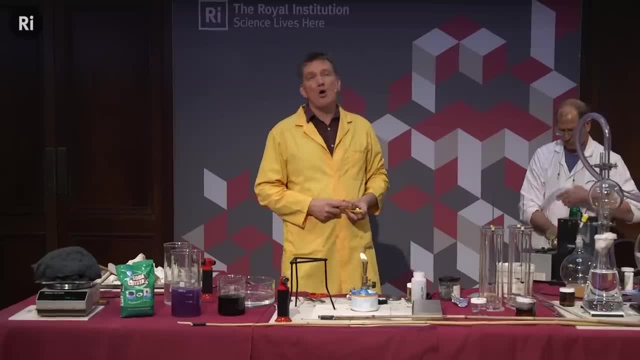 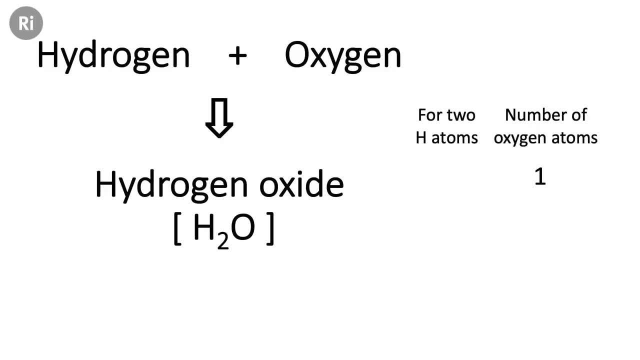 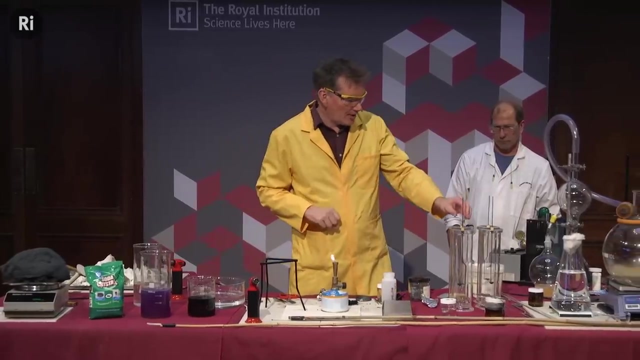 When hydrogen reacts with oxygen, we get H2O. So two atoms of the element, two atoms of hydrogen combined with one of oxygen. But it isn't just hydrogen that this is the case. Other elements can also form similar Compounds with similar formulae. 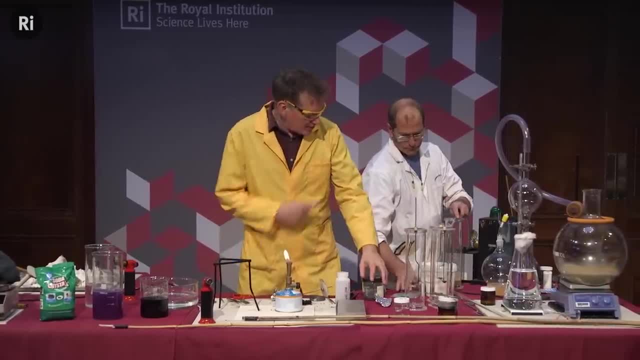 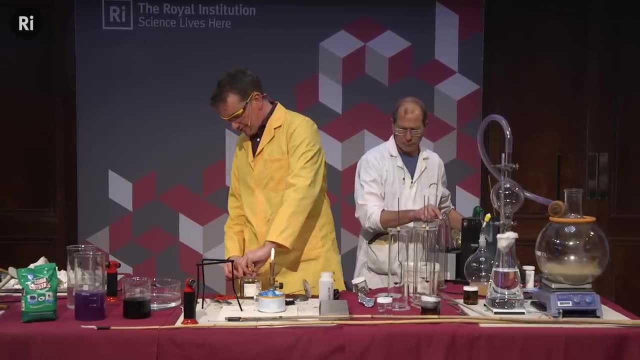 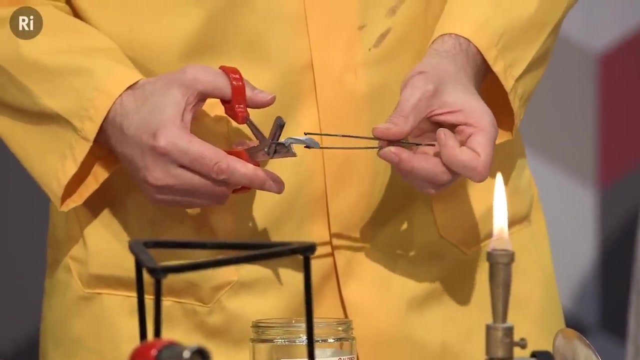 I'm going to show now a reaction of lithium. So Chris, here is just putting some oxygen into the gas jar And I'm going to take a little piece of lithium. So this is lithium foil. So I can easily cut this with the scissors here. 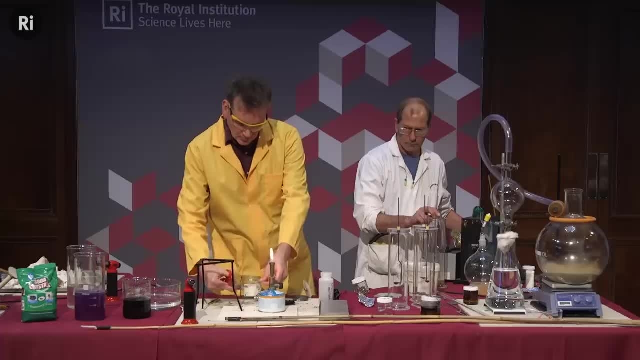 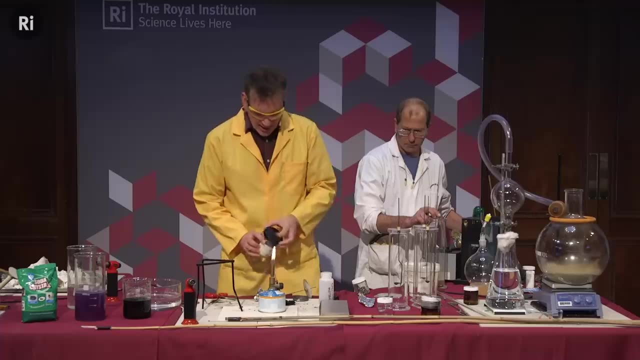 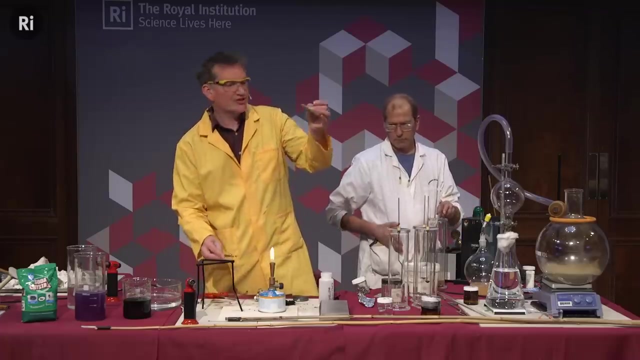 So I'm going to cut a little piece of foil. Actually, I'll take a little snip. another little snip off there We can use in a moment. I'm going to go for a different reaction. Excuse me, I'm going to put my lithium on this. 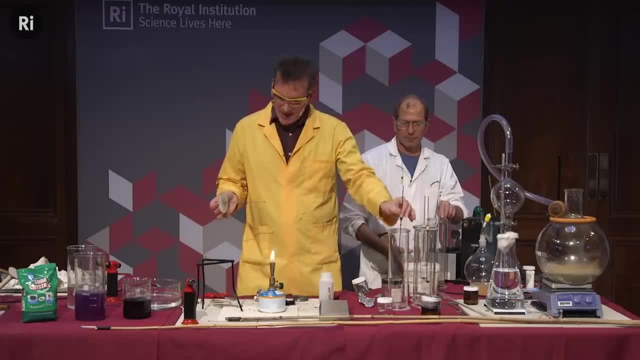 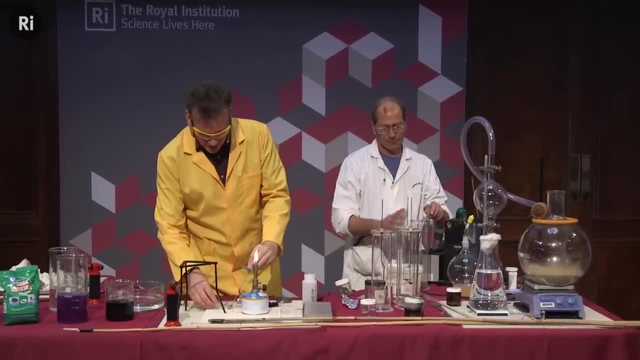 Well, this is called a deflagrating spoon. It's meant to have a spoon on the bottom. This one doesn't, but never mind. Anyway, you'll see why in a moment, So I'm just going to put this, hang this on the bottom here. 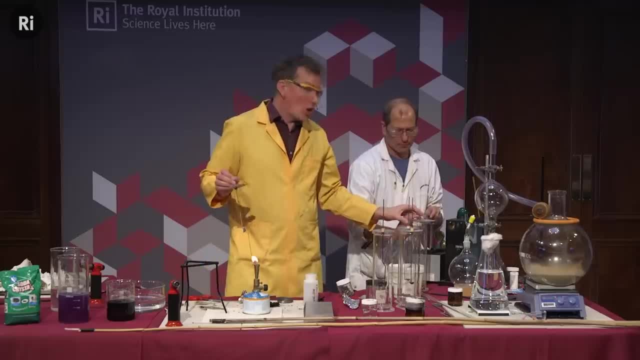 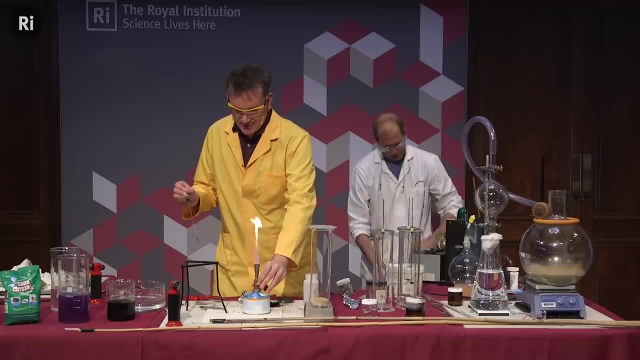 That's my lithium wrapped around the bottom there. So we've got oxygen in the jar And I'm just going to get this burning Now. lithium compounds, when they're introduced into flame, often give a really nice brilliant red color. 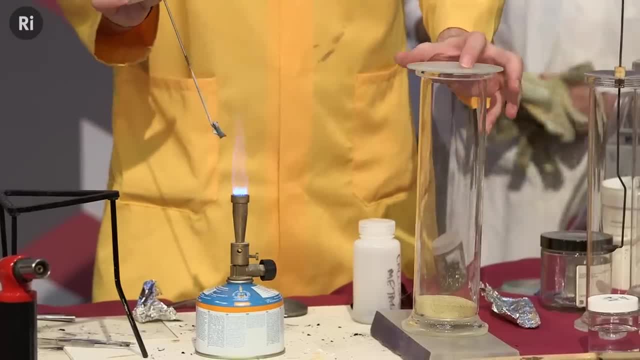 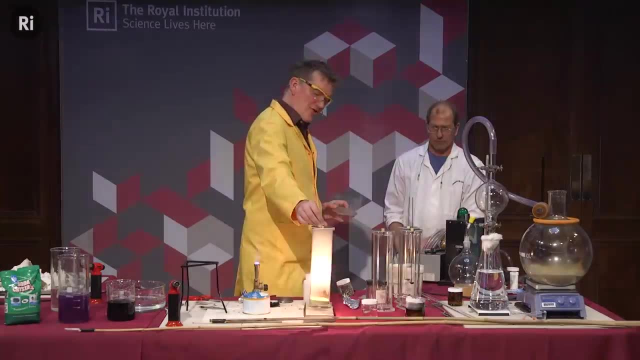 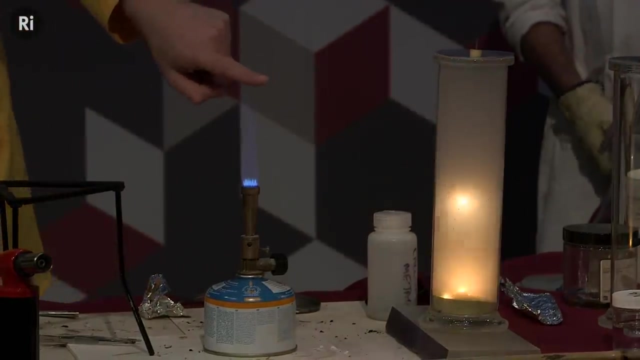 So you may see a little bit of red color, But then hopefully you'll see the chemical reaction taking place, So an incredibly vigorous reaction taking place there. In fact, this one is so vigorous that it's actually now the iron that's burning in the oxygen there. 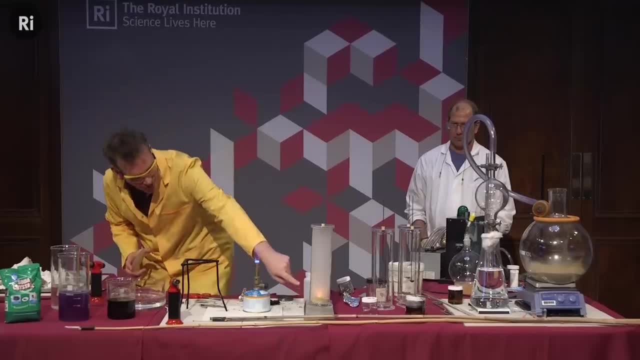 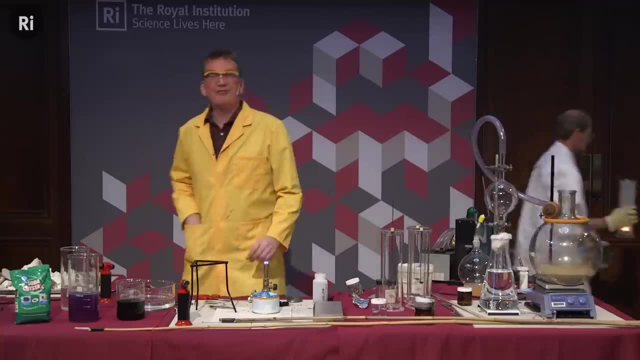 That glowing thing is the iron, And the end of the iron has just fallen off And my rod has got much smaller. I shall give that to Chris, Thank you, But the formula of the oxide that we're making is Li2O. 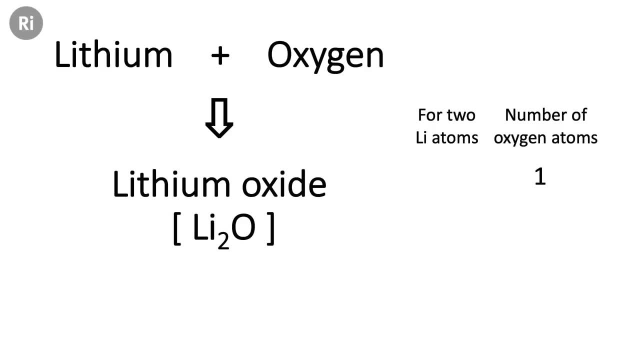 So, like H2O, we have Li2O. So two atoms of lithium with one of the oxygen there. OK, if I dissolve some of that smoke in water. it is also an alkali. It easily dissolves. It's the opposite of an acid. 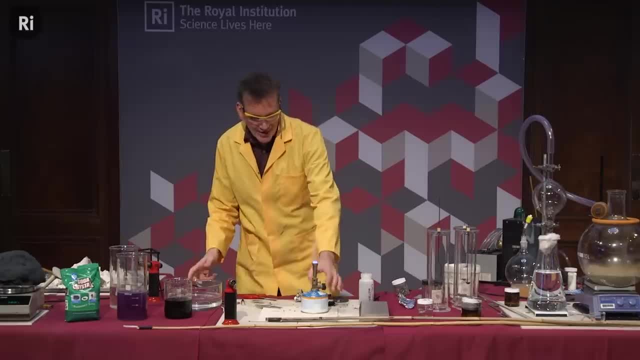 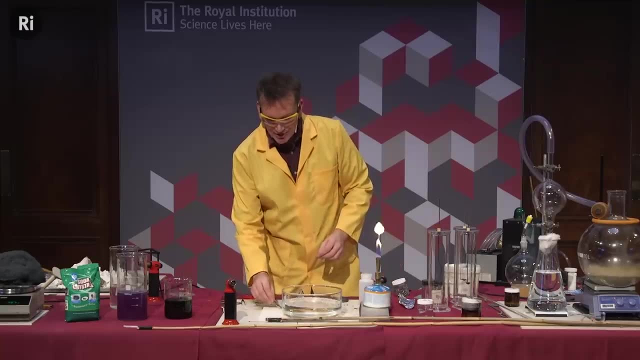 But I can make that same alkali by reacting some of the lithium metal with water, And this is what I shall show you now. So, remember, I snipped off an extra little piece here, So I'm just going to add this to the water. 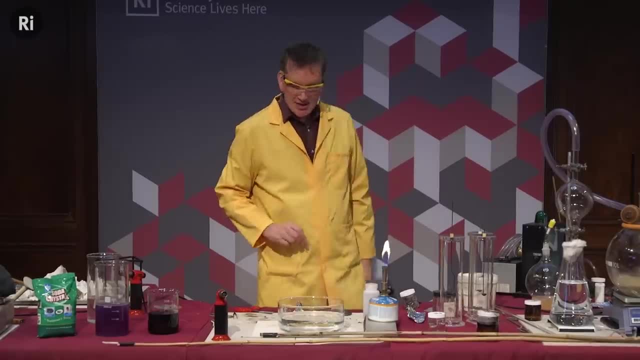 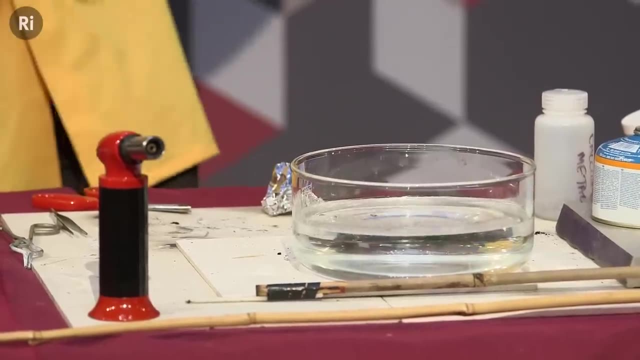 And we can see some interesting things. So let's add this to the water. There it is. Now, remarkably, this floats on the surface of the water, And this is because- well, this is element number three. It's only got three protons, three electrons. 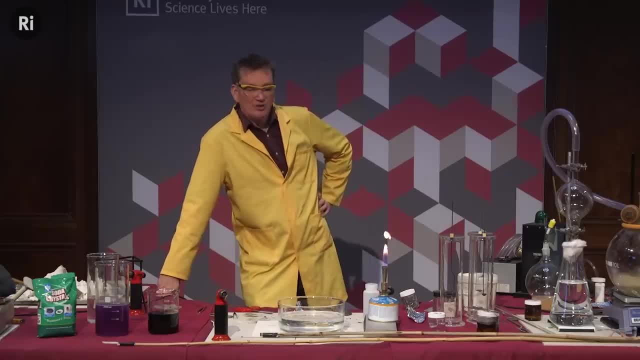 and some neutrons. It's actually light enough, less dense than the water It floats on top, But it doesn't mean to say it would make a good material to make a boat out of, because well, actually it's now. 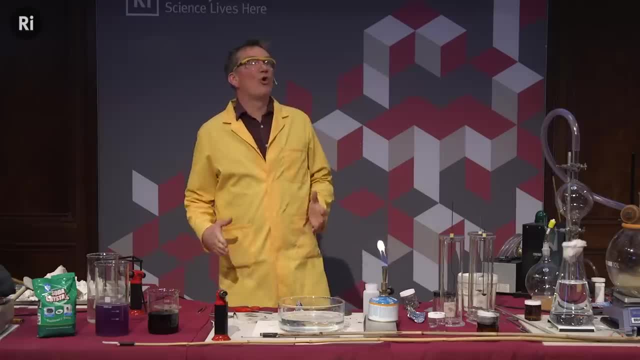 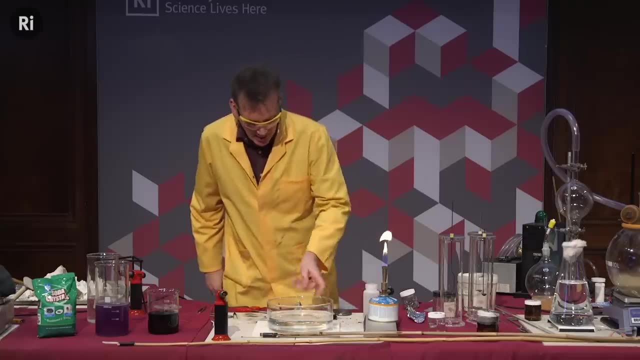 disappeared. It's reacted with the water to form lithium hydroxide. OK, so we formed lithium hydroxide and hydrogen gas- OK, completely disappeared. Well, actually it's not just lithium that does this. Some of the other elements do. 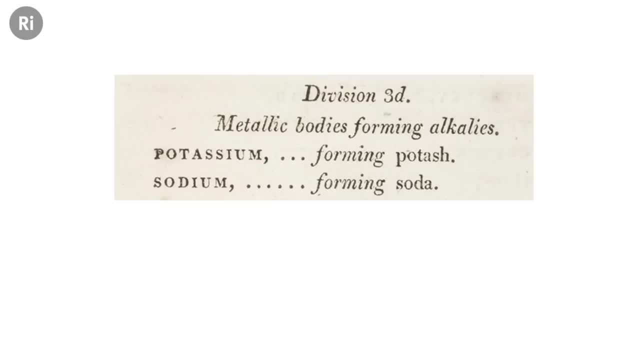 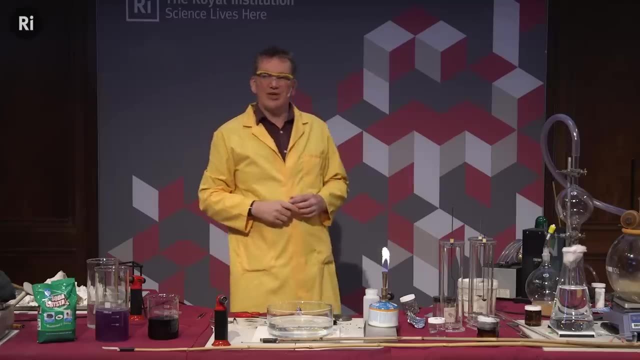 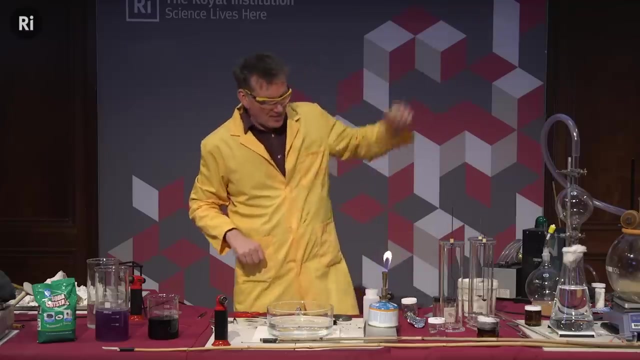 These also react with hydrogen. OK, So we're going to add this to the water to form alkalis, potassium and sodium. Lithium isn't in this list because it hadn't been discovered when Marseille wrote this edition of the book. Let's try the next element underneath lithium. 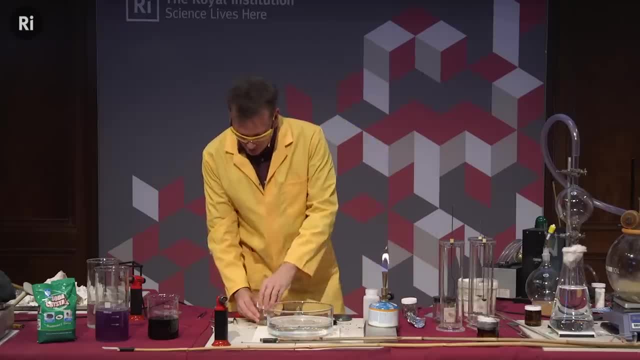 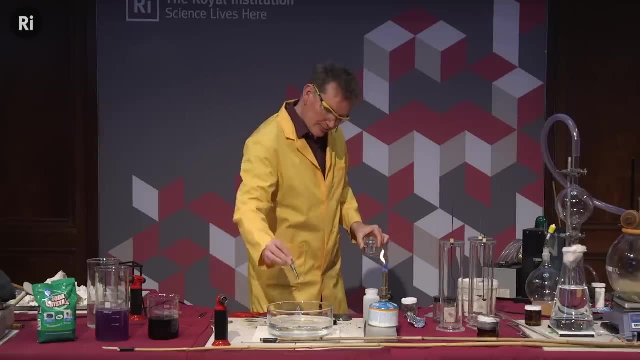 And this is the element, sodium. So we're going to try some sodium with water. So I'm just going to take a tiny little piece here of sodium and add this to the water. I hope There it is, And it's actually fizzing around. 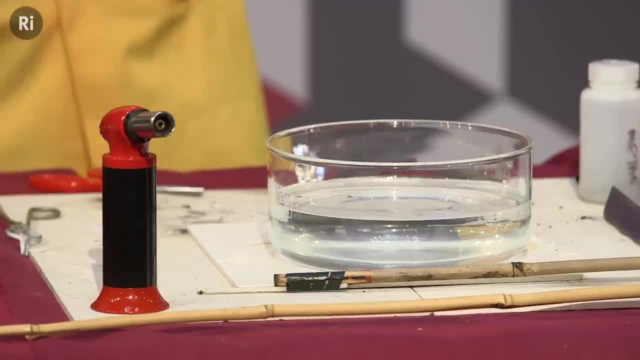 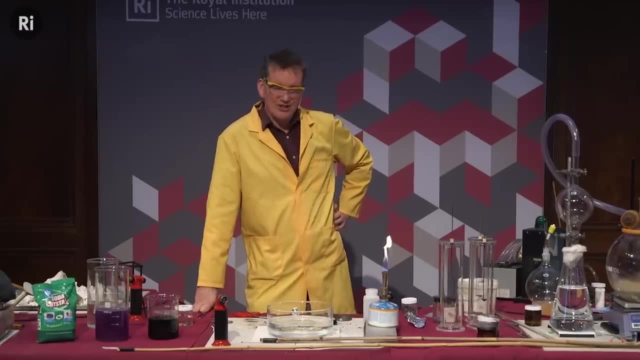 on the surface of the water. Oh, there's a little flash of flame there. This is a remarkable substance. I mean nothing like this had ever been seen before. When Davy first isolated this here, he thought: is this even really a metal? 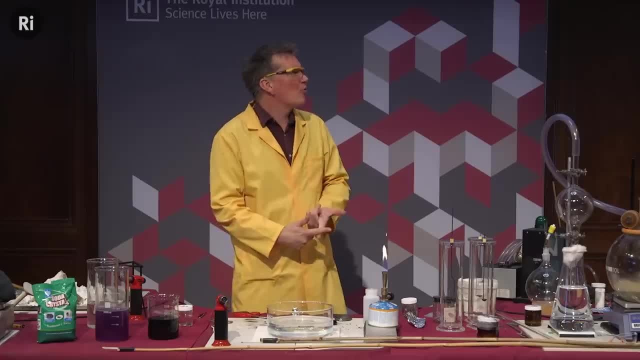 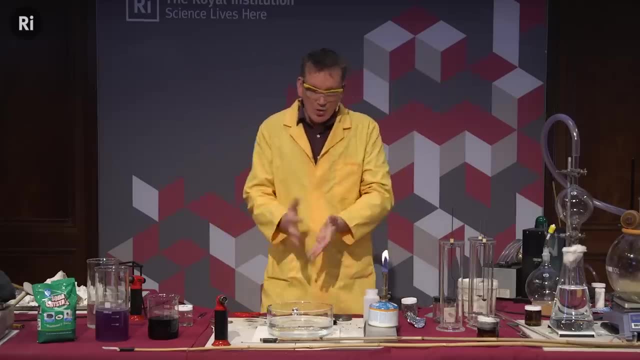 Metals aren't lighter than water. They shouldn't float. They don't react with water like this. This was something that had never been seen before, But all of our group one elements apart from hydrogen, which is a gas, they all react with water in this same way. 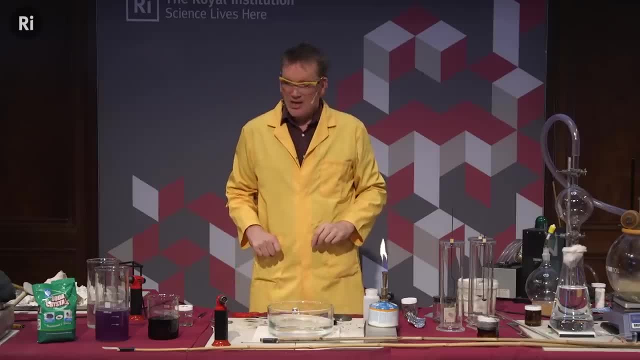 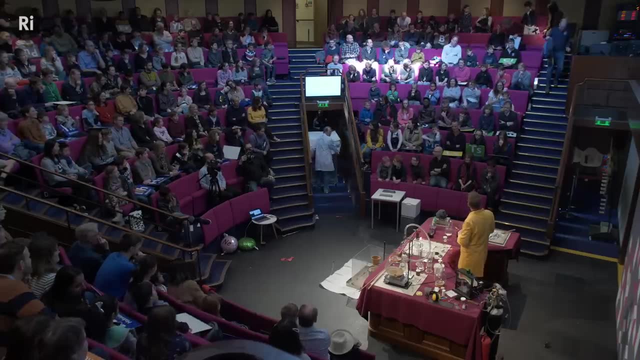 Now, that was a little bit disappointing. You couldn't really see what was going on there. Should we try a larger piece? What do you think? Should we try a larger piece? Yes, OK, Right, OK. so Chris, I think, has a special piece of apparatus. 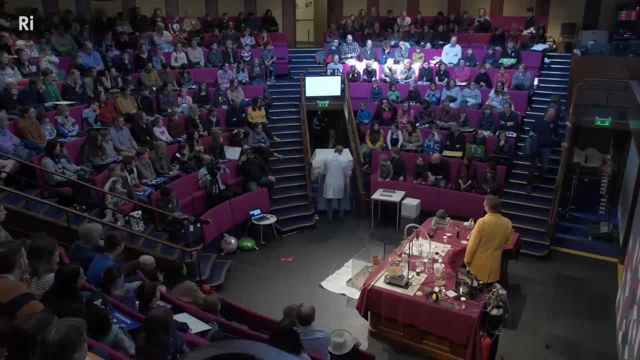 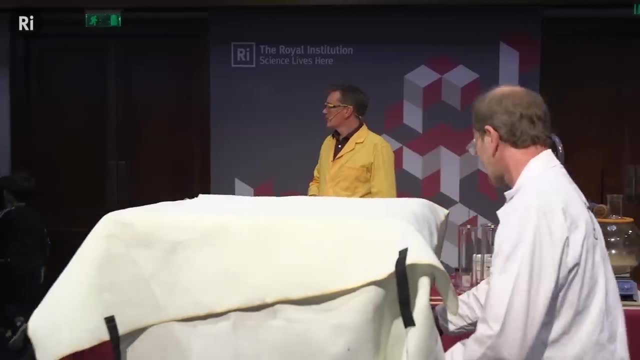 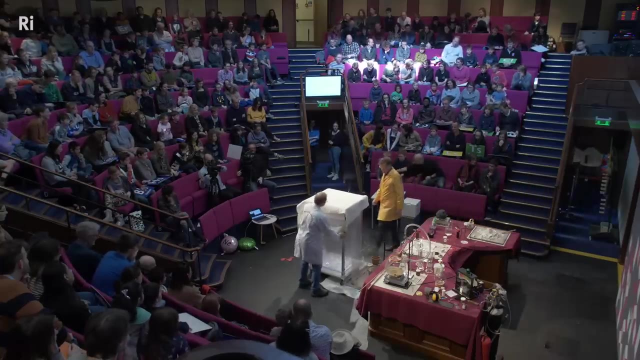 designed to do this reaction safely, OK, OK. so this is a special tank designed to do this reaction, And I can just ask you for this one. if you can just move back just a little bit, This is one that you'll need to do that. 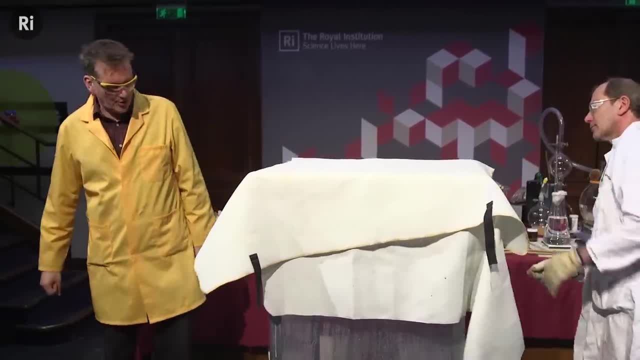 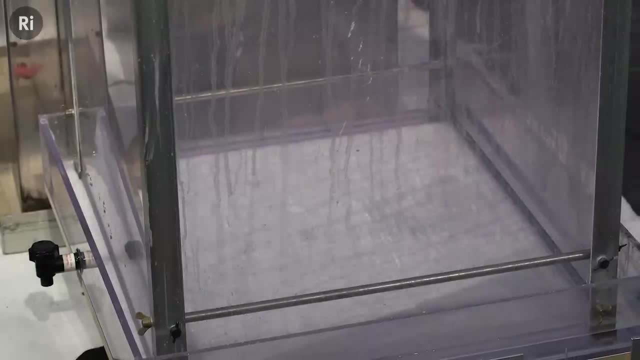 Good, thank you. So this is made of super strong polycarbonate. There's water in the bottom of the tank And there's actually three different lids on top of this, And this is to make sure that this is safe to do the experiment, because we're 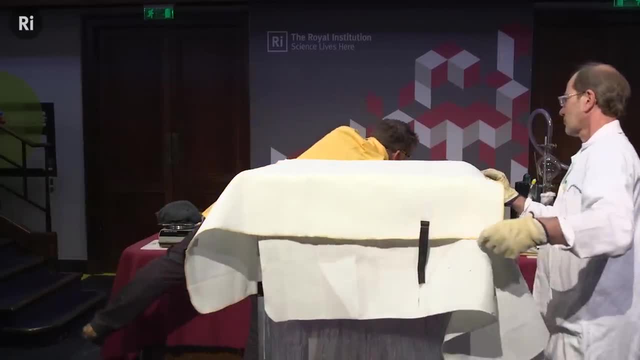 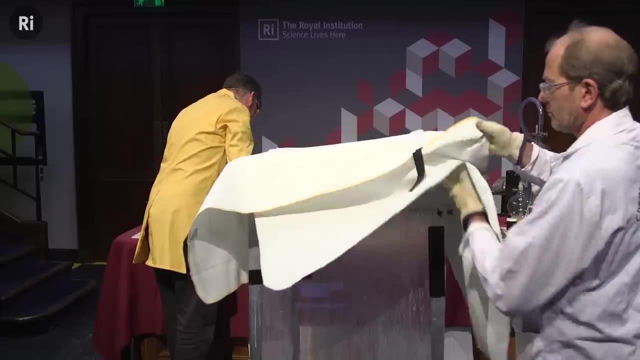 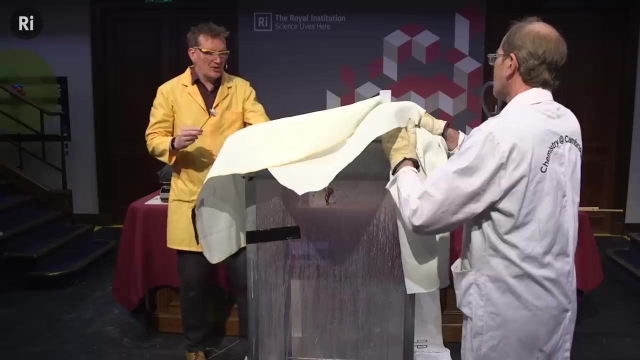 going to use a larger piece of sodium, So I have some larger pieces here. OK, and here is my larger piece. It definitely is larger. Now I need to be slightly careful when I'm adding this because, as I say, there are three different lids. 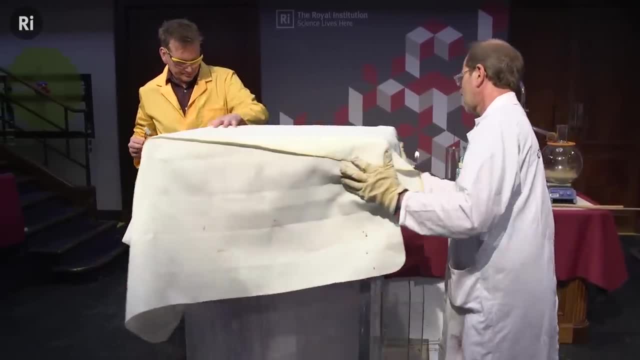 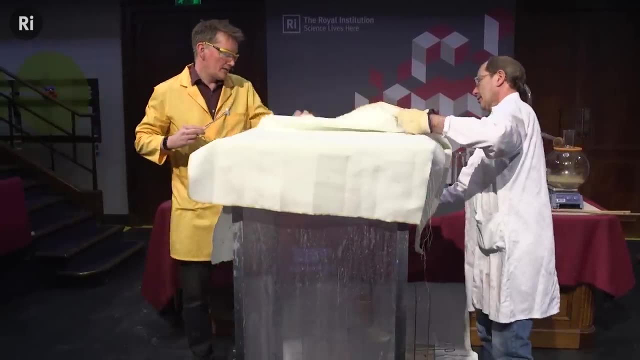 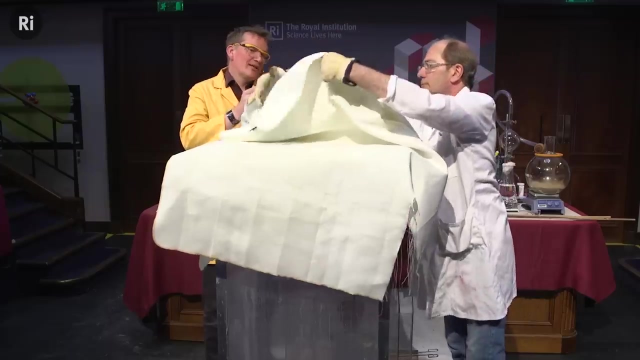 Which way? Is it the right way around? OK, OK, we're coming in this way, are we All right? Always slightly nerve-wracking this one, OK, All right. OK, we're ready with this. So I need to make sure I get this. 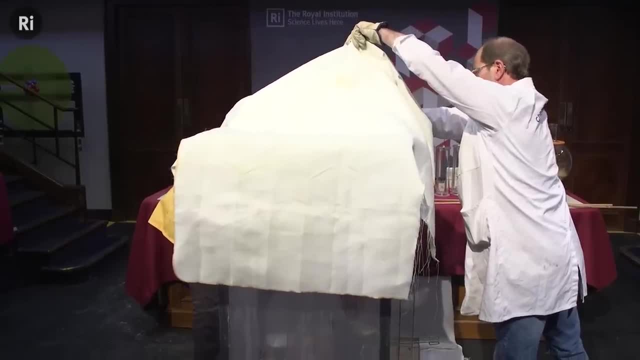 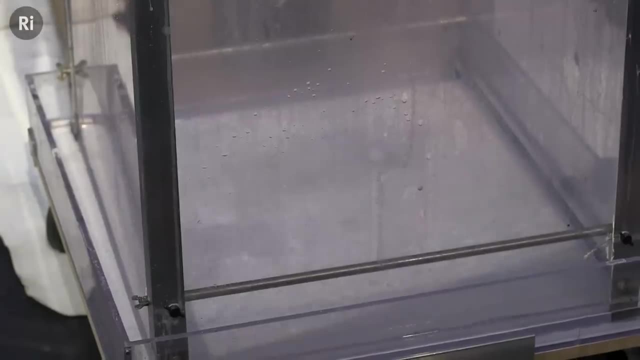 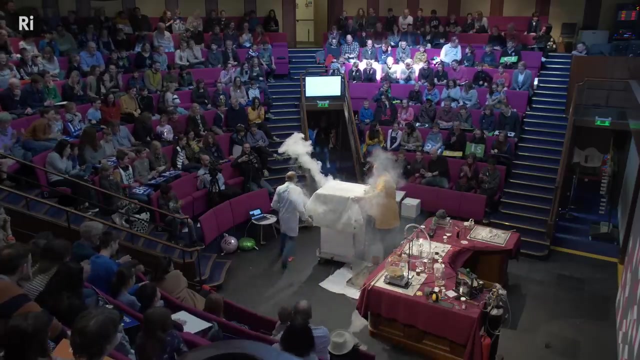 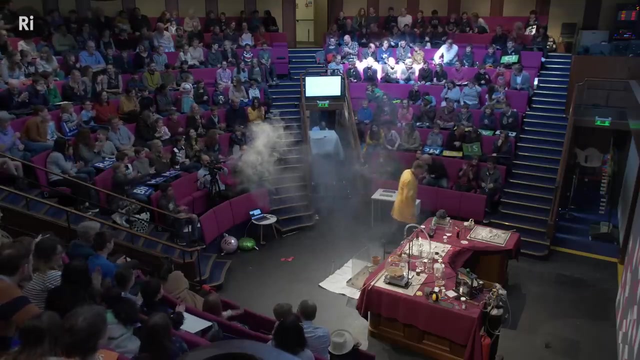 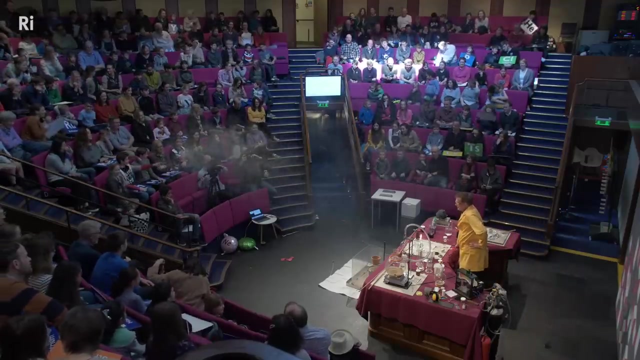 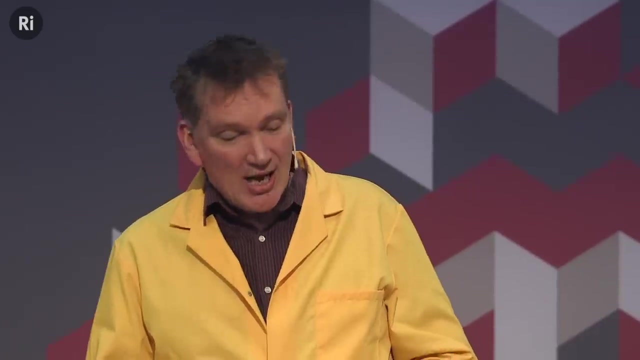 There are, say, three lids and three holes that I need to get this aligned. OK, we're ready. Oh, OK, Chris. Well, OK Now. I particularly like doing that experiment. I think it's a really important one to do because this: 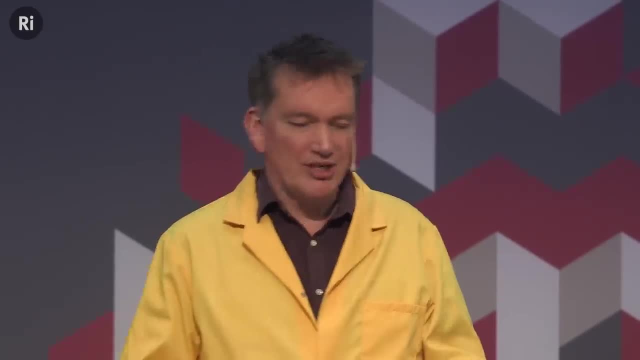 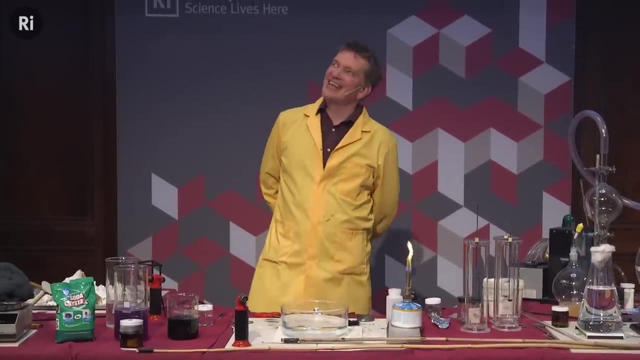 is one of the elements that is often shown at schools. In schools- it's in the GCSE curriculum- The teacher tries the little piece on the water there, as you saw, and you can hardly see anything, And then it's go on. use a bigger bit. 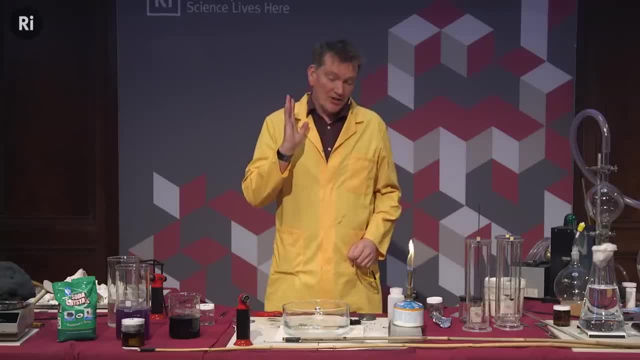 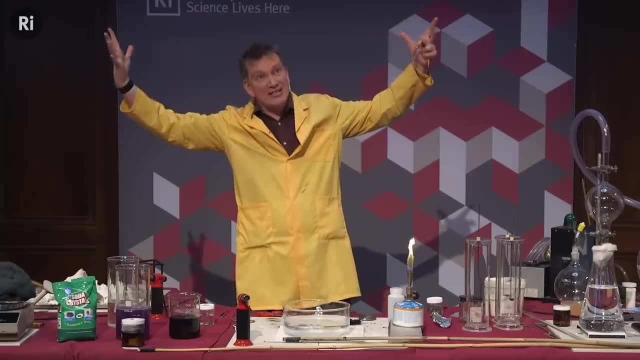 And then they say, OK, I'll use a bigger bit, OK. So I tell you, I have heard so many, so many cases where what's happened there is, the sodium has been on the water and has exploded and then showered burning molten sodium. 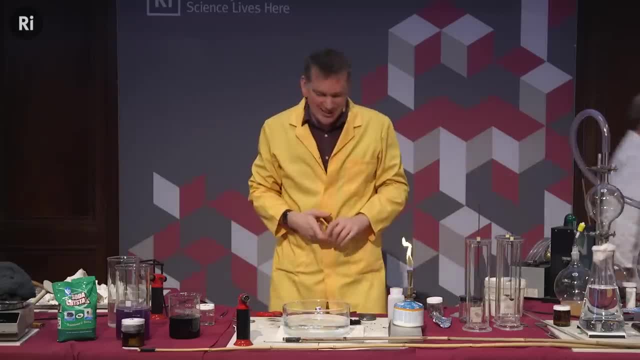 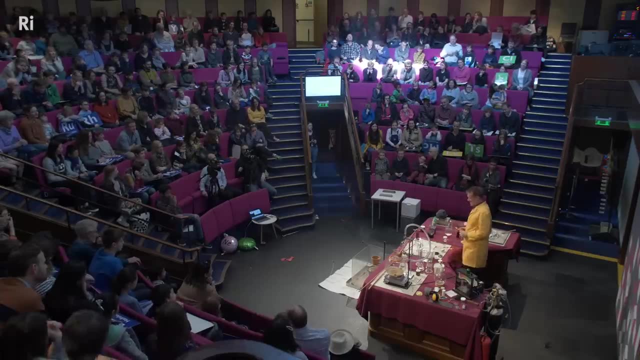 everywhere, which sounds hilarious, unless you're one of the students getting coated in burning molten sodium, And so it really is very important to show this Curiously. in the A-level descriptions you say that lithium just fizzes quietly. sodium fizzes. 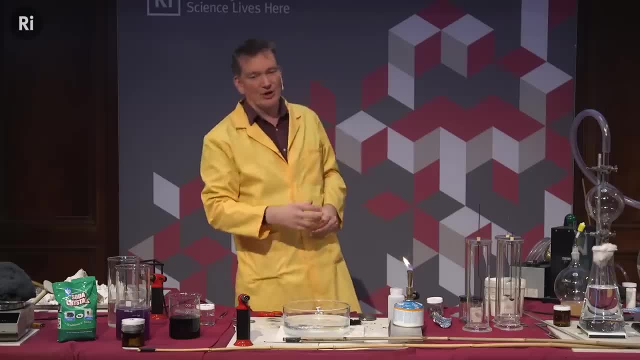 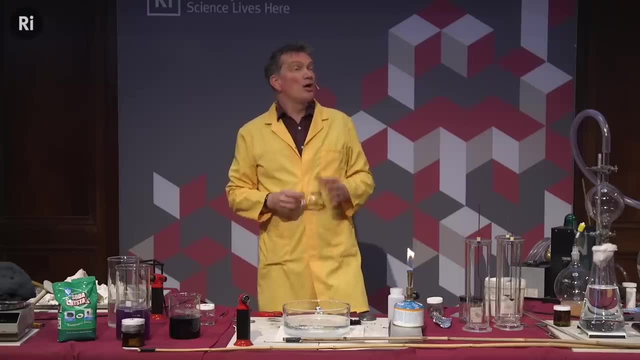 but there's no flame. Potassium goes with the flame. Well, as you saw, it's nonsense. We certainly get a flame there from the sodium But remarkably, even though this reaction has been known ever since Davy's time, this explosion. 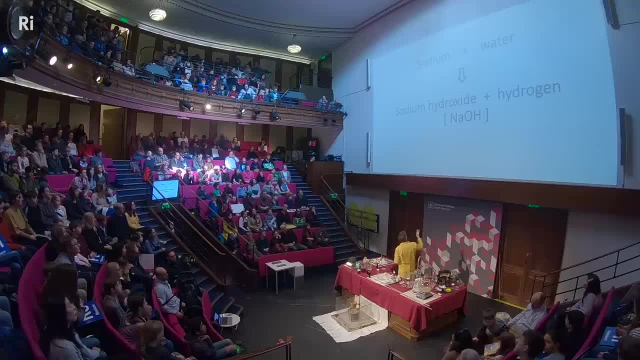 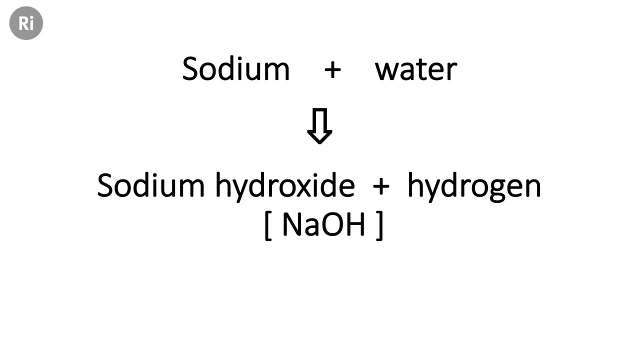 it was thought that it was exploding because of the hydrogen that's given out during this reaction, But actually it isn't, And the reason for this is only recently, within the last few years, been discovered. What's happening during the chemical reaction is: 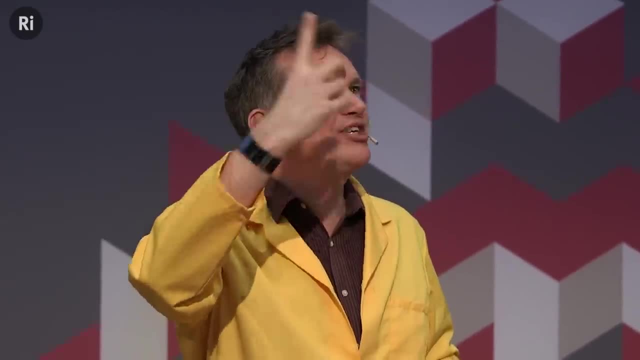 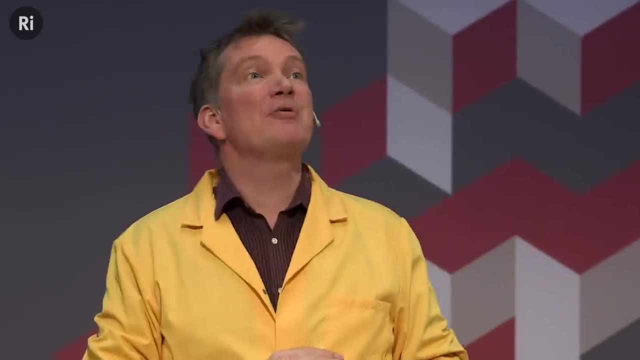 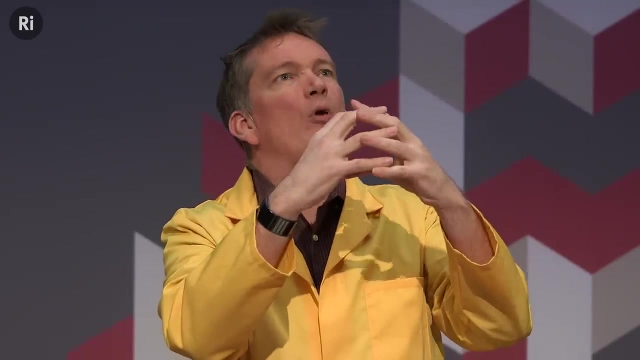 the sodium. remember the outermost one, electron, that was whizzing around with all of our group, one That electron is easily lost. And if an atom loses its electron it becomes positively charged. And what happens here? The charge on our molten sodium is becoming more and more. positive, is becoming more and more and more and more positive, And of course we know that, like, charges repel each other. And so what happens when the charge builds up too much? It pings apart. It's called a coulombic explosion or a charge. 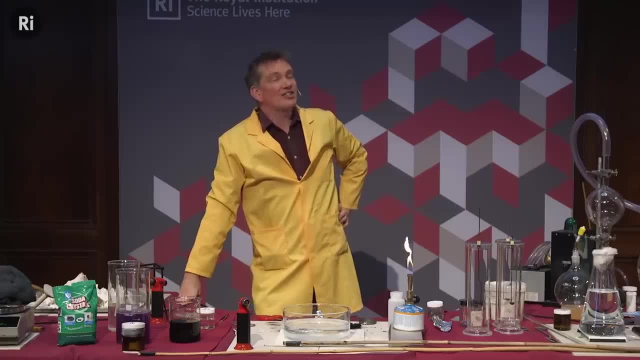 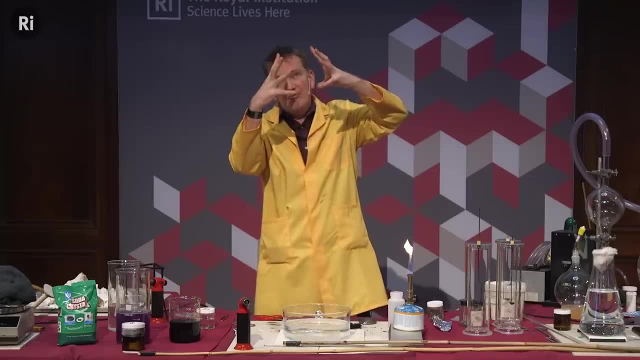 explosion. That's the reason that we get the bang there. This has only recently been studied, So with high speed photography you can see the sodium literally forcing itself apart, And this has been modeled using theoretical computers. theoretical modeling to show that this. 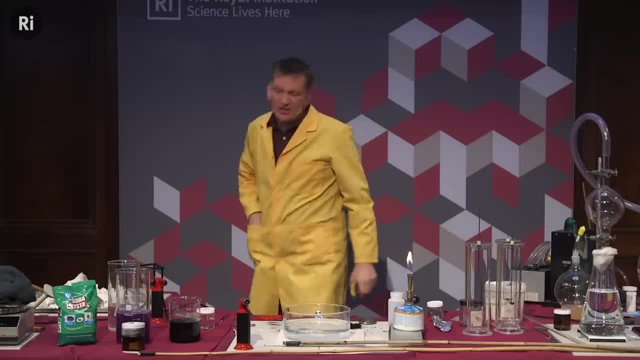 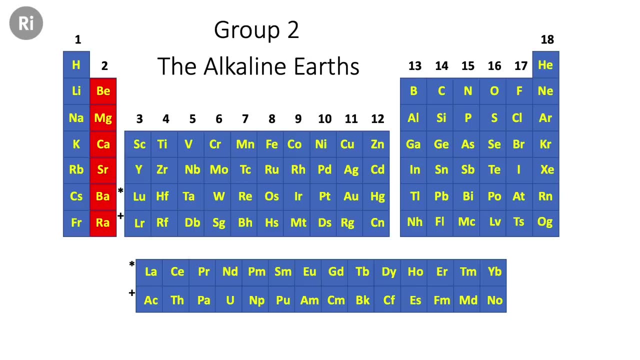 is what's happened there, But this is all relatively new. OK, so well, let's go to our group. two element. So these ones, remember, all have two electrons And they're in their outermost shell. I'm not going to show you any beryllium. 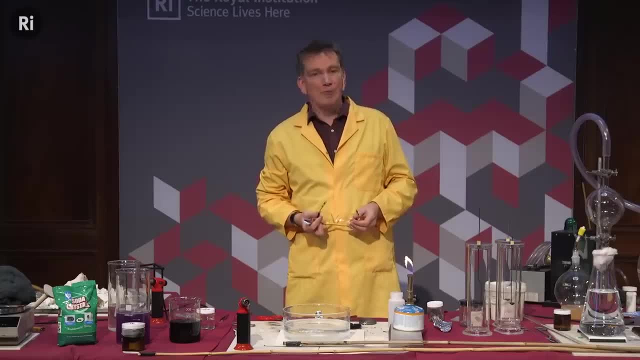 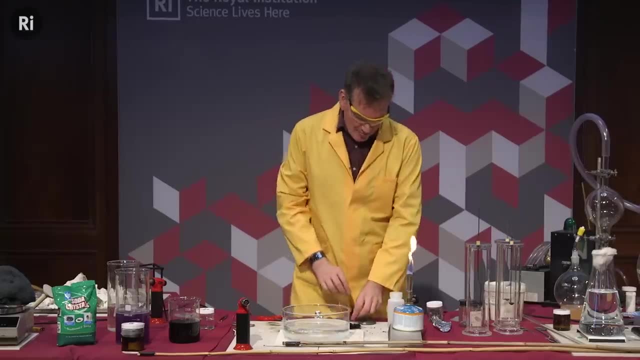 at the top of the chart here, because the compounds of beryllium are all very toxic, So I can't show you any beryllium, But I can show you some of the other ones. In fact, we're going to look at the element magnesium. 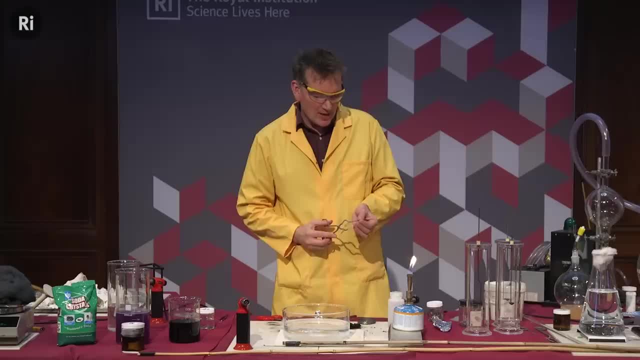 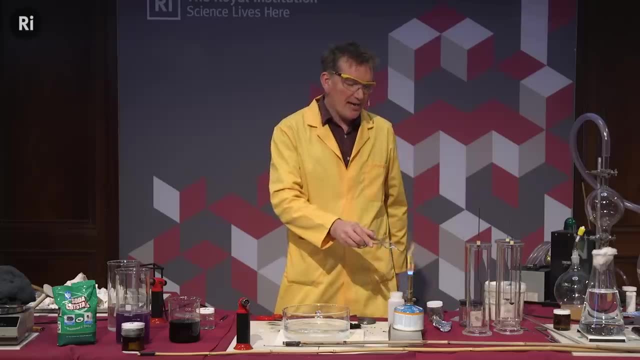 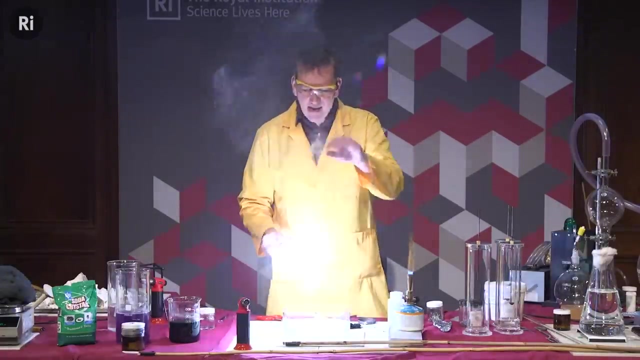 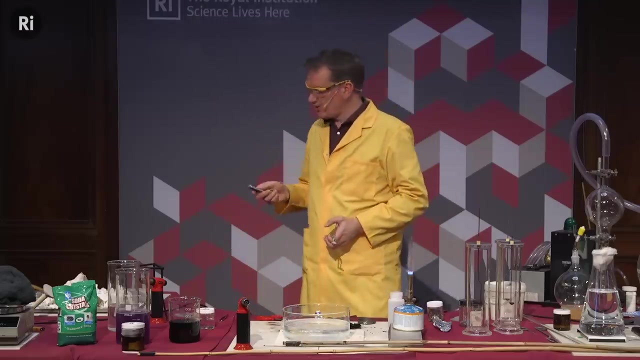 And I have a little piece of magnesium here And this reacts with the oxygen from the air, Got a fantastic brilliant white light. The white smoke here is magnesium oxide. OK, but the formula for the magnesium oxide that we're making there is well, now it's. 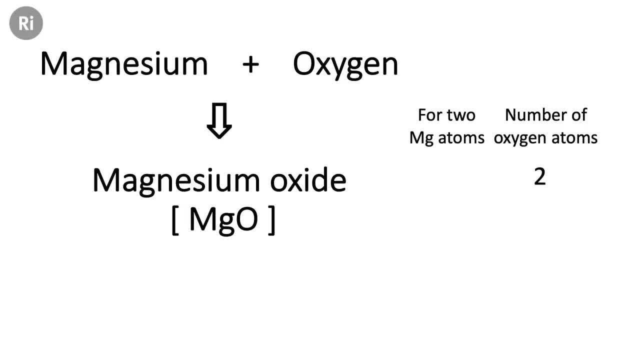 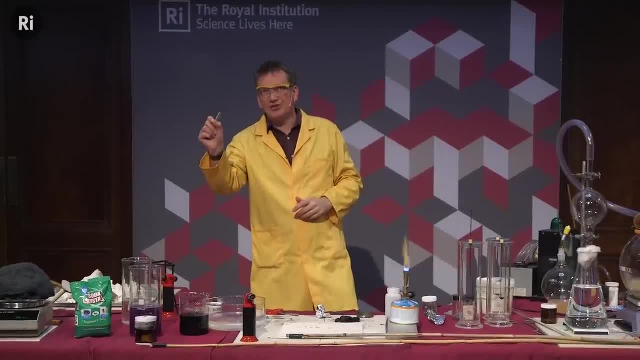 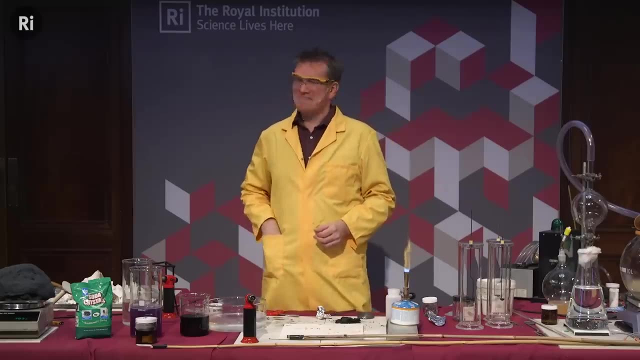 one magnesium to one oxygen, Or using Mendeleev's system, there two atoms of the element, so two magnesium combined with two oxygens, And magnesium is in group two. OK, so should we try a bigger piece of magnesium? Yeah, exactly. 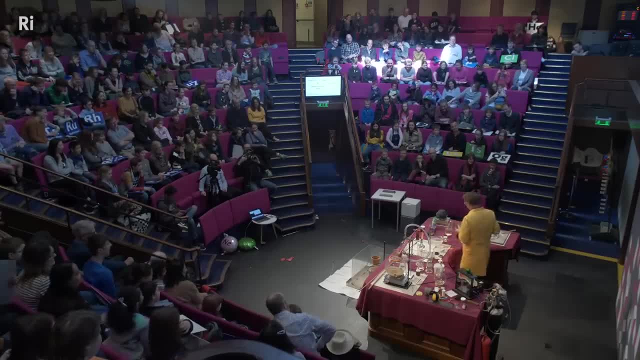 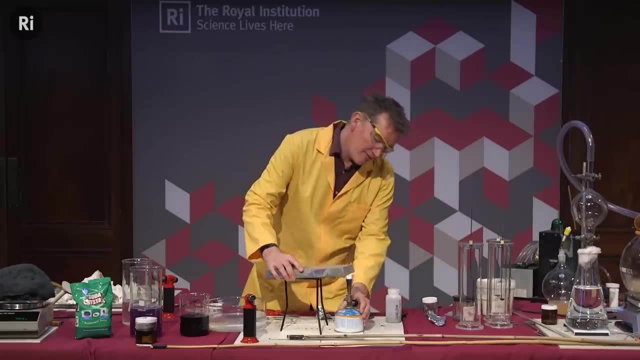 OK, I have a nice big piece of magnesium. This is magnesium. It's really very, very light, So this is pure magnesium. So I'll just put this in the flame. OK, I'll heat it up on the end there. 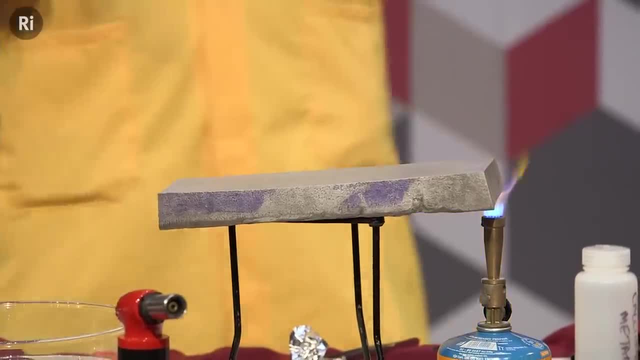 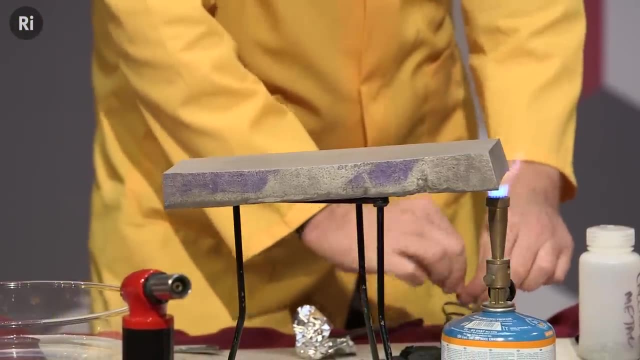 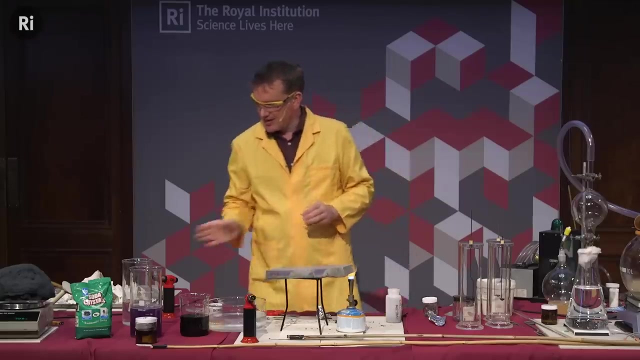 So while we're waiting for that one to get going- well, we saw the lithium and the sodium react very violently with water. What about our magnesium? So, if I take a little piece of the magnesium, this is the magnesium ribbon. so here is the magnesium. 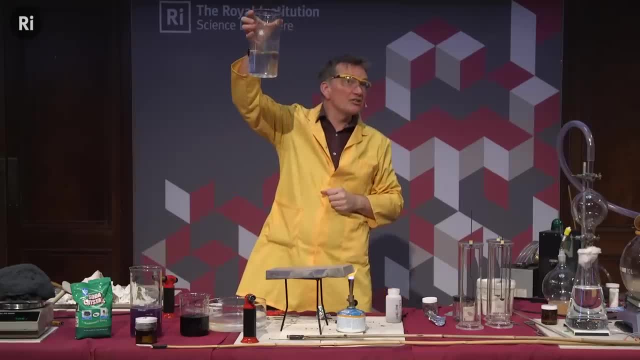 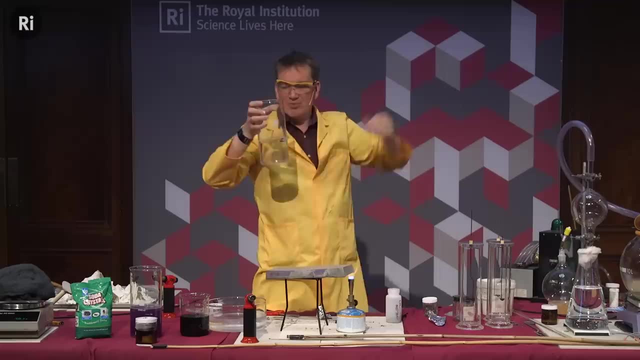 If I add this to some water, well, it sinks. In fact, it's only our group one metals, only the lightest of those, So it's lithium, sodium, potassium. These are the only metals that are less dense than water. 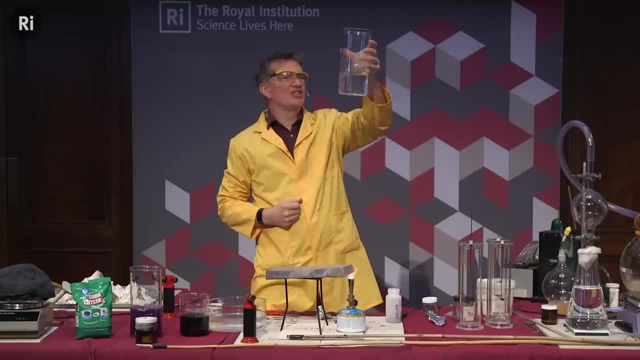 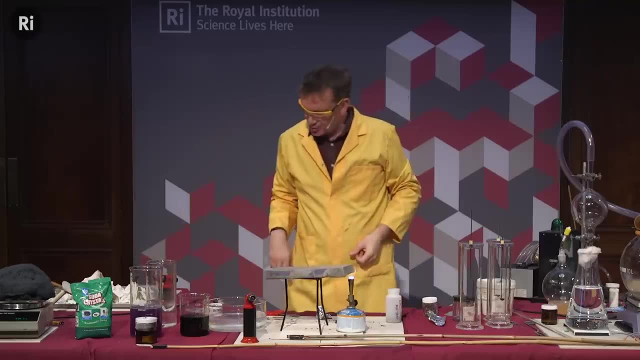 So even all the ones from group two sink. But actually even this is not reacting very quickly. It is very, very, very, very, very slowly reacting. If I heat it up the water to a high temperature, it would react. 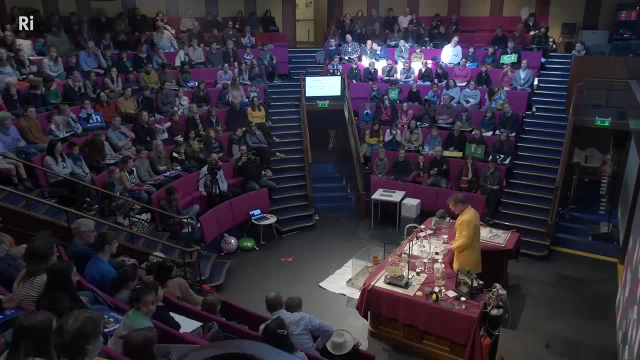 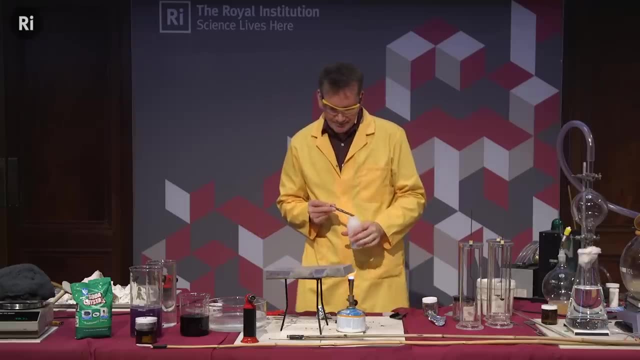 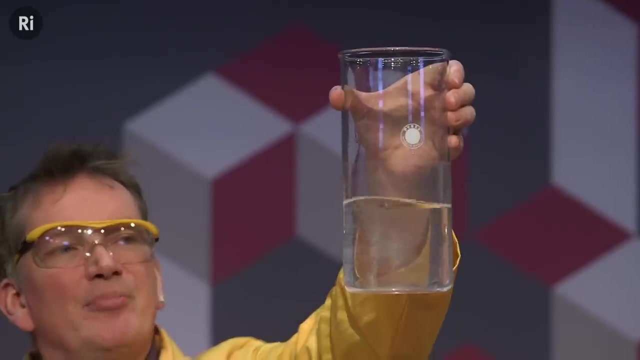 But if I pick the element underneath magnesium, well, this is calcium. this one does react a little bit more vigorously. So if I take a little piece of calcium, so here is some calcium. Adding this to the water, again the calcium sinks. 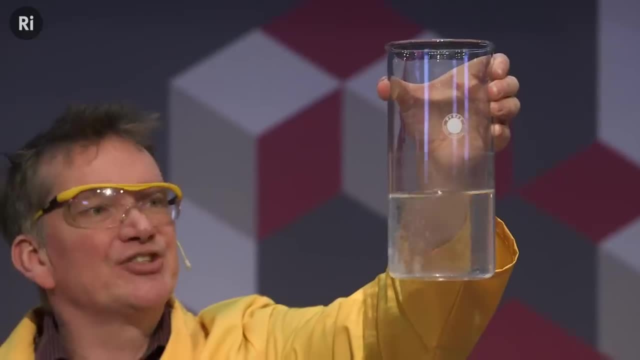 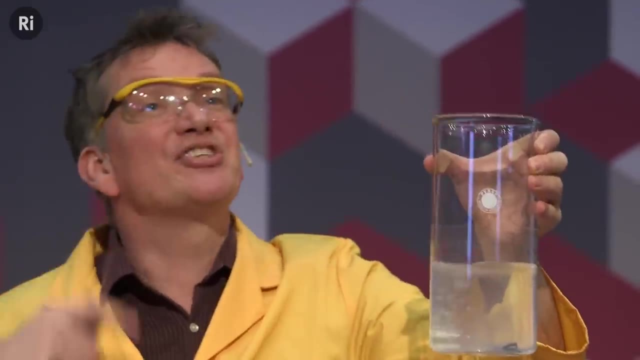 But instantly we're getting bubbles of hydrogen gas given out. here The chemical reaction is: the calcium reacts with the water to form calcium hydroxide. Well, that's the same, That's the same substance that we made here. the reaction with our calcium oxide with water. 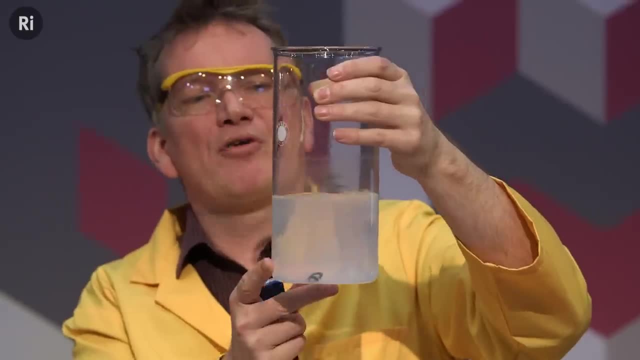 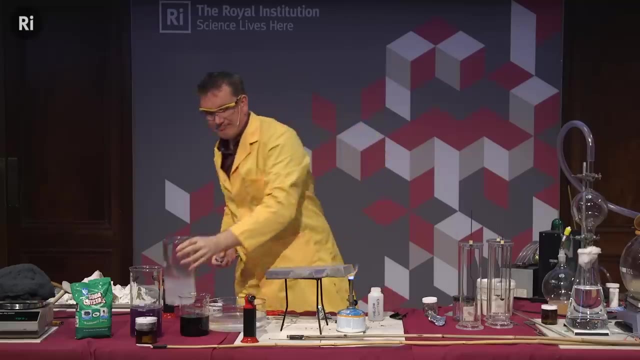 So we're making calcium hydroxide. That's what's making the water go very cloudy here at the moment, because it doesn't really dissolve very well. But we're also getting hydrogen gas there given out, OK. Well, what about my magnesium? 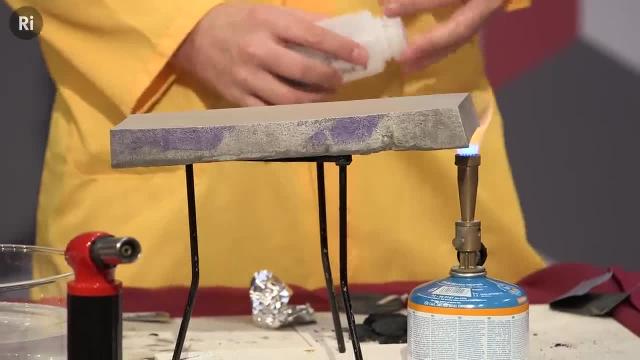 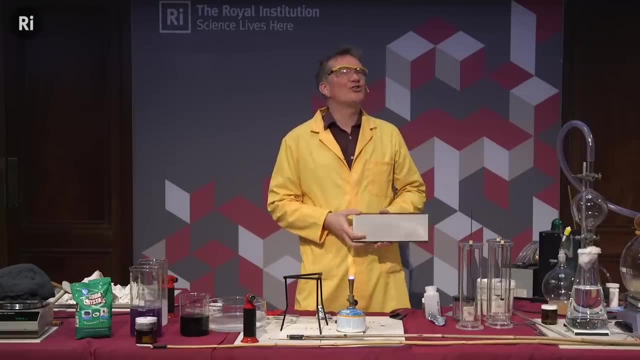 It doesn't seem to be reacting, And actually that's probably a good thing. It would be a bad day if this caught fire, But it's because It's too big. OK, It's too big to react. This is because, at the moment, it's. 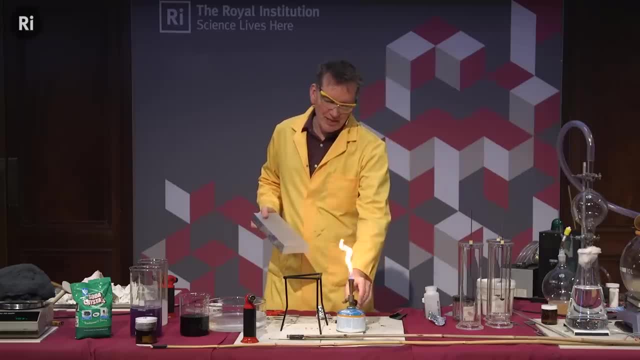 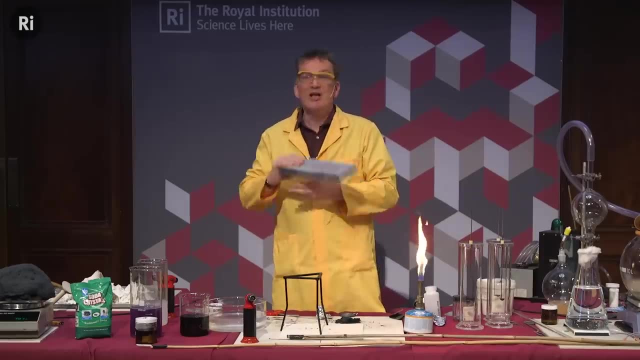 taking all of the heat from this Bunsen, as I was heating it there, And the heat is being spread out And it's being slowly absorbed into the block here and dissipated from the block as well. So it's actually I can still pick this up. 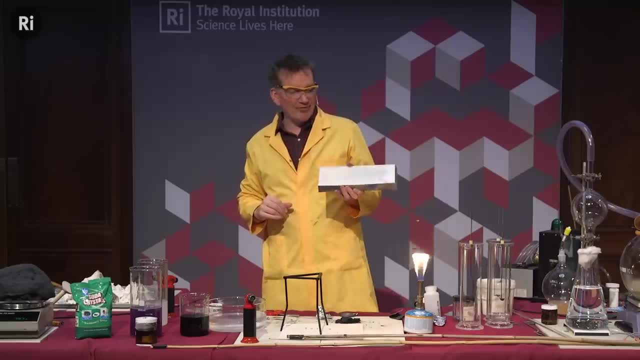 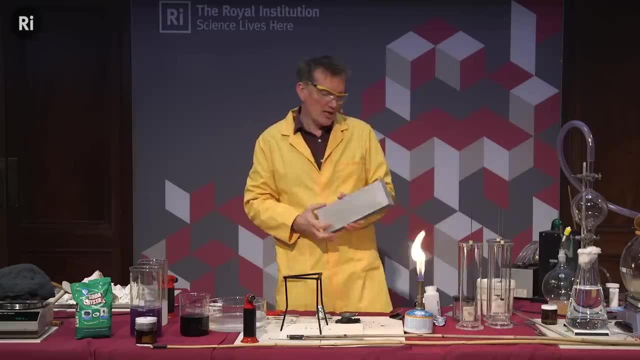 It's not hot enough yet. It can't get hot enough for the reaction to actually start. for this to combine with oxygen, OK, It's just too big, OK, And so, yeah, What we need actually is the very thin magnesium ribbon. 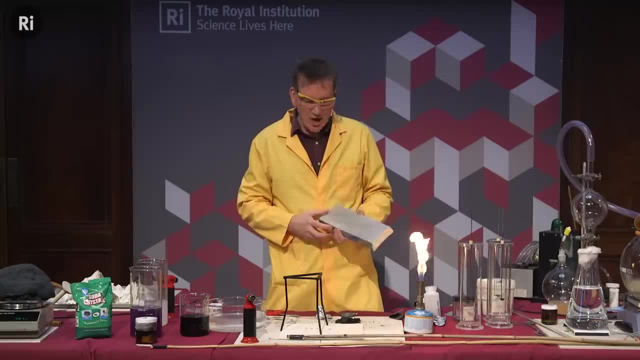 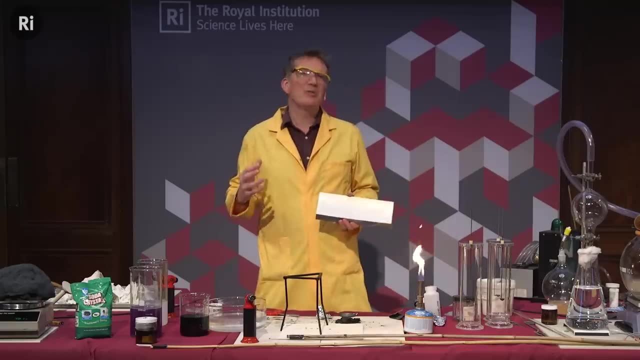 to get a nice quick reaction here, So this was just too large there to react. In fact, this was chopped off from an even larger piece, an ingot of magnesium that was made by pouring molten magnesium into a mold, And this would actually melt before it. 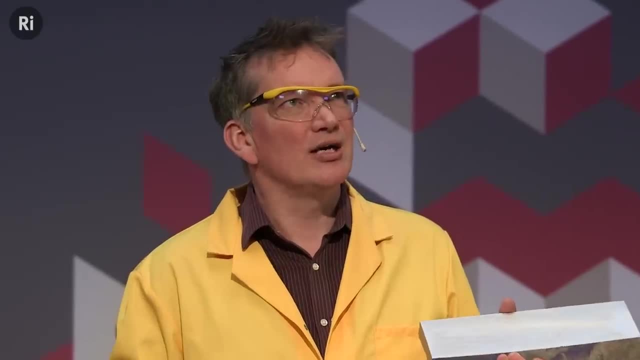 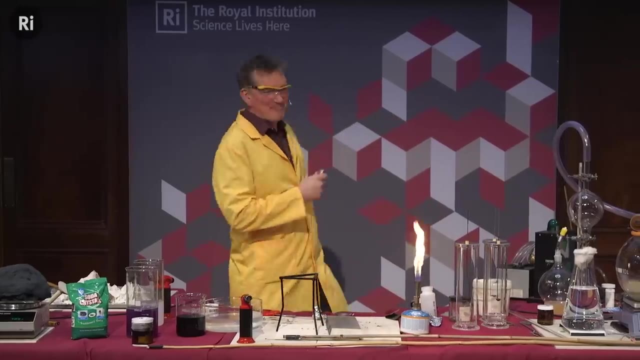 reacts with the oxygen from the air and bursts into flames there, OK. So yes, it's perfectly safe to heat that one up, Phew, But I still feel relieved nonetheless. Anyway, Now let's go back to Mendeleev's table for a moment. 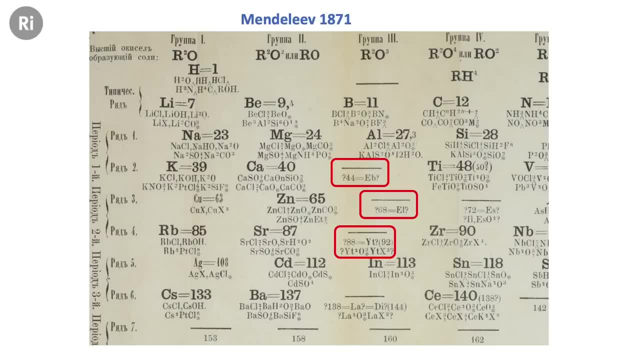 And we'll see. one of the real genius things of Mendeleev was- and this is probably why we're celebrating the anniversary of his table and not the true first table- This is because of some of these gaps that he has in his table, these horizontal lines. 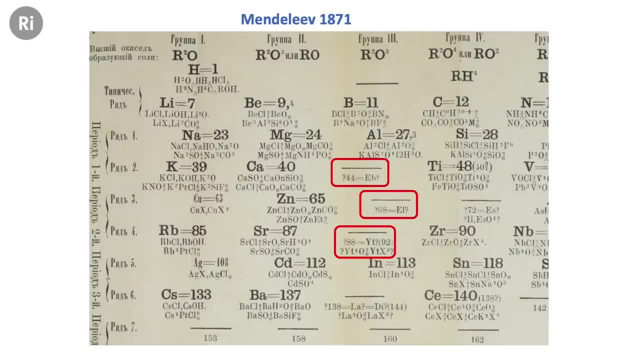 Well, some of them so. for instance, the line that we see here: this is where he thought maybe the element yttrium ought to go here, So underneath he's put YT question mark. Well, YT isn't the symbol that we now use. 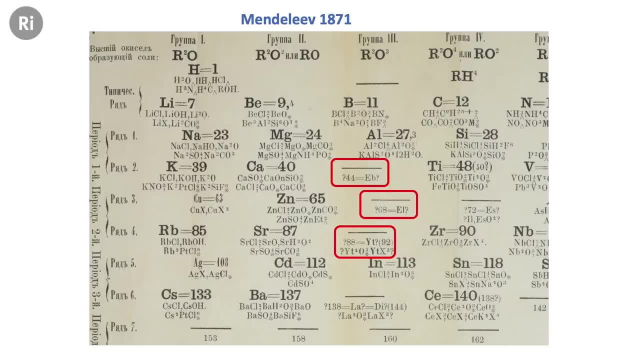 It's just Y. But he was quite right. Yttrium ought to go in that space there. OK, So that one was a known element, But some of them- so these two were actually elements that were not known at the time. 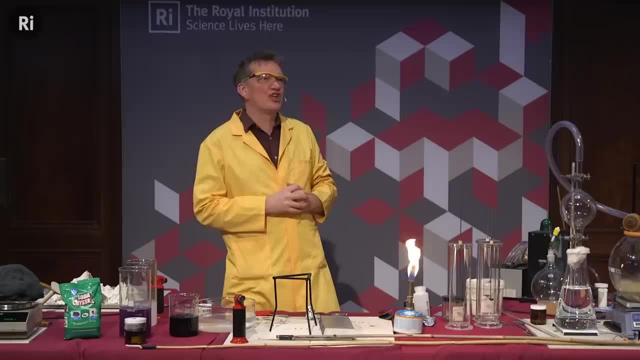 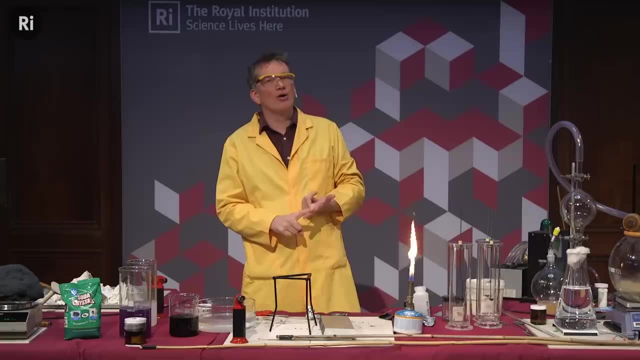 And so Mendeleev said: well, he thinks there should be some elements here, And he even predicted the properties of these elements and the compounds of these elements. And he was spot on And this is what got him recognized And this is probably why his system- everyone paid attention. 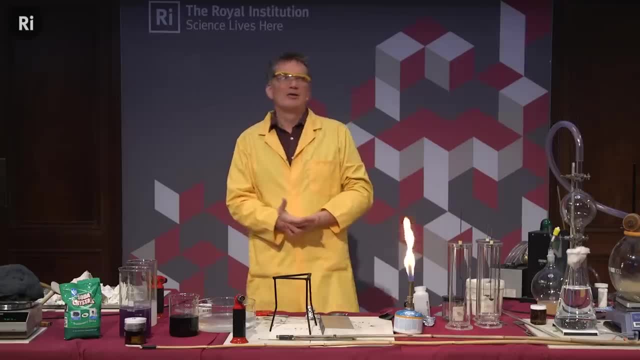 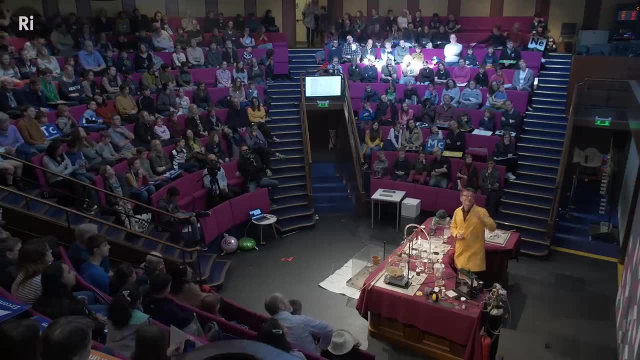 to this. They thought: well, if he can predict these properties so well, there must be something in his system, And so this is why we're celebrating his system today. So let's have a look at one of these. So we have the symbol EB. 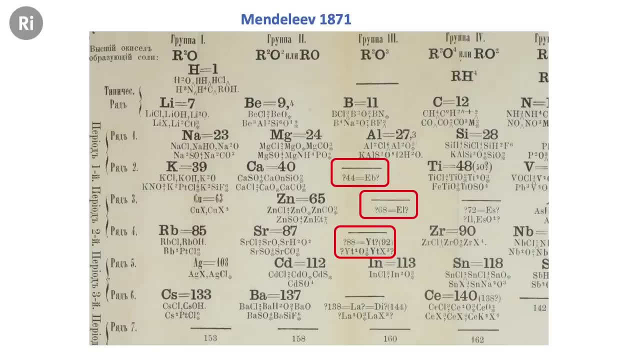 And this is well sort of underneath B. We have B, then AL and then EB, EL. So EB- this stands for ecoboron. Eco was the Sanskrit meaning one. It's one space below the boron there. 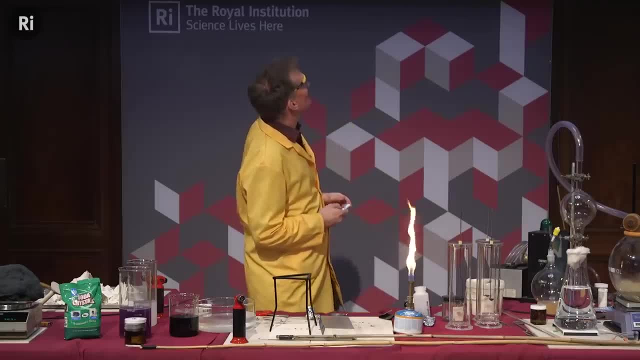 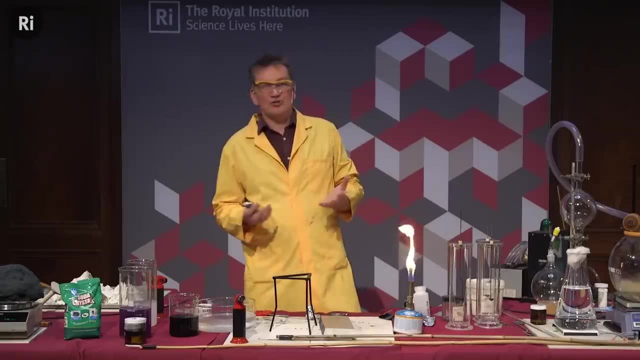 if we ignore the aluminum, And the EL is one space underneath the aluminum. So this element, EB, was discovered shortly afterwards And it was named by the discoverer of the element. scandium. Mendeleev predicted its atomic weight to be 44.. 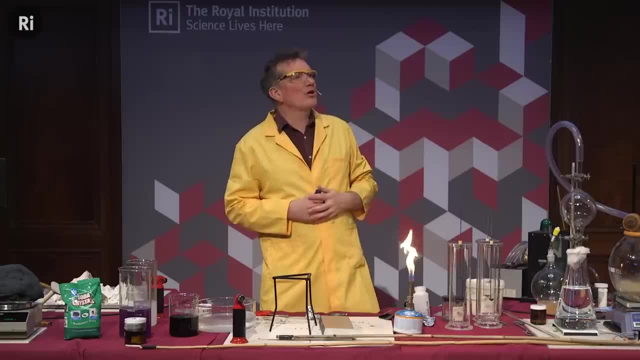 It turns out to be 45.. But importantly, he predicted the formula of the oxide of this and how it behaves. So he said the formula should be well, two atoms of the element with three atoms of oxygen. And when scandium oxide was discovered, it was found out. 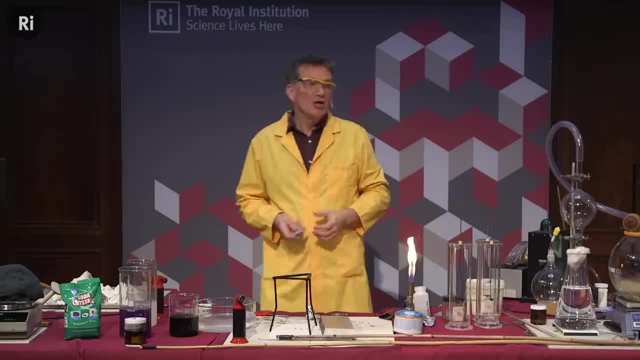 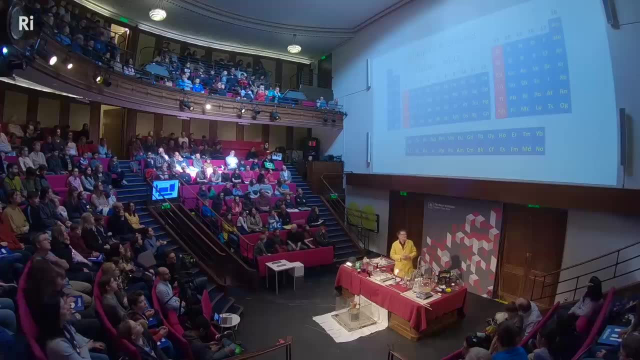 to be. well, two atoms of scandium with three of oxygen there. So all of Mendeleev's predictions were spot on, OK. well, so where is scandium In Mendeleev's system? there, he actually mixed up some of the elements from group three. 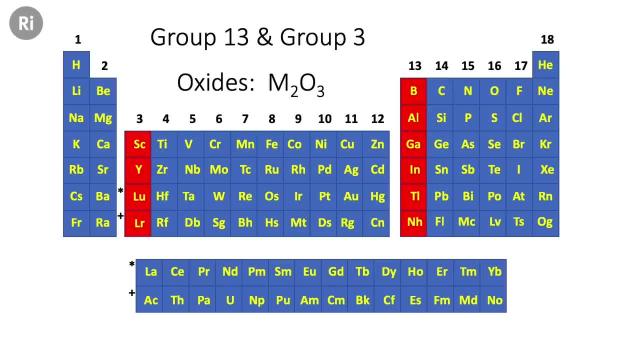 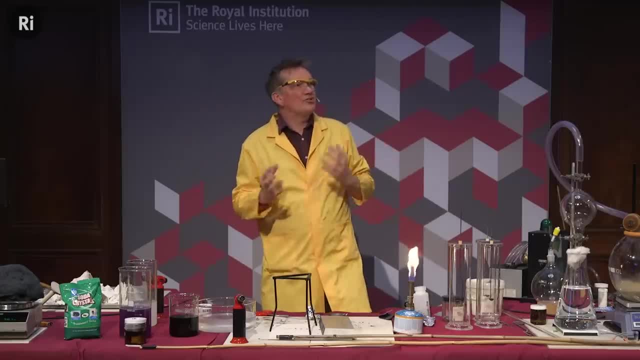 and with those from group 13.. This is because, well, both of these groups have three electrons in their outermost shell that are available to form bonds with, And so this is why they're sometimes, in his system at least, grouped together. 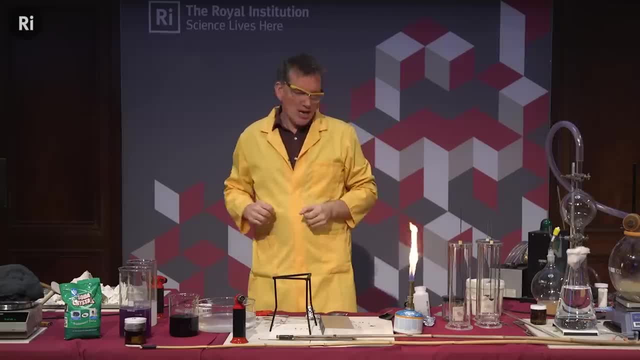 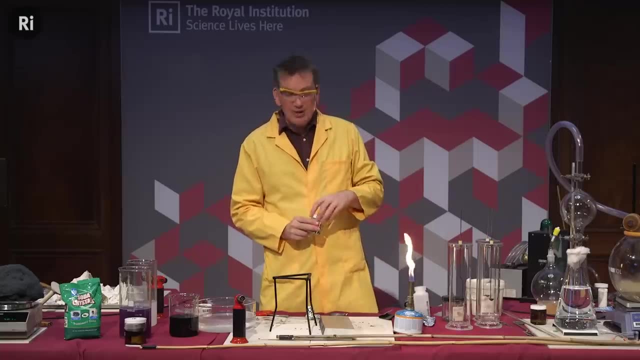 OK, But they ought to be- It's modern form- separated, like this. OK, well, let's have a look at some scandium. So I have a little bit of scandium here. It's very expensive because actually it is very rare. 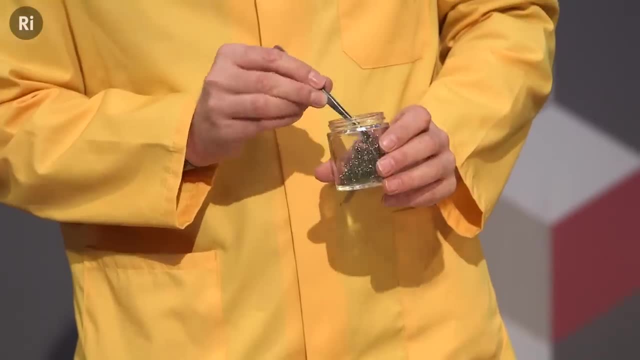 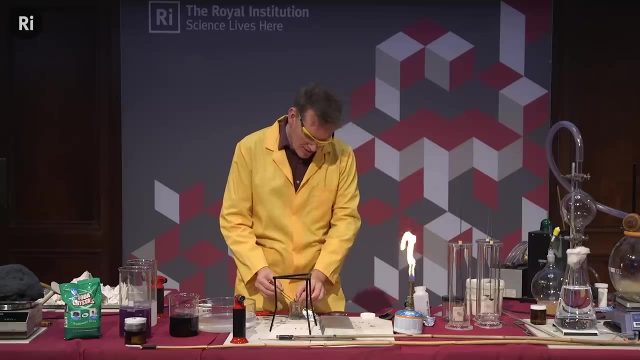 This is why Mendeleev didn't know about it, because it hadn't been discovered, because it is quite rare, So it's quite expensive. But I thought I should get some to show you, because I'm sure you want to see how it burns. 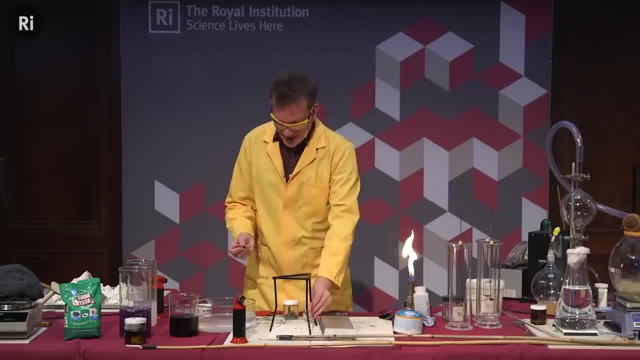 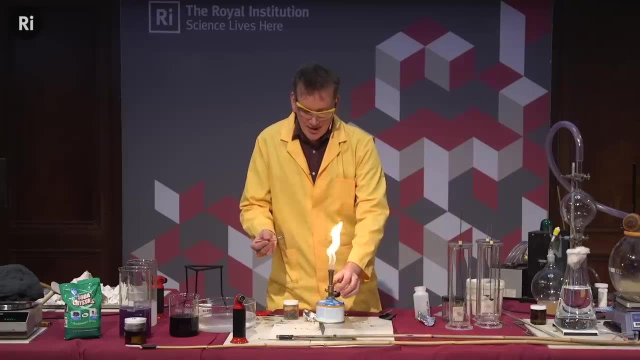 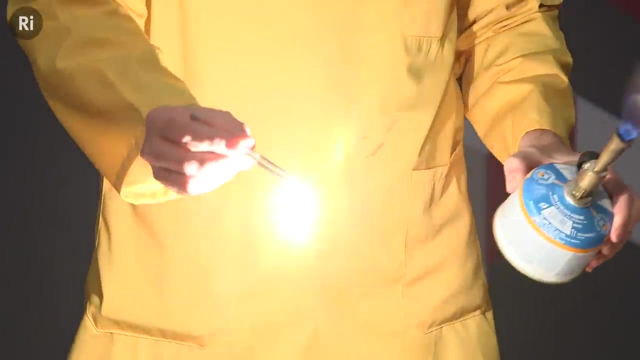 Who wouldn't? Yes, I had never seen scandium burning before, So let's give this a try. Let's give this a go. So I have some very finely divided scandium here, And if I heat it up it should burn. 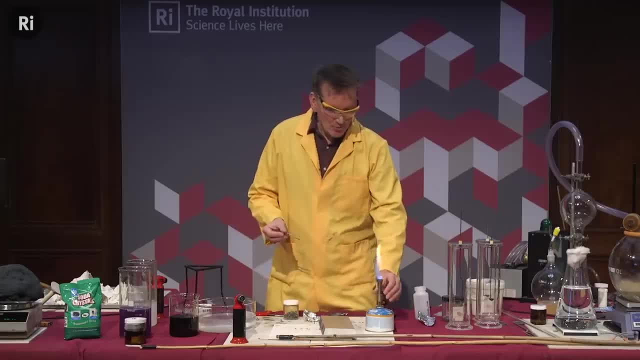 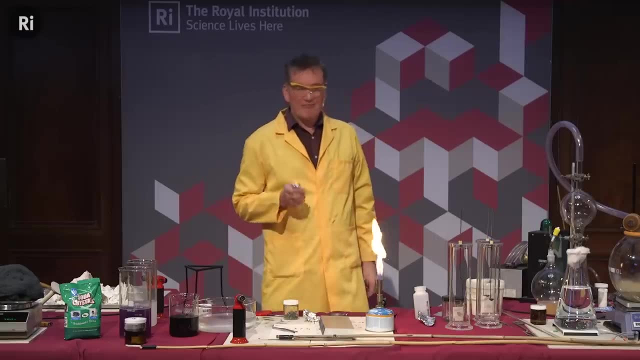 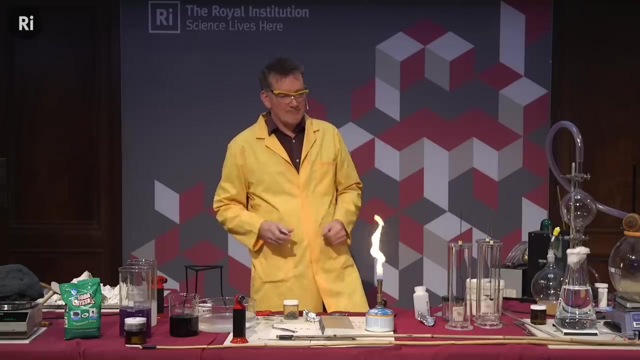 with a brilliant white flame. That was quite exciting, wasn't it? With a brilliant white flame forming scandium oxide. So a very violent reaction there. But indeed it is two atoms of scandium with three atoms of oxygen. OK, 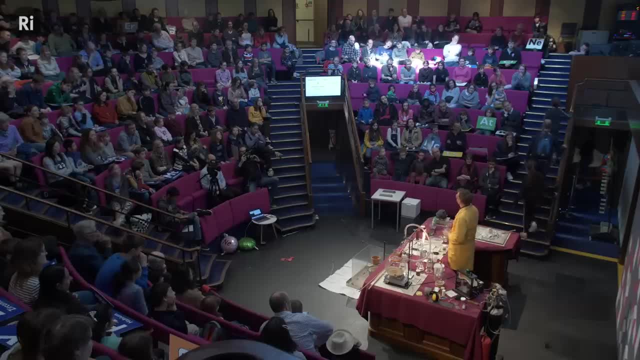 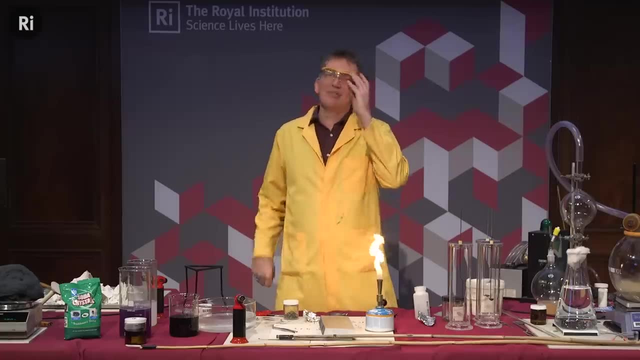 Right? Well, let's pick one of the elements from group three. So we have boron at the top and underneath boron we have aluminium. Can we do the same thing with aluminium? So I have some aluminium Now. who thinks the aluminium is going to burn very easily? 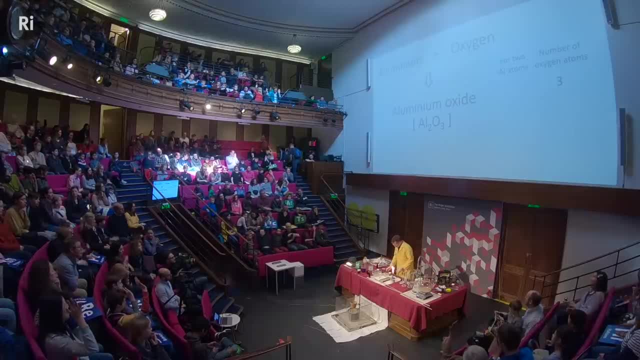 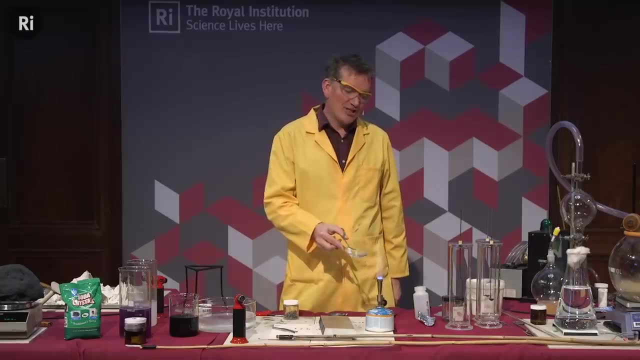 Who thinks it's not going to burn very easily. Well, let's try. So I have some aluminium foil. Well, of course it doesn't burst into flames. We wrap our turkeys with this when we put them into the oven. 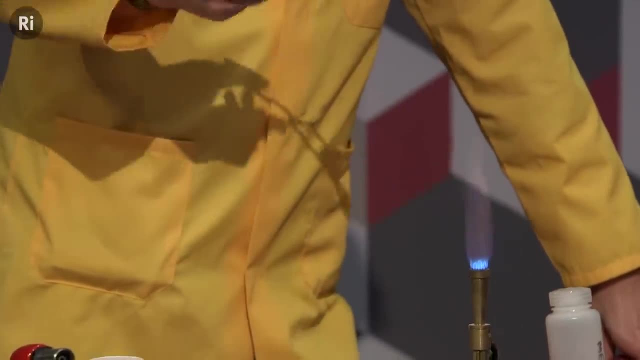 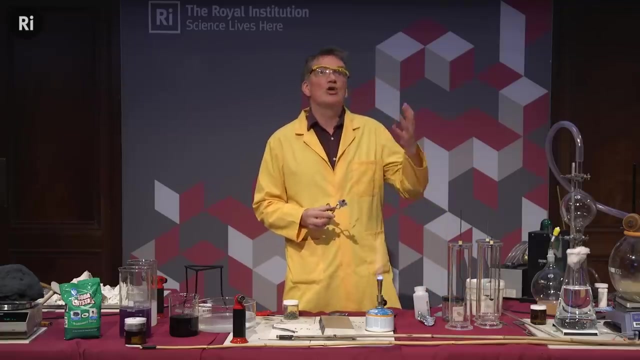 Well, I don't, Because I'm vegetarian, But anyway. but it doesn't burn And actually part of the reason it is forming the oxide. And the formula for the oxide is again two atoms of the element with three atoms of oxygen. 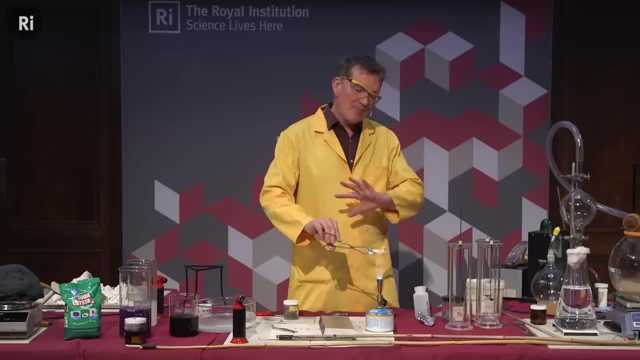 But that's part of the reason why it doesn't burn, because it's actually being protected by a layer of this aluminium oxide which stops it bursting into flames, which is probably a good thing when we're using it Or, of course, with our saucepans if we have a large 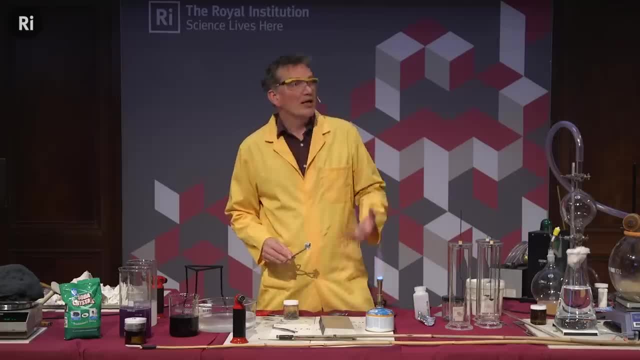 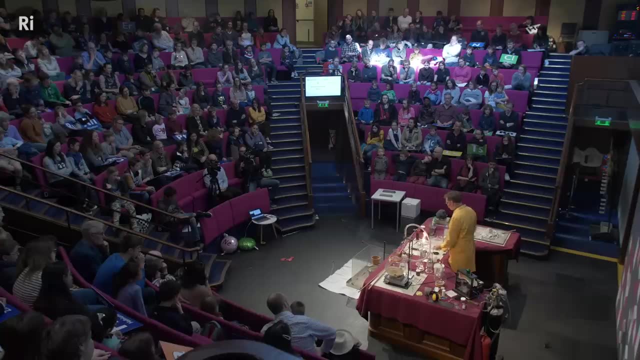 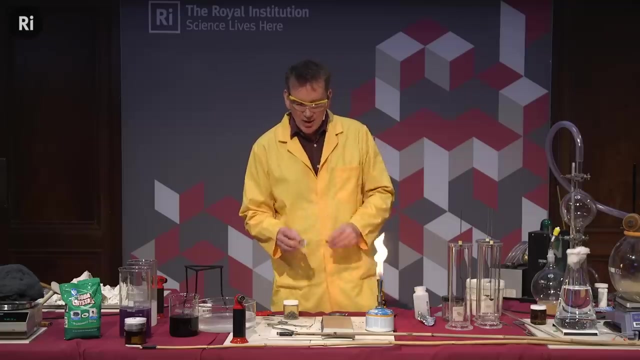 aluminium saucepan. it doesn't burn instantly, And again, it's because it's quite large like this one, But it's also protected with a fine layer of the aluminium oxide. Well, but it is forming the oxide, And so this probably has quite a bit of the oxide on it now. 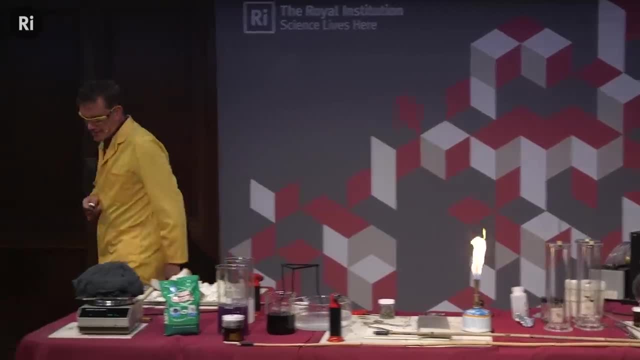 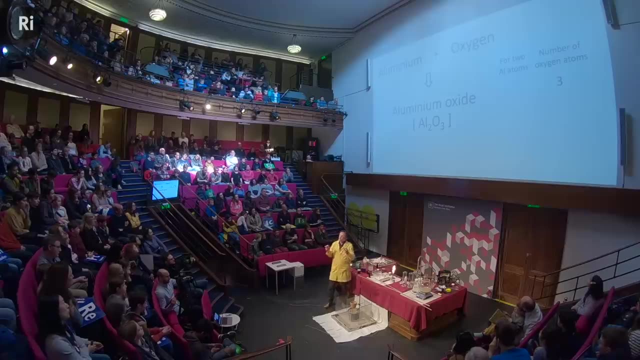 So we can form this oxide And I'm going to try this in a different way. The formula for aluminium oxide is two atoms of aluminium with three of oxygen, And I can make it, but I need a really finely divided aluminium. Remember my big block of magnesium? didn't really react. 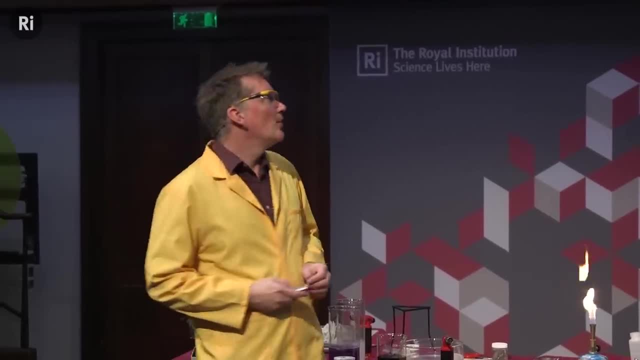 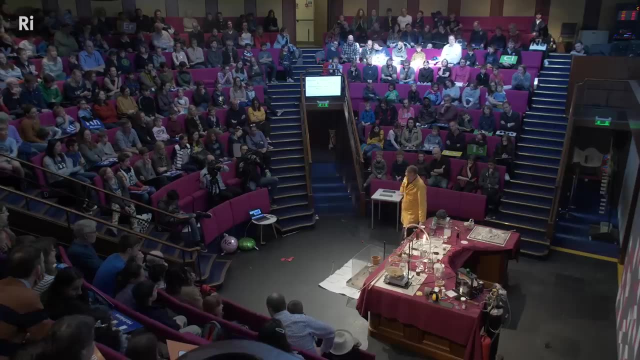 If I have very finely divided aluminium, it should, But I'm going to do this in a slightly different way. What I've got in the flower pot here is aluminium powder mixed with iron oxide. Now the aluminium really does want to combine with the oxygen. 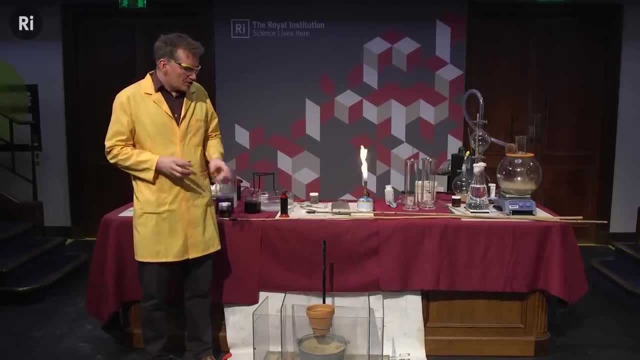 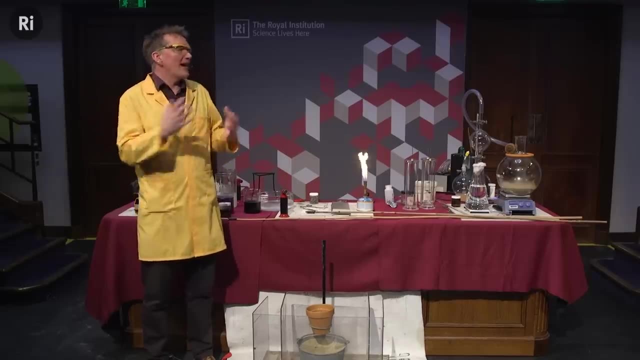 It is a very vigorous reaction when it forms the aluminium oxide. So what's going to happen here? The aluminium powder is going to steal the oxygen from the iron oxide And this is going to form aluminium oxide. That's the driving force for this reaction. 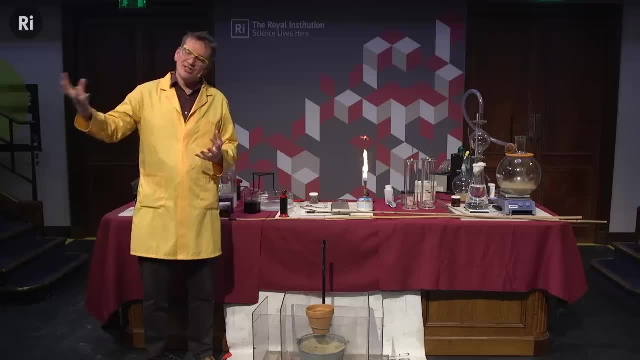 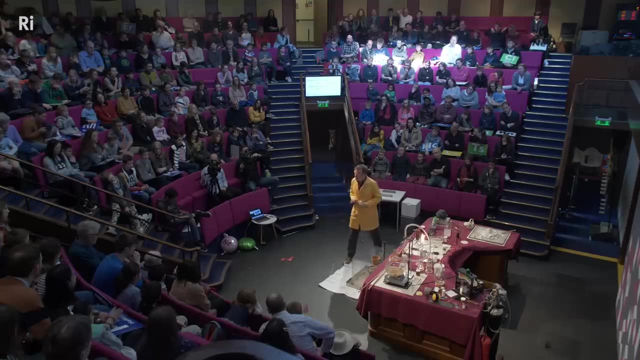 But the other byproduct of this is: well, if the iron oxide has had all the oxygen taken away, we're going to be left with iron, So we should be making some iron. This is another one. I'm just going to ask you just to move back just a little bit. 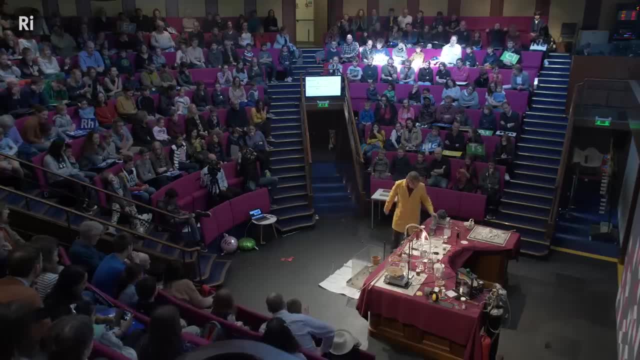 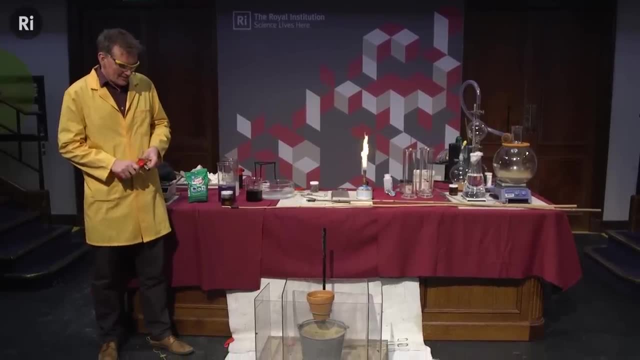 if you wouldn't mind. Thank you, It will be in your best interests, Right? OK, so maybe just a little bit more. You can come back afterwards. That's great, That's lovely. OK, thank you. So, sticking out of this, I've got a little bit more. 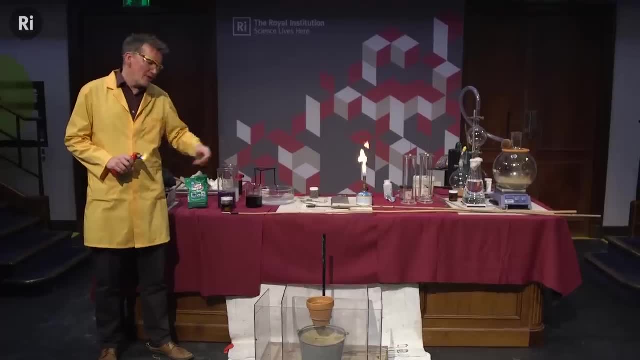 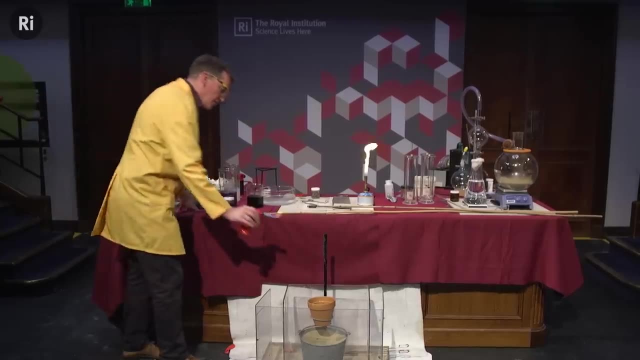 A little piece of magnesium ribbon. So initially I'm going to light that And that will then get the reaction started. So you'll see a white flame, the white bright light from the magnesium and some of the magnesium oxide smoke. So let's just start the reaction. 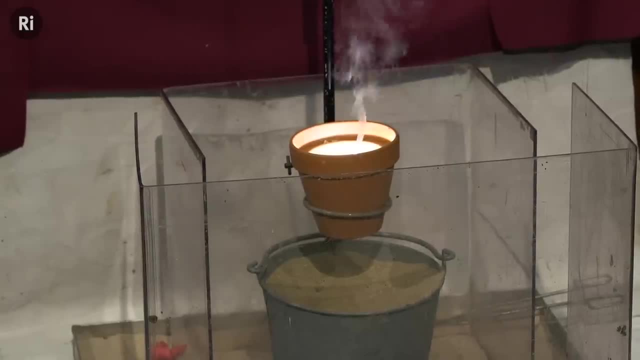 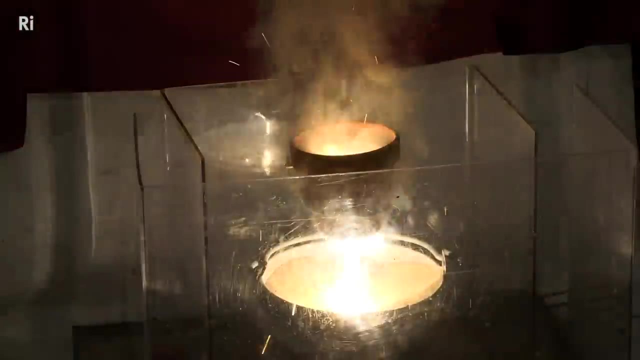 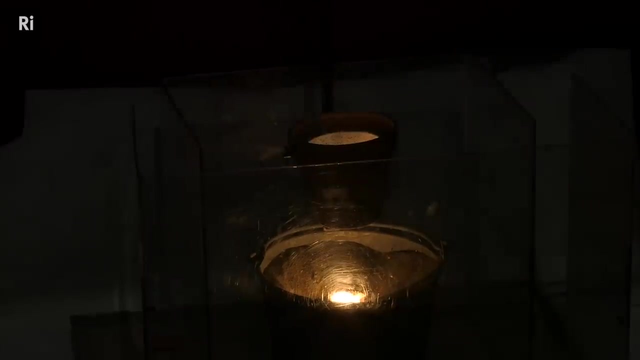 There we are. So that's the magnesium going, That's the bright light of the magnesium forming the smoke magnesium oxide That eventually will get down to the mix and start the proper There. it is OK, that's good, And if you could put the lights down for a second please. 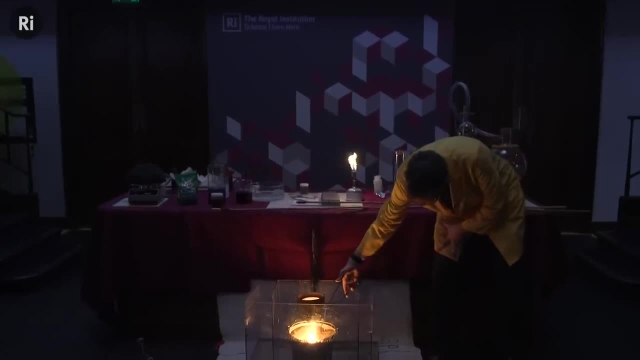 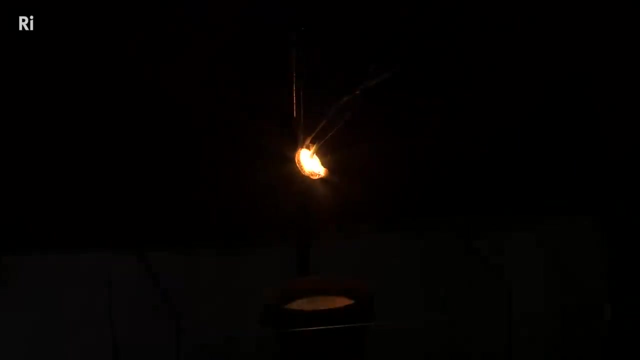 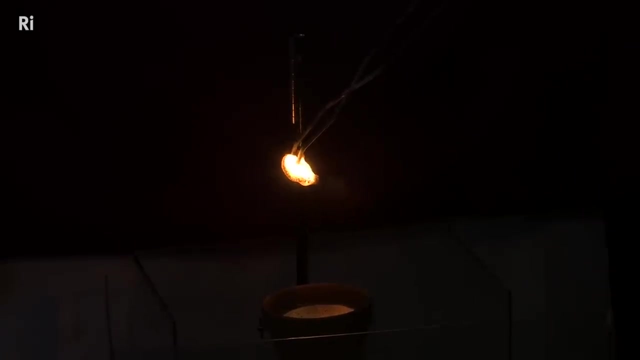 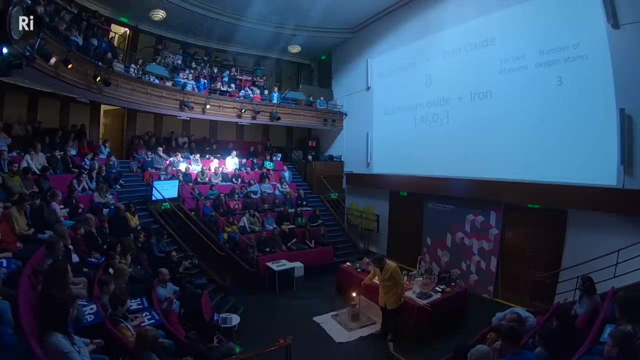 This is. this reaction generated so much heat, And that heat came from the reaction of the aluminum reacting with the oxygen from the iron oxide that it actually produced molten iron. So this reaction is known as the Thermite reaction. OK, and it generates so much heat here. 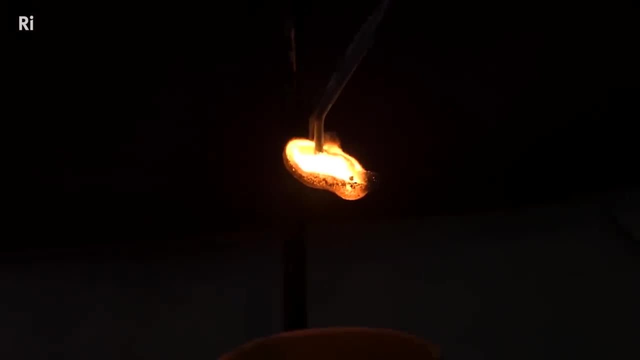 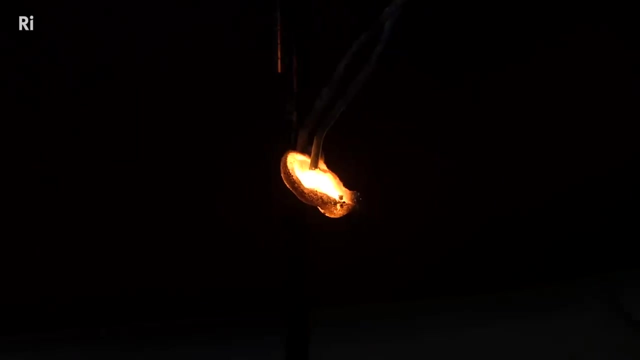 it actually liquefies the iron that's made, And so that was molten iron. coming out the bottom It's still red hot. This is actually very useful. This could be used to make liquid iron- molten iron, when it's needed in rather inaccessible areas. 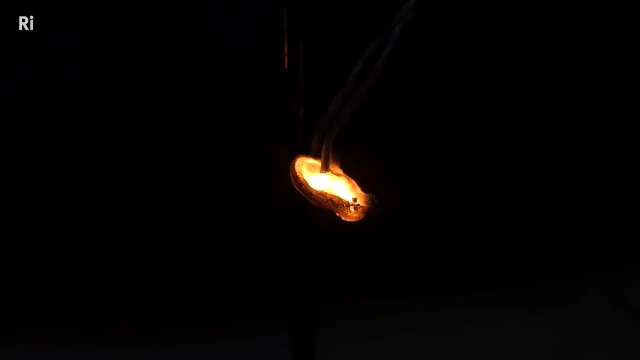 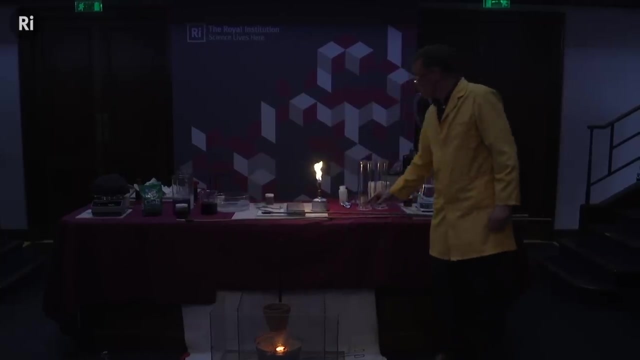 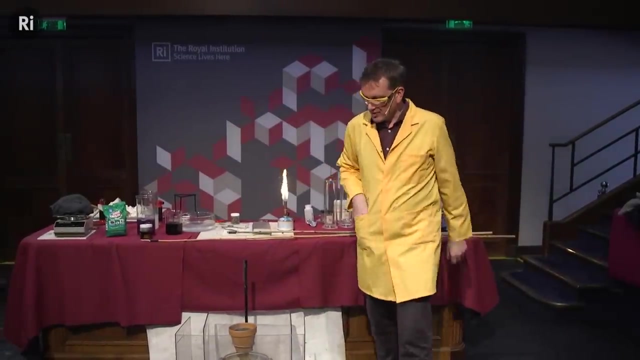 So, for instance, in the construction of railways, you can use this to make molten iron to weld the tracks together. OK, incredibly violent reaction leaves us with molten iron, But it's Given by the strong bonds between the aluminum and the oxygen there, forming aluminum oxide. 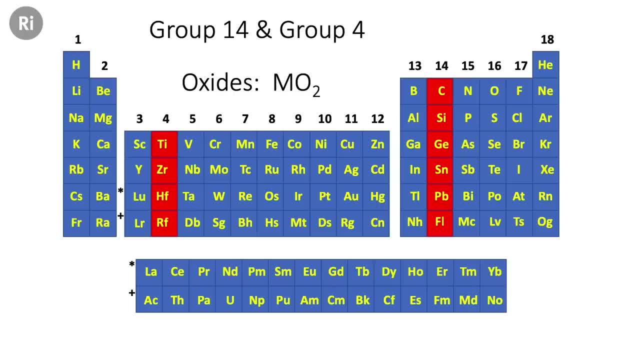 OK, well, let's keep on going through our parent table. Let's go to the elements from group four and group 14.. We have, for instance, the elements titanium, zirconium in group four, But in group 14, we have carbon. 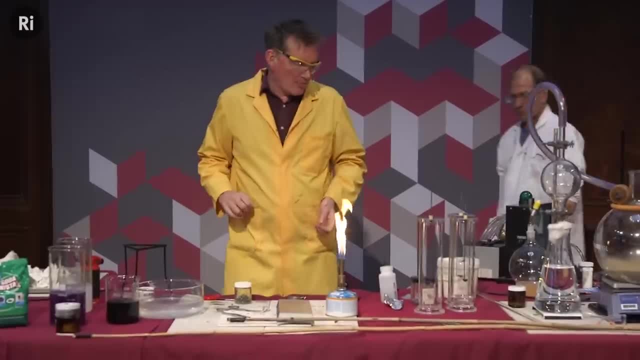 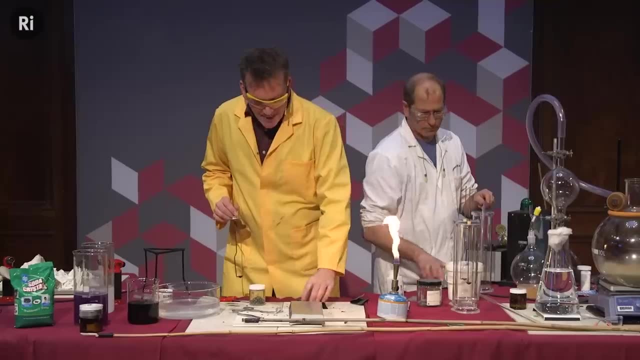 So all of these have four electrons in their outermost shell. I'm going to try a little reaction with some carbon. So Chris is going to put some oxygen into the jar again I have. well, this is some impure carbon. It's actually charcoal. 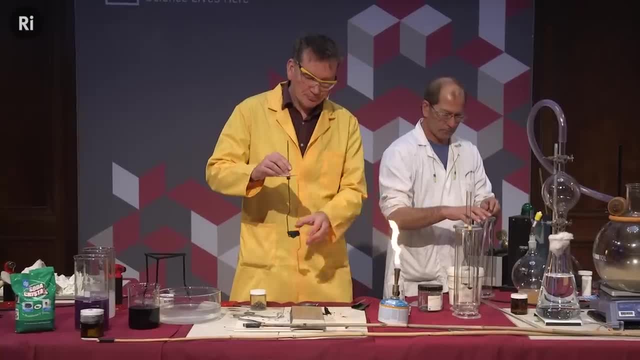 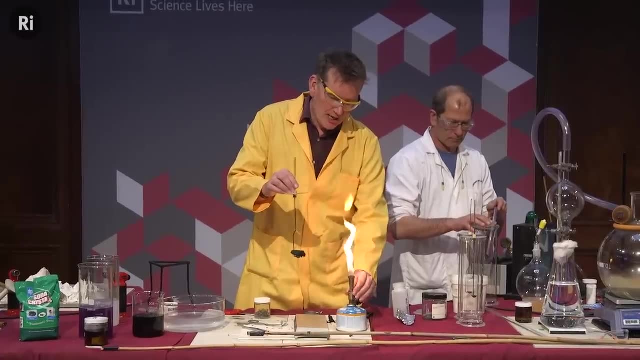 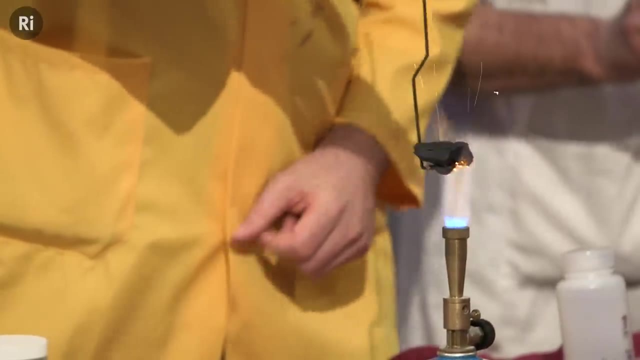 So this is just what you might use in a barbecue. So I'm going to put this on my little spoon here Now. we all know how hard it is to start a barbecue. So you're heating up your charcoal, trying to get it to go, fanning it and whatever. 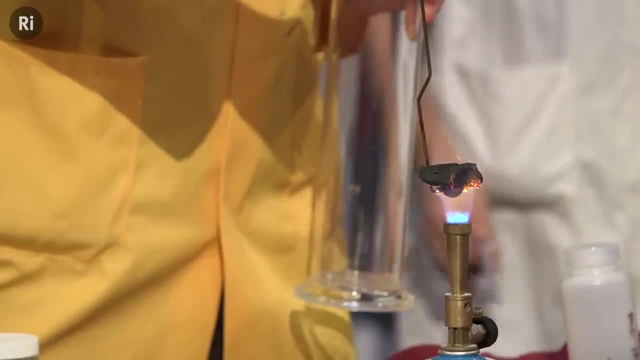 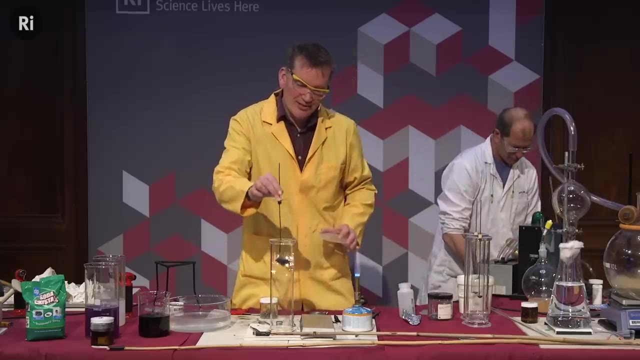 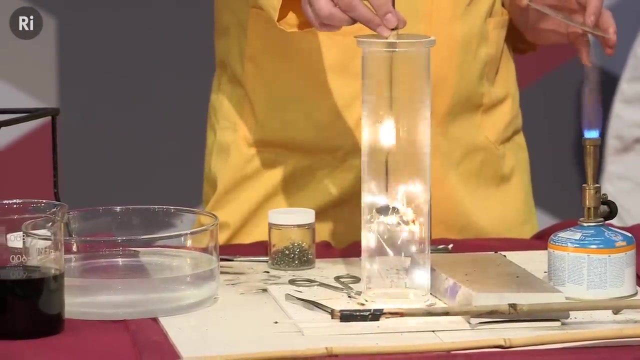 Well, what you really need is some oxygen. So if you have some oxygen to hand- preferably liquid oxygen, always very good, But if you use that, you get a much more vigorous reaction taking place here. So it goes very easily. This is combining with plenty of oxygen. 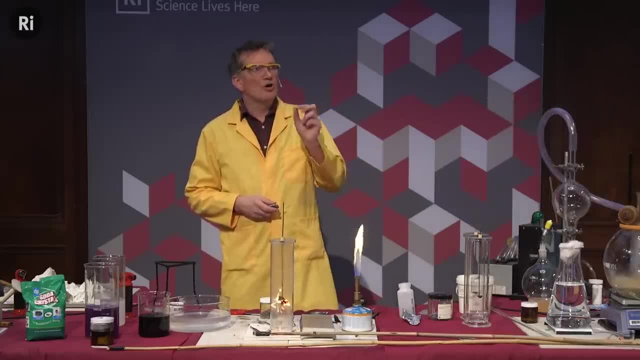 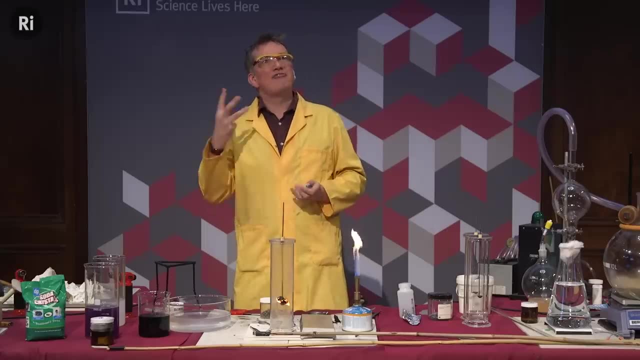 We're going to form carbon dioxide, So one carbon with two oxygens, Or as Mendeleev was looking. so he said how many oxygens combine with two of the atom? So with two carbons we can get four oxygen atoms there. 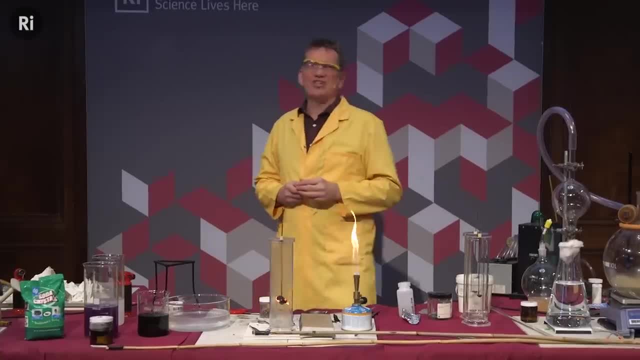 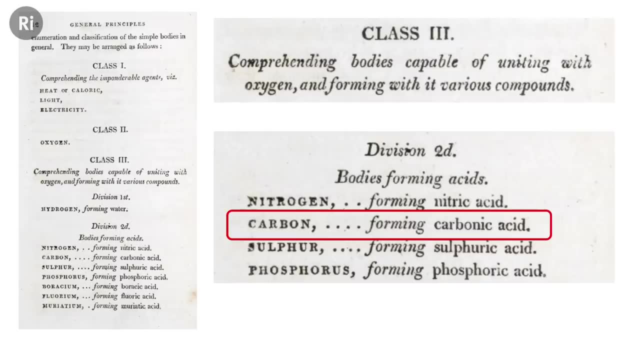 And carbon is in group four. Now remember Marseille's system. She says: well, what sort of compounds are we making when they do combine with oxygen? Well, unlike all the ones we've seen so far, which actually form alkaline solutions. 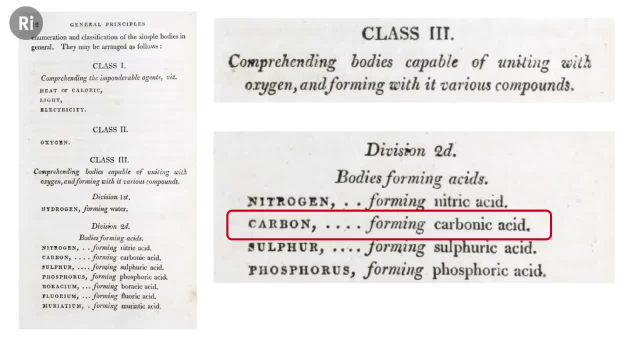 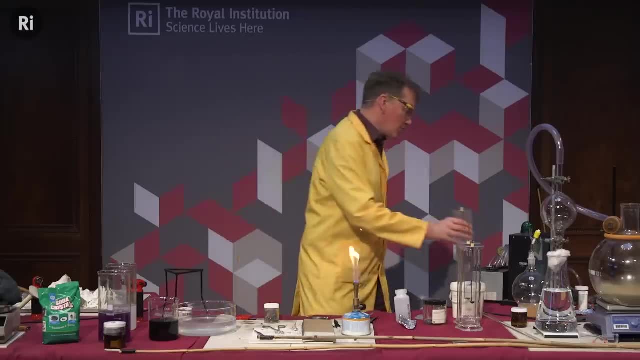 this now forms a very weak acid solution. So if we dissolved the gas here- carbon dioxide in water or fizzy water- it's weakly acidic. We can also call it carbonic acid. We get stronger acids if we keep moving across the periodic table. 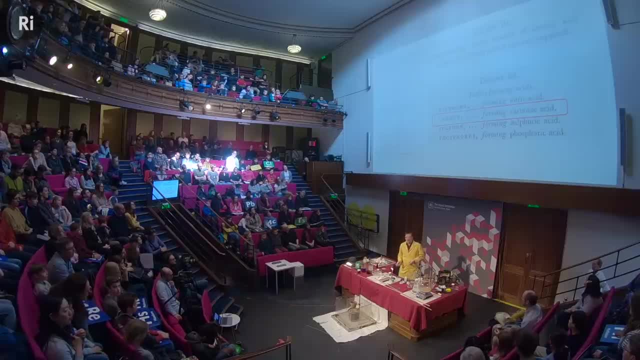 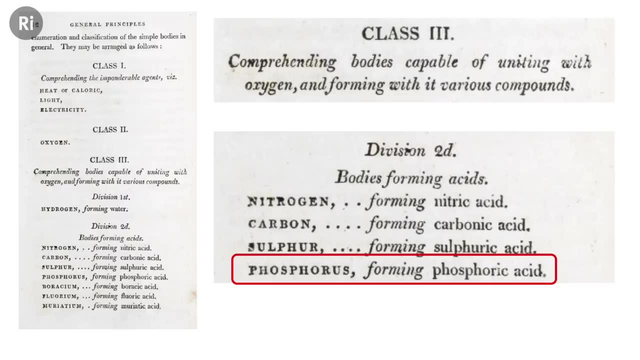 So from group four or 14, we go to group five or 15.. And at the top of that we have phosphorus. When phosphorus reacts with oxygen we get an oxide. This has the formula: two oxygens with three or up. 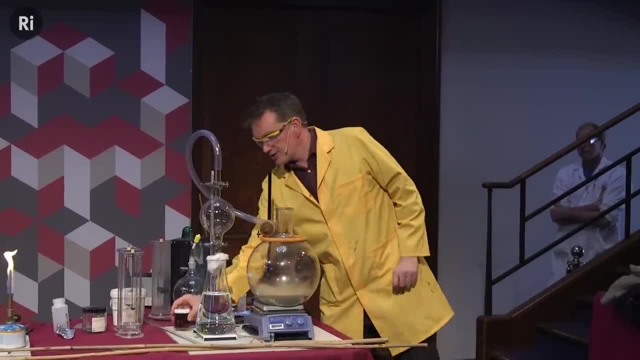 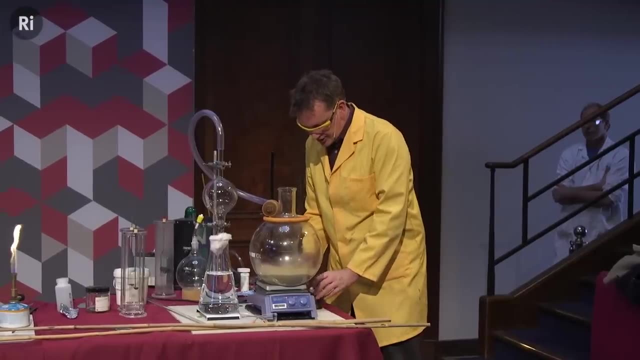 to five oxygen atoms, And if we dissolve the smoke in water, we end up with an acid, phosphoric acid. So I'm going to show this now. I have a little piece of phosphorus here. I'm going to add this to the flask here. 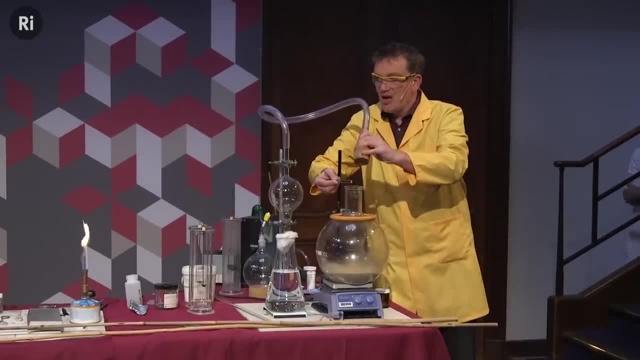 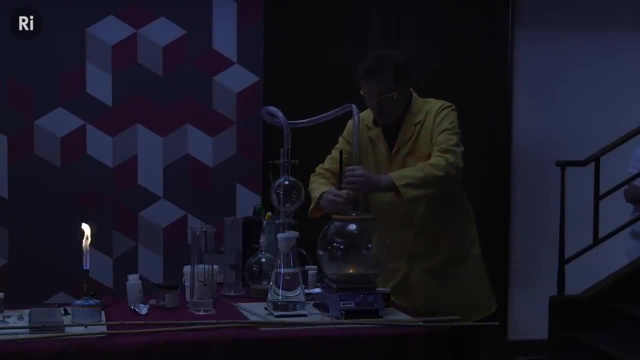 The flask is full of air And there's some hot sand in the bottom- If we have perhaps the lights down for this, please- So I'm just going to drop my phosphorus in. So it's on the surface of the sand. 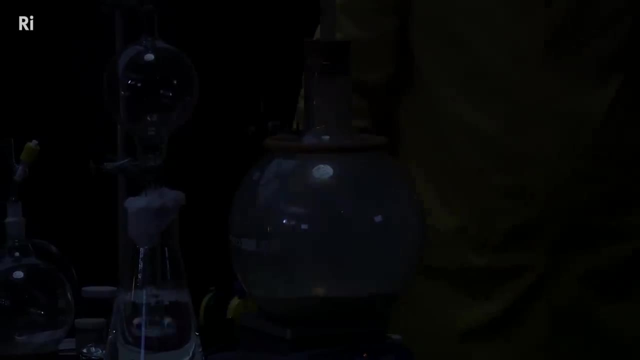 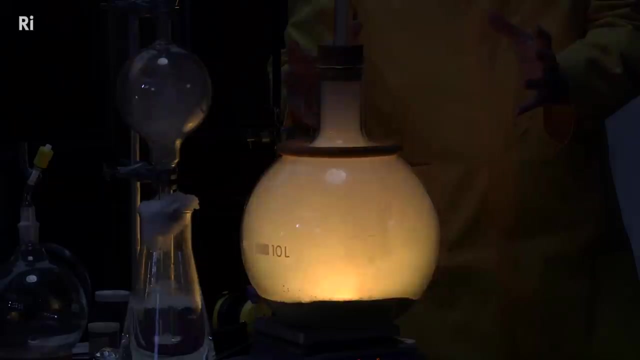 And it's instantly reacted And it's burst into flames And it's giving out a fantastic light. In fact, the name phosphorus means the light bringer. It's giving out a lot of lovely light here, So that's how it gets its name. 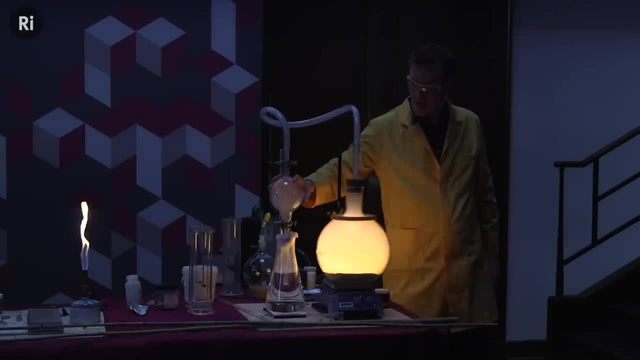 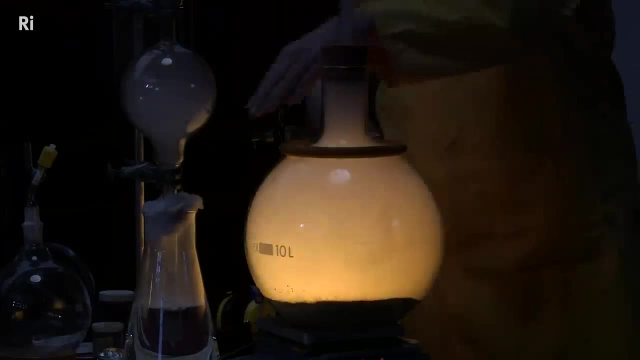 But the smoke that has been safely absorbed by the apparatus here. well, this is phosphorus, the oxide It's. here We can have up to P2O5.. It forms phosphoric acid when it reacts with water. So this is making an acid. 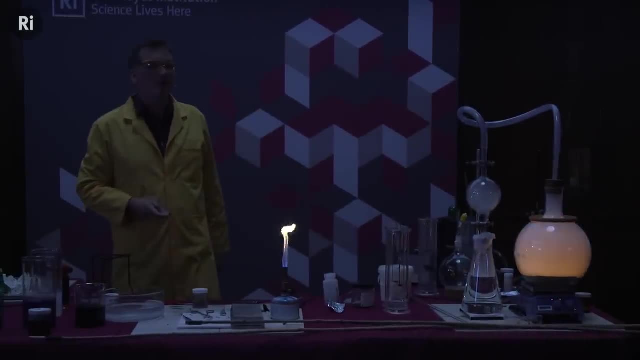 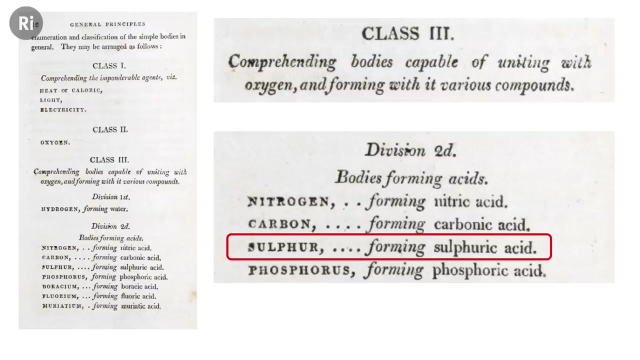 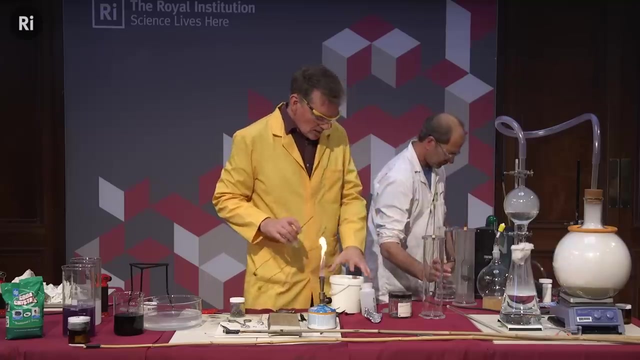 Two phosphorus, though with five oxygen. Well, let's keep on going. After phosphorus in group five, we have sulfur in group six. I have some sulfur in here And again. Chris is just going to put some oxygen into the gel. 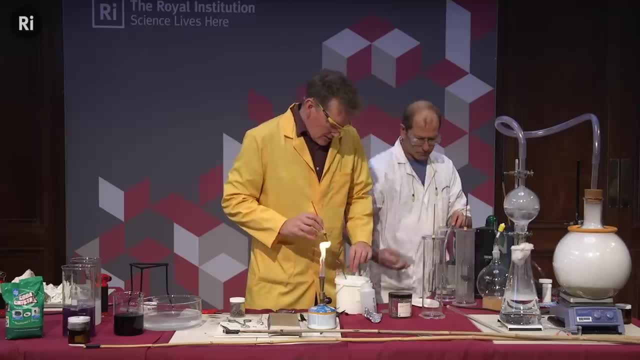 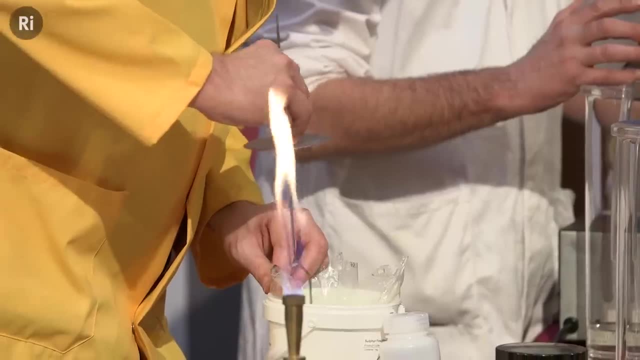 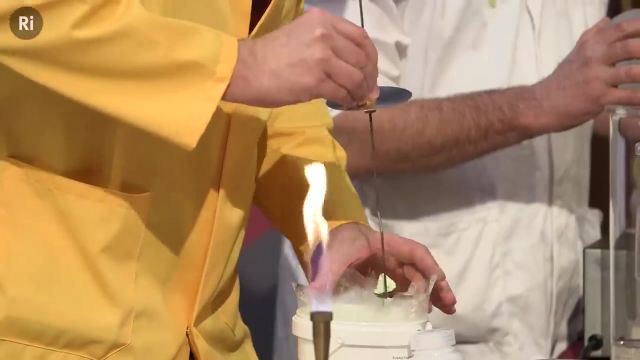 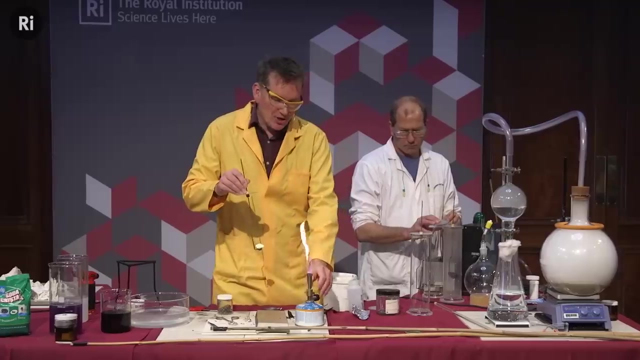 And I'm going to pick up a little piece of sulfur. So here is some sulfur. Now, sulfur, an old name for sulfur. in fact, the name that occurs in the Bible for this is brimstone, And this is because, well, you can find lumps of this lying. 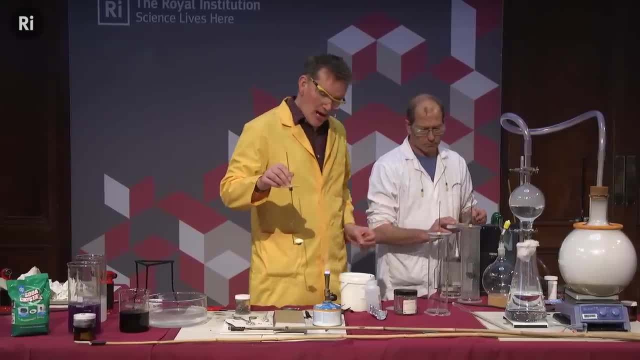 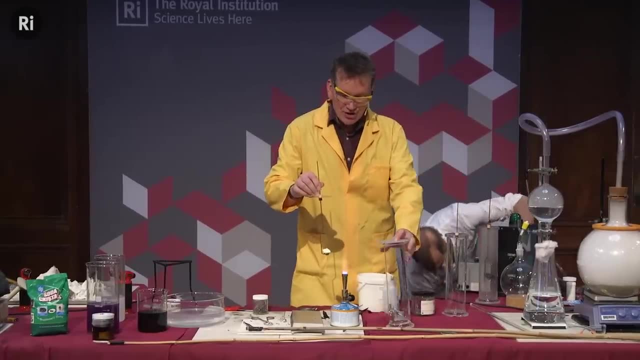 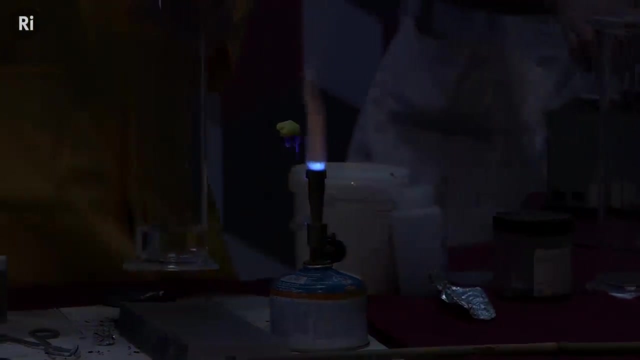 around, especially near volcanoes. So it's thought to be a mineral. But the name brimstone means burning stone or the stone that burns. So, if I just start this, to react with the oxygen there And again, if we can have the lights down, perhaps for this. 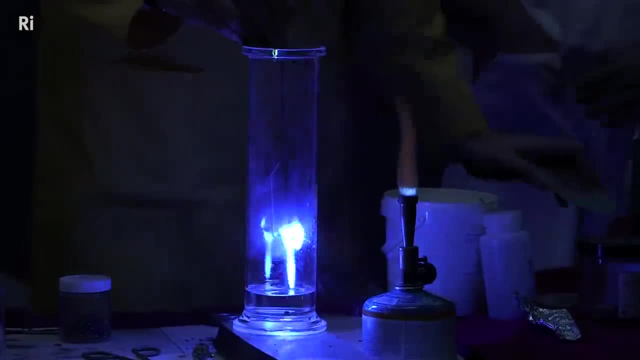 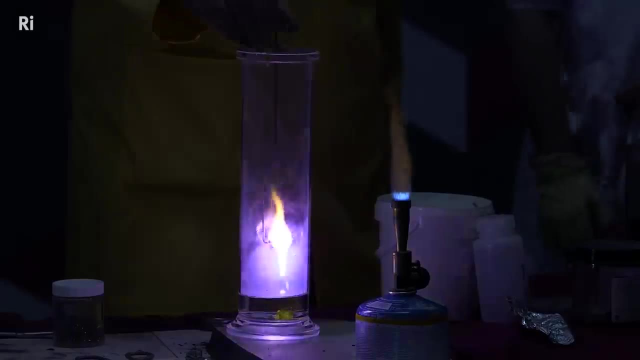 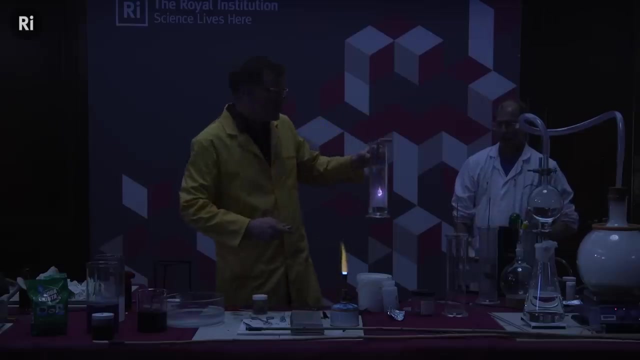 So I think it's now going. If I lower this in, we get a fantastic blue light as the sulfur is burning. OK, that's rather nice, And again the smoke that's being absorbed with the solution. at the bottom there is an acid. 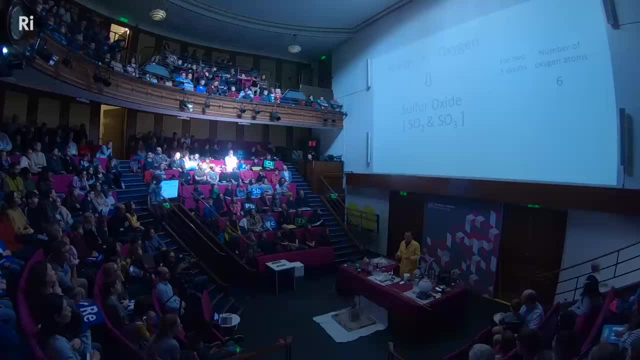 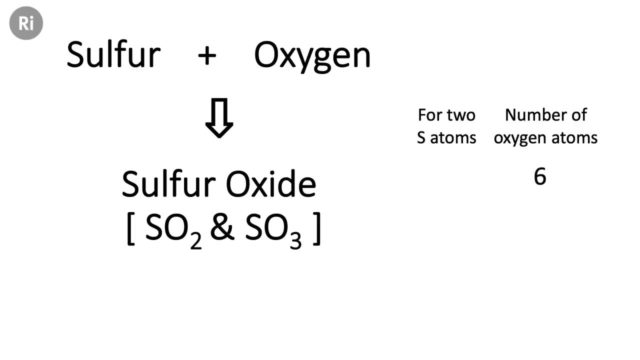 But the formula for this is? well, we can have one sulfur with two or three oxygens, Or as Mendeleev, when he was considering how many oxygens combined with two atoms of the element, So two sulfurs would combine with up to six atoms of oxygen. 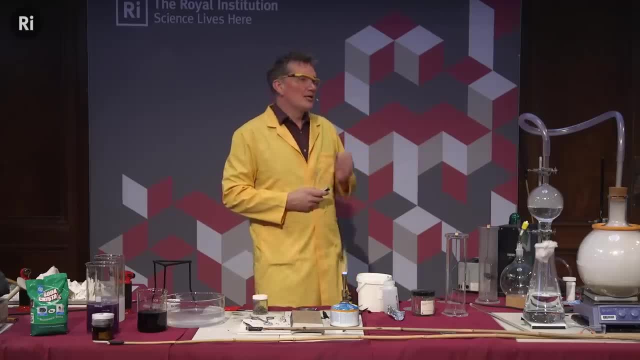 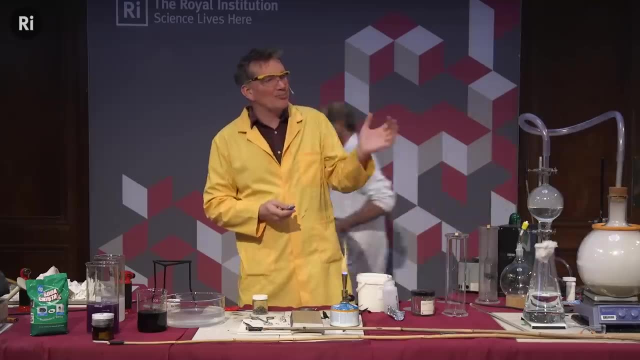 And sulfur is in group six of the periodic table. So if we look at Mendeleev's system again, he was saying how many atoms of oxygen combine as we go across the periodic table. This was all because, Because of the number of electrons. 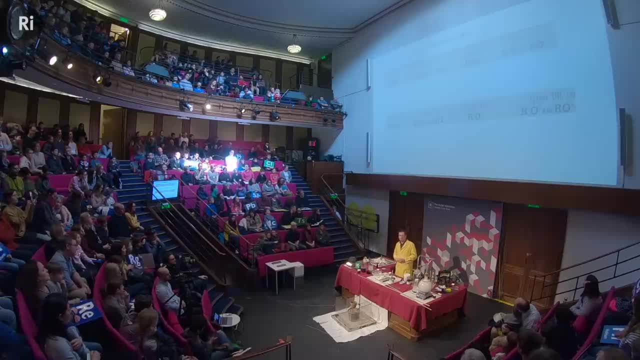 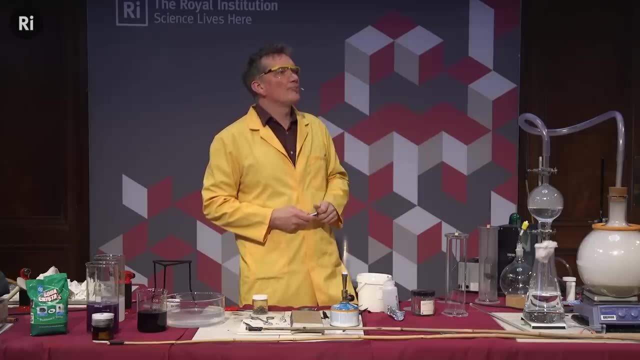 that these atoms have in their outermost shell that can be used to form bonds. So we saw, for instance, hydrogen and lithium both react with oxygen, with two of the metal with one oxygen, Whereas from group two we have two with two. 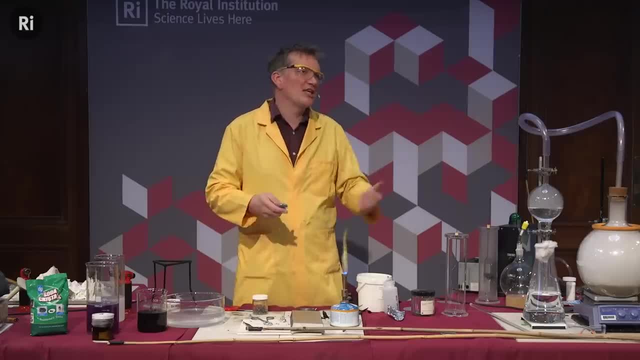 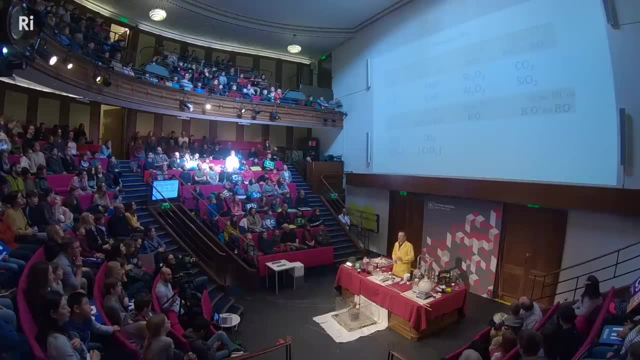 Or well, we'd now say that the formula for magnesium oxide is MgO, or CaO for calcium oxide. But as we keep on going across, we're increasing the number of oxygens that are reacting. We got as far as sulfur. 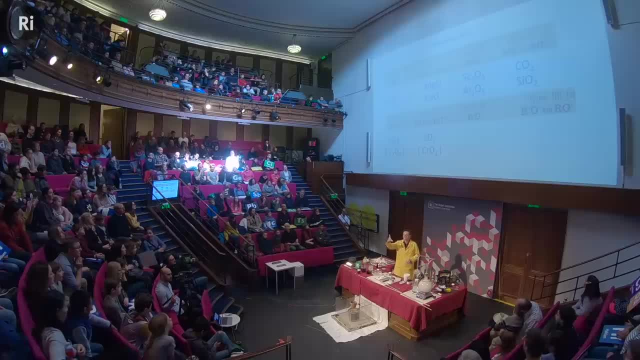 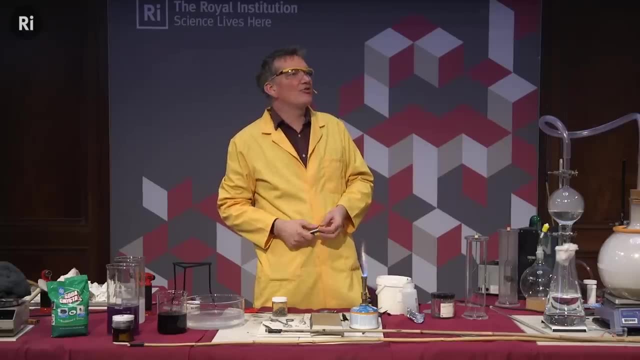 That was from group 16.. We could have had Chromium from group six. it forms an oxide, Chromium trioxide. We could have continued and I didn't. We could have elements from group seven and even from group eight, and they still fit the trend. 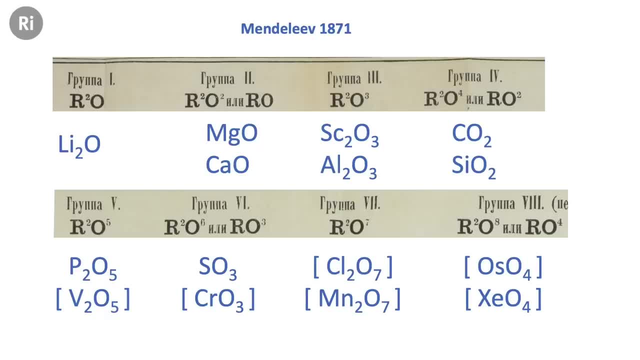 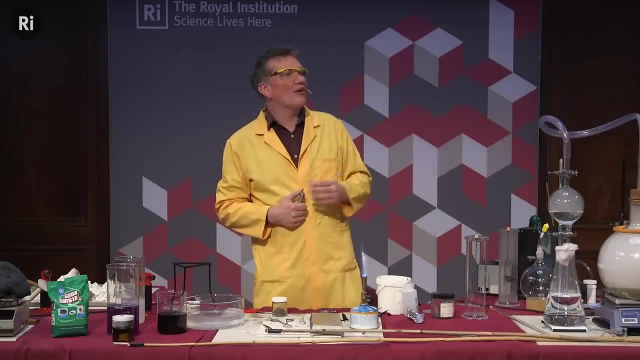 The reason I didn't show these, of course. well, chlorine is very poisonous And these compounds are very poisonous and also highly explosive. Similarly, for the osmium tetroxide that we have there, it is rather poisonous. And the xenon tetroxide, well, it's not poisonous. 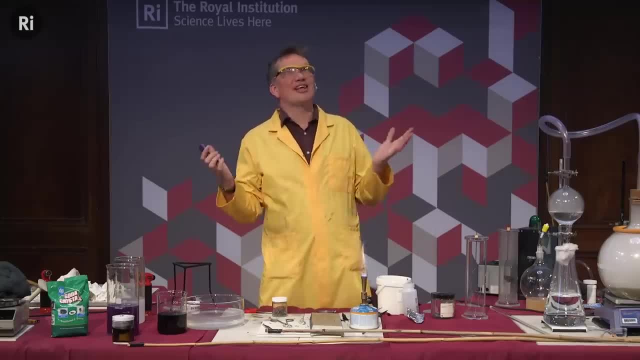 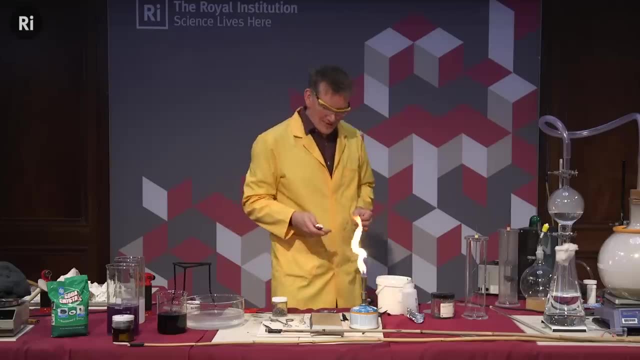 Because all it does is explode very violently and forms the harmless gases Oxygen and xenon. But it's because it's very difficult to make this compound and it is highly explosive. That's why I couldn't show you any of that, But the trends continue throughout the periodic table. 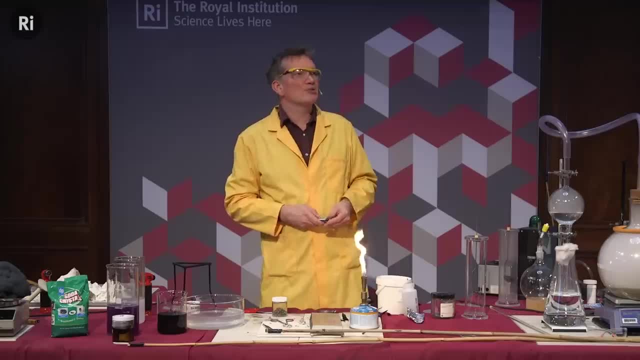 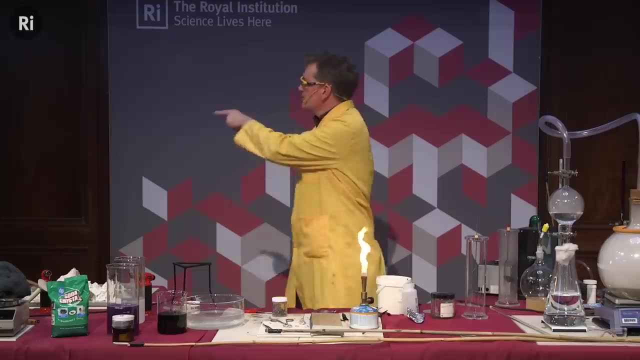 OK, What I want to do now is now. I did say that I'd try and explain why it is that our noble gases exist as single atoms, And in order to do this, we need to use the bonding machine that we have here. 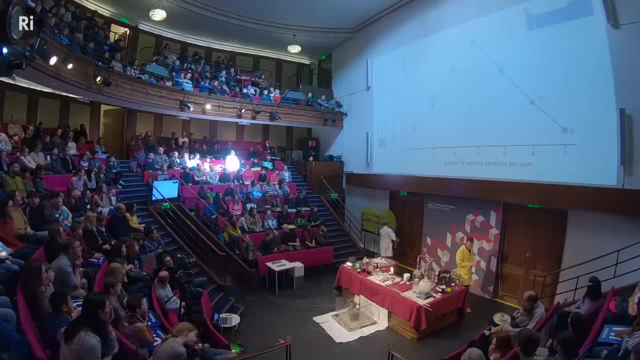 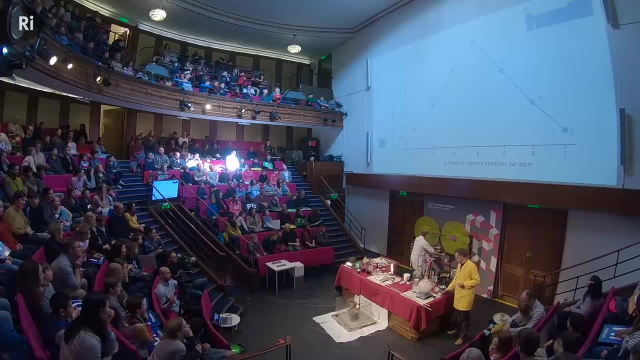 So Chris is just going to bring this on And we're going to look at. well, why is it that some of our elements, in fact most of them, are metals and form very strong bonds between the atoms, whereas for our noble gases they? 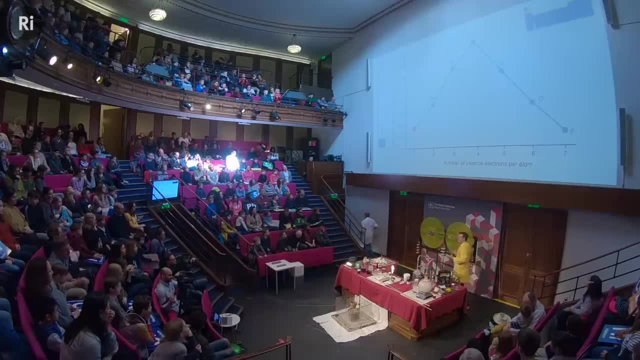 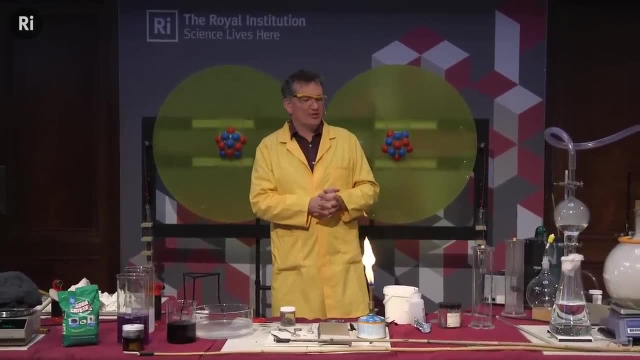 exist as individual atoms. Well, it's all to do with how many electrons do these atoms have that are available to form bonds with their neighbors? So when I have a sample of metal, such as a sample of lithium, for instance, this is my titanium. of course, we 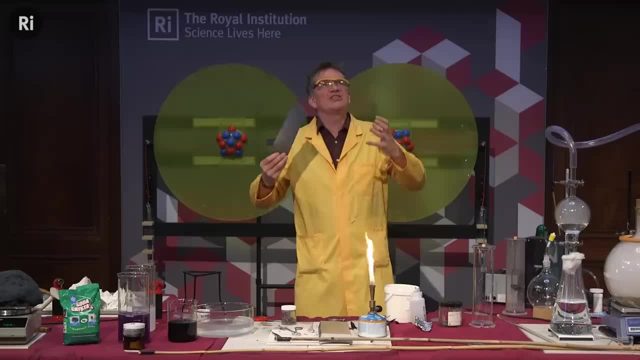 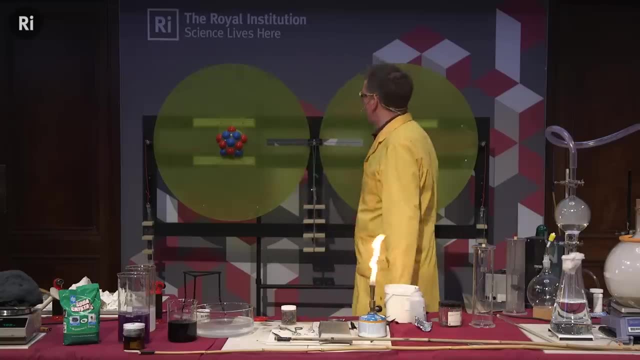 have many, many countless atoms here, OK, And they're all bonding together, But they are bonding together Using just the outermost electrons that they have available. Now, if we have lots of lithium atoms, each lithium atom, it can only use its one outermost electron. 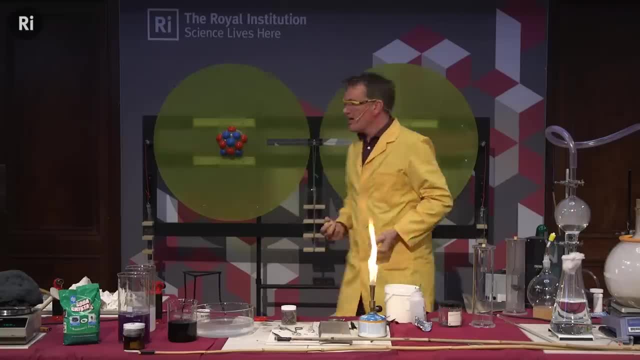 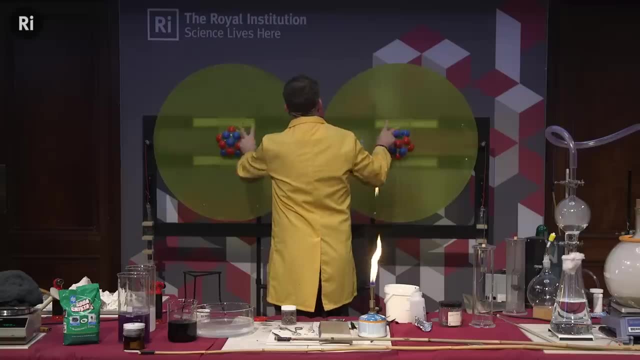 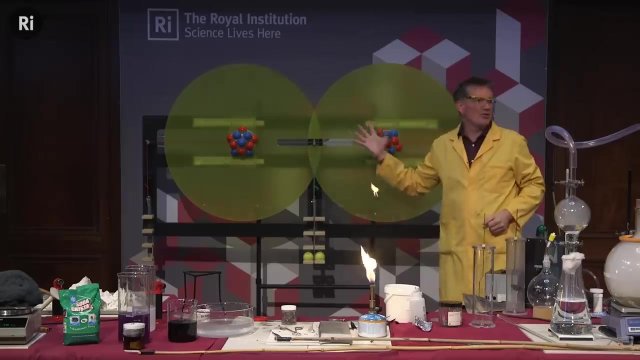 to form bonds to its neighboring atoms. OK, Now, these electrons do form bonds. We can think of these as the negatively charged electrons going in between the nuclei of neighboring atoms, And this helps glue them together. That is our bond. So we have our electrons in between the nuclei here. 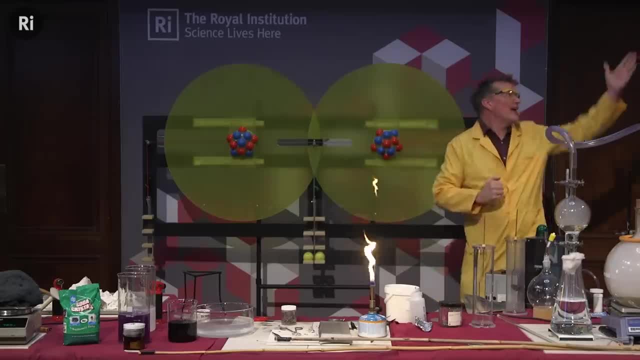 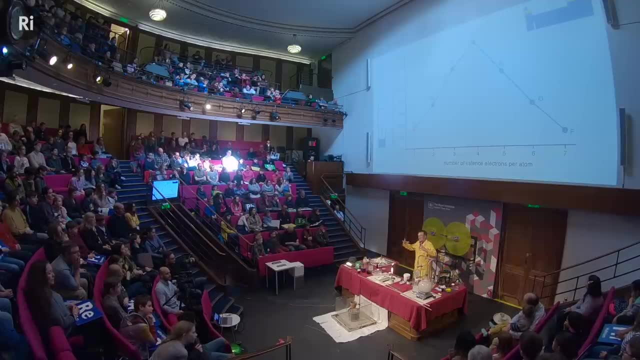 to give us our bonds, But we only have one electron for any of our group, one elements to form these bonds, And this means that we don't need much energy to separate the atoms again afterwards. OK, And this is what this graph shows. 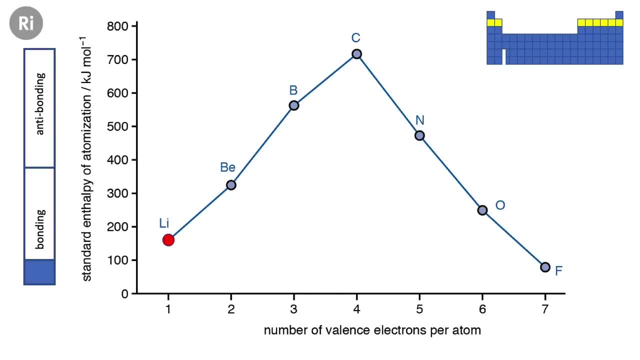 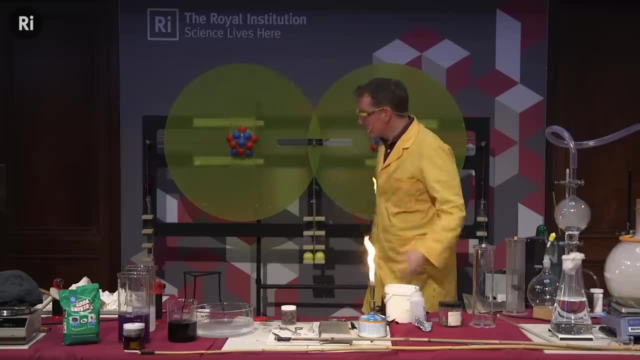 So this graph shows how much energy is needed to separate a given number of atoms of any of the elements in their normal form. So to separate lithium, we don't need an awful lot of energy If we move across from lithium to beryllium. because each beryllium atom has two electrons that it can use well. these help to hold all the nuclei even stronger together. So we form stronger bonds. So we need more energy to separate a load of beryllium atoms from the solid than we do for lithium. 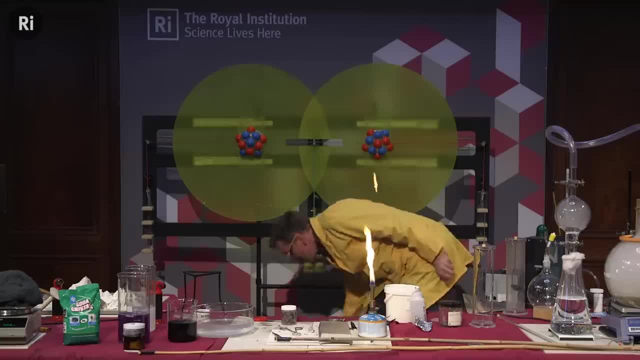 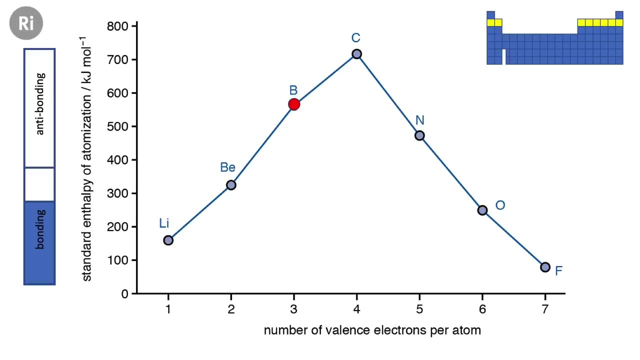 If we keep on going, we get them to boron and we have three electrons per atom to form all our bonds And this means the bonds are even stronger now, So we'd need more energy to separate the boron. And if we keep on going, we get to carbon and carbon here. 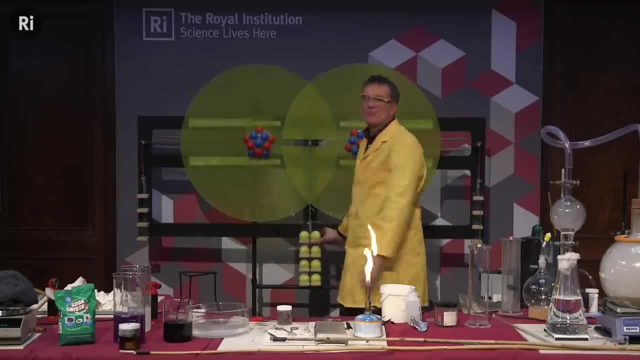 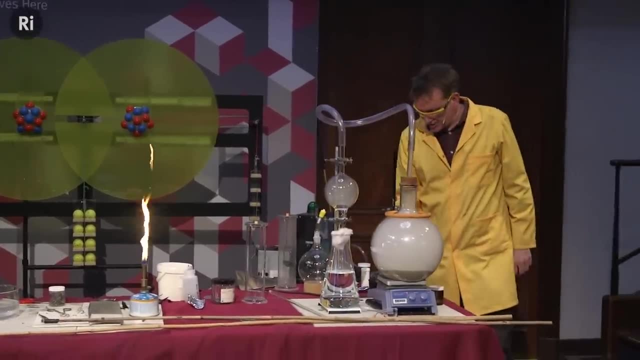 with four electrons And if we keep on going we get two electrons per atom and we get three electrons per atom to form really strong bonds. We'd say that each carbon atom forms four bonds around it to the other atoms that are near it. 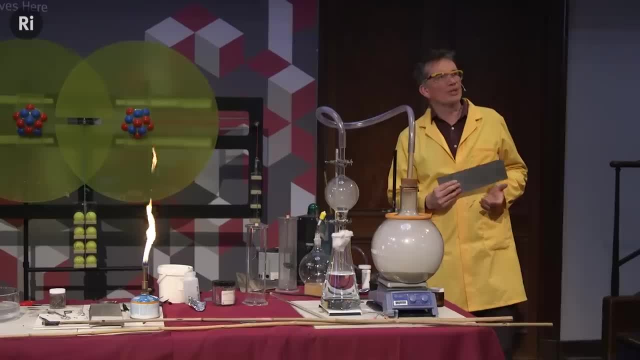 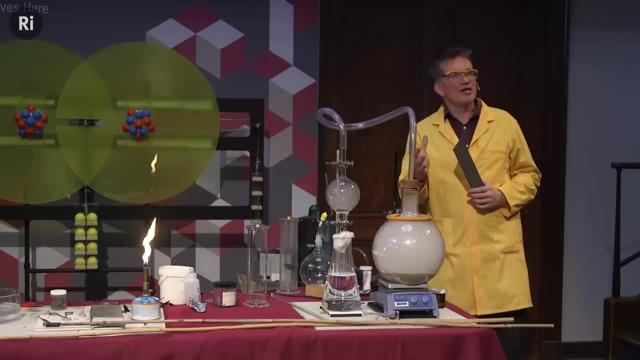 So this is well a form of carbon. This is actually graphite, And it turns out, then, that carbon has the highest boiling point and melting point of all of the elements, with perhaps one exception. So this is because it has just the right number of electrons. 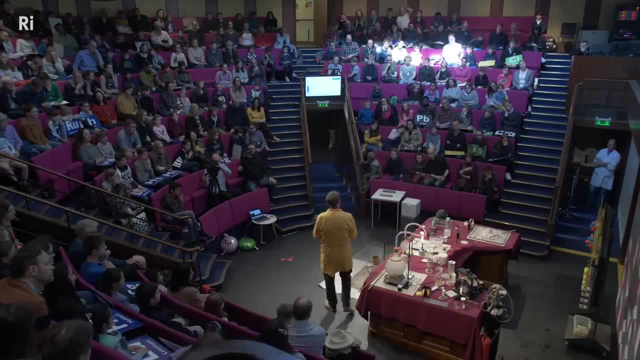 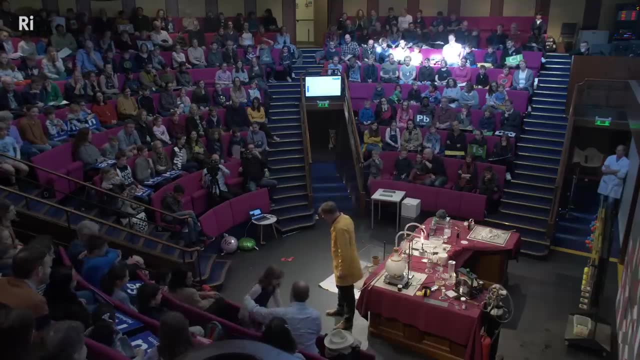 I have a little demonstration that I'm going to show you here, but I need another volunteer. Oh, your hand went up very quickly. yes, Would you like to just come round to the front then, please? Okay, excellent, very good. 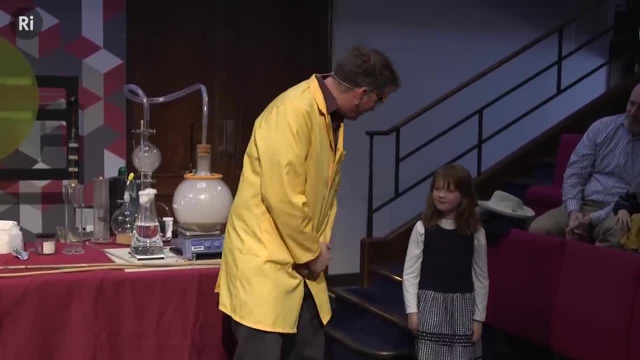 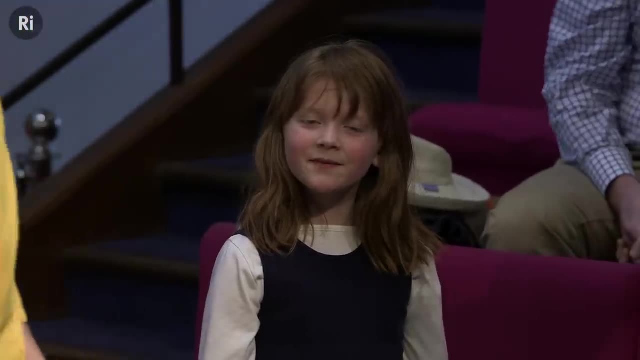 Okay, do you like carbon? Yes, you do good. Which is your favourite form of carbon? Do you like charcoal, or do you like graphite, or do you like diamonds? Oh, diamonds, there's no hesitation there, Right, well, okay, if you come round this way, please. 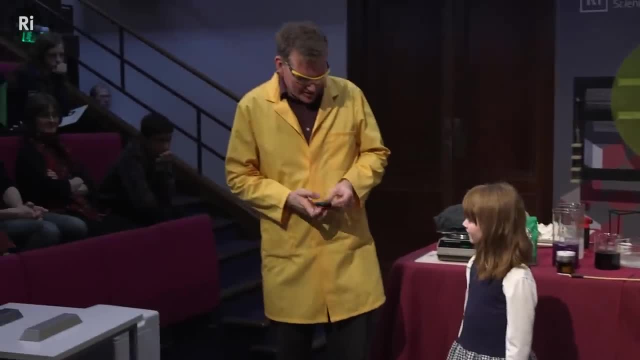 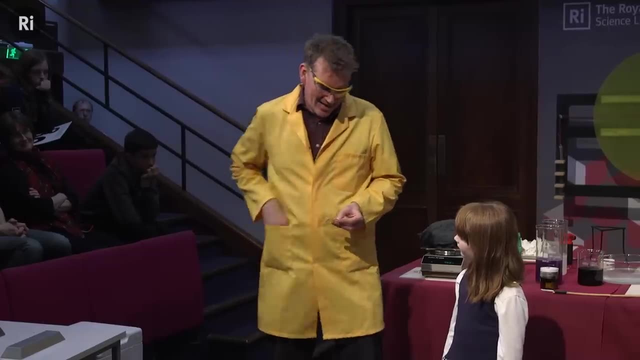 I have a diamond in my pocket. This is a real diamond and it is several thousand pounds worth, so please don't break it. So if you just hold that for me, that's right, that's good. Okay now. so that is a real diamond. 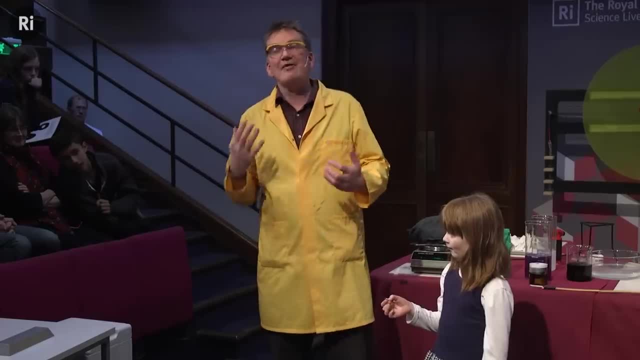 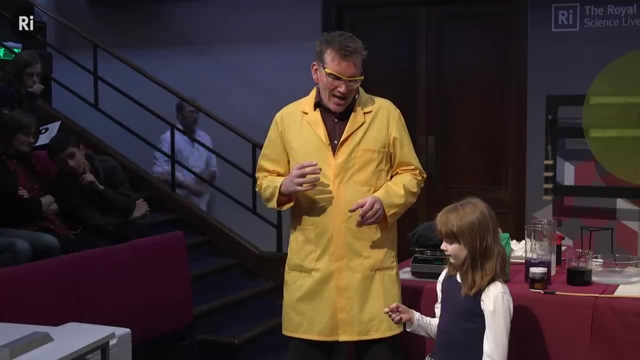 Diamond does actually have well, diamond and graphite. they have some of the highest melting points, boiling points, okay, But also because the bonds are so strong, this means you might be able to break it, so don't try, because it is several thousand pounds. 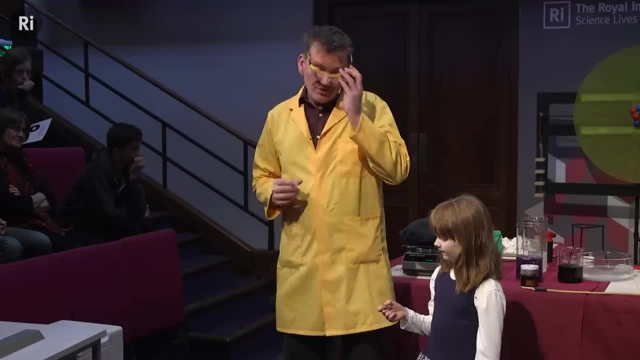 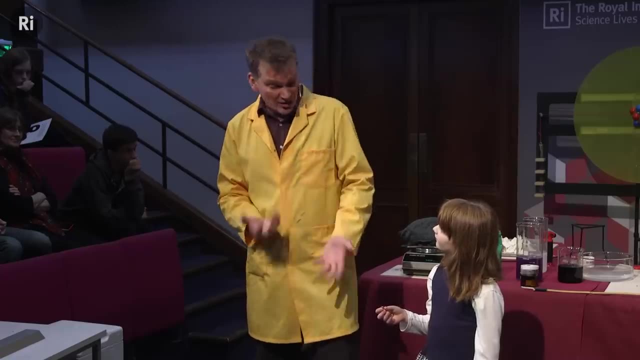 But it is the hardest substance and so this means that actually, that diamond there, you could scratch anything with that. okay, You could scratch glass, you could scratch metal. nothing is harder than that. It doesn't mean to say it's indestructible, it isn't. 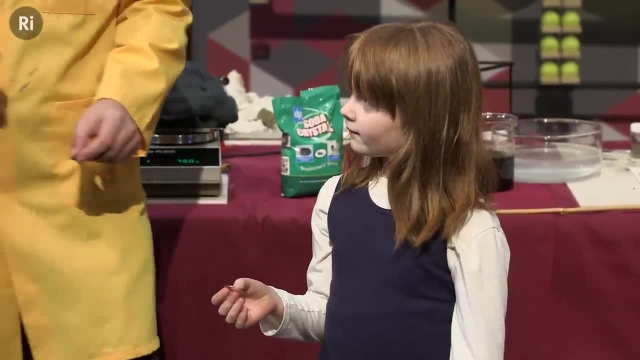 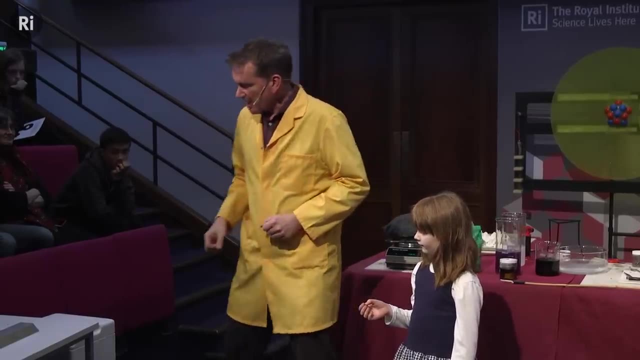 So this is something you can try later afterwards. I shall leave the diamond for people to have a go with, But there's another really interesting property which is what I want to show you now, and this is that diamond is also the best component. 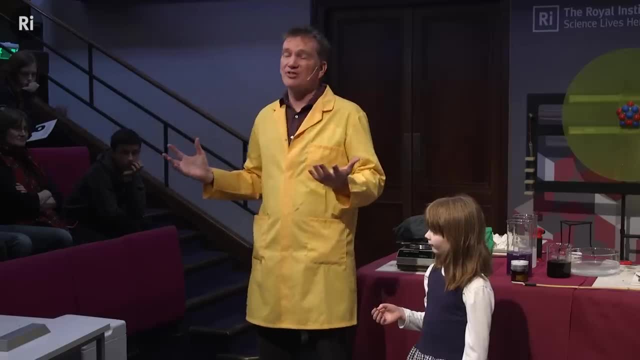 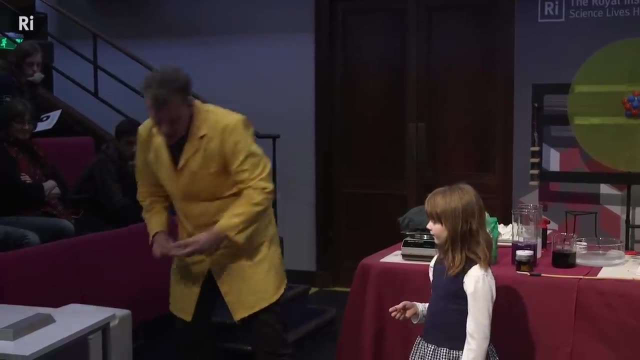 and the best conductor of heat of all substances. There's nothing better, And this is because of the really rigid bonds that we have between the atoms here. Now, what I have is just a little piece of ice Now, at the moment, how does this feel? 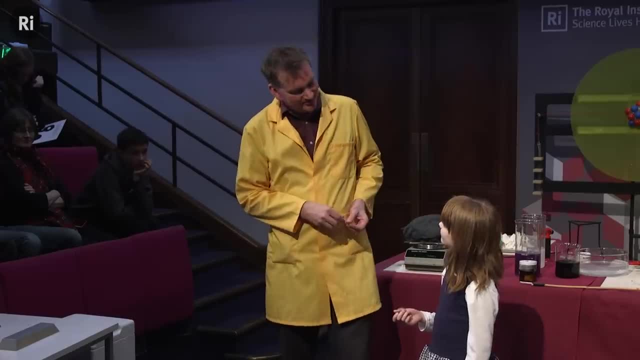 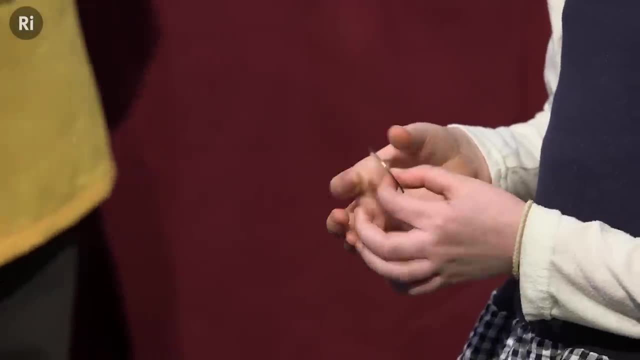 Does this feel hot? Does it feel cold Or is it room temperature In the middle, exactly room temperature. Now, what I want you to do is just hold it like that. That's it like. just hold it. that's it just on there. lovely, like that, yes. 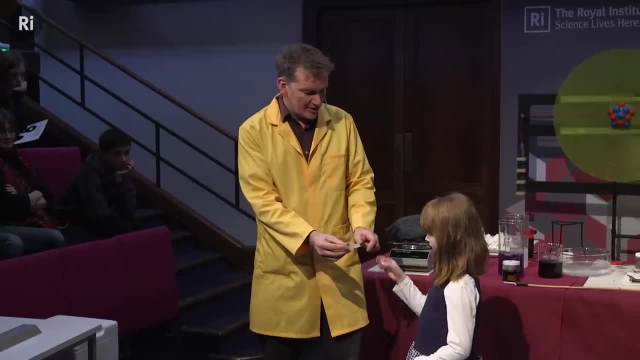 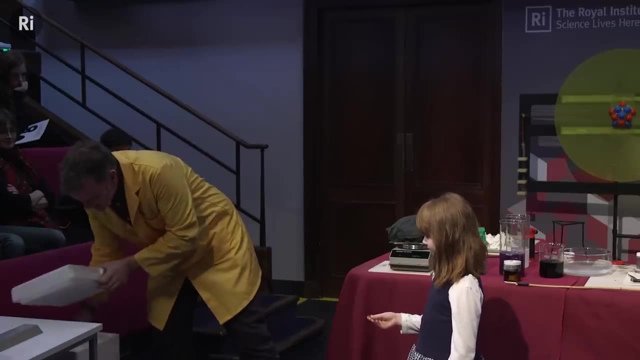 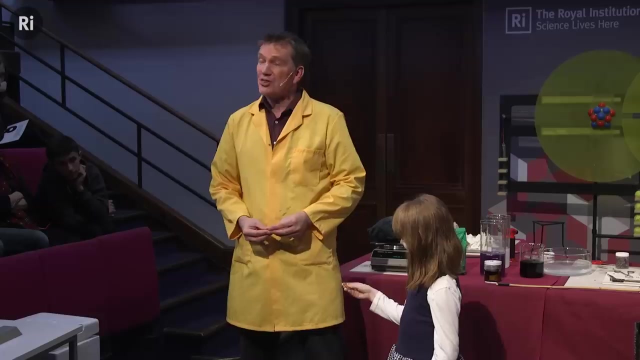 Now just push gently, push gently onto this, onto my ice. Now what did you feel? Did you notice anything? It went cold. it went instantly cold. And we'll just try this again. just try pushing down So instantly it goes cold and you cut through. 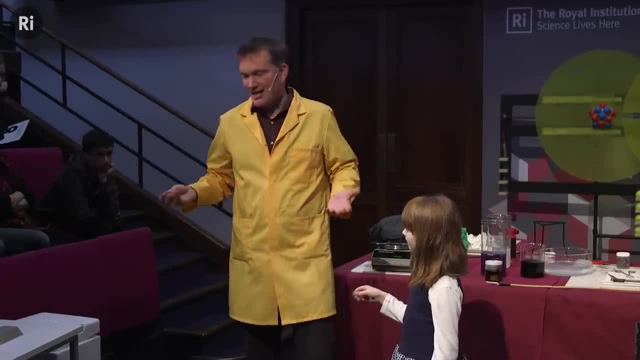 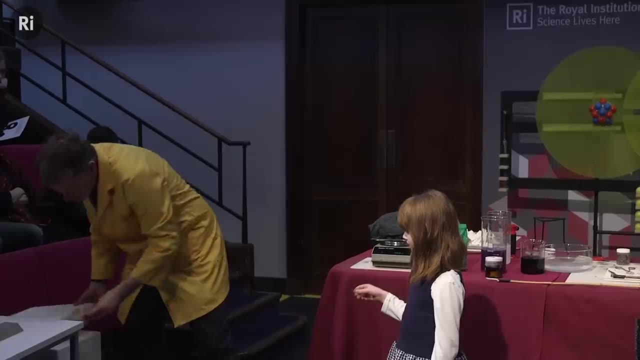 You're cutting through, not because it is hard, which it is okay, but you're cutting through because it's using your body heat. Let's have another little piece of ice here to have an ice cube. So just push against that. so just gently pushing. 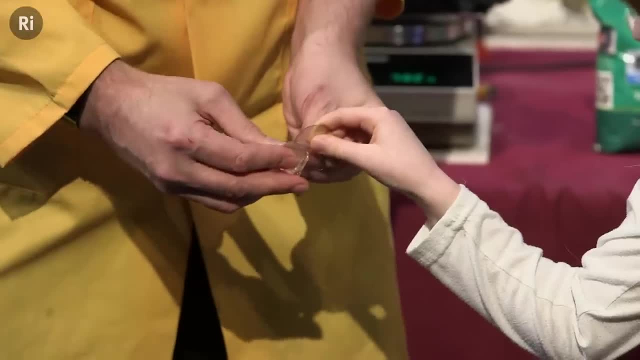 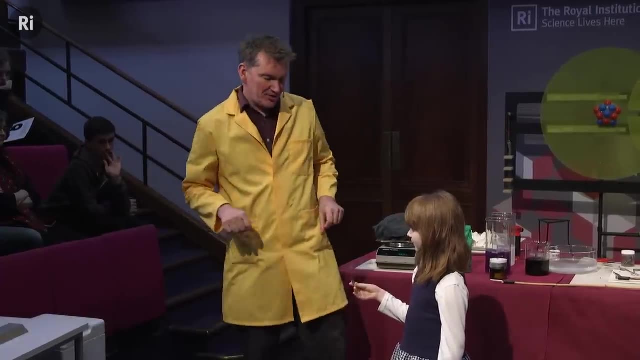 and you can feel it instantly slicing into this, And it gets very cold, doesn't it? And that's because it is the best conductor of heat. It's better than any other substance. So of course we would normally. I'll just take that one back, thank you. 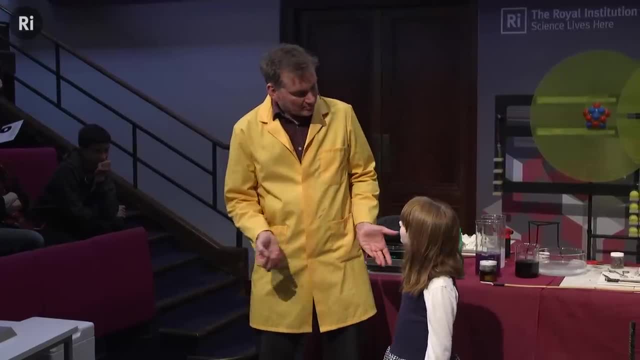 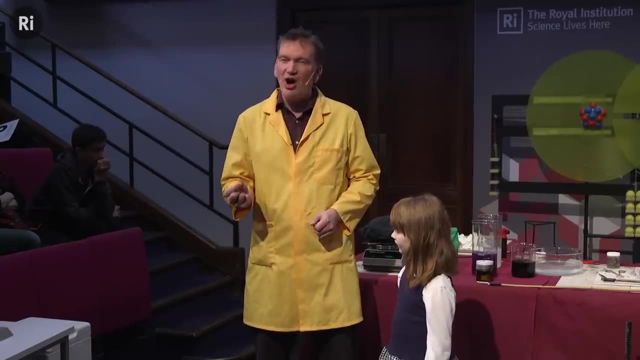 So we would normally, of course, use metal for our cooking pans at home, for our saucepans okay, because they are very good conductors of heat, But actually the best substance you could use would be diamond. So I'm predicting now that in the future you will get diamond frying pans. 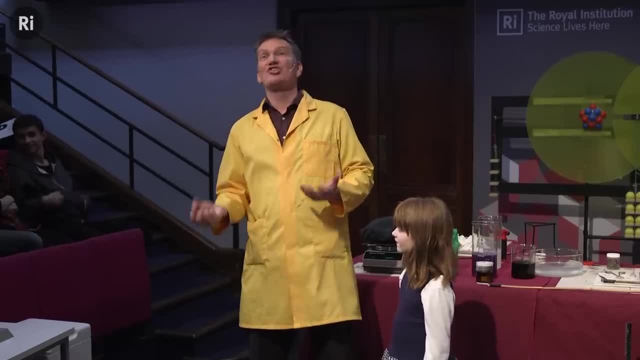 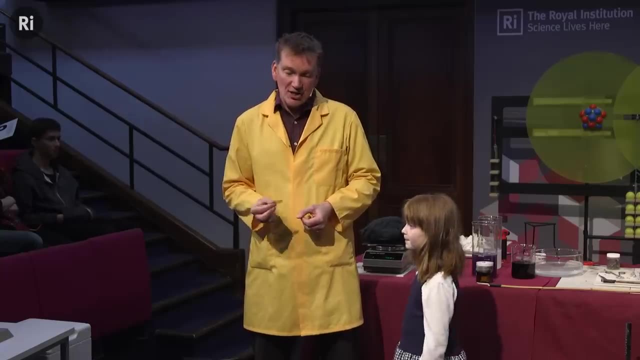 Okay, it would be great because you know it would be wonderful and see-through. You won't be able to scratch it with anything, okay, apart from maybe another diamond, And it's a really good conductor of heat, the best conductor of heat. 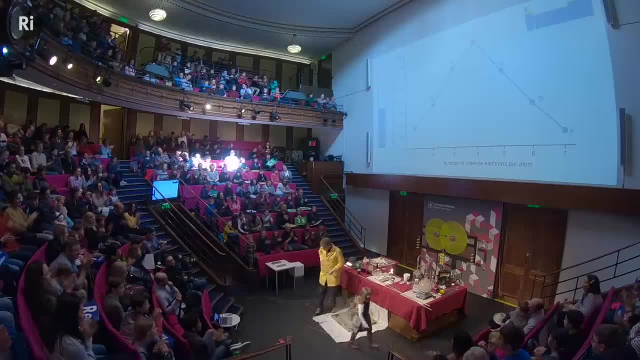 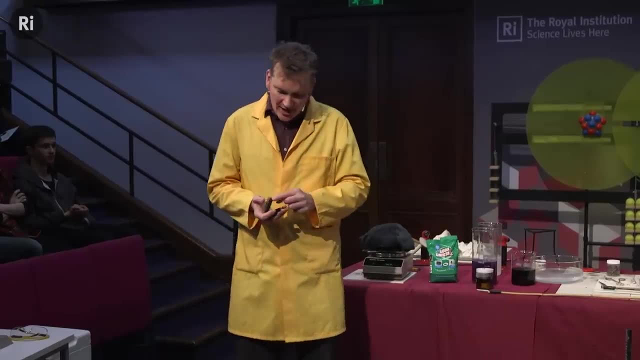 So, I think, a round of applause. thank you very much for your help there. Now, as I say, I will take this outside afterwards and people can have a go for themselves. Please do be careful with this. I say it isn't indestructible. I don't want to test it. 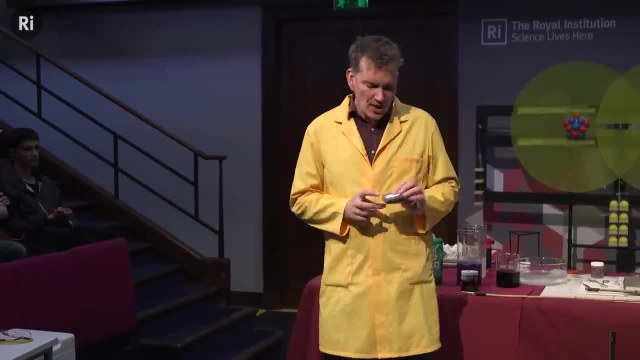 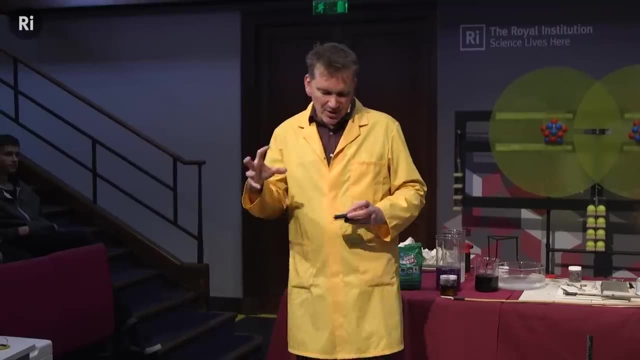 It is extremely cold. It's extremely expensive. This is a synthetic diamond. It's made by a process called chemical vapour deposition, where the carbon atoms are laid down, sort of one at a time, from the gas phase there to form the diamond structure. 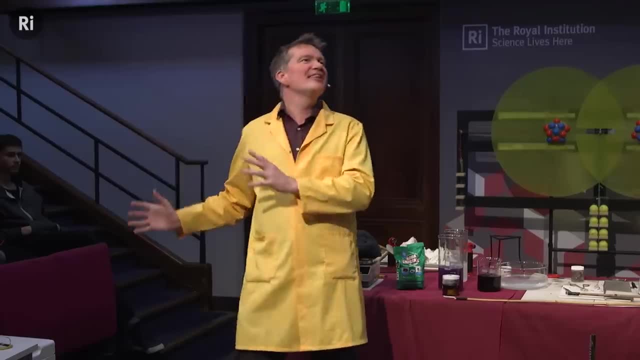 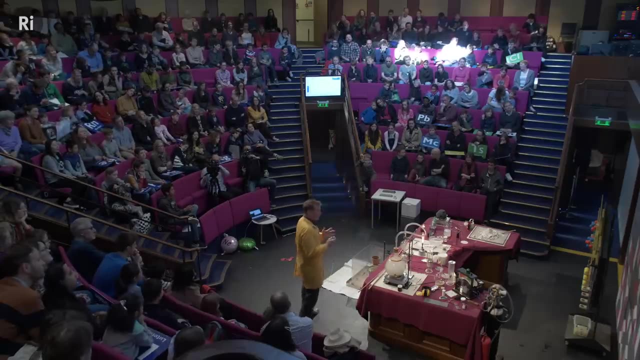 So it's an artificial diamond, but it is a diamond. It is expensive but it is quite remarkable. So do that, have a go with that. So that has the strongest bonding between any of the elements there, the atoms of the same element. 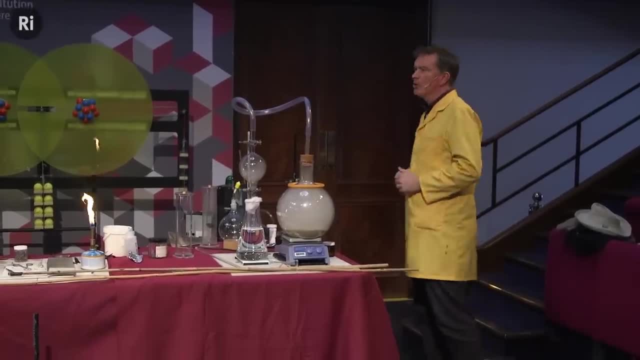 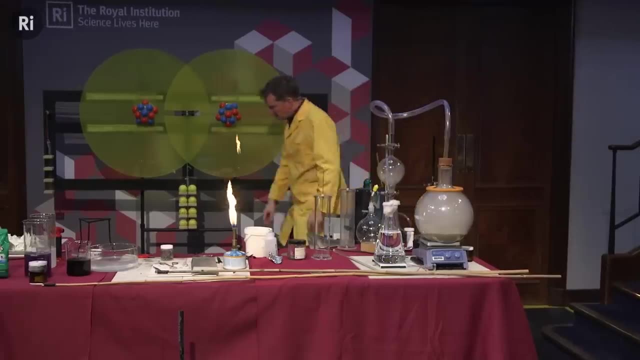 But surely, if we keep on going across our periodic table, we can be adding more electricity, We can be adding more electrons, and the bonds should get even stronger. Well, actually they don't okay. Well, as we move from carbon to the next element, to nitrogen, 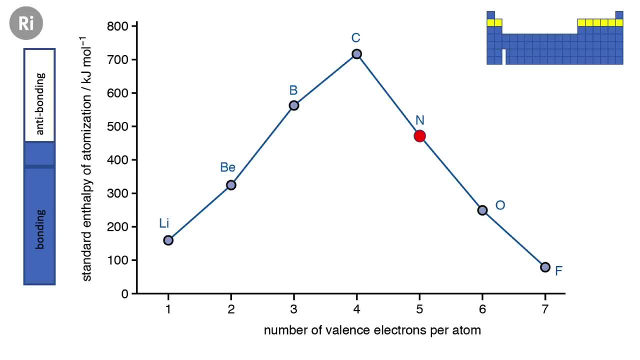 the bonds get a little bit weaker. They're still pretty strong. Remember the formation of, in this case, nitrogen- molecules with two atoms of nitrogen. These are still pretty strong, okay, But they're not as strong as the bonds that we have. 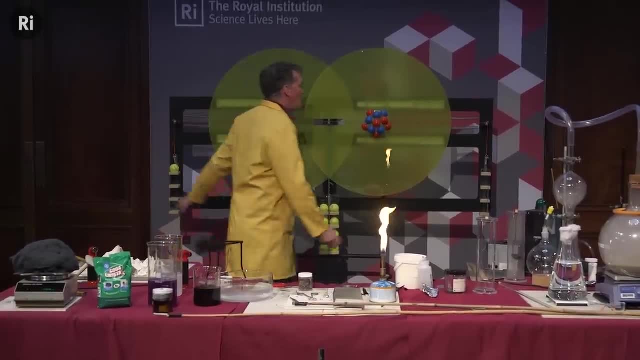 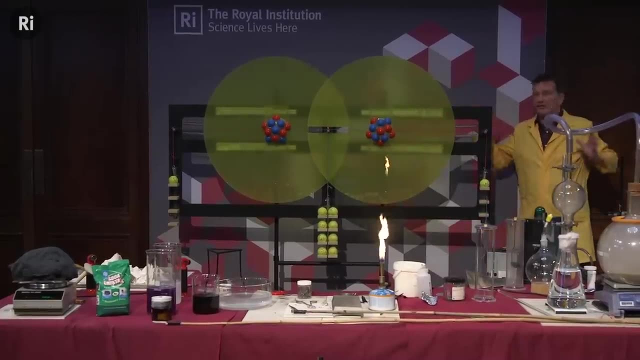 between carbon atoms in our graphite and in our diamond. And this is because, well now, the extra electrons that we have essentially do not go in between the nuclei, They go more outside the regions here, and this begins to pull the atoms apart again. okay, 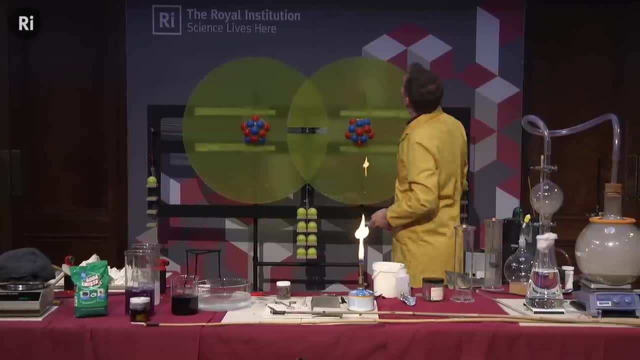 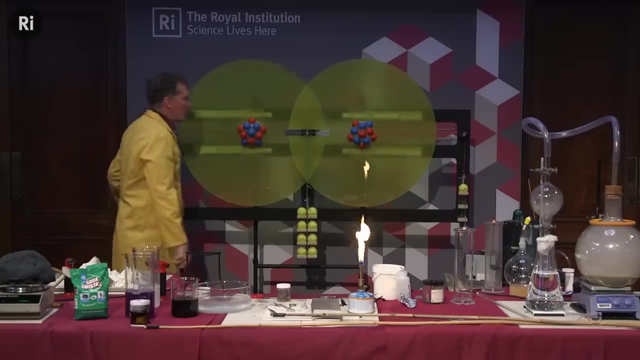 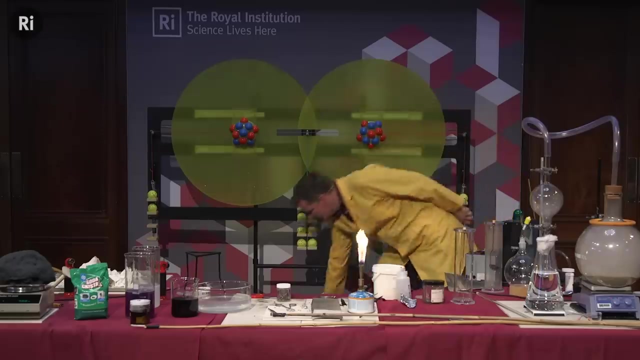 If we go from nitrogen to oxygen, the bonds get weaker still. We have one extra electron per atom And again these electrons now are in regions outside the two nuclei here and they are beginning to pull the atoms apart. We say that these electrons have to go into antibonding levels. 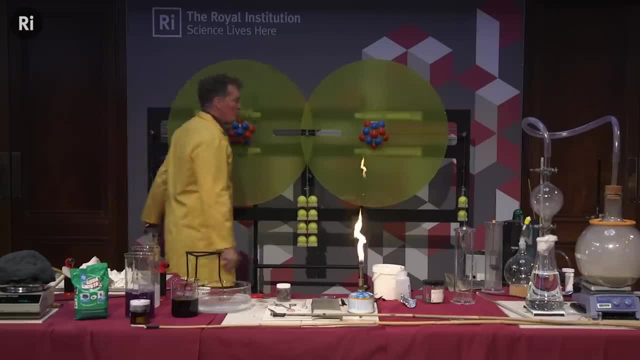 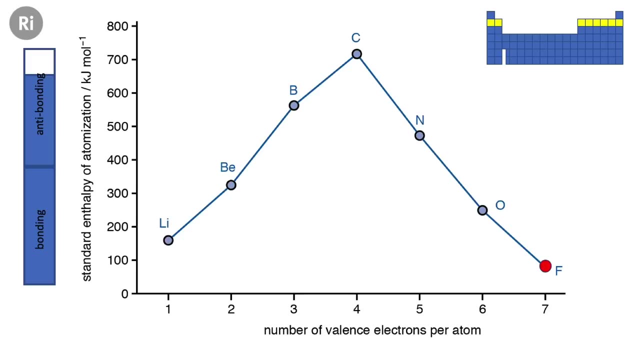 The ones in the middle here holding it all together. these are bonding electrons. We say these ones here are going into antibonding levels, And if we keep on going to fluorine, they're getting weaker still, so almost pulling it all apart. 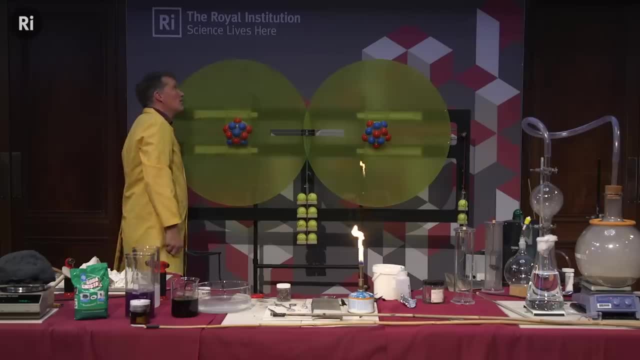 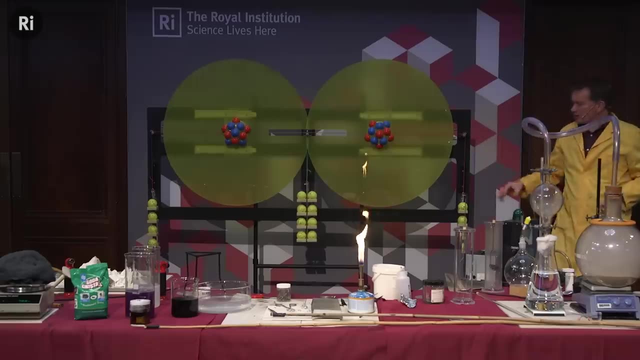 And then, finally, if we went to neon, well, neon has just the right number of electrons that any bonds that we had would be completely more than cancelled out by these electrons. in these antibonding levels, There's no bond at all. That's why all of our noble gases exist as individual atoms. okay, It's because of that. It's because we cannot have any bonds, Because we have too many electrons, we'd form equal numbers of bonding and antibonding electrons. there no net bonding. 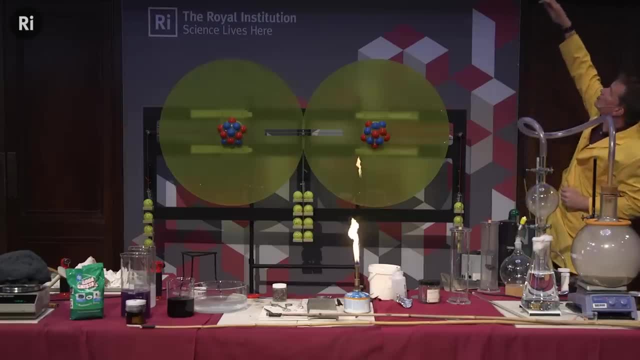 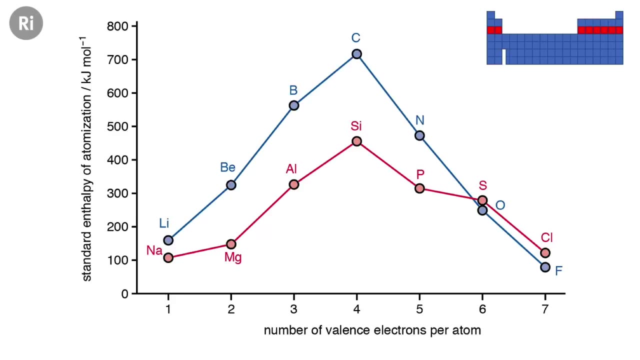 This same pattern when the bonds get stronger and stronger and stronger, and then weaker and weaker and weaker. we see not only as we go across the first row of the periodic table, but also as we go across the next row. so the elements underneath 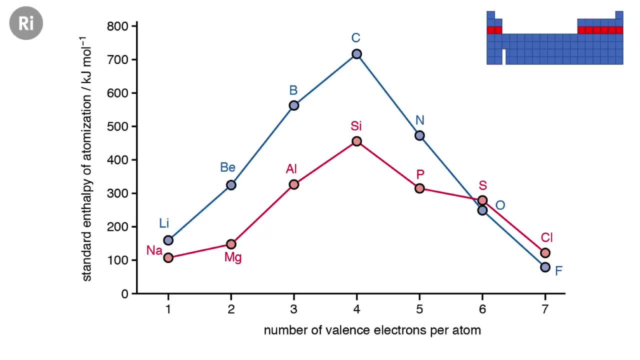 we see again the same spike in the middle for the element underneath carbon. This is the element silicon, and it goes down again. We see the same pattern in the next row, where we see germanium in group 14.. Okay, with the strongest bond. 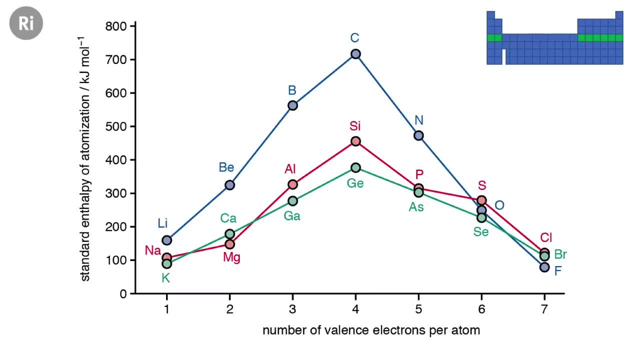 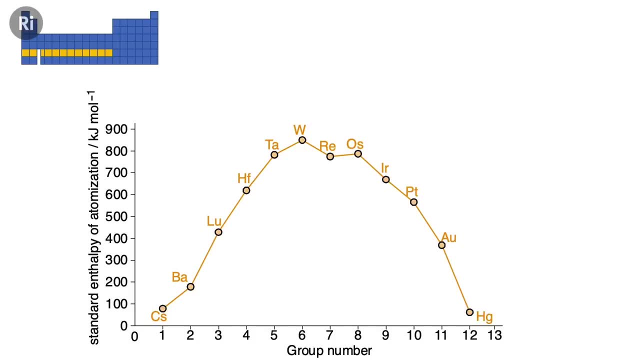 And then they get weaker and weaker again, and individual atoms for our noble gases In fact, remarkably, we even see the same pattern because of the same reasons, as we go across the row with the transition metals. This is our last one, and this is quite fun. 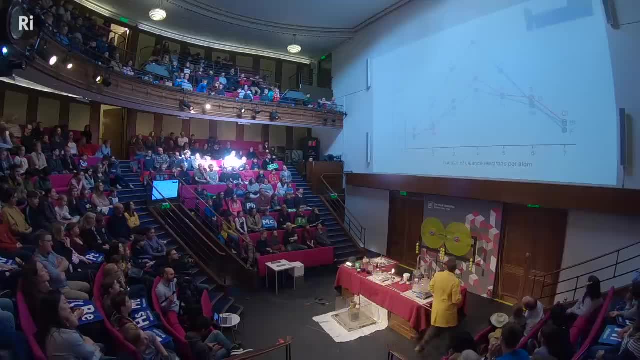 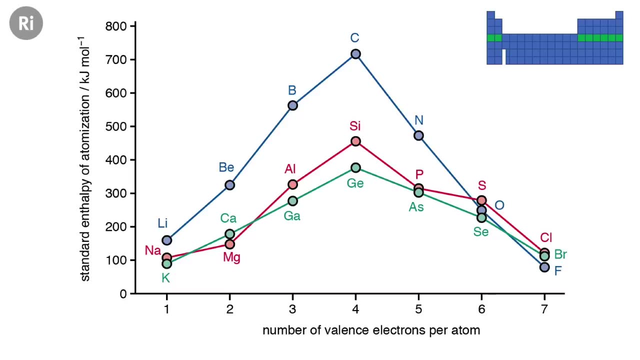 Now, actually, before I show this, I'll just show you a different way of seeing this. So we see the same pattern here. So the bonds with potassium, with sodium, with lithium are all very, very weak and really strong bonds in the middle with carbon. 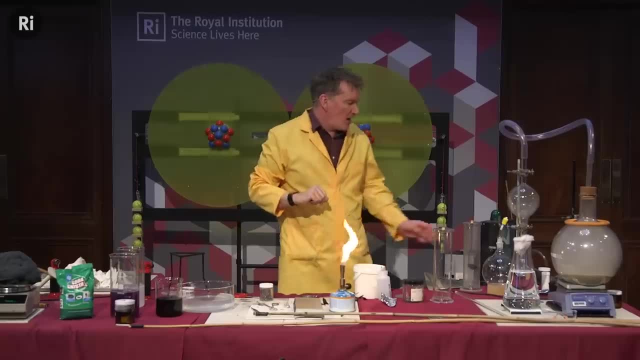 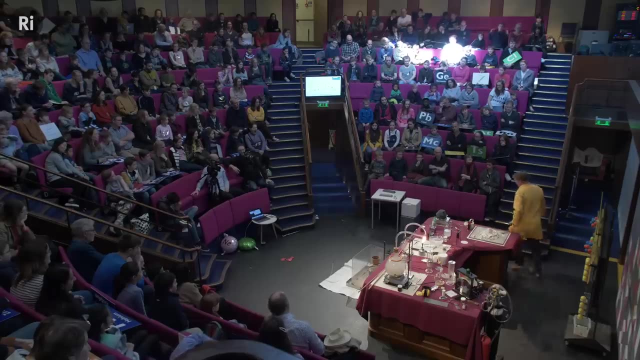 and then individual atoms down the other end, But I can show how weak the bonds are with my group. one elements: Where's my goggles? What have I done? Oh there, Thank you. Yes, All right, I shall just put these on. 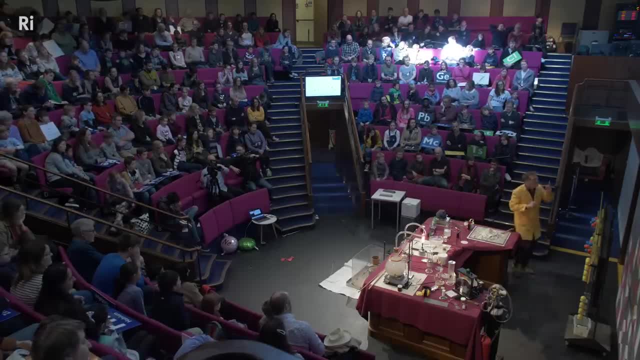 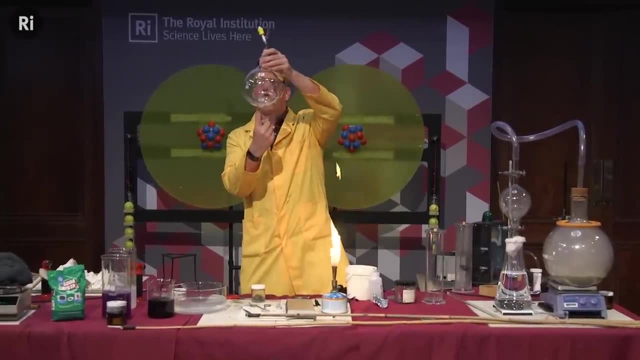 I'm going to show you how weak the bonds are. So remember: the graph here says how much energy is needed to separate these atoms. Well, what I have here is lots of atoms of potassium. So this is a lump of potassium metal, And what I'm going to do is just heat up this lump. 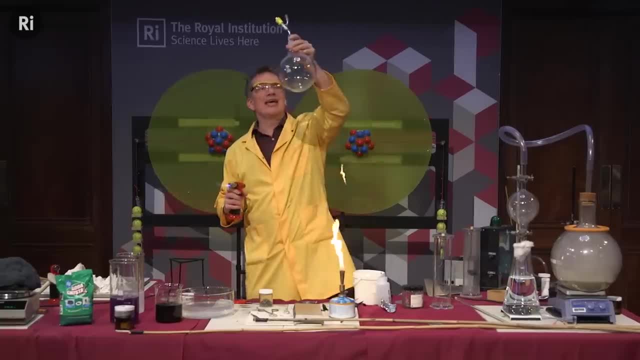 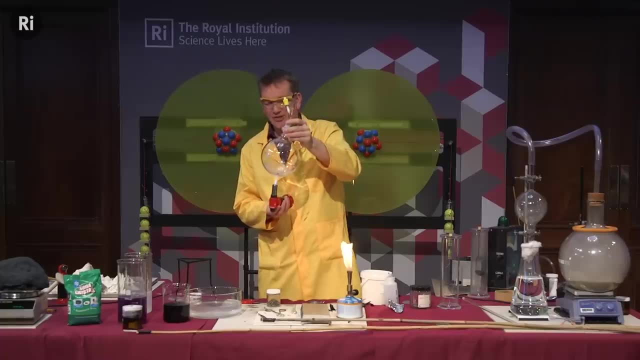 Now there's no oxygen in my flask to react to these atoms, I'm going to heat it up with the potassium, So we've completely evacuated the flask. So it's empty apart from the lump of potassium at the bottom, But I'm hoping that we should be able to see a reaction when. 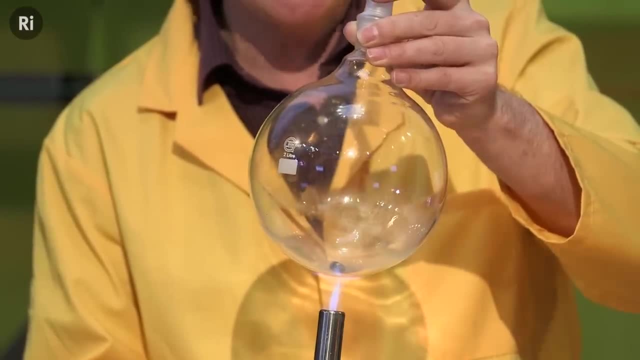 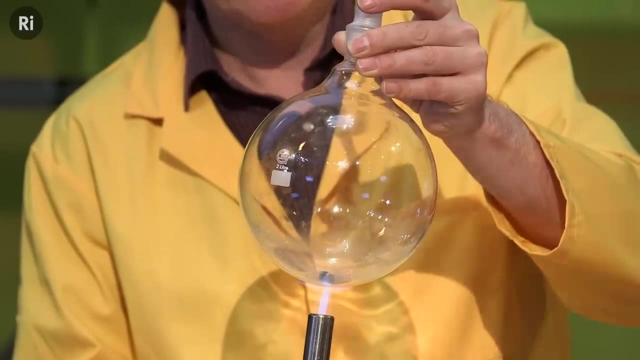 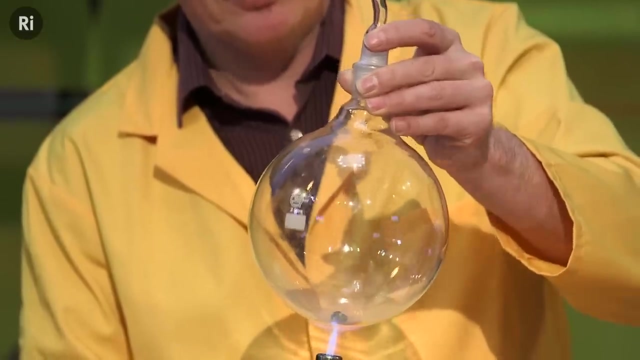 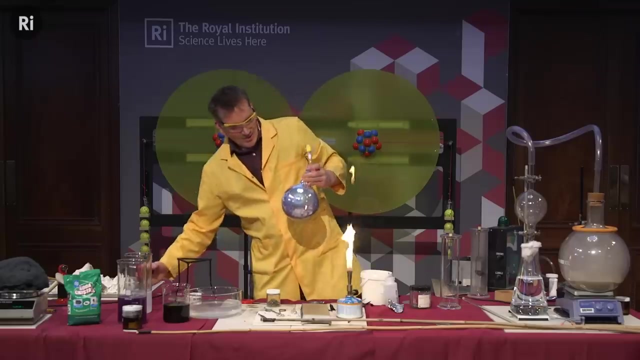 So just heating this up, just warming this, I'm hoping that it should be quite easy to separate the atoms of potassium. So this is what I'm trying to do. So if I heat this up, Hmm, Which is quite fun. So this has now made a potassium mirror. 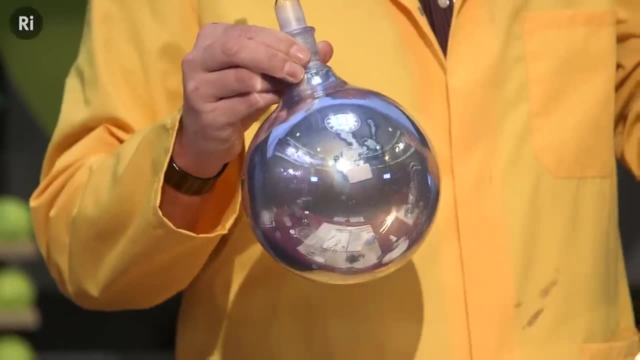 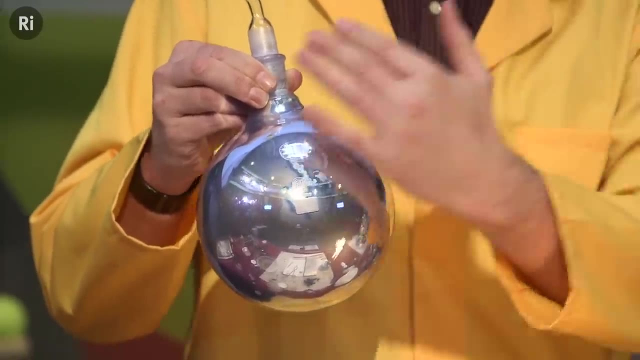 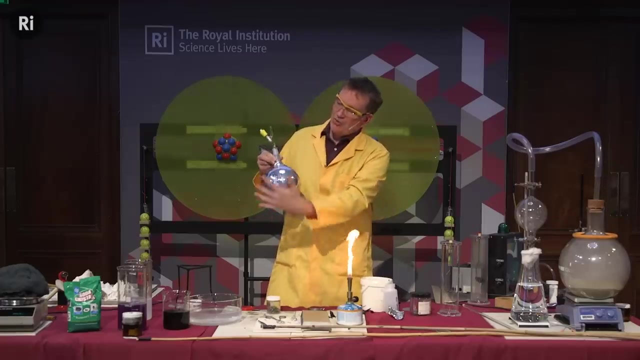 So because it's quite easy to separate the atoms, just by heating this lump of metal up, it easily boils and turns into potassium gas, which is now condensed on the cold flask. There's nothing for it to react with, So it instantly just coats the whole of the flask. 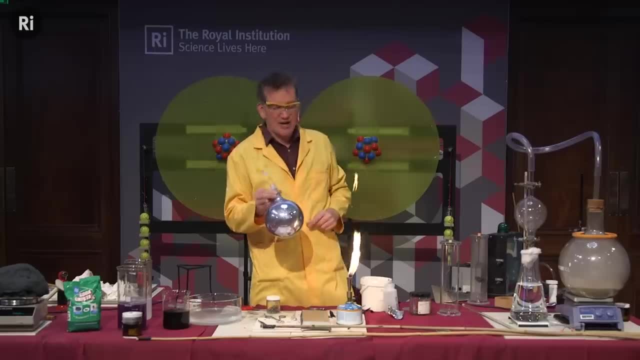 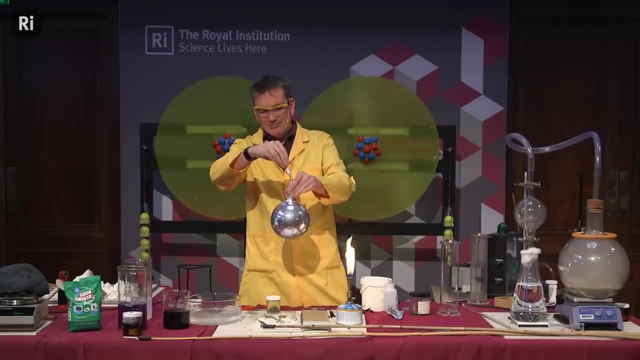 with this beautiful potassium mirror. If there was something for it to react with, it would react. In fact, if I open the tap and let some oxygen in, it will gradually react with some of this And you see, it's already losing its colour there. 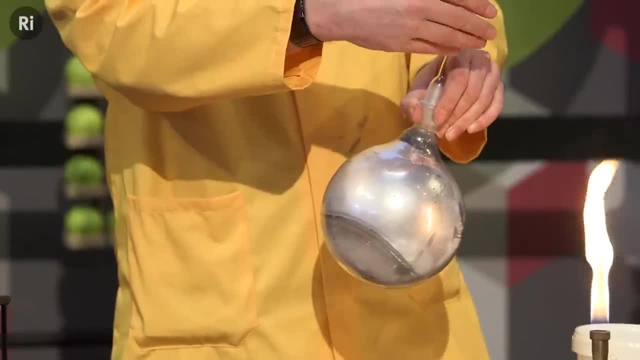 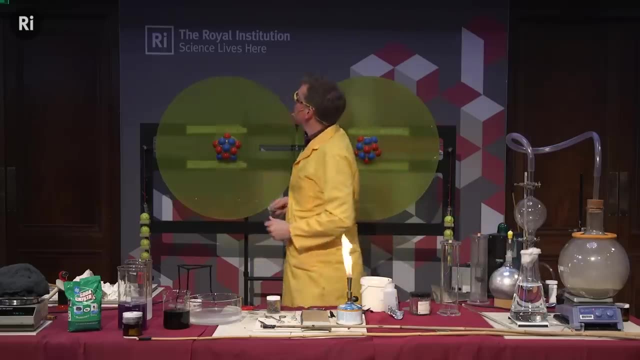 and it's forming the white potassium oxide there as it's reacting with some of the oxygen from the air. So, but a beautiful experiment there. So easy to pull these atoms apart, But, as I say, as we move across one of the last four rows of the periodic table. 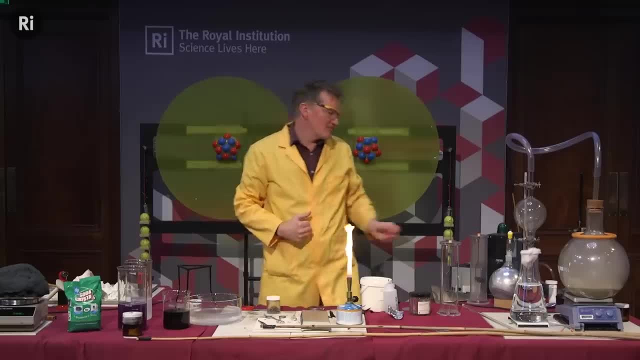 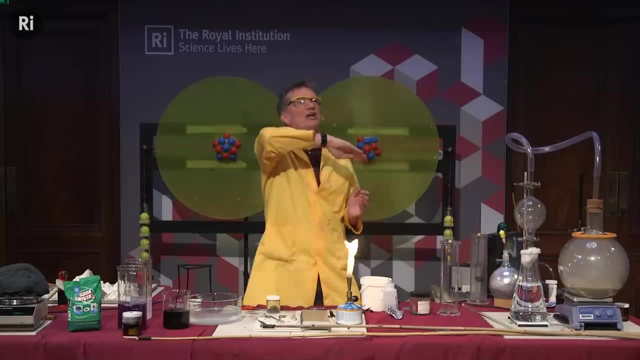 we see the same patterns. It's easy to separate the atoms of caesium. I could have done that, but caesium is even more reactive and it's more expensive. So I could have made a nice caesium mirror. And as I go across, we're putting electrons into nice bonding levels. 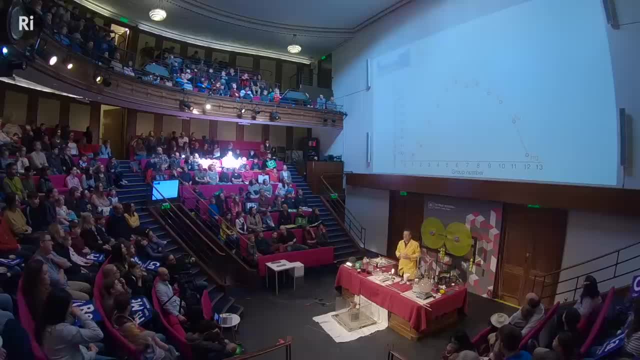 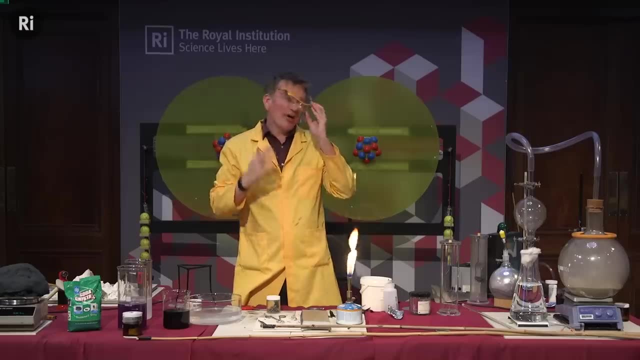 We get really really strong bonds in the middle with the element W. What's W? It's tungsten. Oh good, Yes, very good, OK, so tungsten. OK, Actually, when I said carbon has the highest melting point, boiling point. 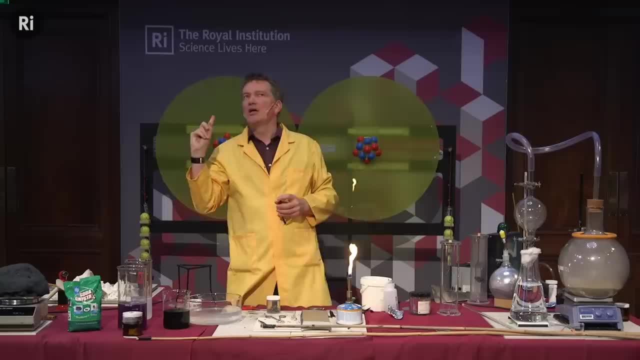 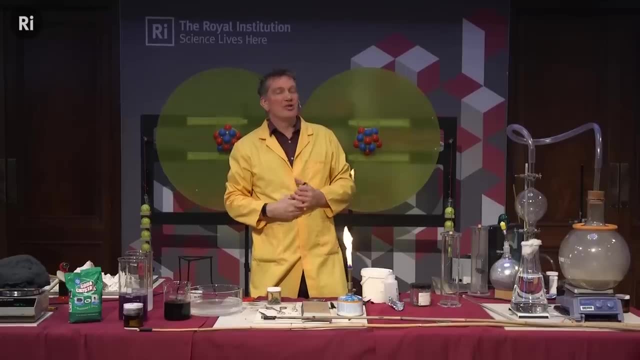 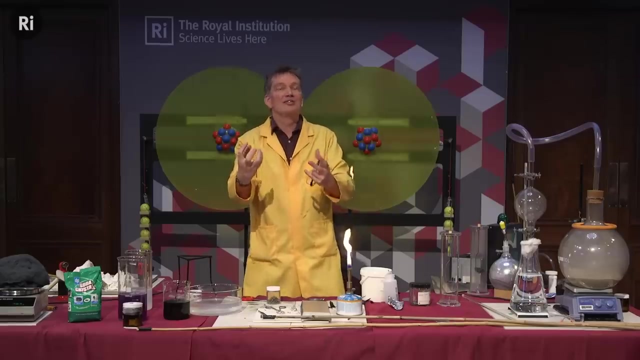 perhaps with one exception. Well, this one exception is tungsten, And this is why tungsten used to be used in the filaments with light bulbs, Because you could heat it up to really high temperatures and it didn't melt or boil, So you'd get it white hot to give out the light. 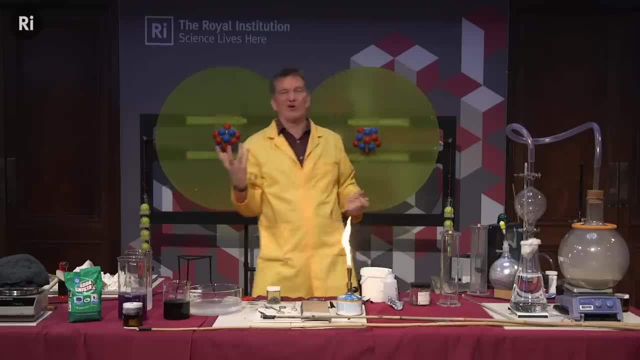 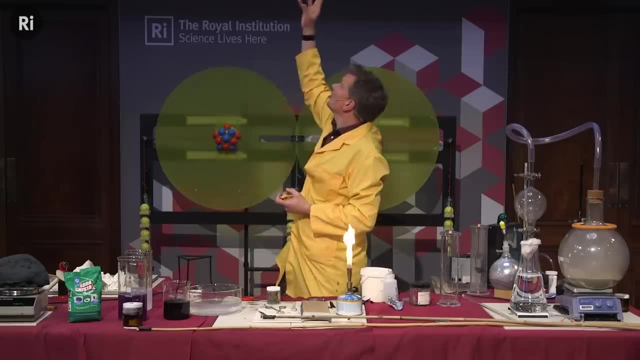 Not very efficient, of course, because it's also very hot. It's white hot. This is why now we have much better light bulbs that are energy efficient. of course, these light emitting diodes So tungsten the highest melting point, boiling point. 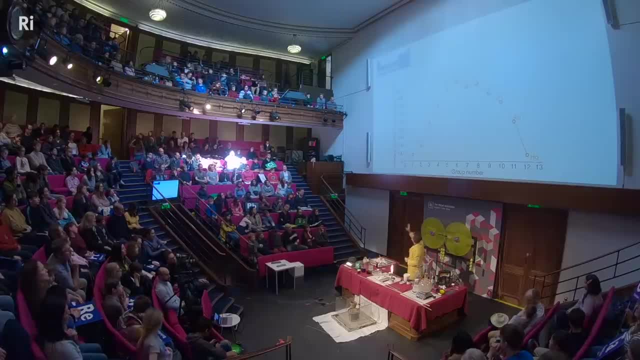 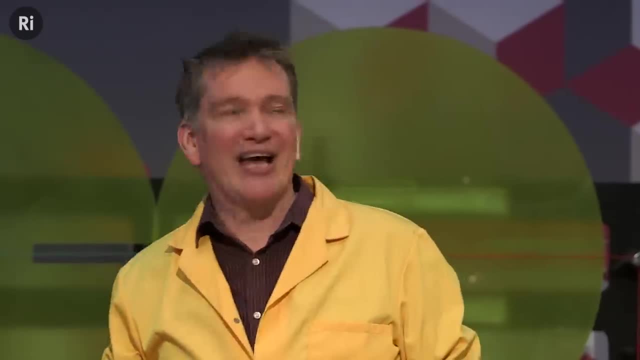 perhaps between that and carbon. it's very difficult to measure, But if you keep on adding electrons, well, these end up with the bonds getting weaker, And this is because, essentially, we are beginning to put electrons into anti-bonding levels. 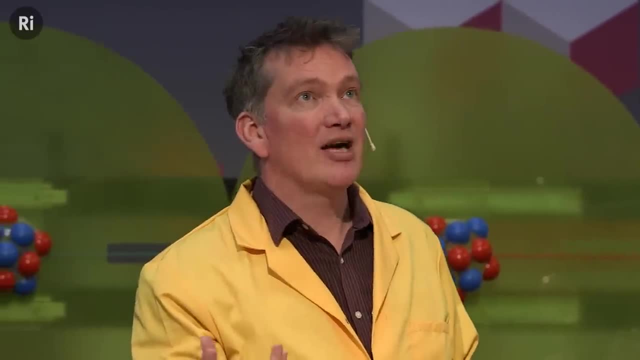 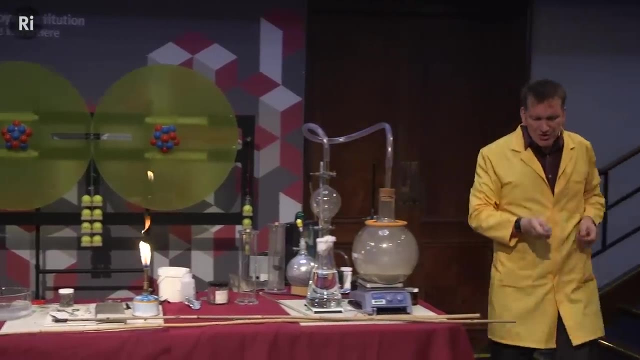 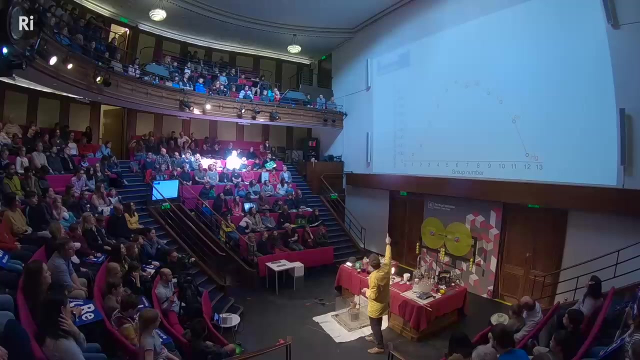 And mercury is a liquid, OK, And it's very easy to turn it into a very poisonous mercury vapour. Now, this actually has one other interesting consequence, And this is with the density of these atoms, The density of these elements, So as I move from one atom to the next, 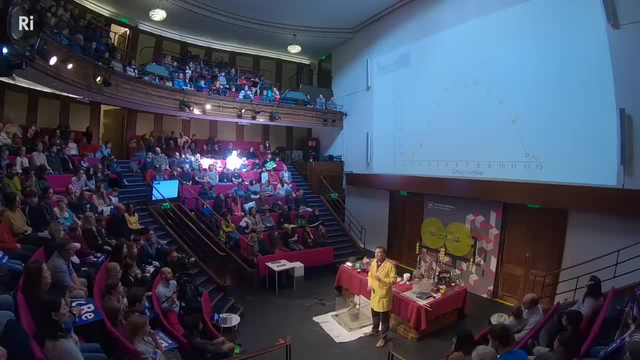 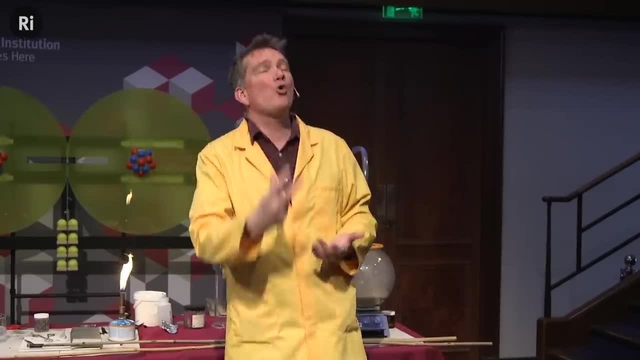 remember, as I'm going across from one atom to the next, we're always increasing the number of protons by one and increasing, maybe, the number of neutrons and the number of electrons. So the atoms are always getting heavier as we go from one to the next. 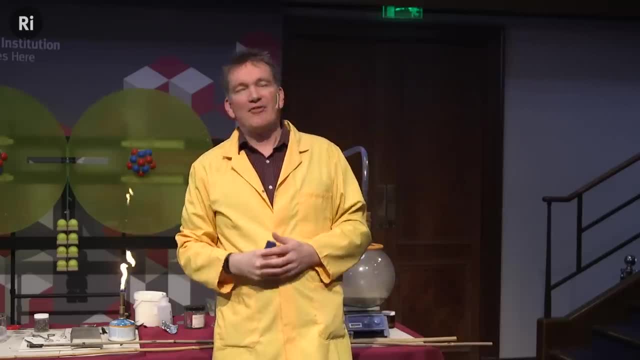 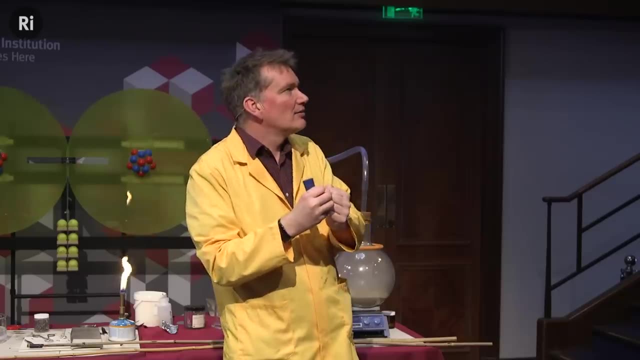 But what about the density? So the density of an element depends on the mass of each atom, but also on how closely they're all packed together. So tungsten has the strongest bonding here. So actually we see a slightly interesting curve with the densities. 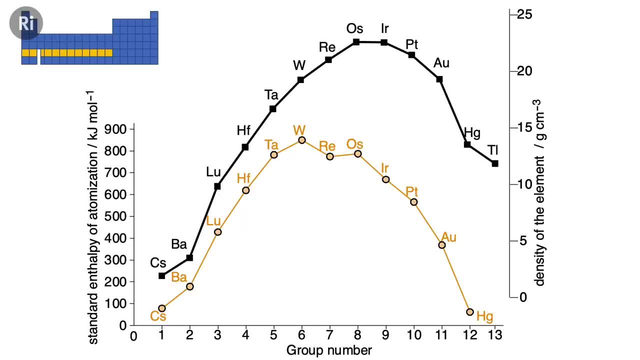 So even though the masses of the atoms are getting heavier, this is showing the density of the solid. There's a slight lag. So it turns out that actually osmium and iridium are the most dense ones. There's still pretty good bonding and the atoms are getting heavier. 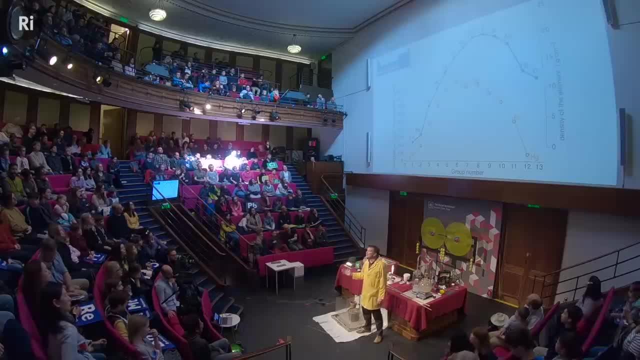 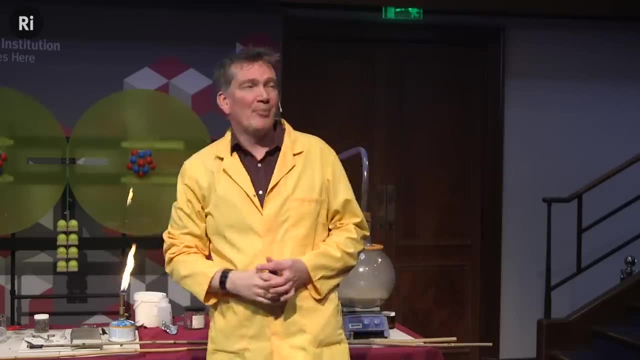 But even though the atoms continue to get heavier because the bonding isn't so good, the density goes down again. It turns out that gold, AU and tungsten W have about the same densities, And this is really pretty heavy. 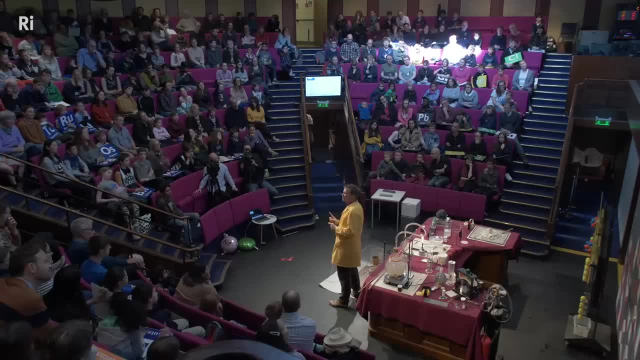 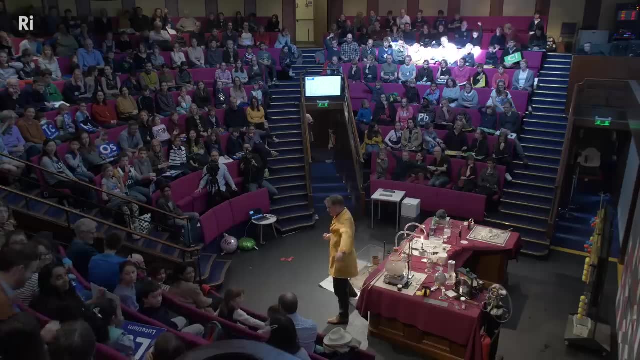 And I need a very strong. maybe someone wants to volunteer, maybe their dad, somebody really strong. Oh, I see somebody's hand went up there. That's good, So right. If you could come down to the front please. 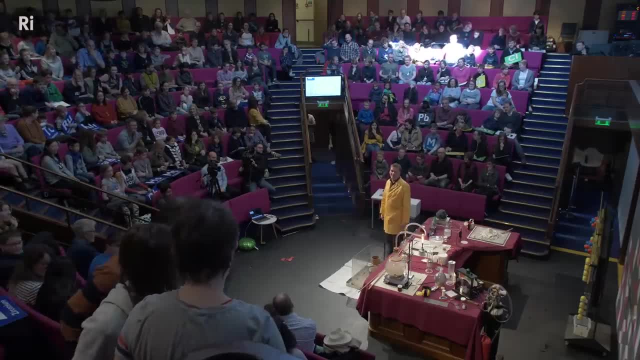 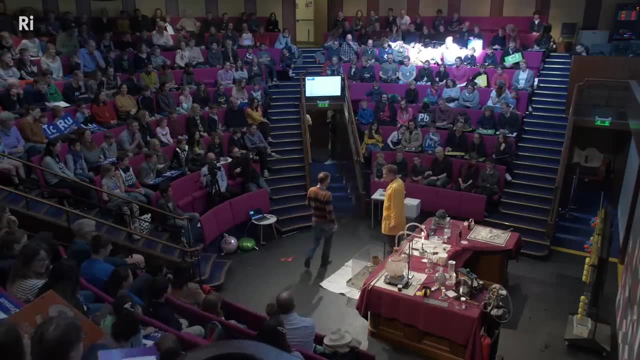 We'll see how strong you are. This could be embarrassing, couldn't it, Anyway? So what I'd like you to do, please, is just pick up the bar, the close bar to me. One hand, no sliding. One hand, no sliding. 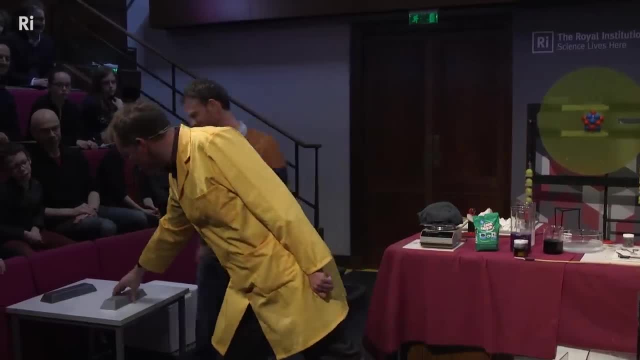 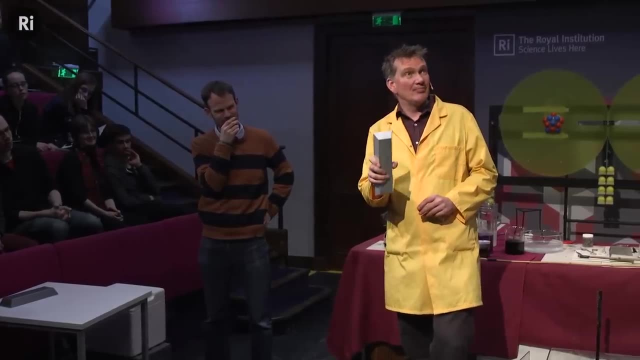 Oh, there we are. Actually, it was very easy, wasn't it? So this actually: oh, don't do that one yet. This is incredibly light. This is solid. It is solid. It's actually made of magnesium. This is even lighter than aluminium. 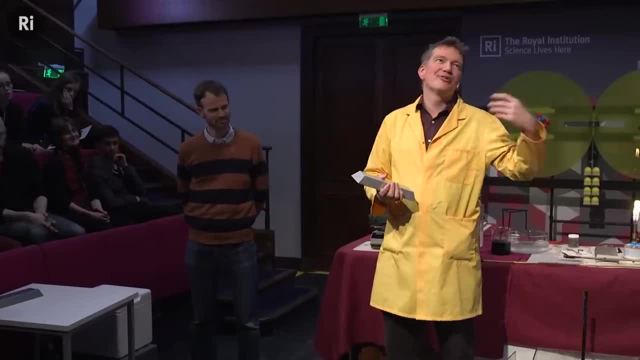 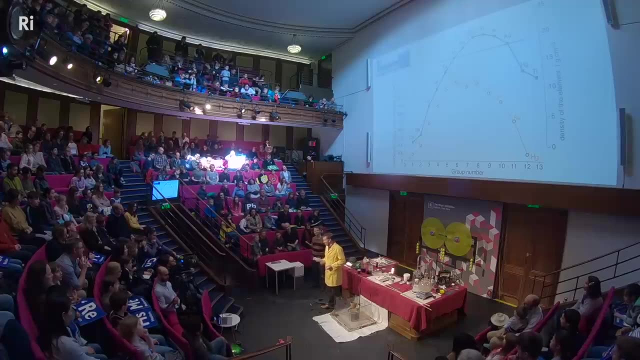 It's one of the very early elements in the periodic table. Not many protons, neutrons, electrons per atom, Not particularly strong bonds. They're quite large atoms. It's really very, very light This one. we have more protons, more neutrons, more electrons. 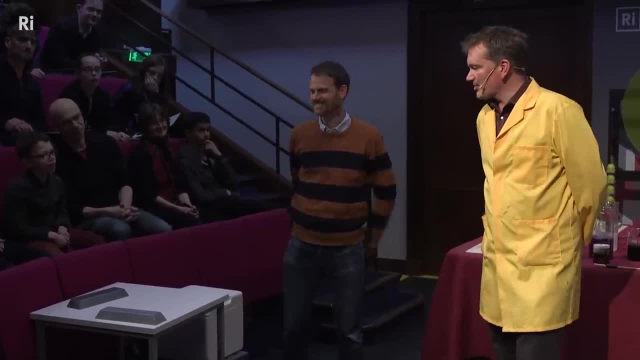 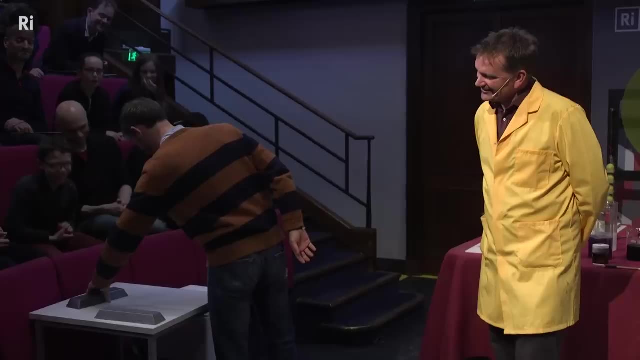 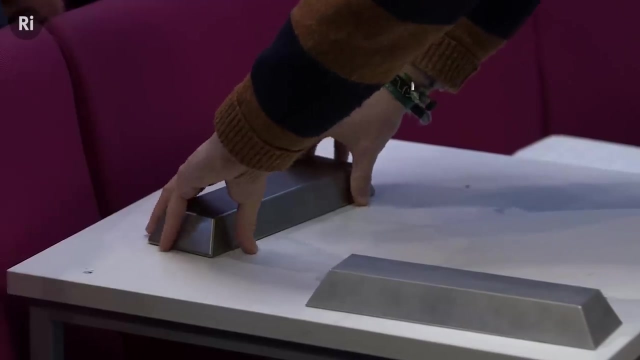 better bonds, smaller atoms. Can you try and pick that one up for me please? One-handed, no sliding, Oh, go on, then You can use two hands. Actually, it is. Actually it is possible with one hand. 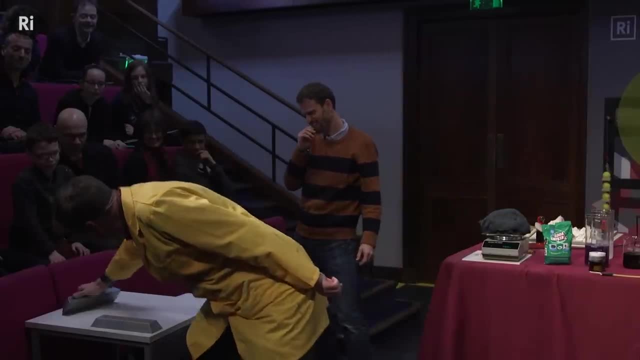 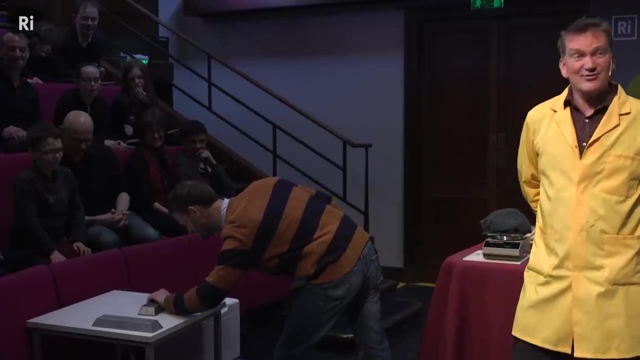 Shall I demonstrate? Yeah, So you can just about. If you're good, you can like that. There we are. Do you want to give that a go? Now? you know how to do it. It is really very heavy. Now you should. 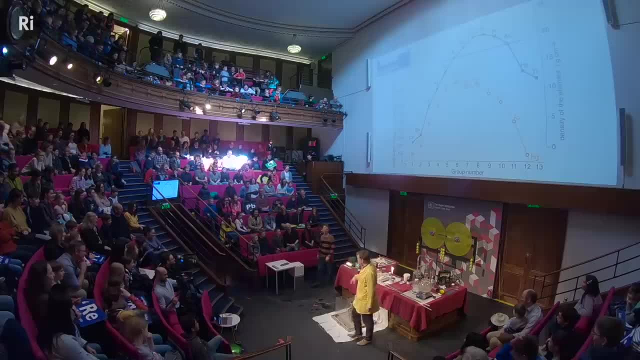 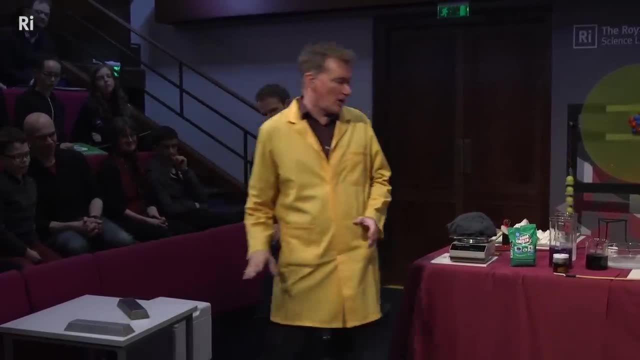 OK, You should try this for yourselves. later We're going to take both bars outside Now. this was completely unfair of me, by the way, because A- I've practised doing that, but B- we've made these the same size. 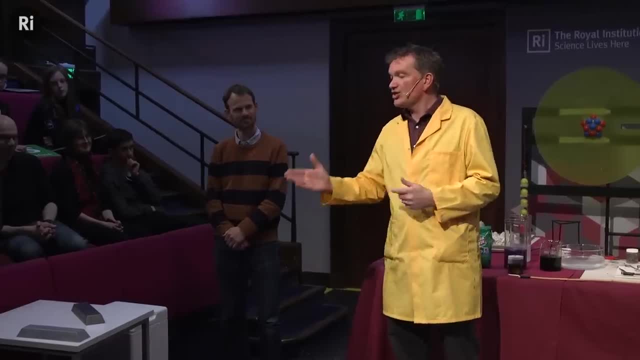 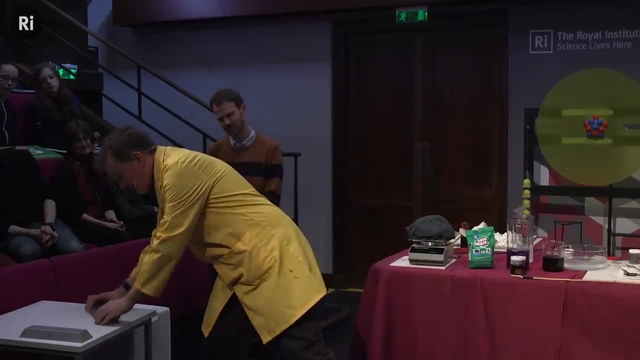 as a pretty standard bar, Gold bar- OK. So this is what a gold bar feels like, because tungsten and gold have the same densities, OK, And it really is quite heavy. So I mean holding this, if you. 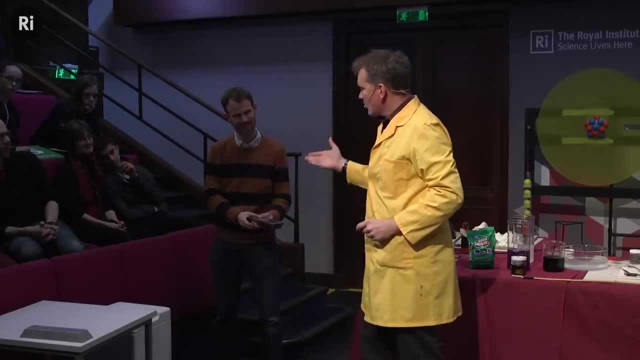 We'll have a go later with everyone. So it really is quite heavy. That's the same. That is what a gold bar feels like. You couldn't run away with many of those, could you? OK? But the other interesting thing is: 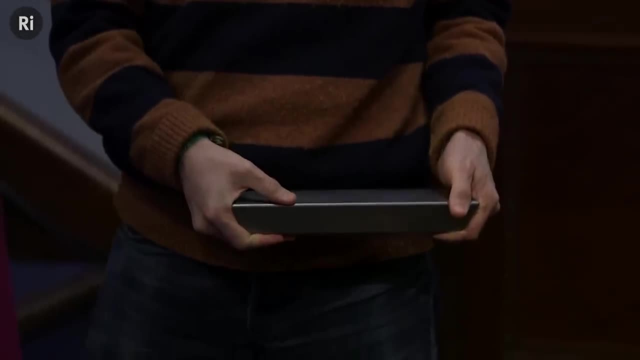 in all the films that you see, apart from the fact that they're clearly not gold bars, because they really are very, very heavy. Remember, in one of the James Bond films, he has it in his pocket and it slides down. You don't. 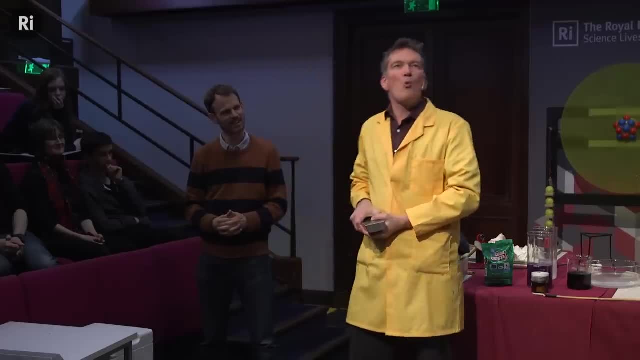 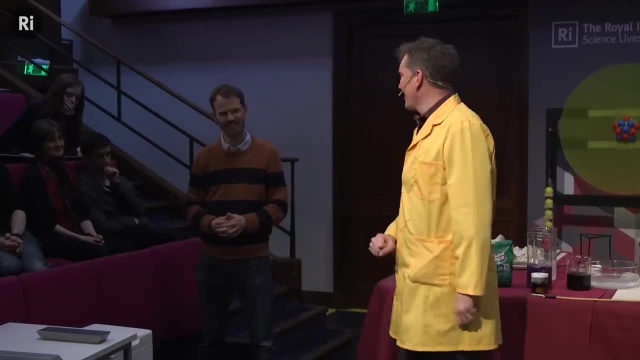 I don't think you could do that very easily. But they always put the gold bars the wrong way up in the films, So they ought to be this way up so you can easily pick them up with one hand. You can do this on now. 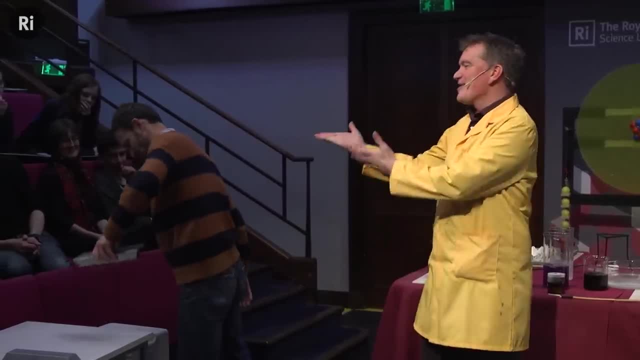 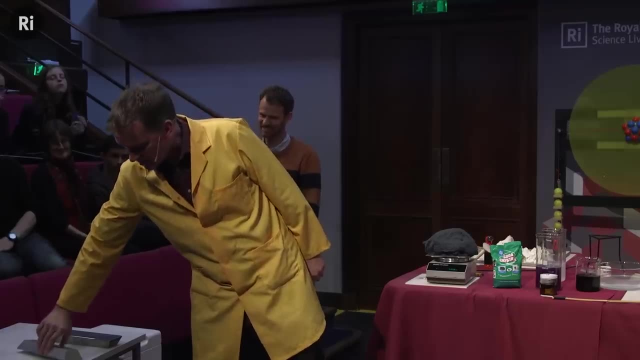 Go on. Yes, yes, There we are Round of applause there. Yeah, OK So, And this way it really is not a sensible way to have them, So that's why they're meant to be that way up. So thank you very much for that help there. 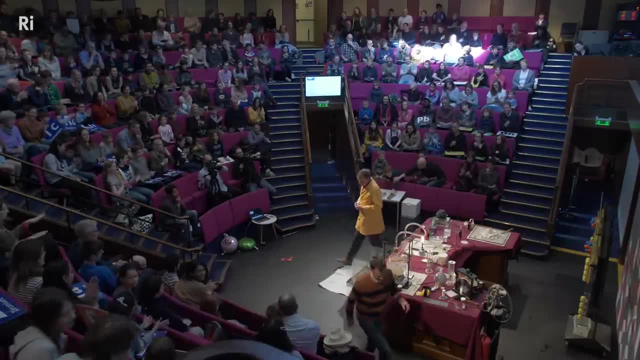 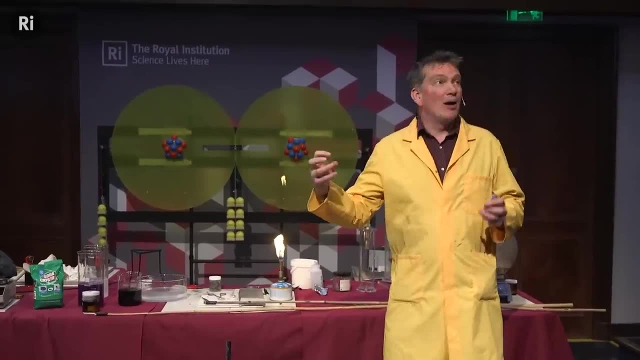 OK, Um, A second question. OK, Tungsten and gold have pretty much the same densities, which is why some very naughty people have actually drilled out the gold bars, some gold bars, and put in tungsten instead and then covered it with gold on the other end. 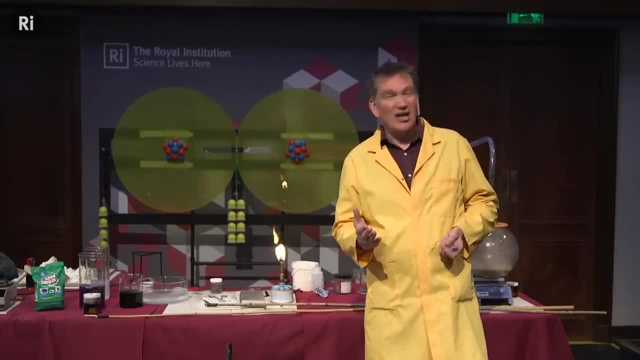 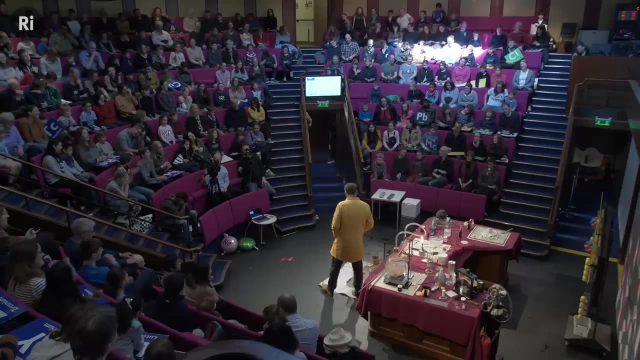 And you can't tell because it has the same density. Only by chopping into it can you see. You can't X-ray it because you can't see through it, So don't, I'm not giving you ideas here. But anyway, so tungsten gold, the same density. 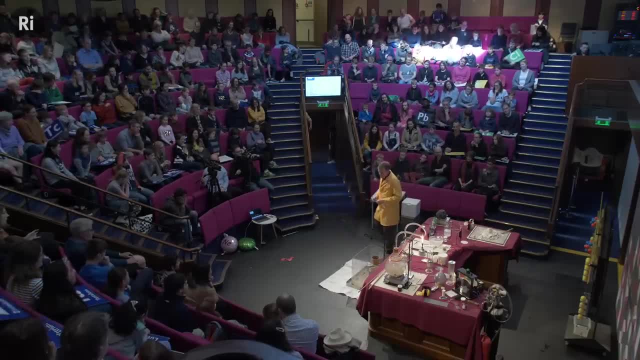 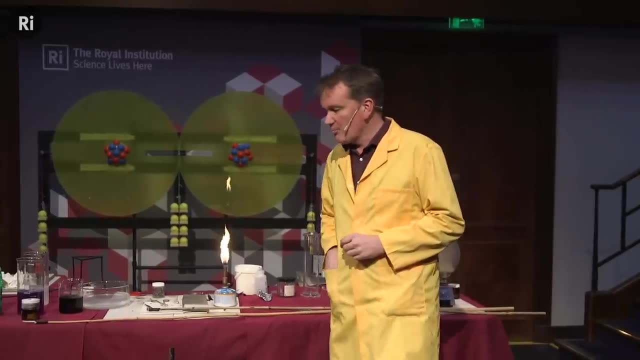 So do have a go with our afters. We will take this outside for you So that it won't be too busy in here. Well, that just about brings me to the end of the lecture. I hope you've enjoyed this. I hope you've had a fantastic time. 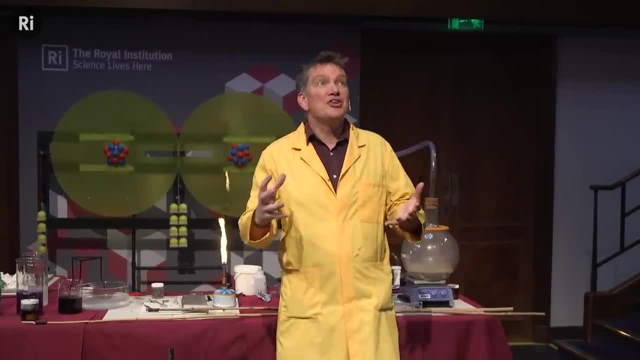 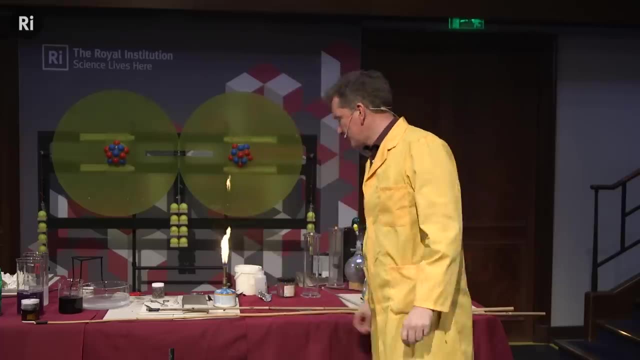 I think before we go, we should maybe look at the most abundant element in the universe, element number one. This is hydrogen. So where are you Up there again? So we're going to look at hydrogen one last time before we go. 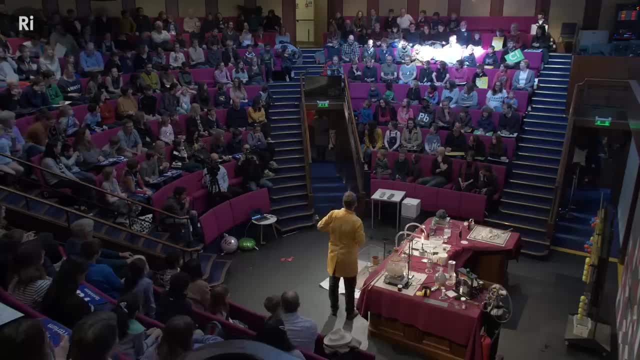 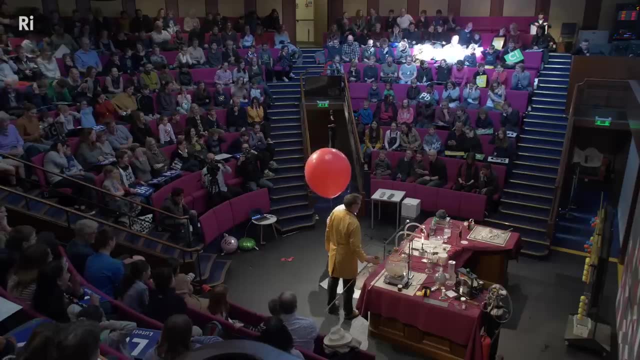 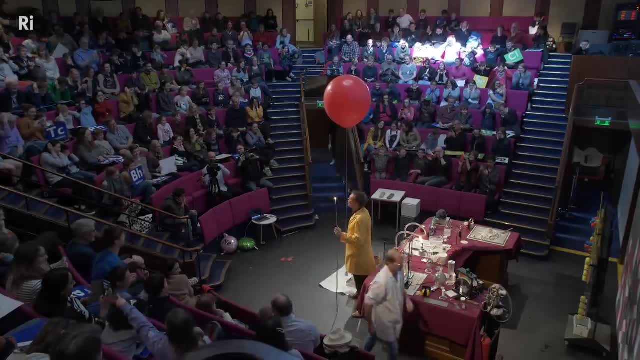 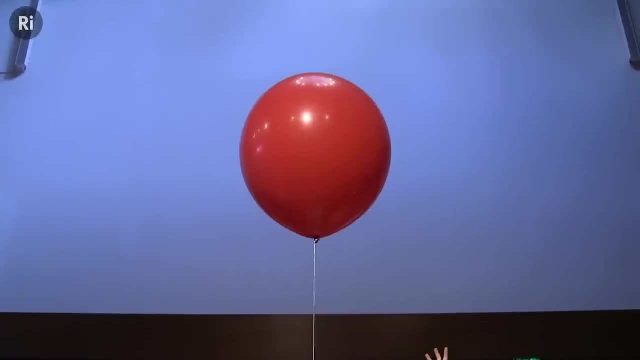 AUDIENCE LAUGHS. Okay, so we do have one more hydrogen balloon. I should just say so this: There's no oxygen inside the balloon, okay, So it's not going to be a very, very, very loud bang, So you should be okay. 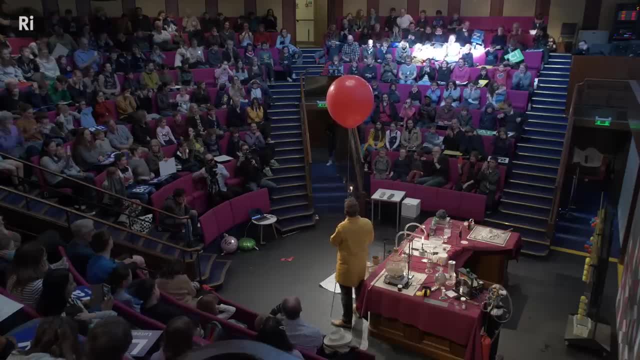 You don't need to cover your ears. If you don't like loud bangs, please do, of course, But you will be okay. But you should. I'm hoping that you should all be leaving with a nice warm glow, okay.